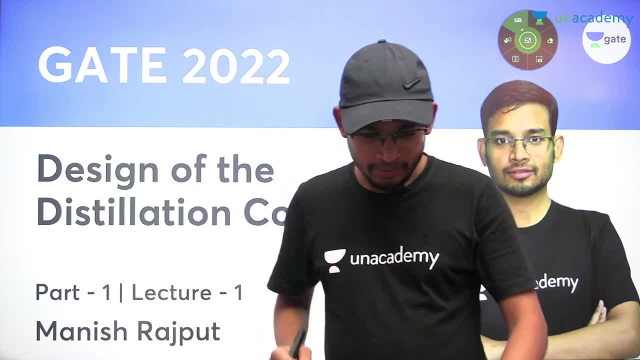 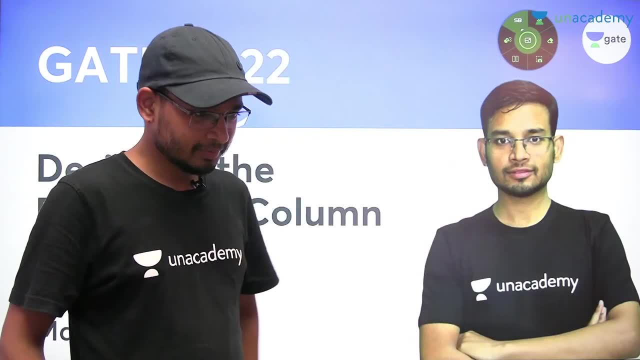 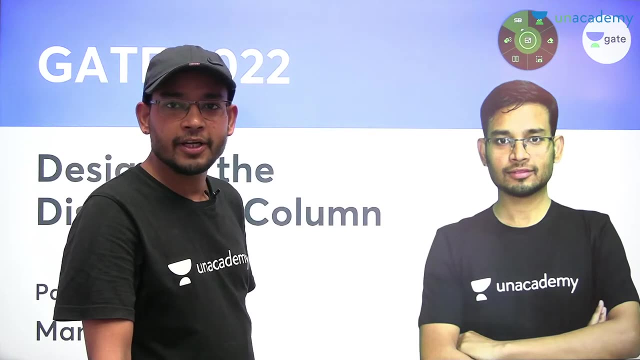 and video are clear. yes, audio and video are clear. hmm, ok, yes, ok, so this is the same lecture. yes, this is the first lecture of designing of the distillation column. ok, this will be our first lecture, ok. 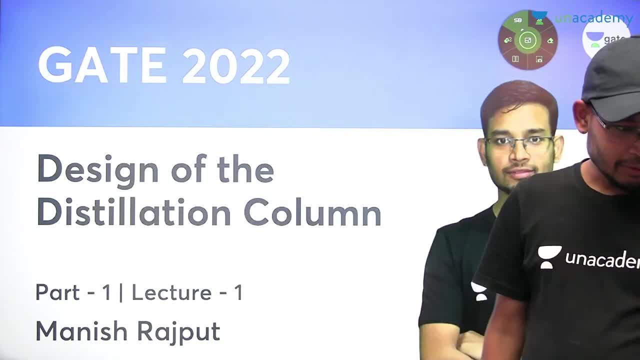 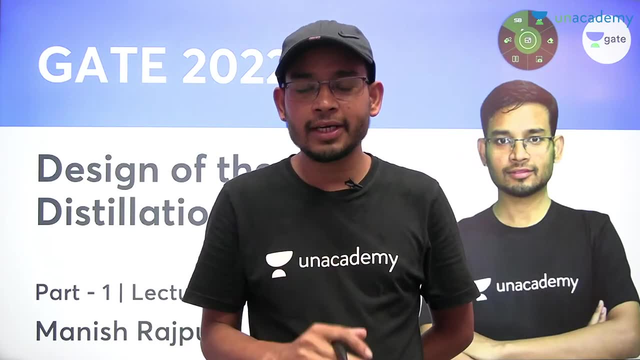 So you will share the session so that maximum people can join. ok, clear, ok, our gap of three to four days was done, which was our one o'clock class. you guys completed the IPC completely last time. then I gave you a time of three to four days so that you can. 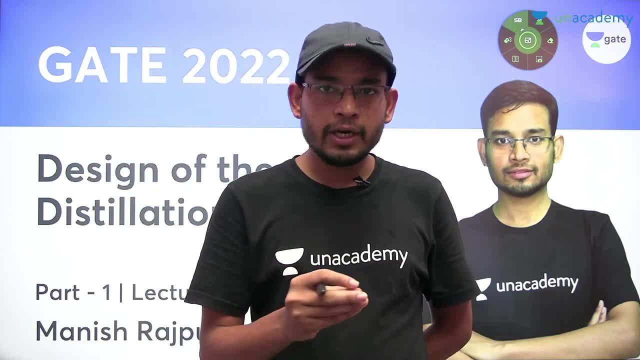 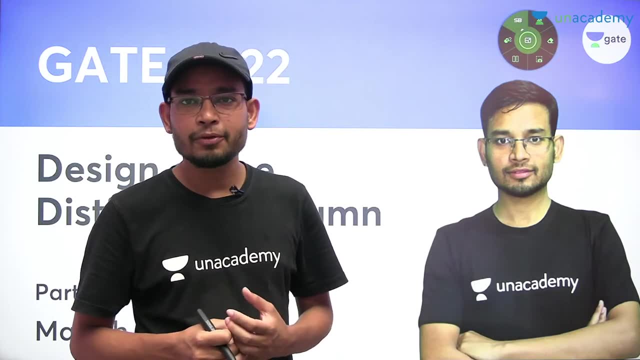 do revision on your behalf and can ask questions on your behalf and those who have not done it. we have started the revision session. some people had a demand that sir bring the revision session so that whatever IPC you have read, it should be revised properly and 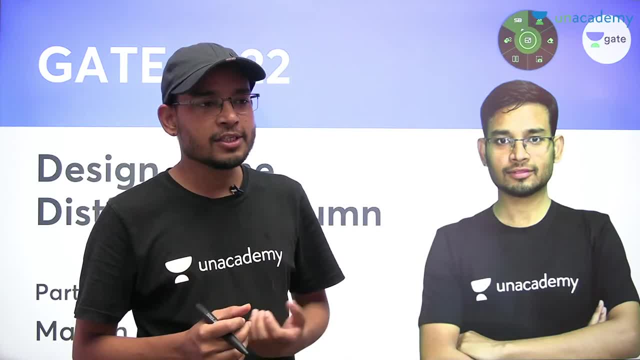 we have started giving test series and so on. So on that basis, a revision session of the IPC has been started. and tomorrow it was 11 o'clock in your night, today morning it was 10 o'clock. daily your class will be at 10. 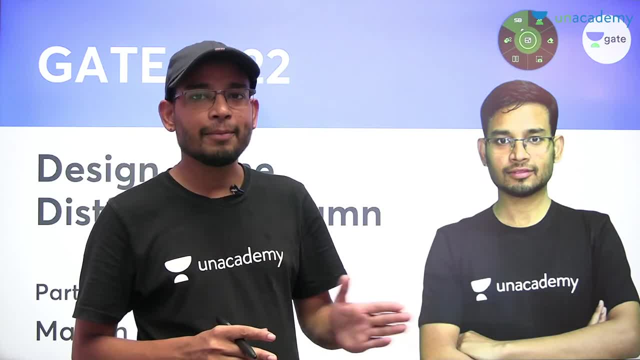 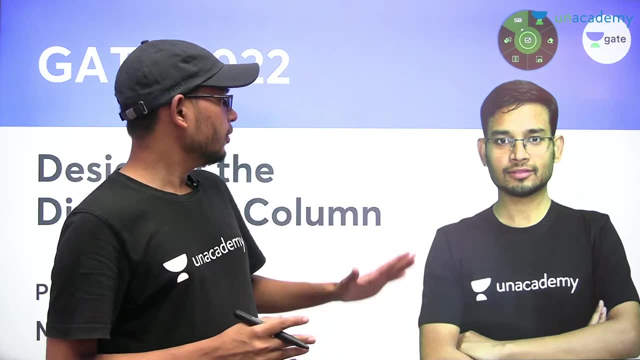 o'clock tomorrow. there may be a shift at 9 o'clock in the morning. ok, I need a good time so that I can finish the revision part of you in a short time. ok, come on, so let's just talk from. here will be a design of the distillation column, so this is your first. 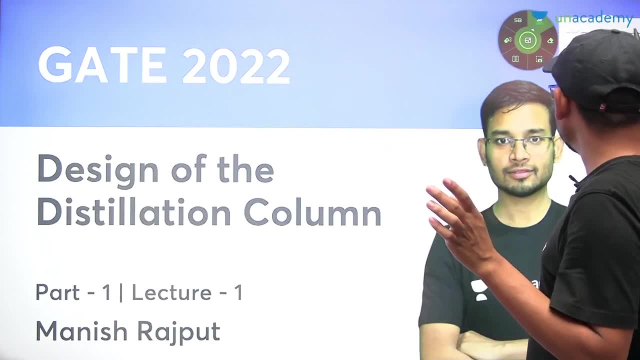 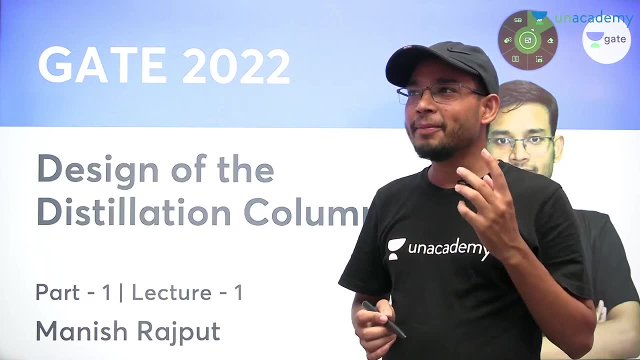 lecture: ok, this is the first lecture of the designing. ok, this lecture was pending since many days. you guys talks on a second plate. it is very good, this is our first lecture. ok, I had told my students that I am going to bring the session very soon on designing. 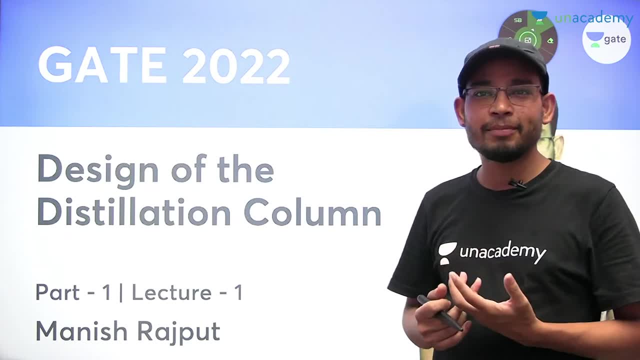 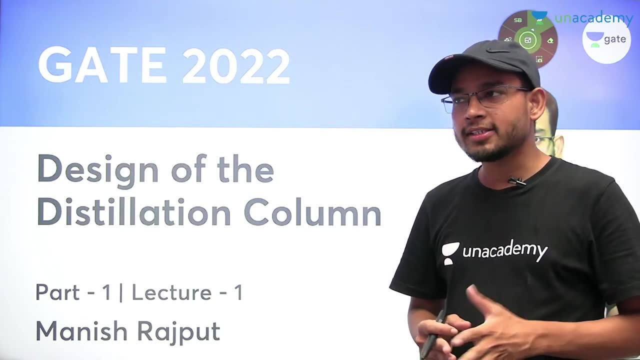 Since then. I have never got time in between, because the objective is always to complete the syllabus. But now both your subjects have been completed properly In six months. it took six to seven months. both the subjects have been completed properly. Now I would like to talk to you a little bit accordingly. 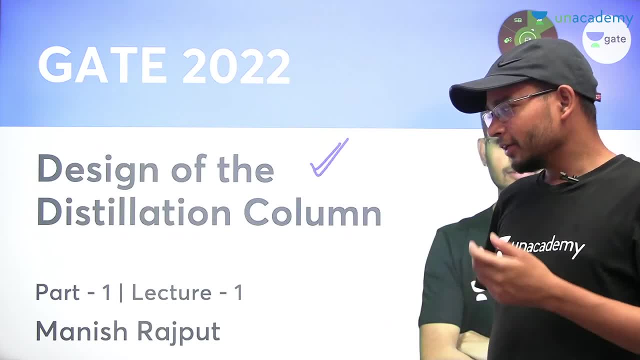 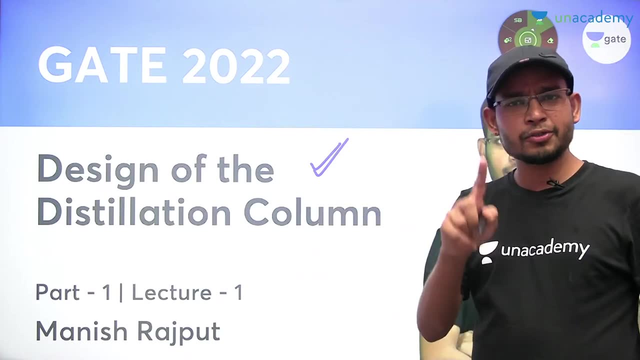 So this designing part was pending for many days. So many students of distillation were also saying that, sir, bring this Now. the written of your bar has been done, So there will be some shortlist for the bar. We will go to the interview. 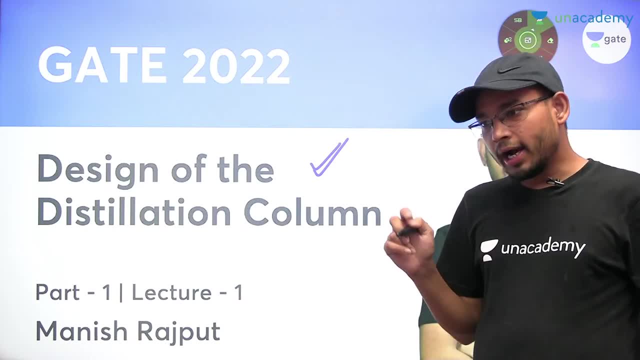 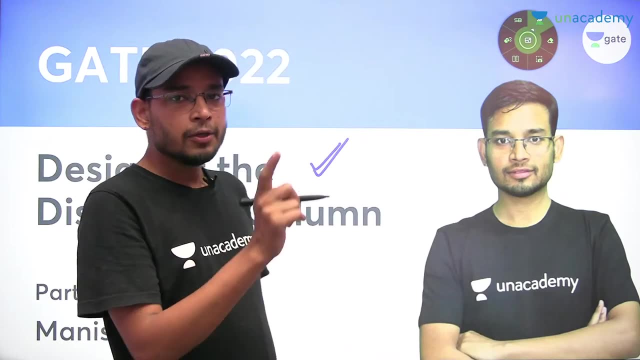 The written of NRL has also been done. We will also go to the interview in NRL. And now you will also go to the ONGC and IOCL- Those who have the gate score in 21. So their shortlist has not been done yet. 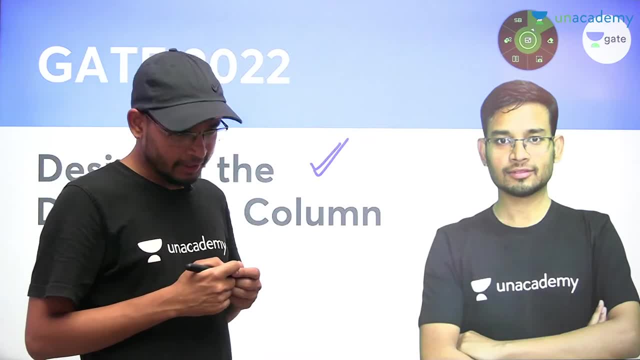 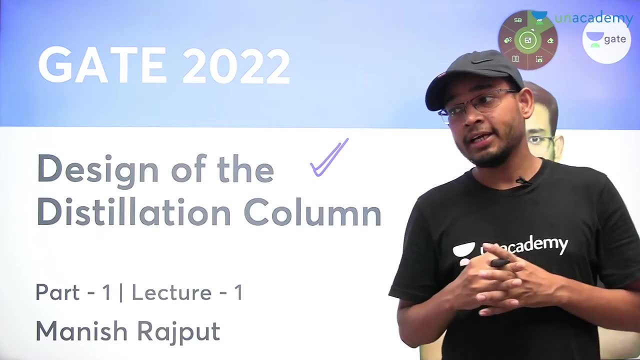 So these people will also go to the interview now. So this is helpful for all the people And probably ISRO will also come this year, as soon as possible. So the shortlist of ISRO is done. Yes, The shortlist is done on the basis of this percentage. 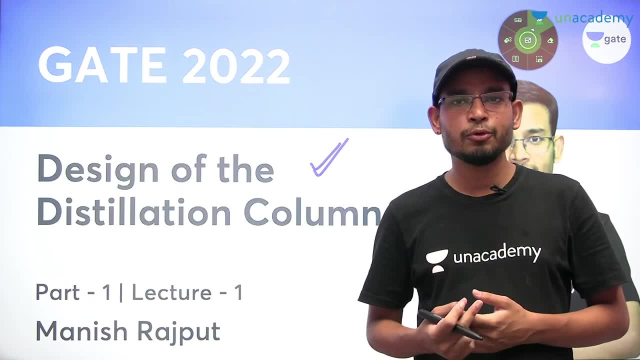 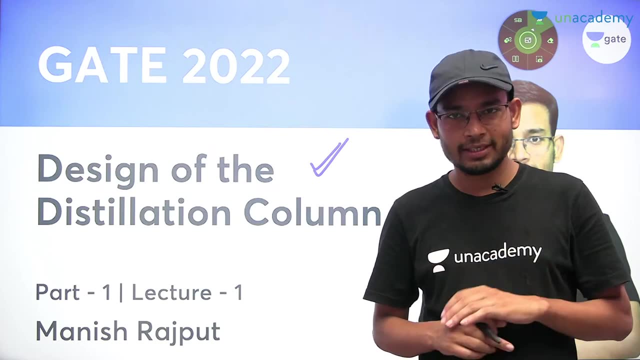 And some of your ISRO have different exams. So there are some exams where they get tested, So where the shortlist is done directly, then they talk a little properly in the interview. ISRO and BARC are two such interviews where they want a little technical sound from you. 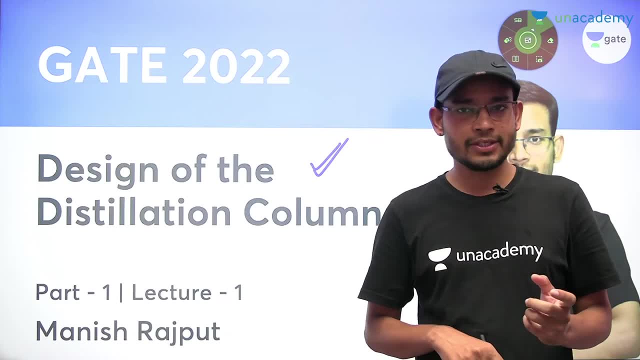 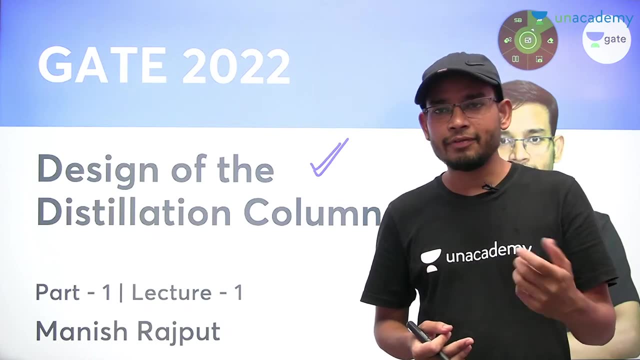 That, whatever candidate I select, it should be a little technical sound. Okay, Yes, If you go to PSU, then the gate's 85% budget is done there. The matter is of 15 marks And 15% is done. 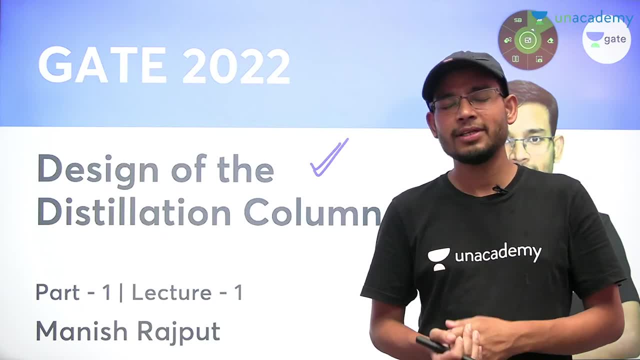 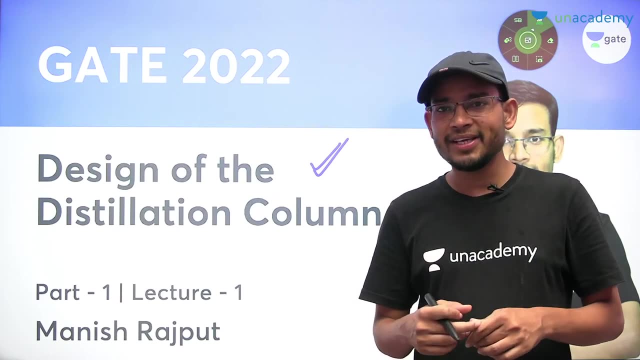 So in that they judge your personality and then give it directly, In that most of you are not out Because it is a matter of 15 marks, But in a place like ISRO and BARC, where NPCIL is there, whatever research organization it is, 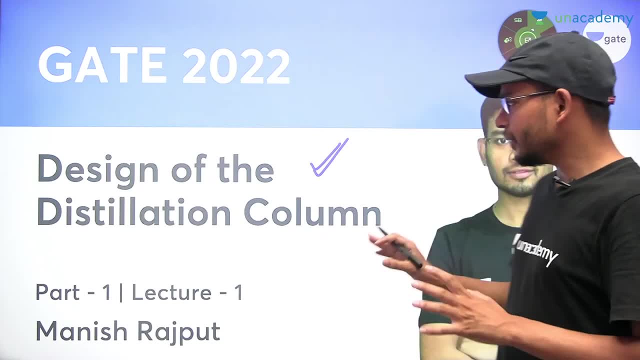 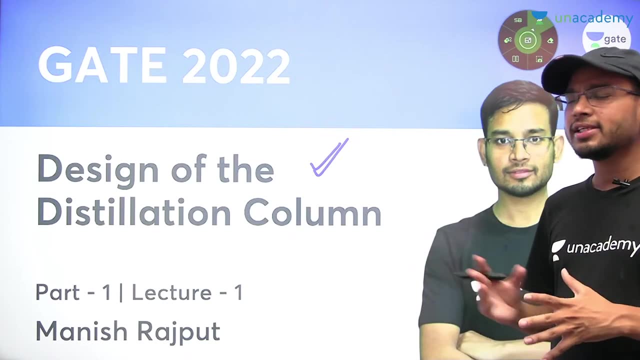 it is very important to have a little technical sound there. Okay, So from today we will start designing of the distillation column. I will complete this in your four to five lectures, But whenever you complete it you will never have any problem in it. 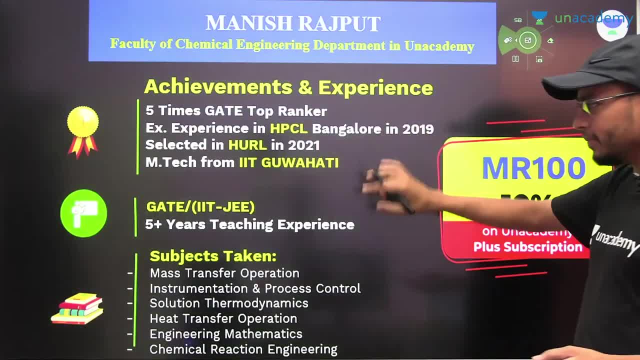 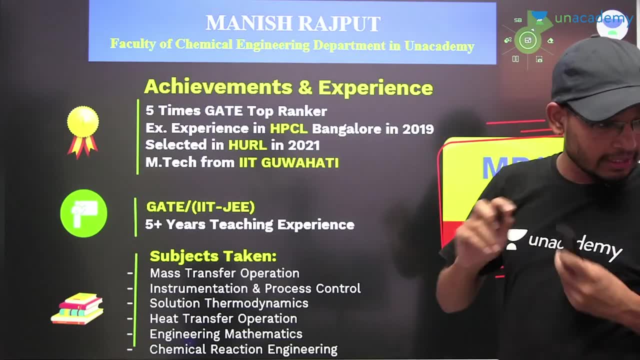 So we are going to talk about it in detail. Okay, So let me just start from here. I will tell you about my new students. Yes, So let me see your comments first. Something like this: Yes, Everything is perfect, Everything is clear. 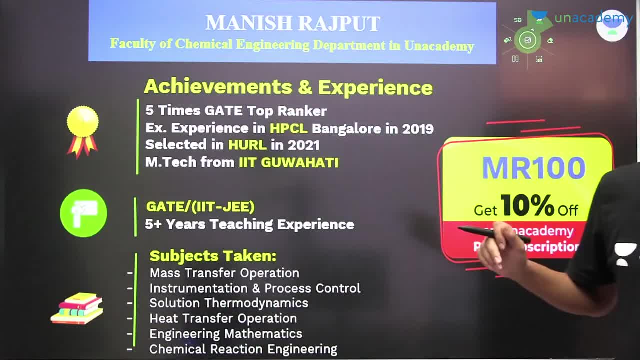 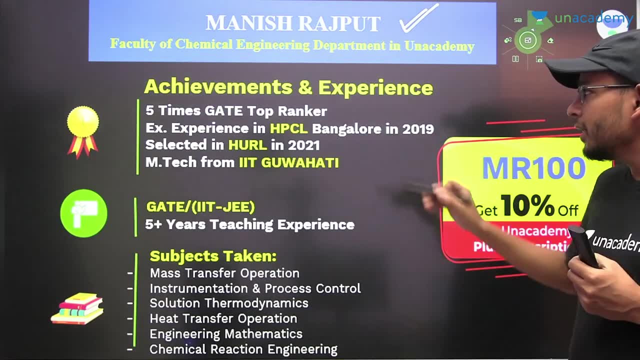 Solution Thermo will start on YouTube from when? Okay, Just wait, Come on Now. I will just talk from here, So those who are joining on their platform for the first time. So my name is Manish And here I will just talk about achievements and experience. 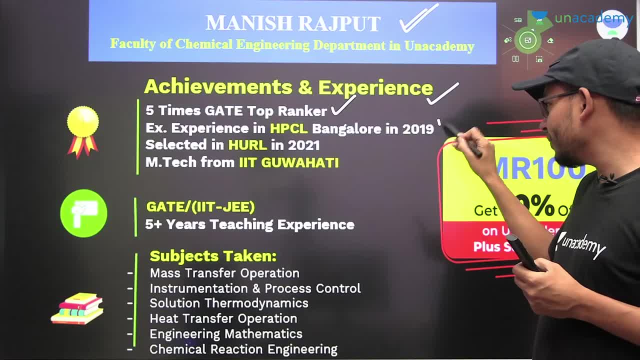 So five times gate qualified. X experience in the HPCL Bangalore in 2019.. And selected in the HURL in 2021. In June, And Mtech completed from IIT Guwahati, Okay In petroleum science and technology. 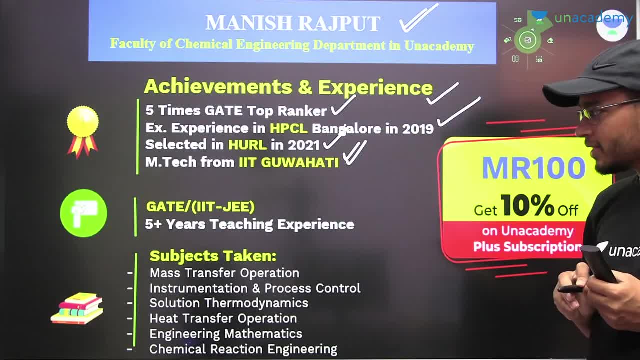 I will just talk from here. Five times, Five plus years of teaching experience, You will talk in this, In which you have the most of your gate part- Okay, One year around you have the JWE experience. Okay, I will talk from here. 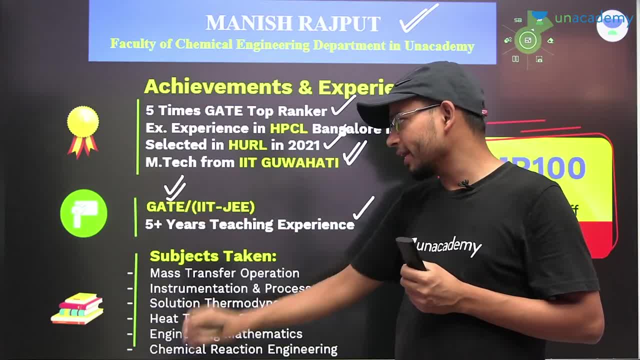 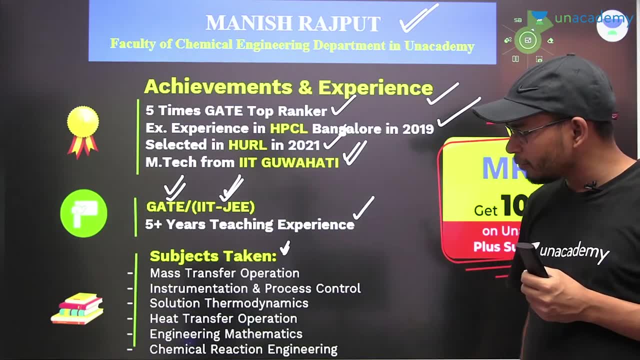 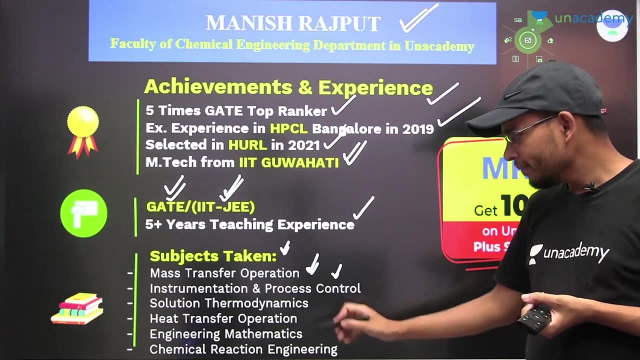 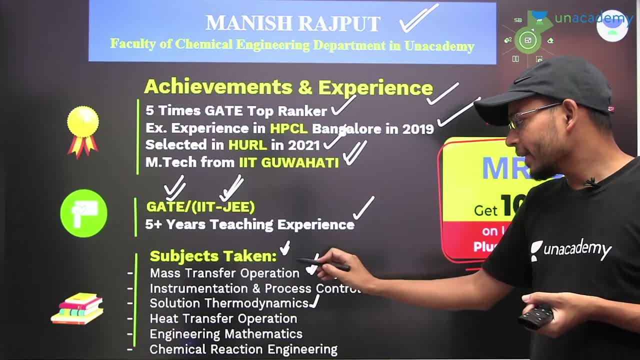 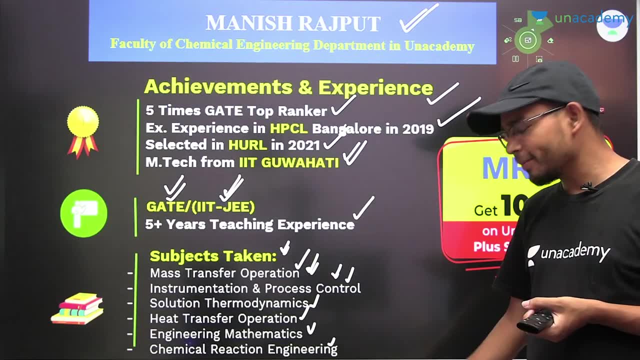 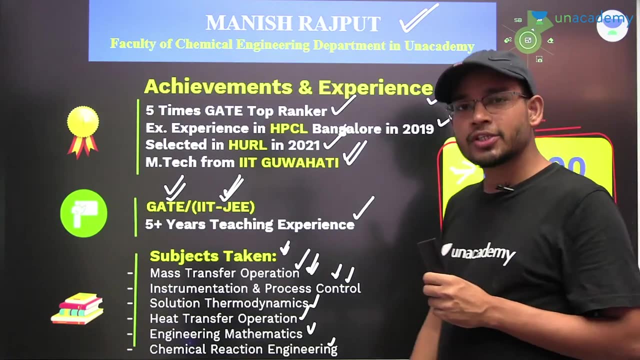 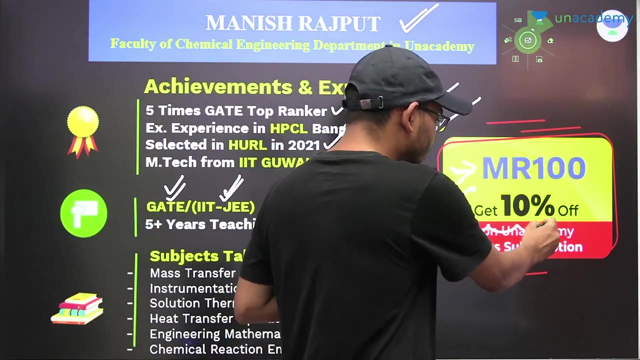 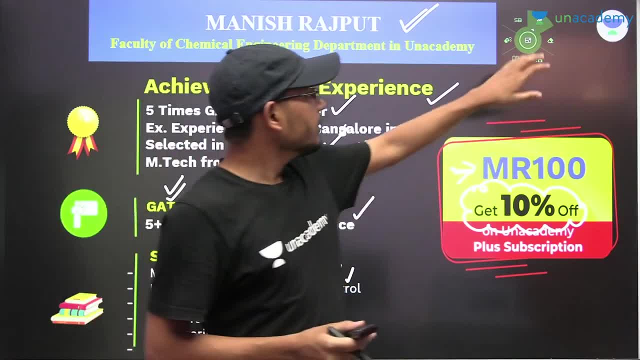 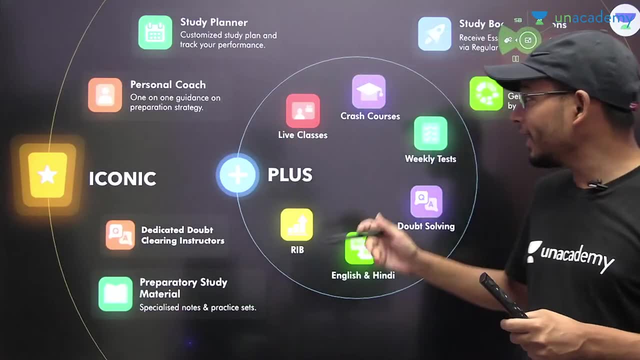 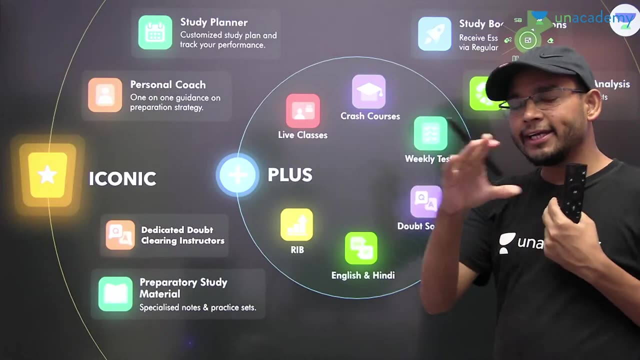 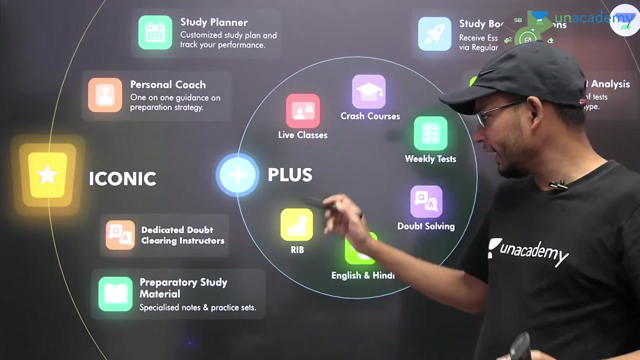 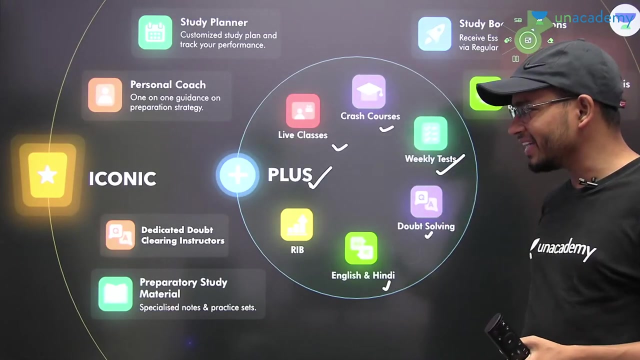 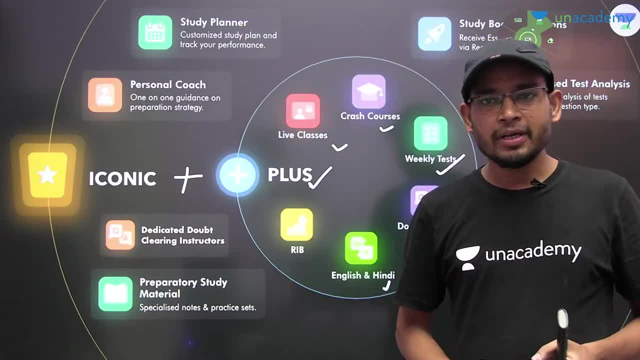 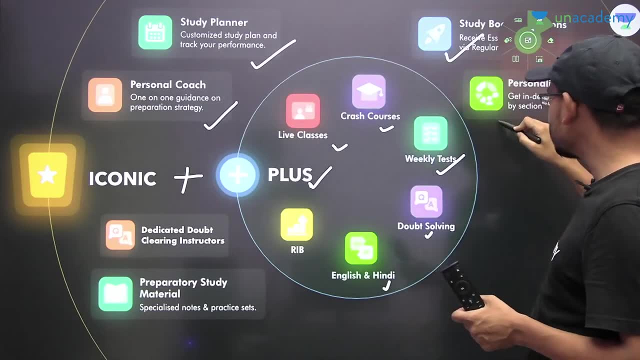 Iconic comes with them. so many offers are also going on in Iconic and many other features are also involved in it. So for Iconic you will get personal coach, study planner, study booster session, personal test. and one more thing is added here: dedicated doubt clearing instructors. 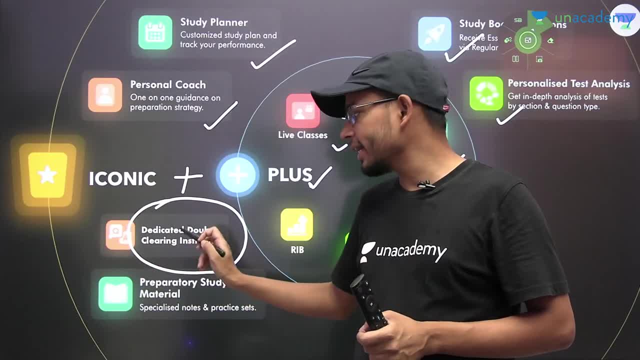 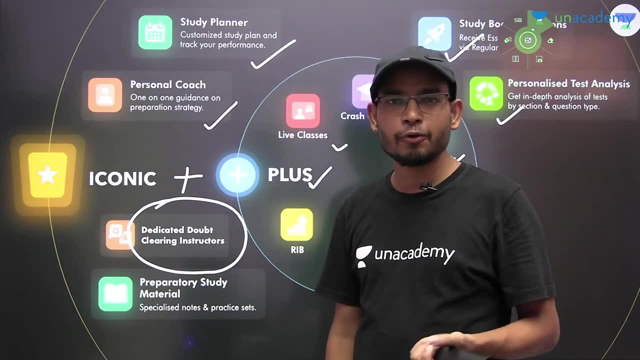 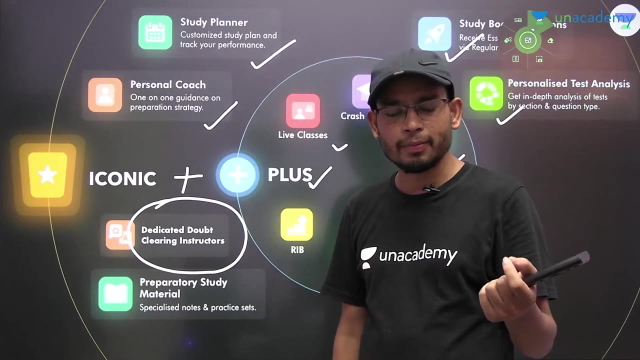 Here especially for you. what will they do for you? if you have any doubt, you will immediately send it here and you will get your reply within 24 hours. It can also be your video solution. it can also be your solution in your PDF form, so you will get that solution properly. 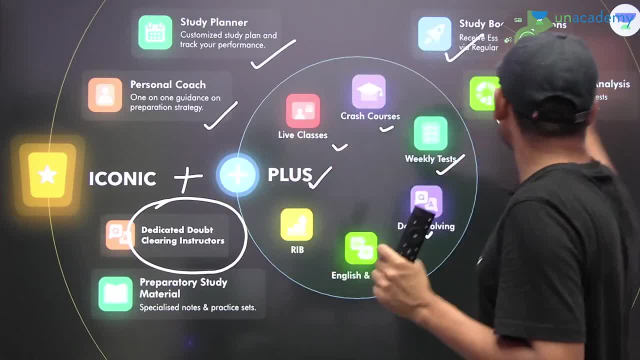 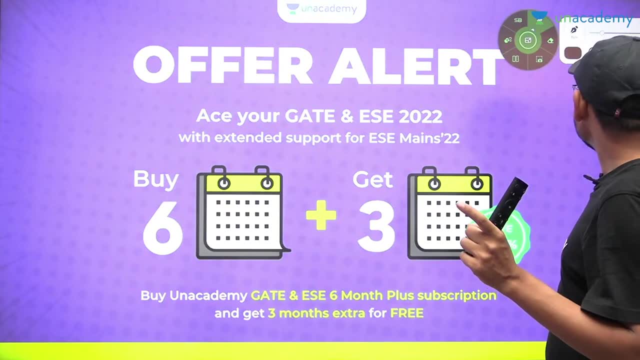 So this is the feature for Iconic students. After this I will talk. after this, I will say that now this offer is going on in the current 6 plus 3 offer 3 months. This was not an offer, yet it has also come. 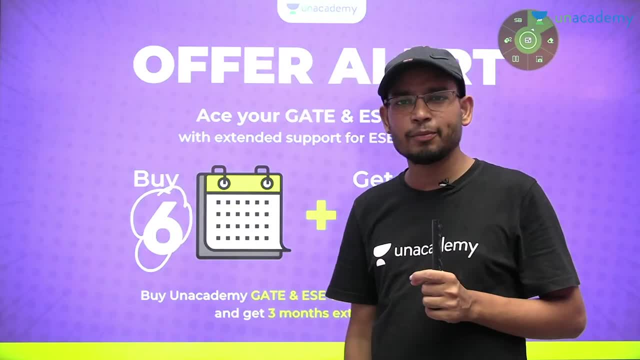 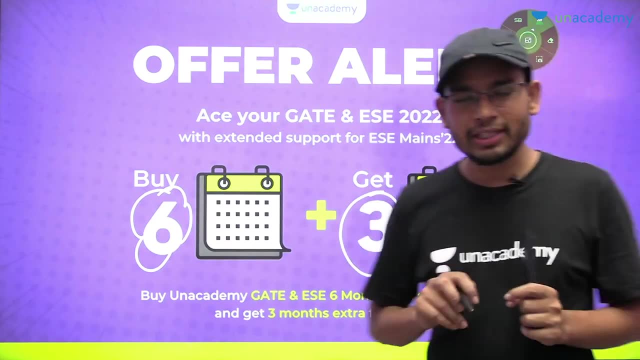 Okay, so 6 plus those who want to move with 6 months now. so along with 6 months you will get an extra of 3 months, Those who also want to take. then you can say that almost 1 year is 9 months. 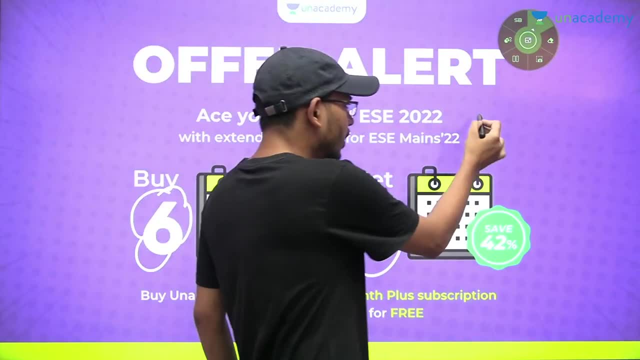 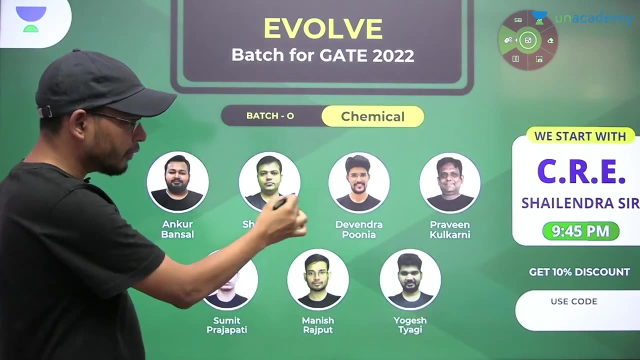 9 months is a good time for preparation, So you will use the code MR100,, right, You will move ahead from here. come on, And this CRE is also running on 9.45.. And along with this, your mass transfer operation, which started on 26th August. 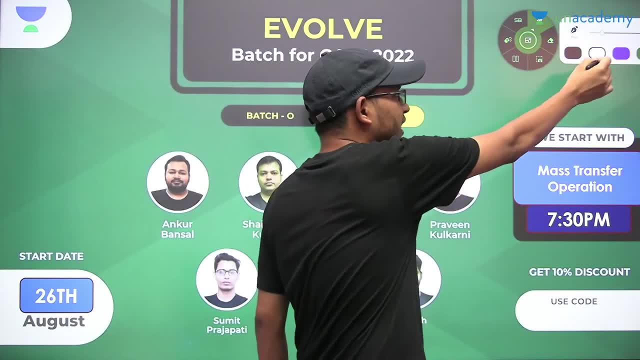 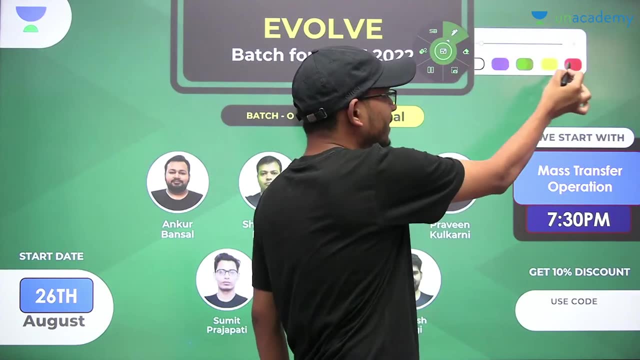 Okay, It started on 26th August. Here I have started via distillation. Here what I have started is distillation Right, So from here also you can move with distillation. Okay, Its timing is 7.30 pm. 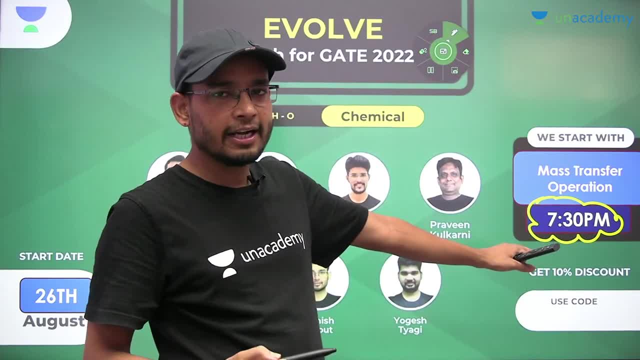 7.30 pm. Okay, Your 30,. now a gap of 3 to 4 days has been given Because 3 chapters, 2 chapters have been done. well, Okay, And your 30% part of distillation has been completed. 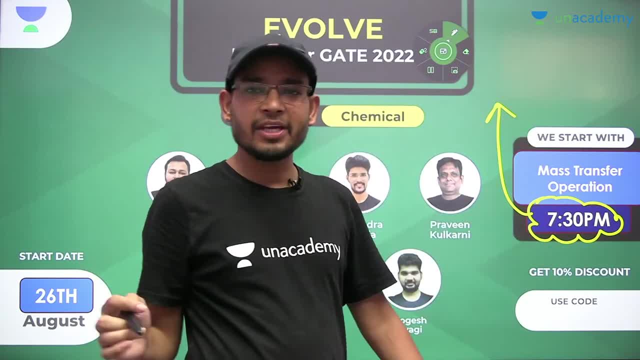 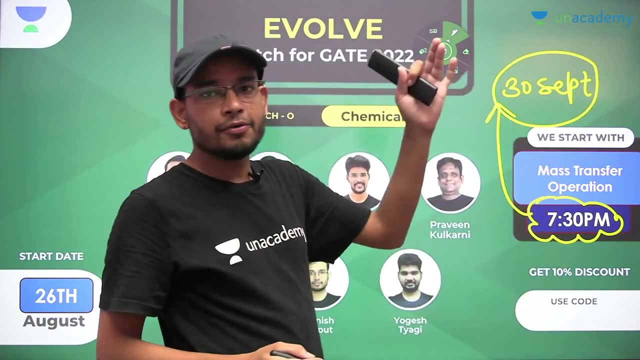 In which you have been timed for revision. These classes will resume for you From 30th of September. Okay, This class will resume from 30th of September, And then it will continue till your October. Okay, And in the first week of November your mass transfer will be over. 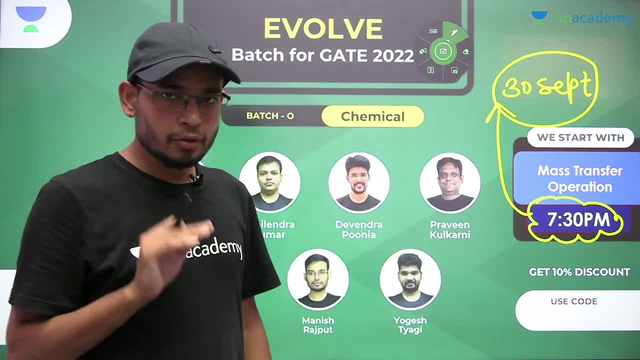 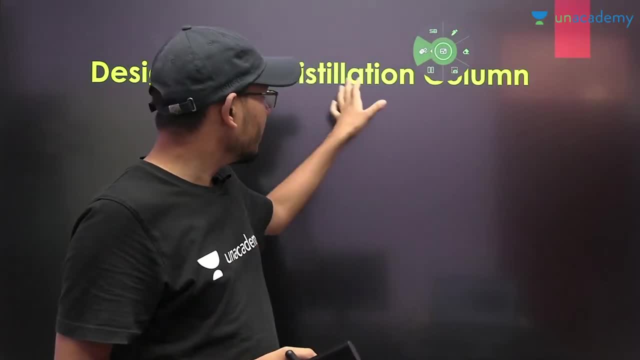 So those who have not yet studied mass transfer- And they are planning- So join us And meet us in the evening at 7.30 pm. Okay, Let's talk about something good. Okay, Come on, Let me talk from here. 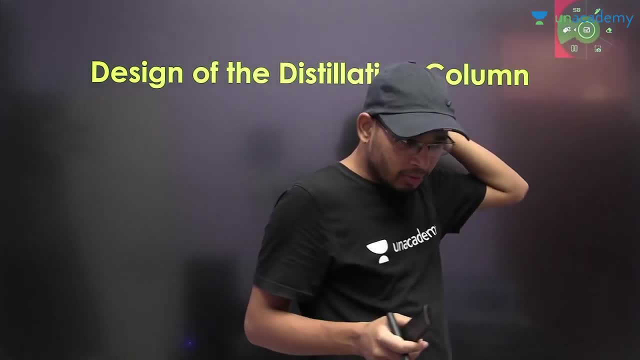 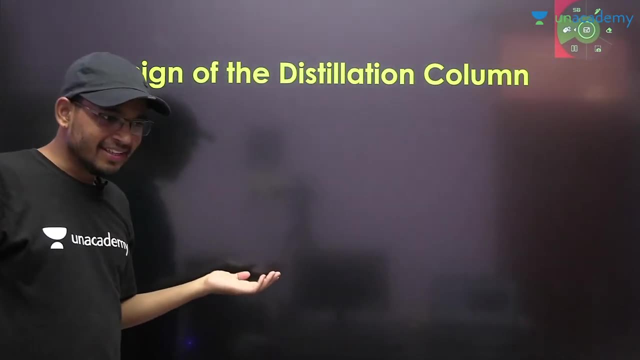 Let's start our process from here And Yes, Yes, Yes, Yes, Yes, That's right. Okay, First of all, we have to focus on design. Okay, First of all, we have to focus on design Again, starting from degrading the current state of your. 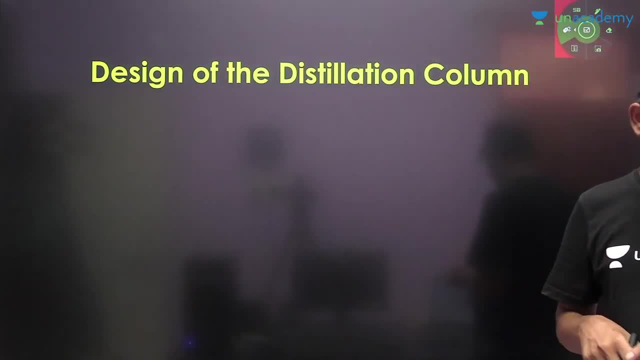 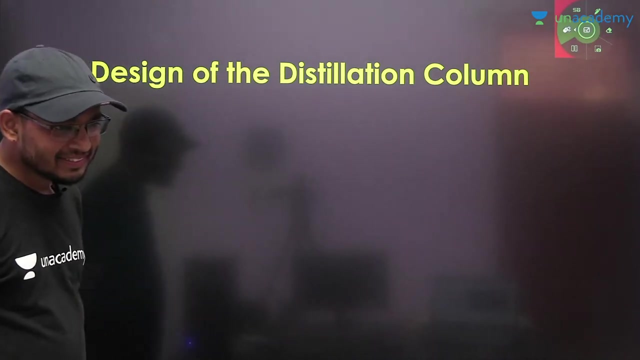 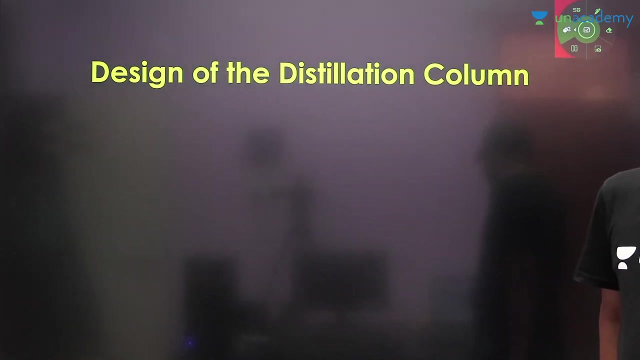 Chinese milk. So you will all have wrong suggestion. Yes, It is wrong. Yeah, Please make it clear. Okay, You still doze well, Okay, empty over here. yes, yes, Nilesh, ok now, if you study in a continuous and dedicated way, then your results will be converted. 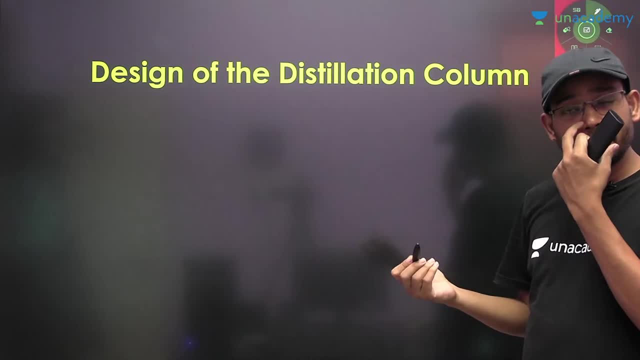 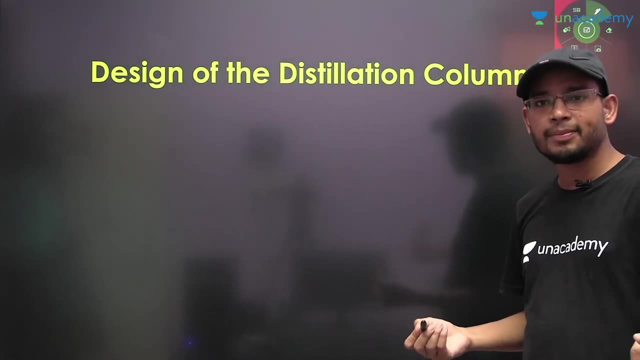 otherwise, the most important thing to get any result is dedication. in case you are doing it properly, then the result is not far away. what is the result? it is the outcome of the process. in case you have followed the process well, then the outcome will be good. 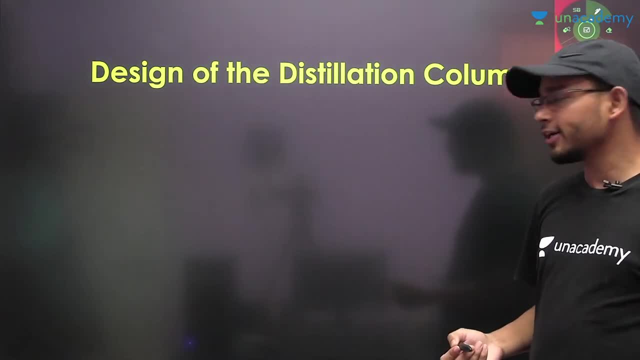 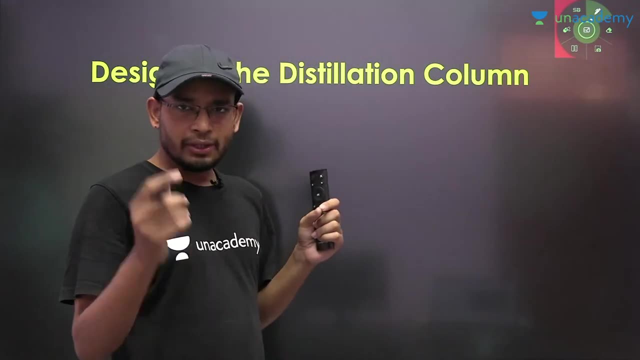 if you have followed the process in a lazy way, then the outcome will come, but it will come in the same way. ok, so we will put heading new page, new page. I will use at least 30 to 35 pages in it. ok, so either make a thin copy of its designing. 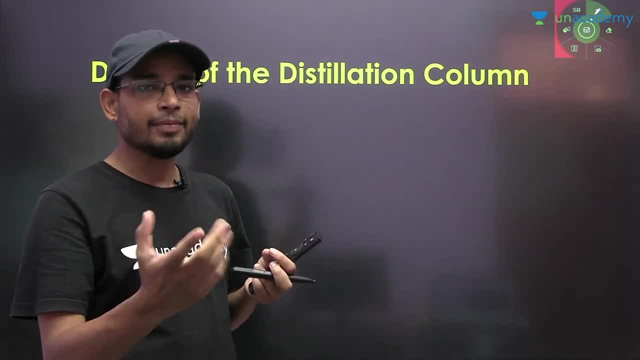 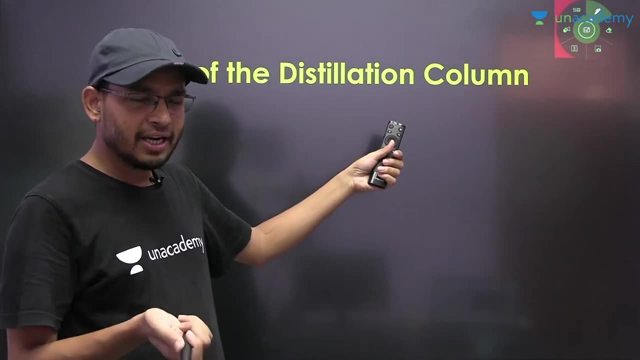 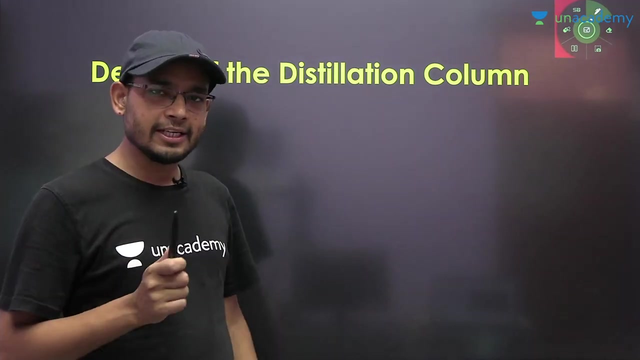 or go to the market and make a thin copy. I will cover all the designing parts in it. ok, so now you will not have the copy. you have to try to repeat it in the next one. make a thin copy and go to give an interview. then go to revise the copy properly. 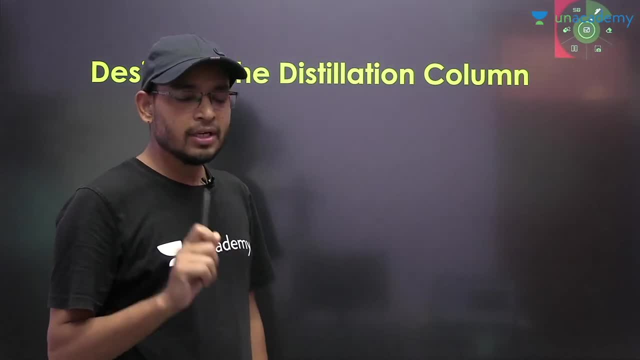 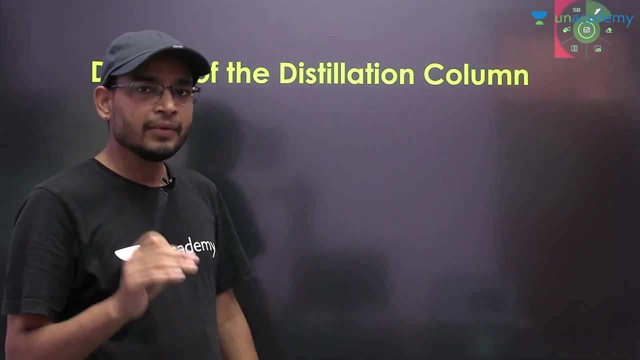 from here, all the theoretical questions of the gate will also be covered. the theoretical questions in the gate get stuck with the distillation. that, sir, the theoretical questions are not covered. the numerical one is done. do this session? ok, all the theoretical questions will be done. numerical will be done. 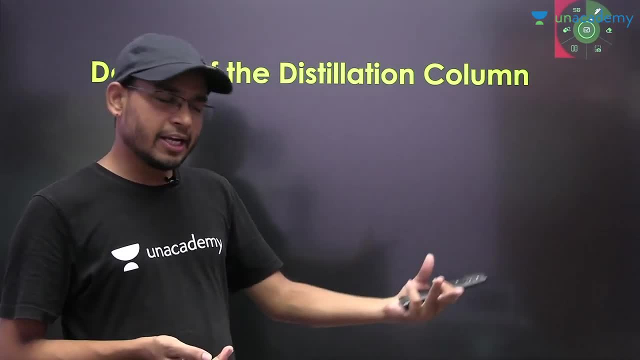 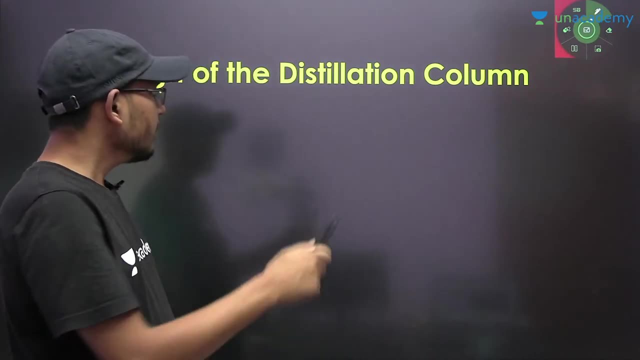 numerical questions are easy. just you know the expression, you know how to use the expression, you will solve it properly. but when a theoretical question comes, when a conceptual question comes, then a little thing gets stuck. ok, so we will try to take you to the whole deep. so. designing of the distillation column. 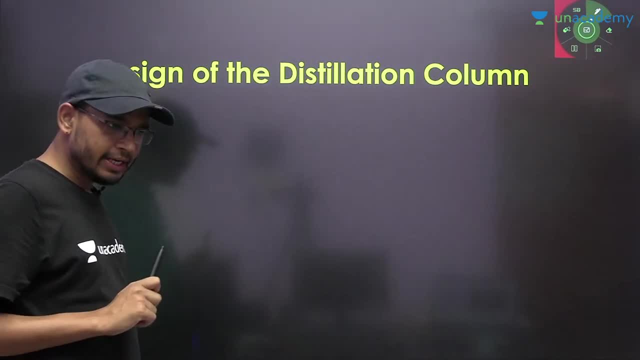 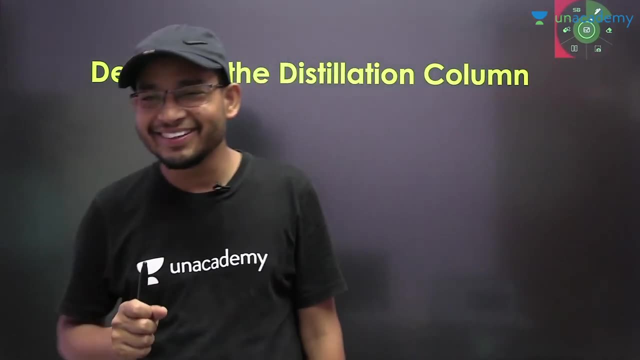 we will put heading in the new page, designing of the distillation column, and are all the people ready? let's start. everyone is ready? yes, ready. we have to make notes. we don't have to listen. ok, listening will fly away. ok, don't be unhappy. 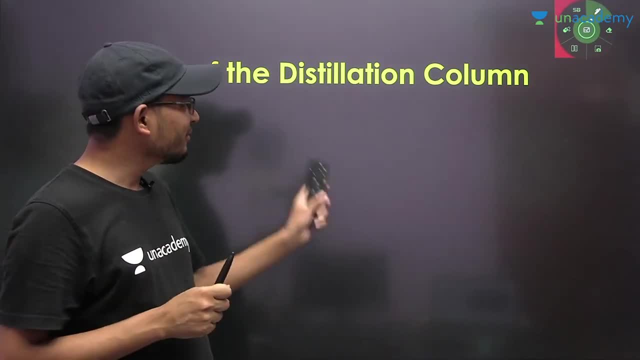 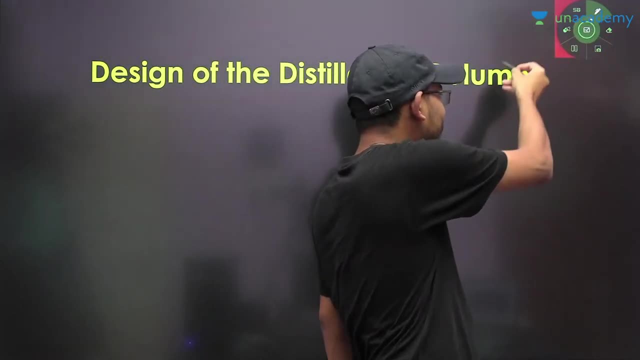 once you listen, copy and paste. it's not like that. ok, it will fly away. we have to write properly. we have to make notes. ok, we have to make very good notes. these are very useful sessions ready. everyone are ready. yes, ready. understand it very carefully. we will do it in designing. 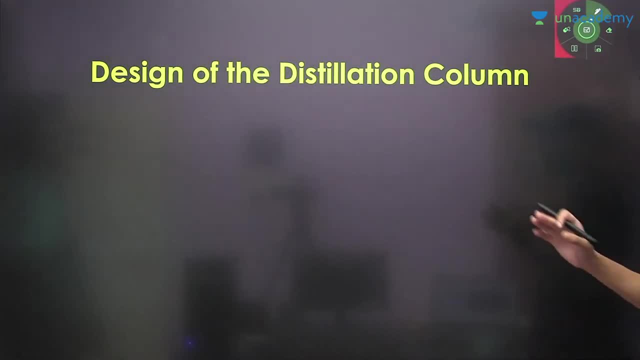 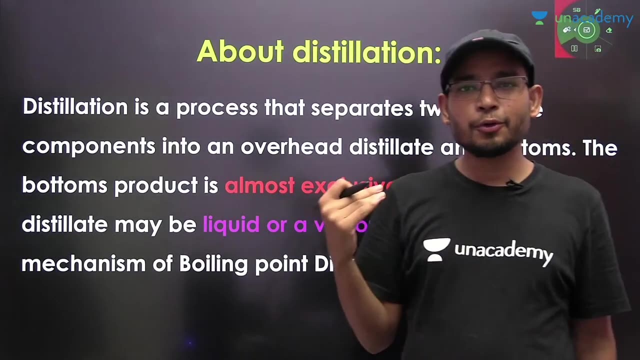 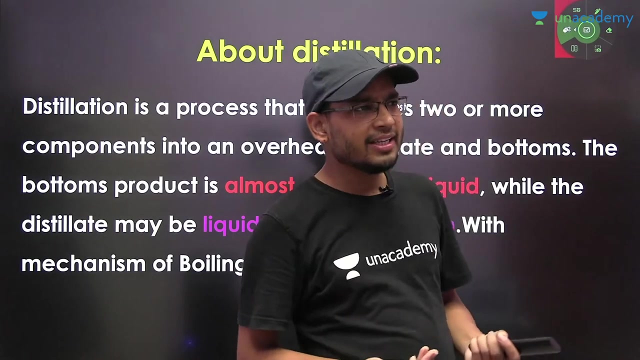 ok, everyone is ready. yes, ready, everyone is ready. everyone is ready. let's start. ok, we are removing all the disagrees. ok, let us start. i know what you like, you want to know. ok, ok, let's start. ok, yes, lets start. ok, it's on. ok, let's start. 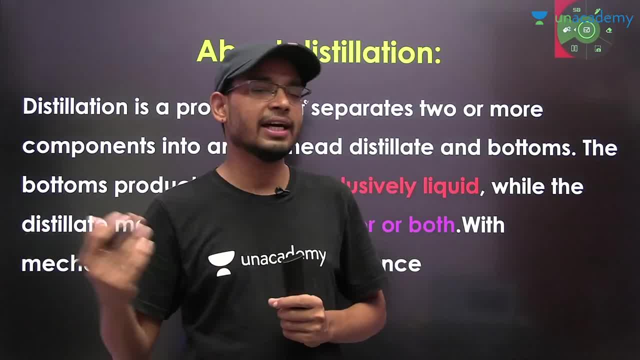 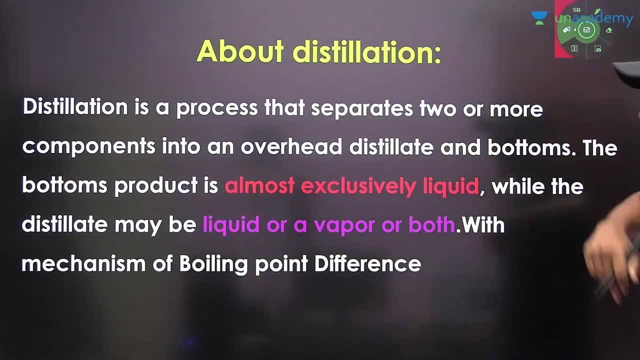 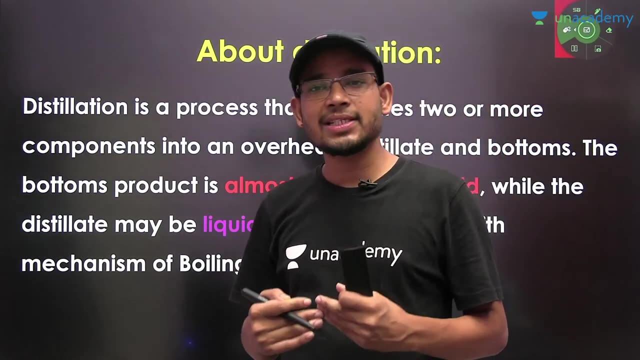 co do i have to list? okay, ready, ready, let's see, let's try. I take that the barrel is like a colostrum, let's see. I will talk a little about distillation. What is distillation? It is a separation technique. Now, separation technique is different. 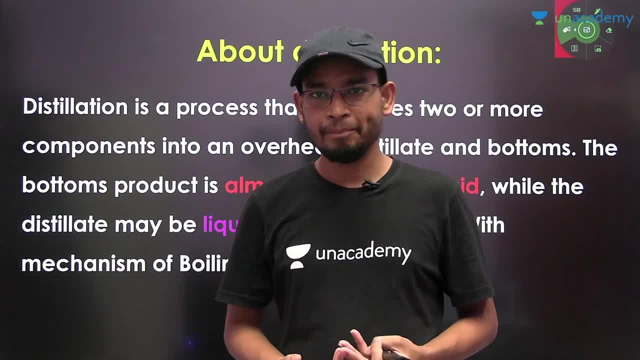 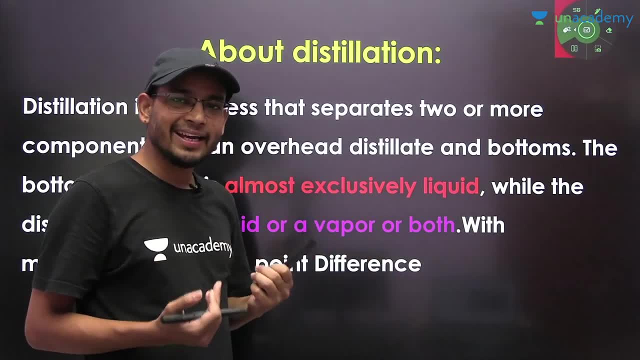 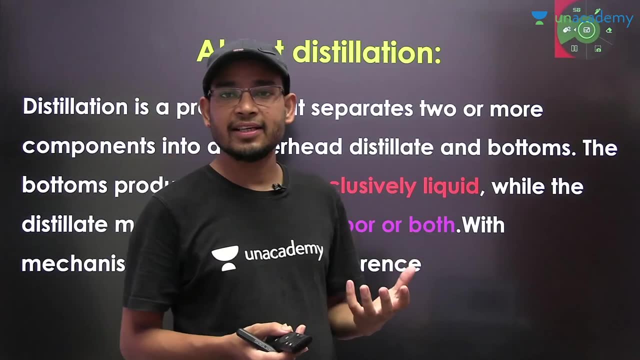 Extraction is also separation technique. Drying is also separation technique. Humidification is also separation technique. So what type of separation technique is distillation? This separation technique is with their boiling point difference. In case there is a difference of boiling point in your component. 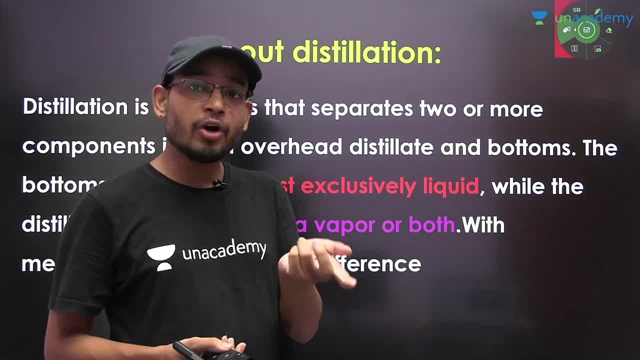 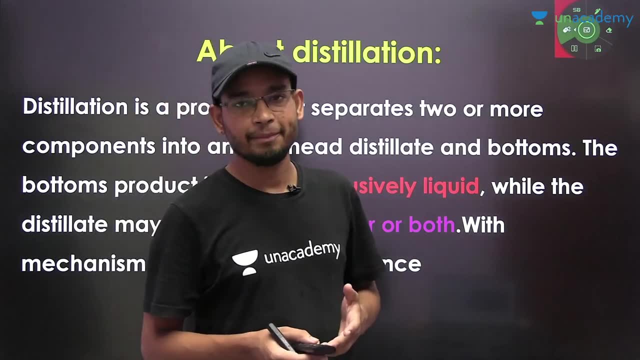 then you can separate it with the help of distillation. There is no difference of boiling point in your component. It is a very close boiling point, So you will not separate it with the help of distillation. It will be another mass transfer operation. 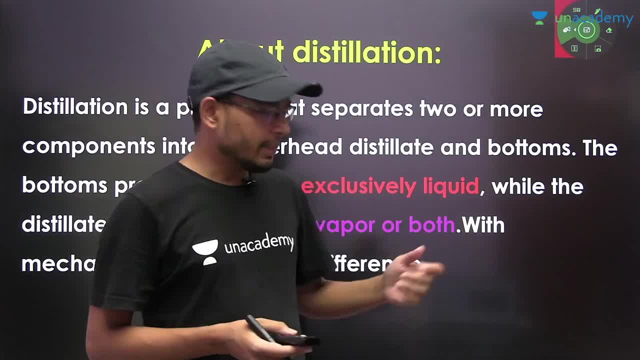 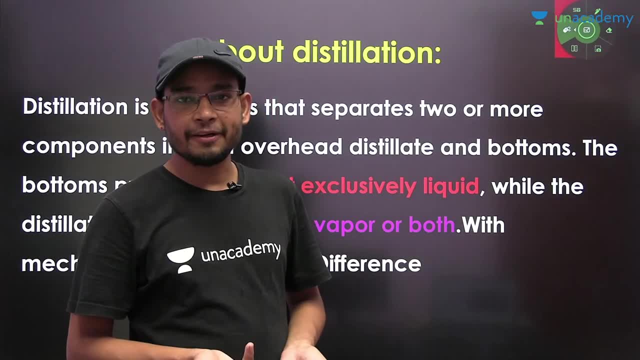 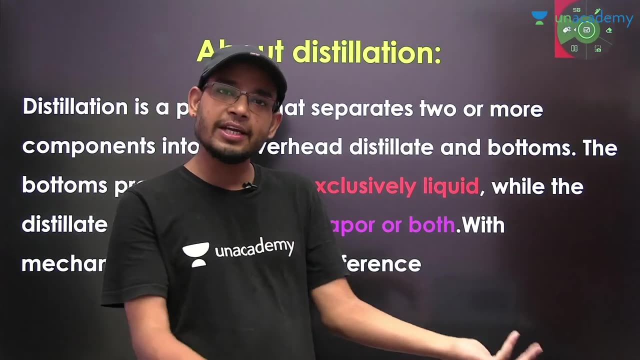 You will separate it with the help of another unit operation. Suppose there is a particle of higher density and a particle of lower density, So there is no need of mass transfer here. You will put a simple filter and separate it, Otherwise it will automatically separate from the gravity settler. 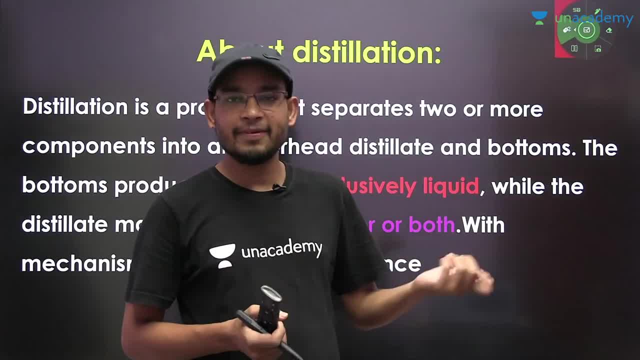 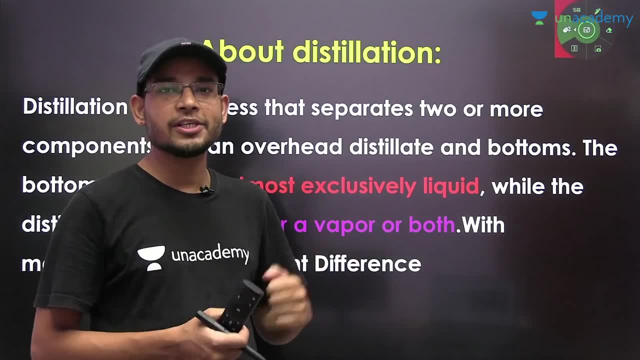 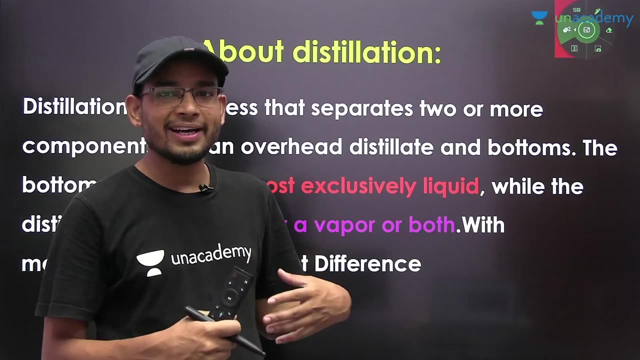 But when there is a misfill component, like benzene and toluene, their mixture is formed. Now it is a misfill And there is a difference in their boiling point, Then they will bring the distillation in the picture. Suppose you have to remove water from the slurry. 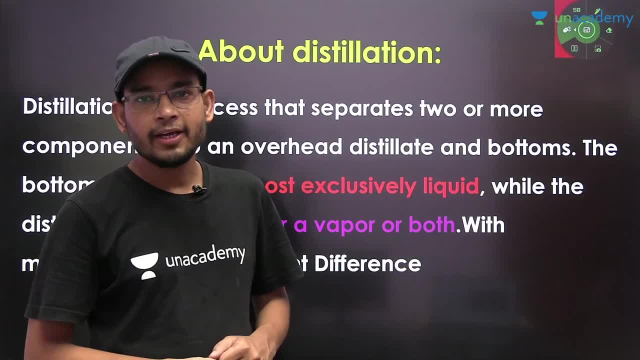 So there is no mass transfer operation there. You will do the filtration work there. There is a solid particle in your gas, So there is no use of mass transfer there. You will just put an illustration. So what will you do immediately from there? 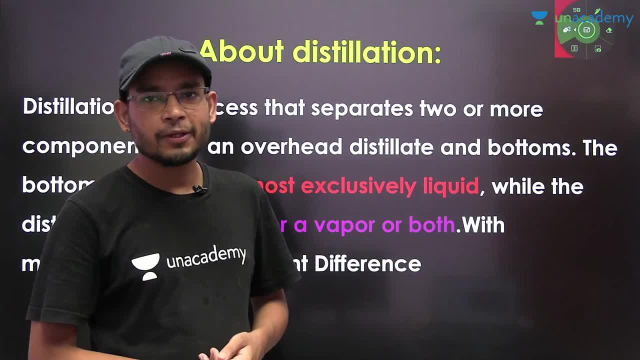 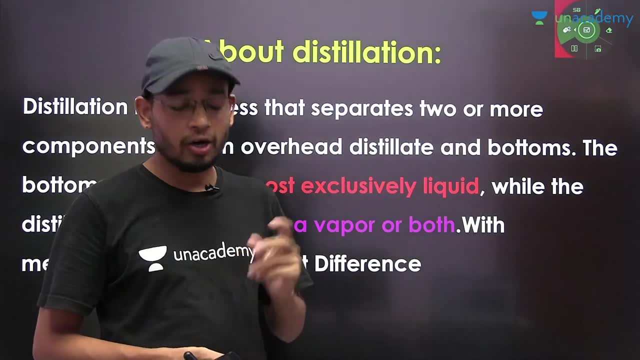 You will put a cyclone separator. Immediately it will be separated from there too. But mass transfer is a different kind of unit operation Where we will talk about it, And in distillation there is a specific region to separation of the components. 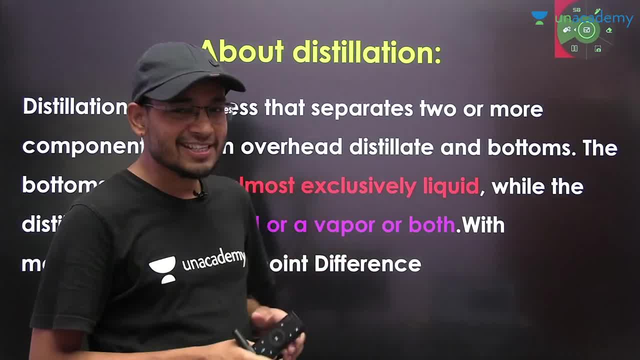 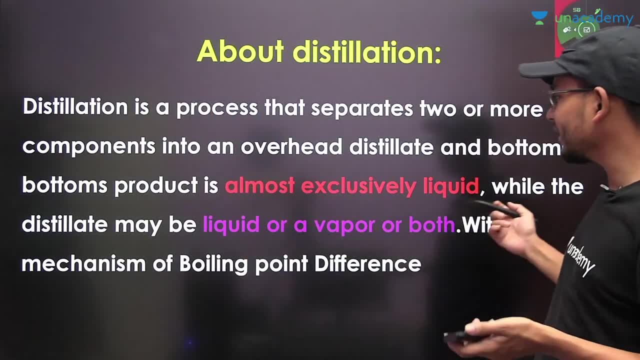 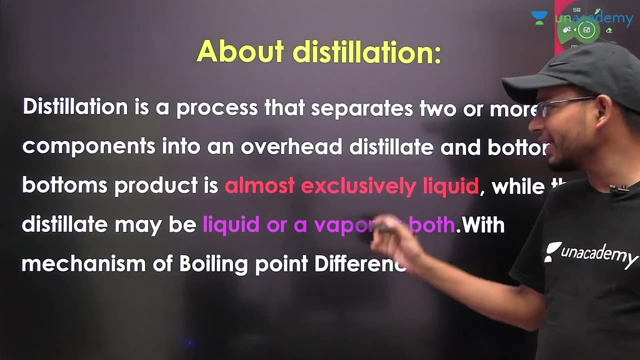 With their boiling point difference. There is a boiling point difference, Then only we will separate it out. Now we will talk about the whole mechanism of this separation. In this, whatever distillation happens, it divides it into two parts. It separates the process and divides it into two parts. 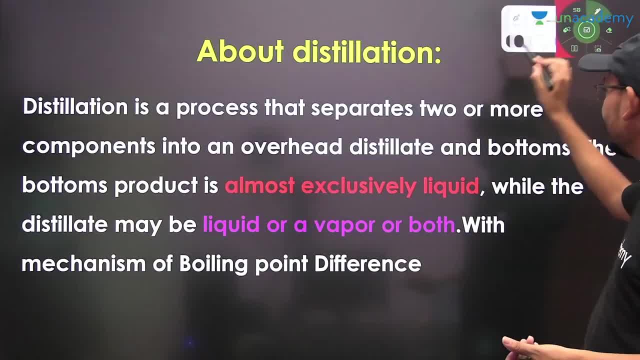 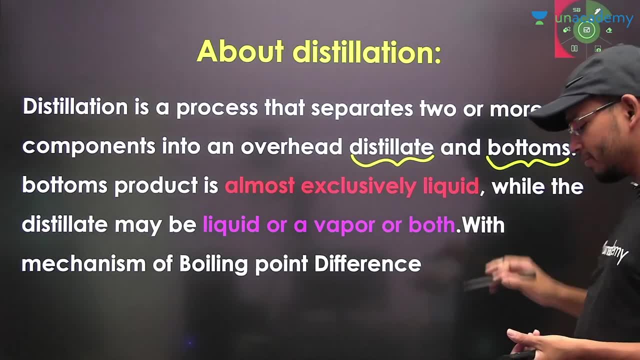 One is called distillate. We will call one part distillate. We will call one part distillate. We will call one part distillate And we will call one part bottoms. What happens in distillate? The quantity of the more volatile component is more. 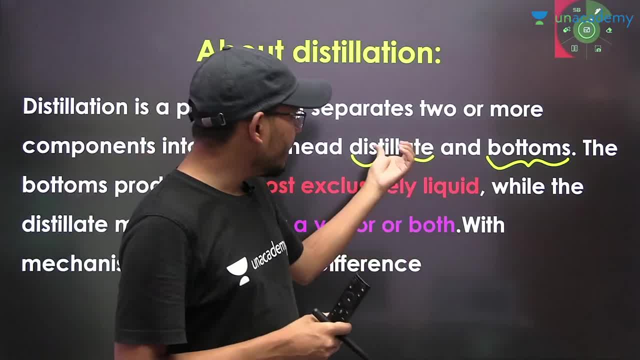 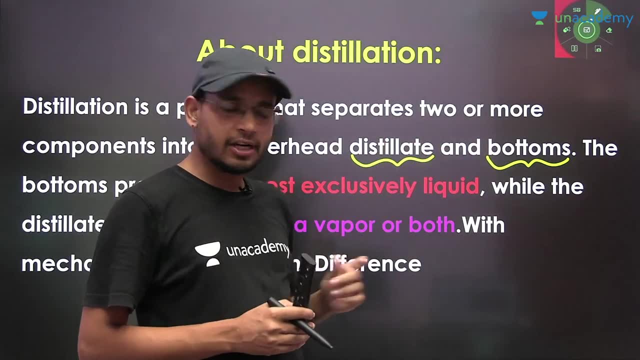 And sometimes we also call distillate product, That this is our product And this is our undesire And this is our desire stream. What is this desire stream? This is undesire stream. So desire stream means product. Product means the desired quantity. 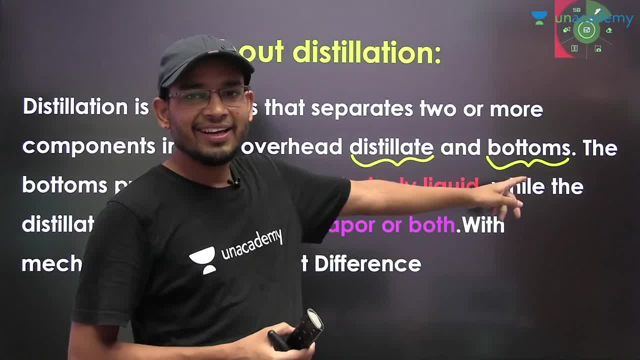 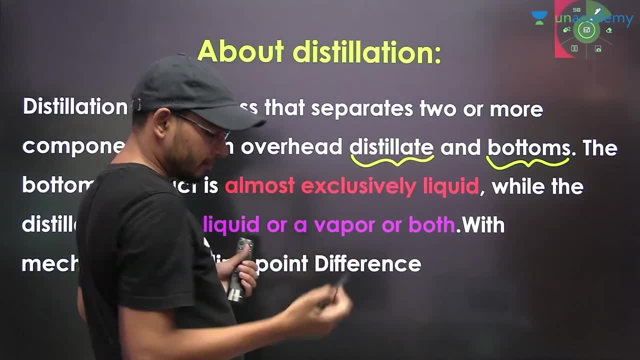 Right, Otherwise the product is also the bottom. But whenever the product is written somewhere, it means that it is talking about distillate, Because it means that So distillate and bottoms. Now the distillate will have two phases. 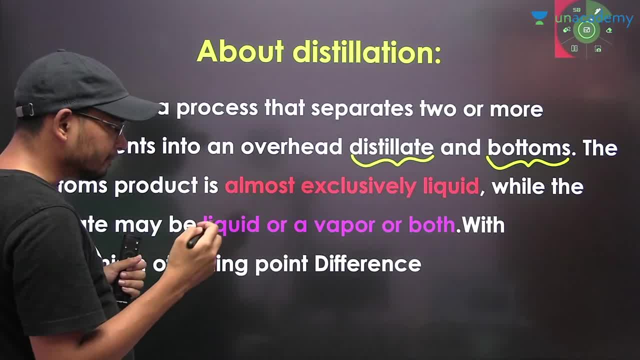 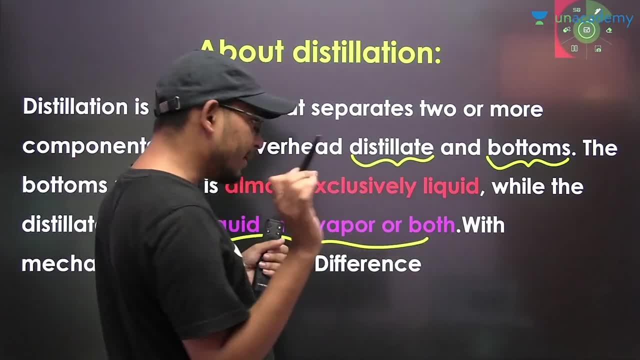 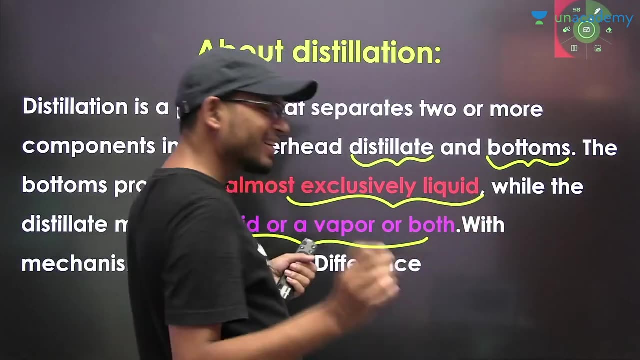 The distillate can be liquid or vapor, And liquid plus vapor can be both, Whereas in most of the cases the bottom is liquid. First of all, everyone understand this. This is the part of designing Right. So what will be your bottom? 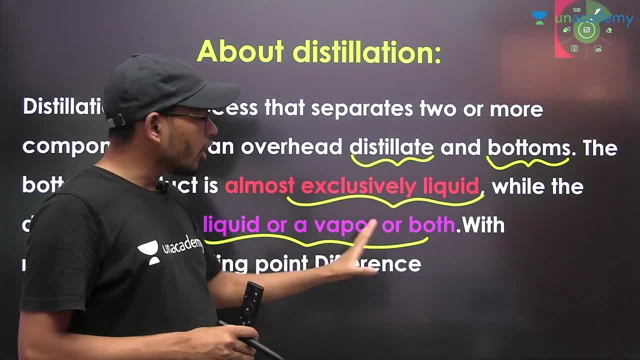 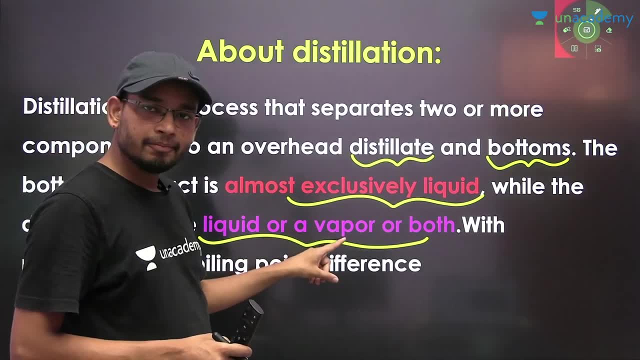 It will be liquid in most of the cases. Alright, And the top product that is coming out, The top product that is coming out of distillate, It can also be liquid. It can be liquid, It can be vapor, Right. 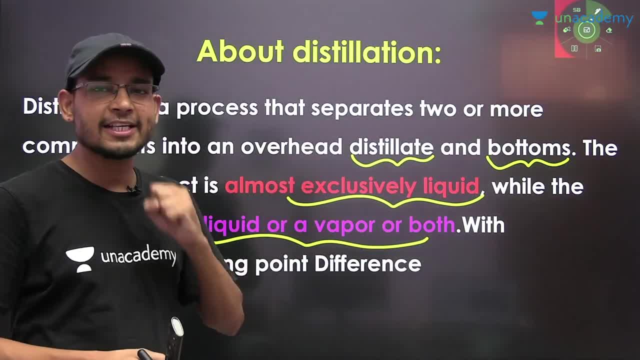 And the mixture of vapor plus liquid can also be there. It will depend on how you have applied the condenser Right. In case you have applied the total condenser, then you will get the liquid. In case you have applied the partial condenser, 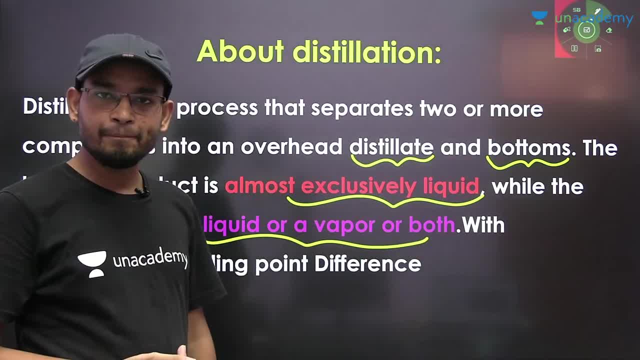 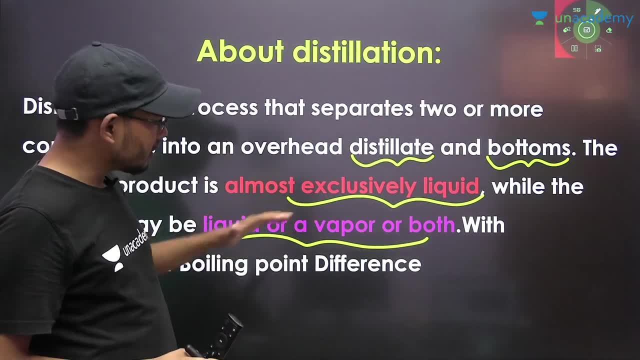 then you will get the mixture of vapor and vapor plus liquid. Okay, So it will depend on the condenser. Now I will talk about the designing of condenser, So just understand this And their boiling point difference. So the things that I have highlighted on so many things. 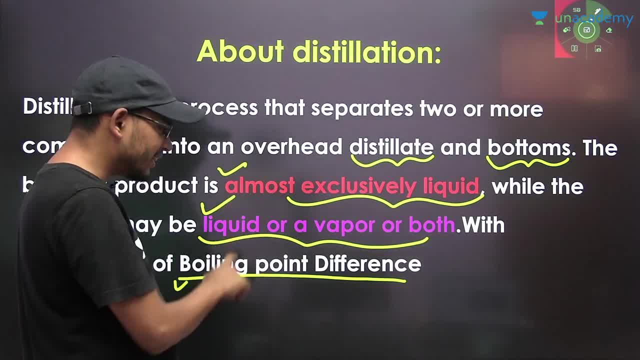 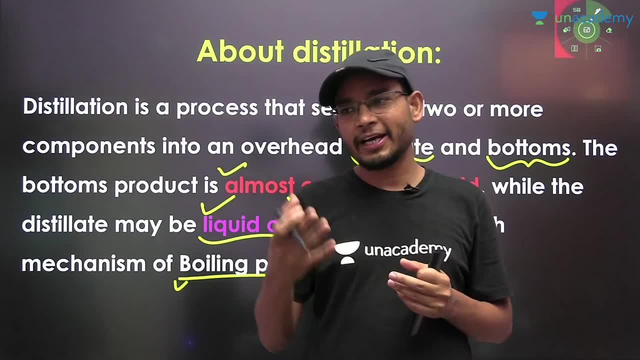 One is from red, One is from purple And this is from white. You should know these three points Right? The column is dividing in two parts. It is dividing in two streams. One will be your distillate, One will be your bottom. 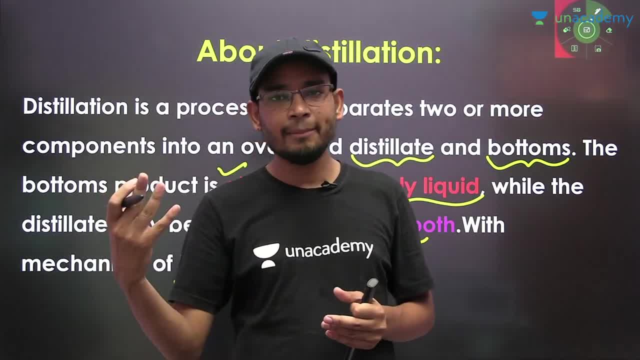 The product that will be coming out in distillate. It can also be liquid in that phase, It can be vapor, It can also be pure vapor, And the mixture of liquid plus vapor can also be there. Right, These three possibilities are there. 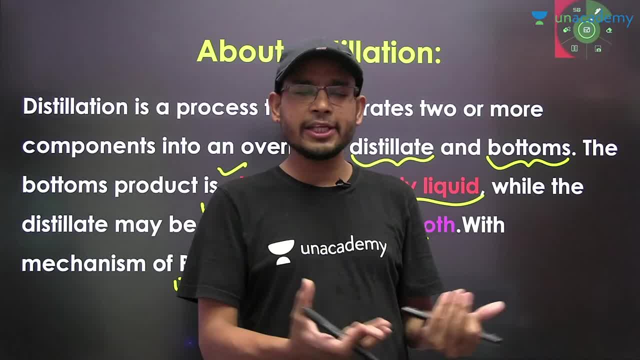 But in distillation, in most of the cases, the bottom is liquid. Okay, So we understood this much And the mechanism of separation will be a relative volatile difference And your boiling point difference Right. So when you talk about this, you will get that: your complete separation. 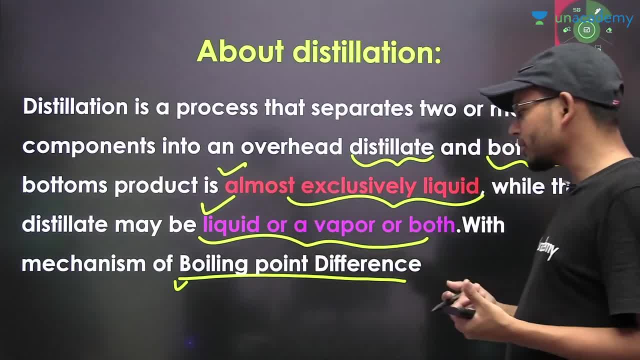 But now on this part which is called the bottom. You have to understand that the distillation will be a bottom as well as a liquid. There are three things: The bottom will be a liquid And the way that you can forget the bottom. 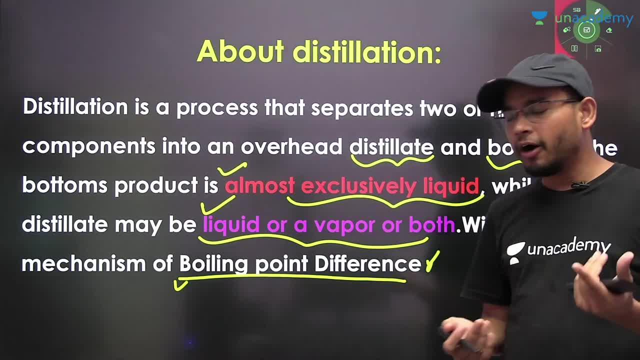 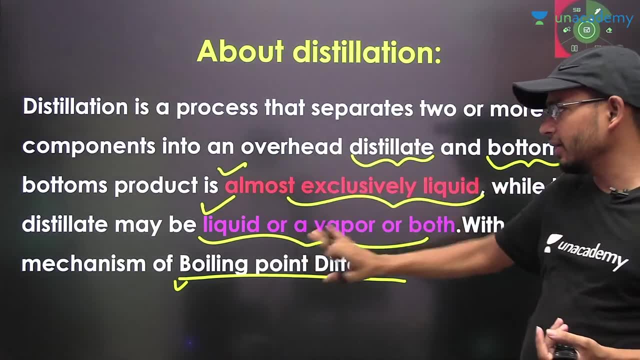 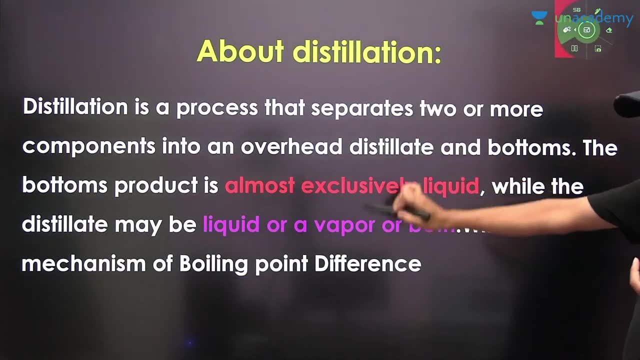 It is the bottom, the relative volatility difference and the boiling point difference. If you talk about this, then this is your whole separation technique. If you want, you can mention this in your copy properly. If you want, then quickly write it in the copy properly. 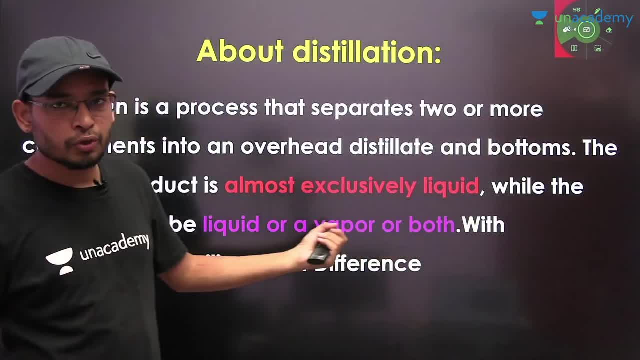 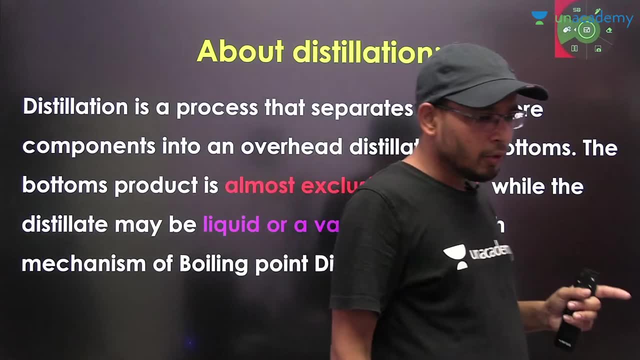 I am moving a little from the side, Because the theory part- you have heard it now- It will remain for 2 minutes. If someone asks after 2 months, then there will be no talk. Write it properly once: The highlight points that I have highlighted. they will also be highlighted in their copy. 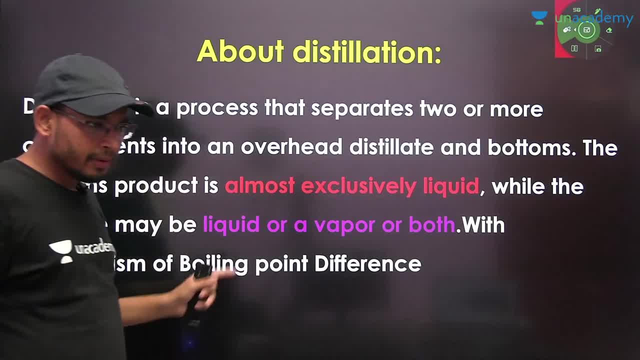 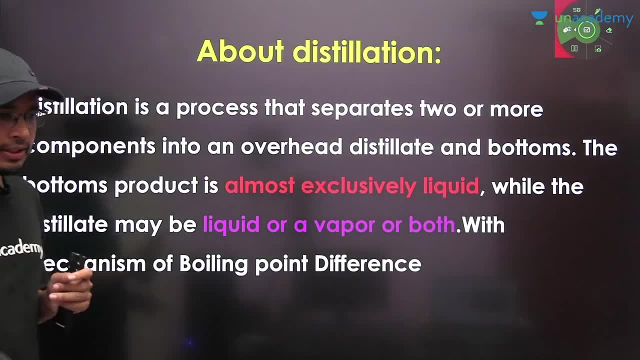 Yes, First of all, everyone will write this quickly, Then I will move this process forward Quickly. We will write it quickly and say: done, Lovely. If you stay stuck, then I am telling you that I will make your distillation amazing. 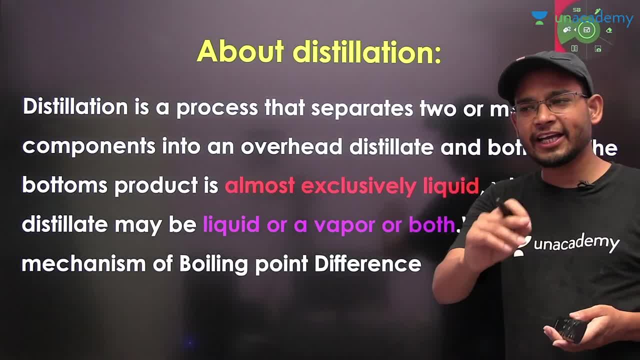 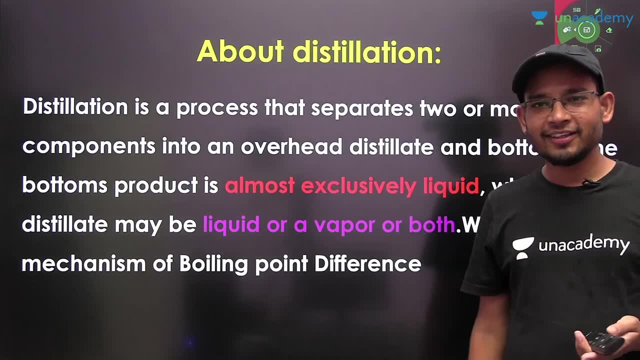 This one with designing. This is the first part. Whenever you go in an interview, in any top India interview, if you do not get a question from the distillation, then this cannot happen. It will ask you 100% from the distillation. 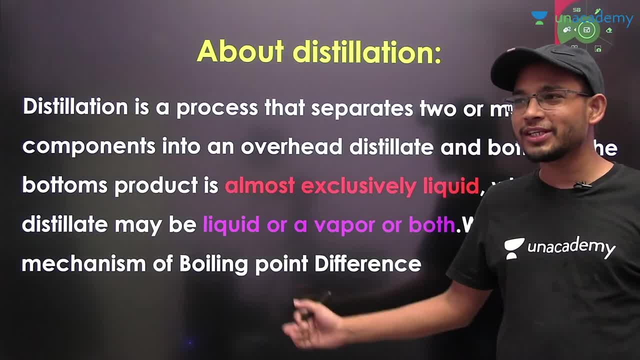 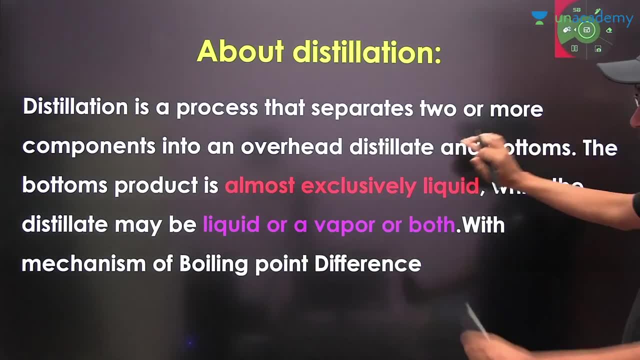 Okay, You will also know a little bit of chemical engineering. He will definitely ask that question from the distillation. Okay, The panel will ask the question from the distillation Done. Keep writing this and everyone properly. Okay, Now I will talk about designing. 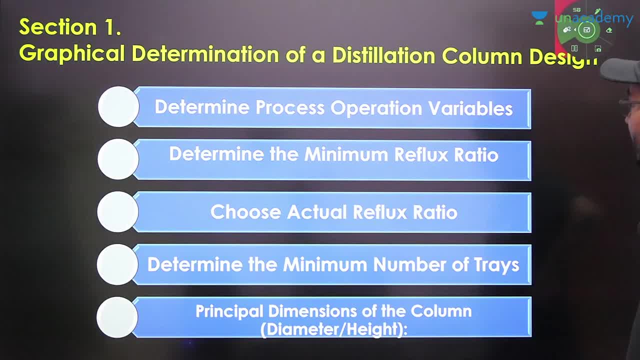 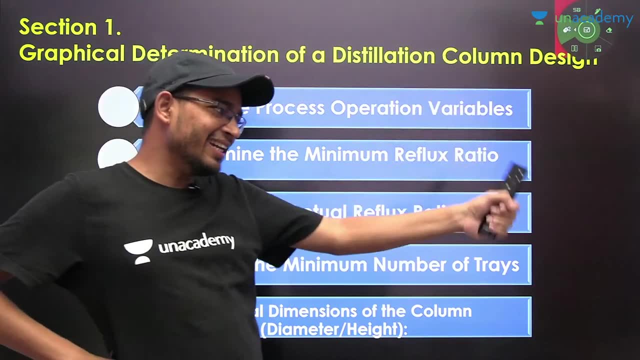 Now I will talk about designing. So it has two methods of designing. One is the graphical method of designing, One is your analytical method. Okay, Any system column you are designing distillation column. How many will you have to design that column? 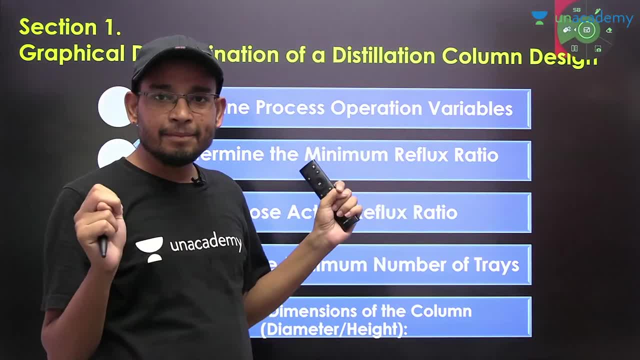 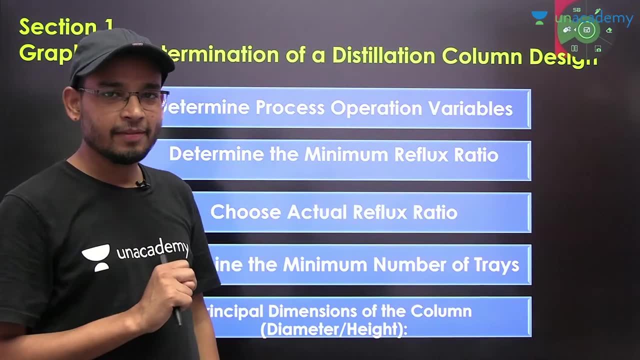 Basically, there will be two methods. One is your analytical method and the other will be the graphical method. So you know that we have a little more interest in the graphical. So first of all we will talk about the graphical method. It is also more interesting. 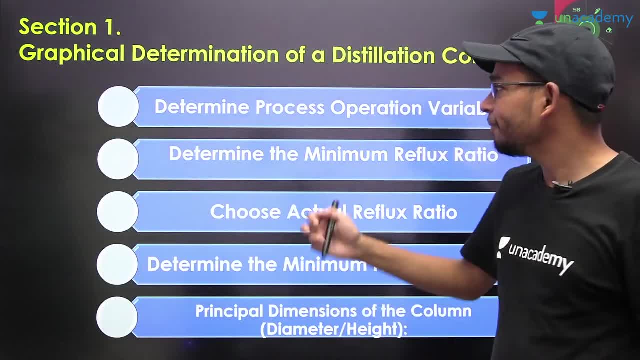 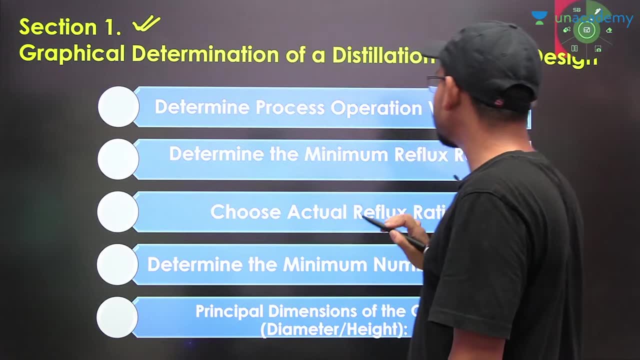 Okay, Interesting method is graphical. Things will not be visible in the analytical Right. Come on. So first of all we will talk about section 1.. The graphical method to determine the distillation column. Okay, Design, The word design. 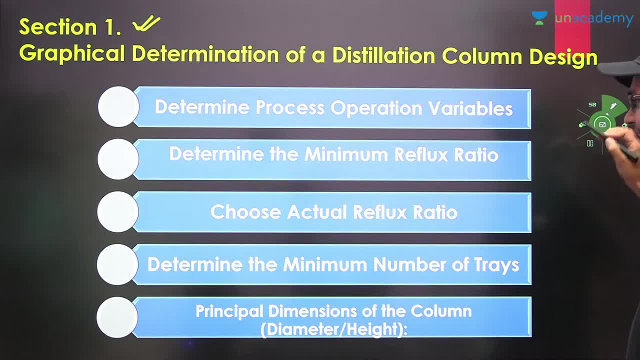 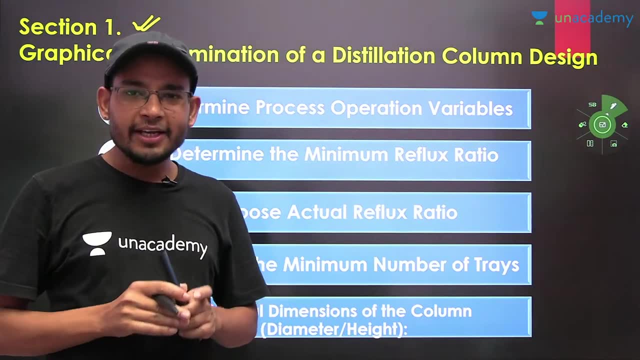 In this. the first thing we will talk about is graphical method. Whenever we design, we will have to keep designing parameters in mind. What are the things that you are designing? Let me ask you this question, Sir. we are came to design the distillation column. 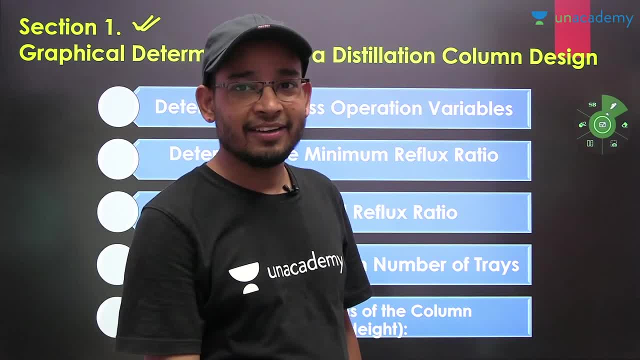 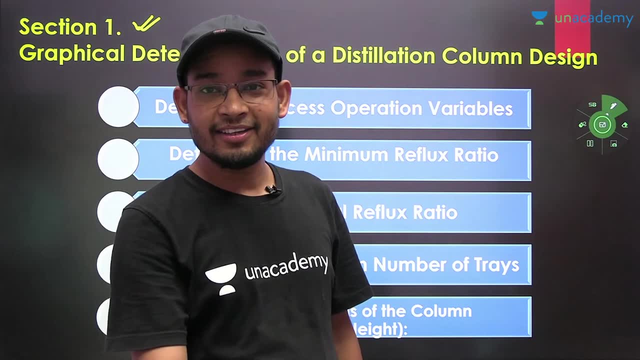 After reading the chemical engineering. Now, what do we have to do? First of all, suppose you have reached, Sir, you have to design the distillation column. How to do it? Okay, sir, Now how to do it. You should know the parameters. how to design. 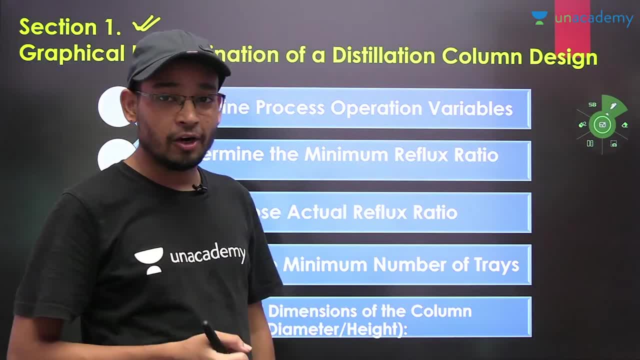 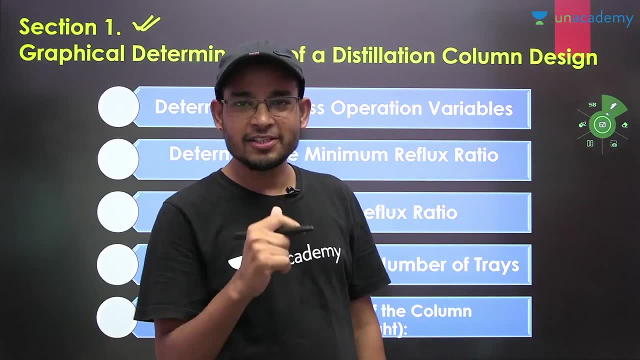 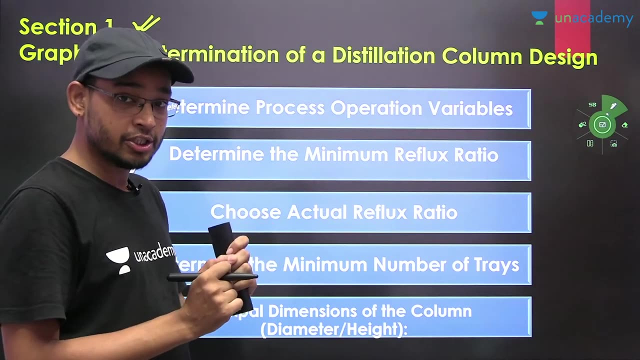 So that is very important. Suppose you have been allotted a project that you have to design a distillation column. Now you will first think from where to start How to design a distillation column. So there are 5 steps for that. Understand very carefully that the whole system is properly defined. 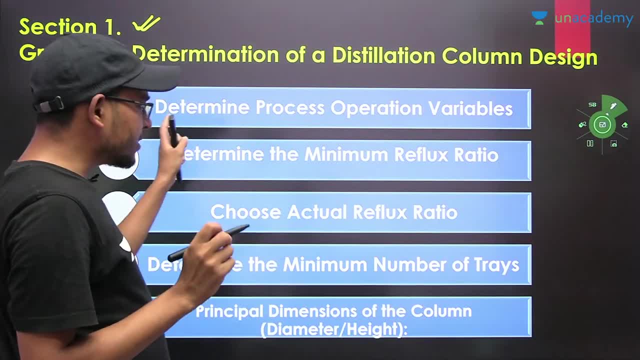 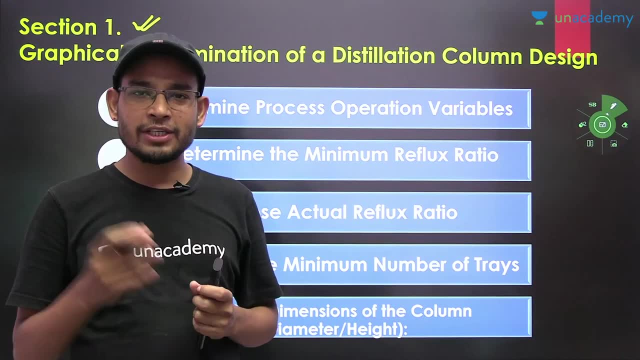 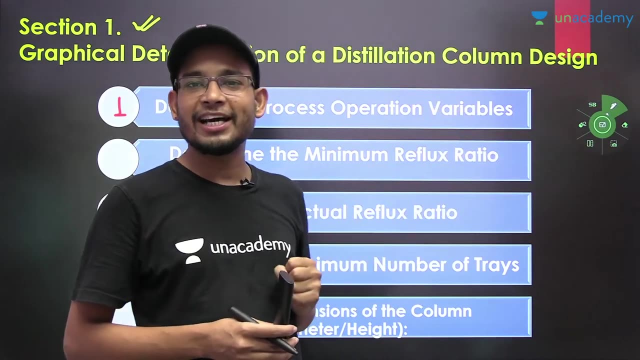 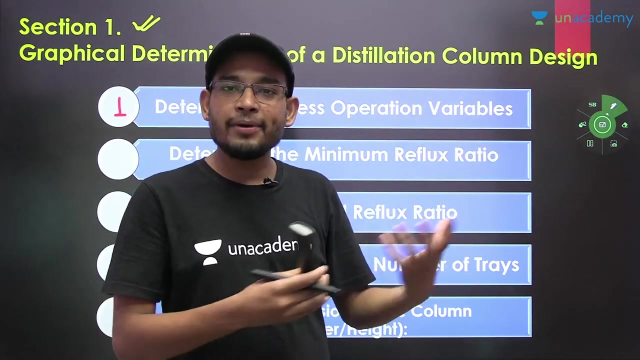 So the first step is to define all the operation variables. All the operation variables like feed flow rate, Feed composition, Quality. How much flow rate is going in the bottom? You should know that. How much flow rate is going in the bottom. You should know that How much percent of distillate is available in the market. 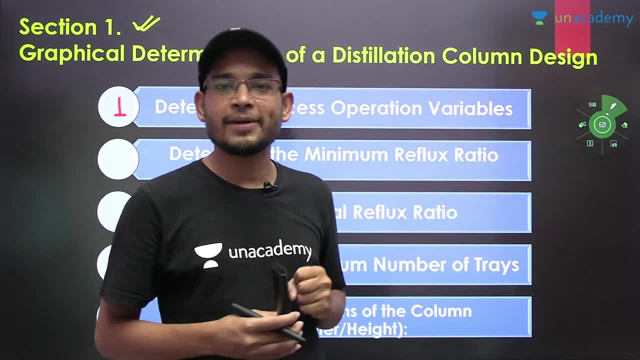 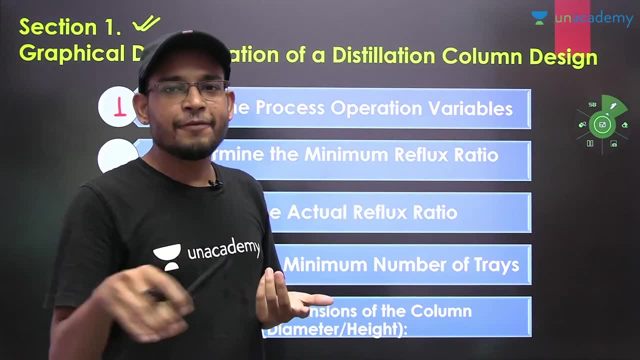 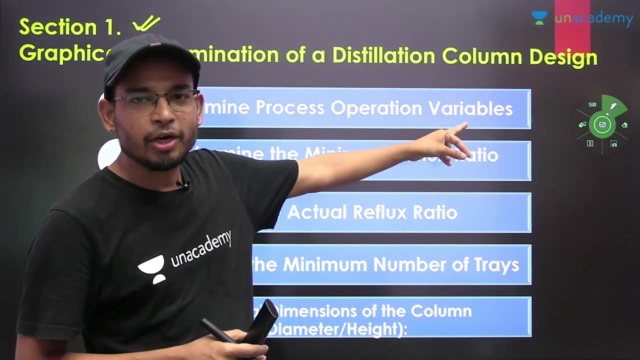 88%, 80%, 90%, 95%. How much percent of quality do you need? These are the operation variables: Feed flow rate, Bottom flow rate. You should know all these, Then you will be able to design. So we will tell you the story of this in detail. 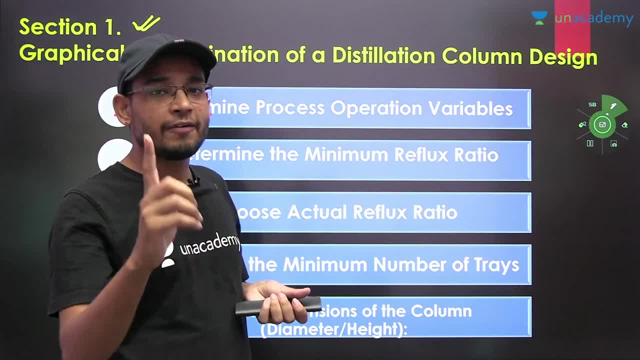 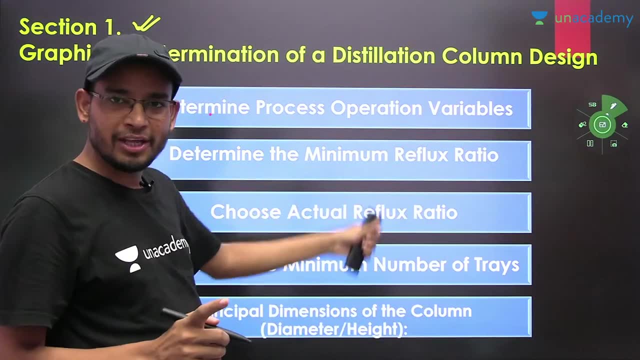 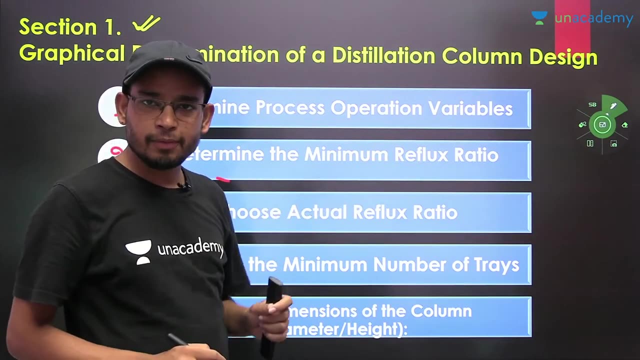 Today's session will be about this. only Understand very carefully. So the first objective will be that The operation variable will have to be defined. Ok, I am giving you an overview. The second thing we will talk about. The second thing: we will talk about Determination of the minimum reflux ratio. 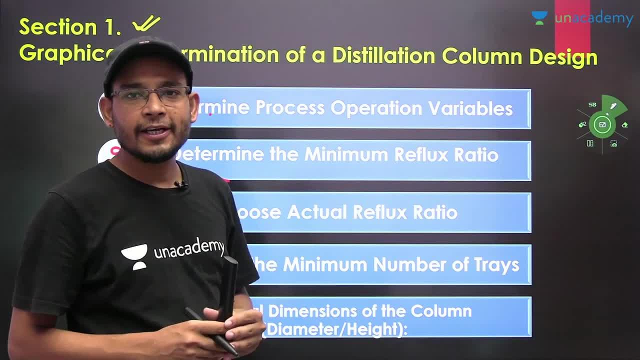 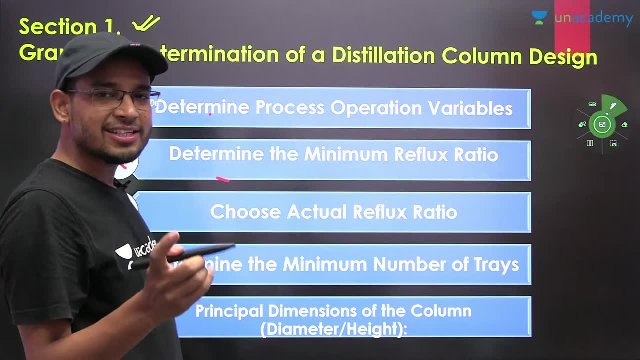 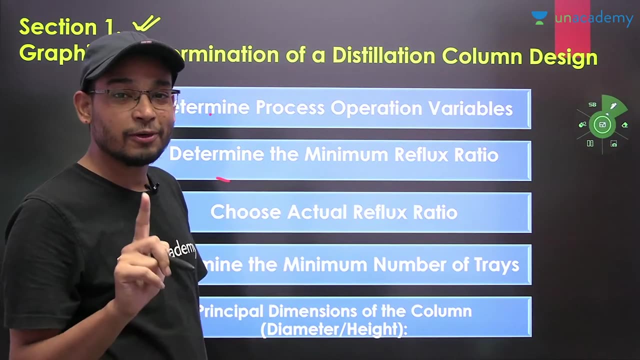 Ok, How to calculate the minimum reflux ratio, We will talk about this in the second step. Right In the second step, we will talk about How to determine the minimum reflux ratio, What you were finding theoretical, It will not be like this. How to calculate the minimum reflux ratio in design. 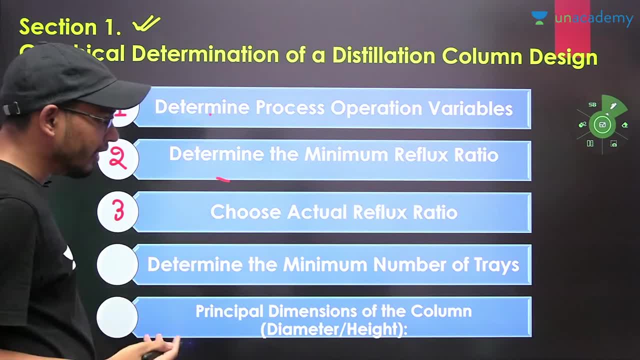 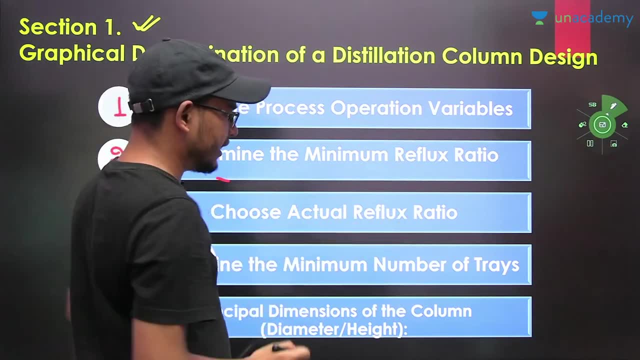 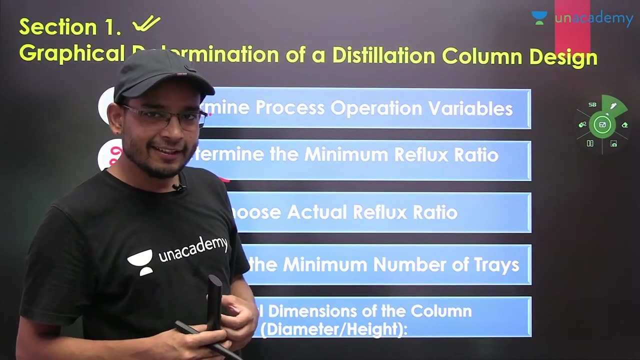 We will talk about that. The third one will ask you this: Tell me the steps for determining. You will have to mention in this way. Third one: Choose the actual reflux ratio. We will not be able to operate on this. We will calculate the minimum reflux ratio. We get an idea. 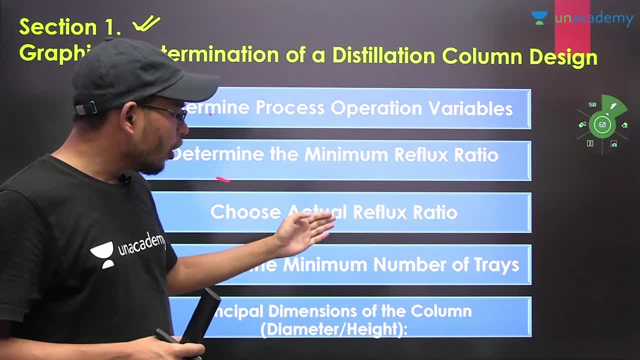 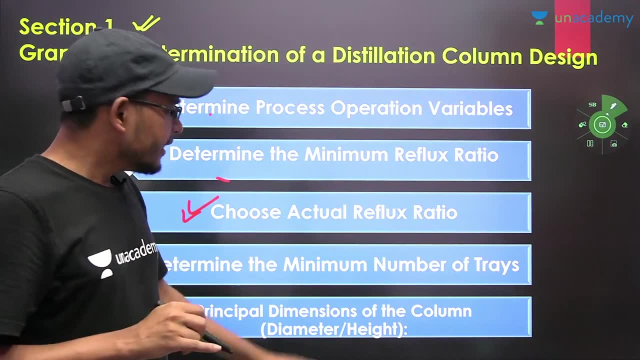 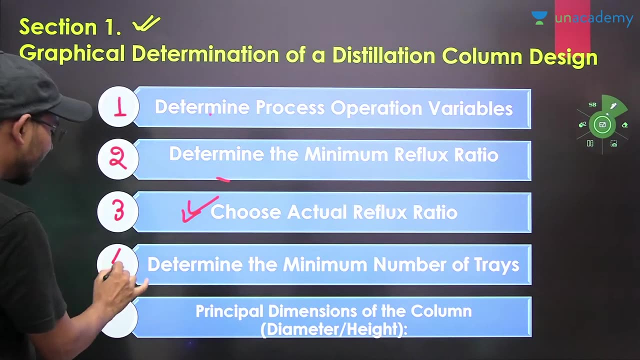 You can separate the system maximum, But On which you have to operate. You have to choose the actual reflux ratio On which you have to operate, On which you will operate the system. What will you choose? The minimum reflux ratio, Fine. third point. I will talk about the fourth point. 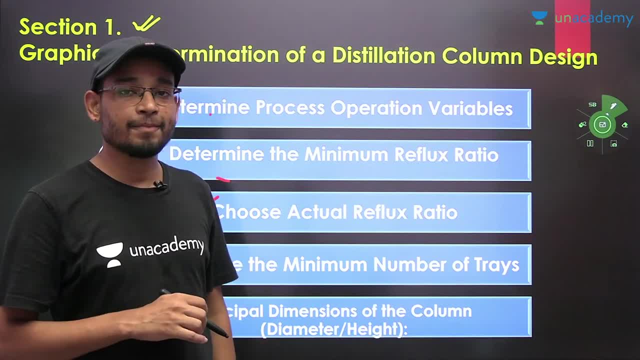 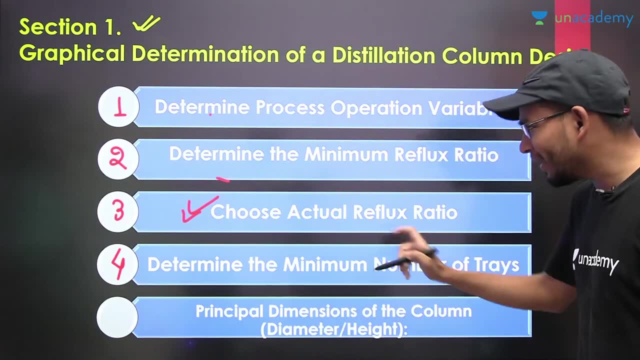 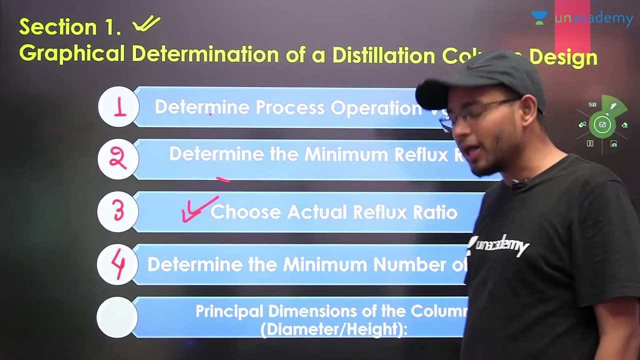 Determination of the minimum number of trace. So, first of all, what will you get? Minimum number of trace. How much minimum number of trace Will be required to operate the system? We will talk about this. Four parts will go on Day by day: Principal. In the last you will talk about 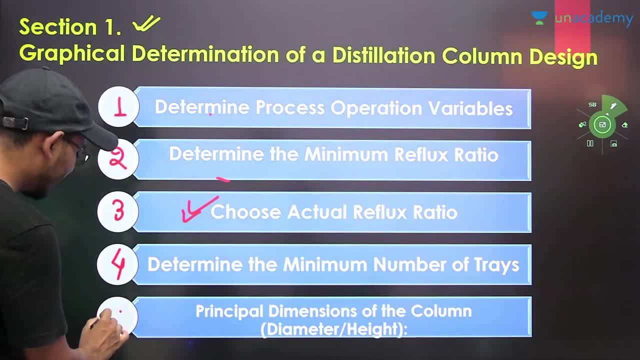 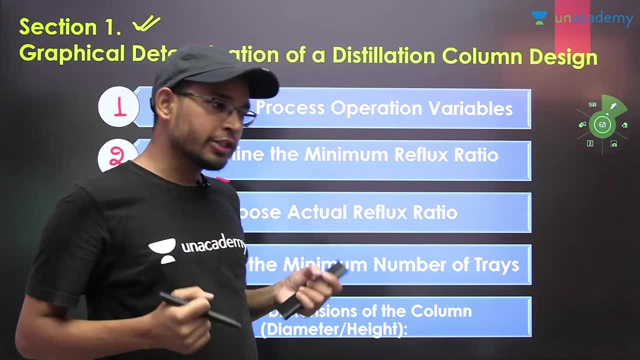 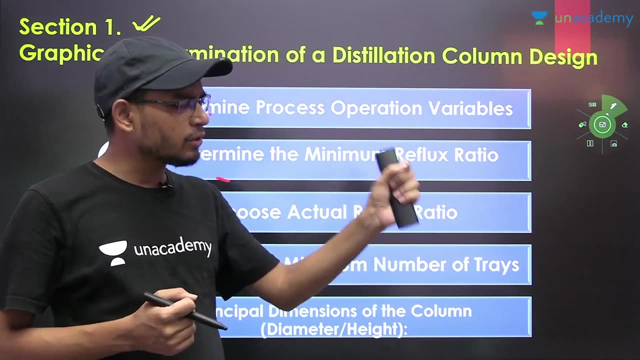 Physical diagram, Physical representation, In that we will talk about Dimensions. How will you choose the height of the column? How will you choose the plate of the column? How will you calculate the efficiency of the plate of the column? We will talk about all these. What is the bubble cap? 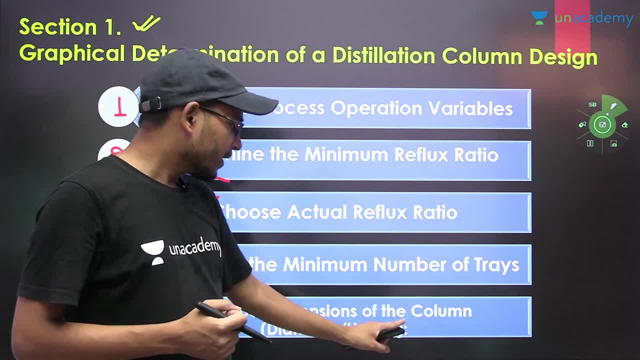 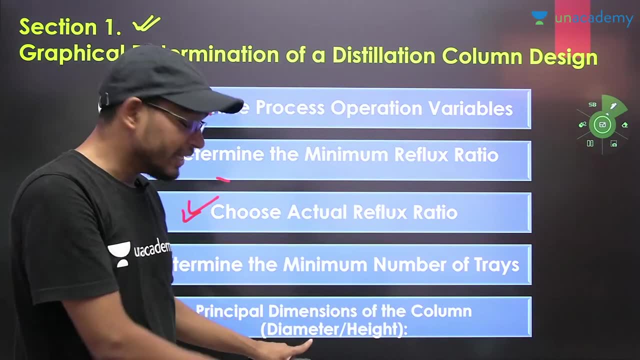 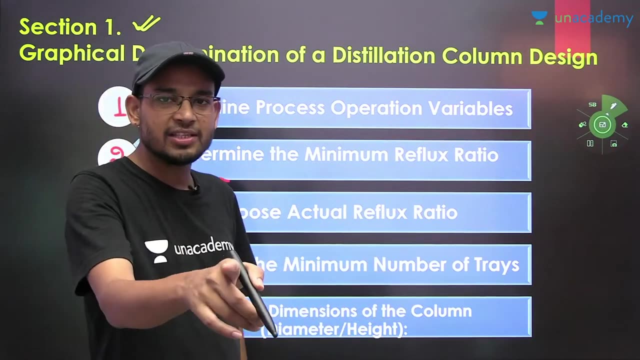 What is the seep cap? What is the packed wet? We will talk about all these. How will you choose the height? What is the concept of diameter? This question has come in the gate. This question is of designing. There are two numbers in this. One comes from operation. 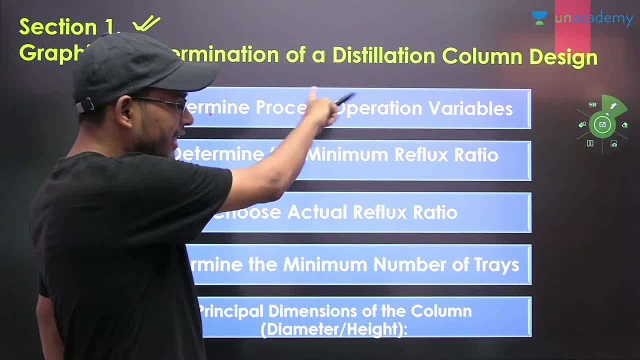 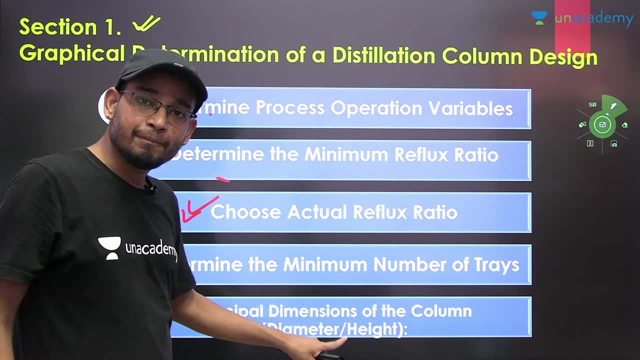 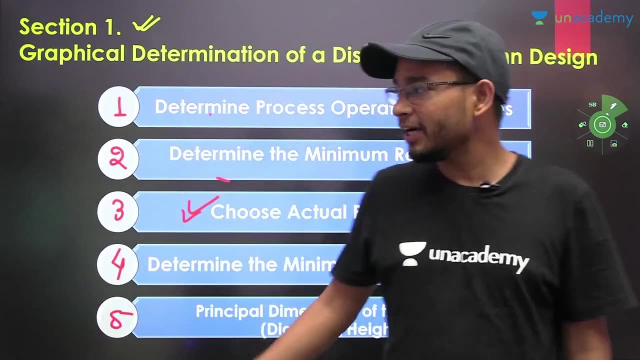 The other comes from designing. When this part of designing is covered, Then you will be able to talk about it. So you have been asked About diameter calculation, Right? So we will talk about diameter calculation. So these are the five objectives To define the system. If you have to define any particular thing, 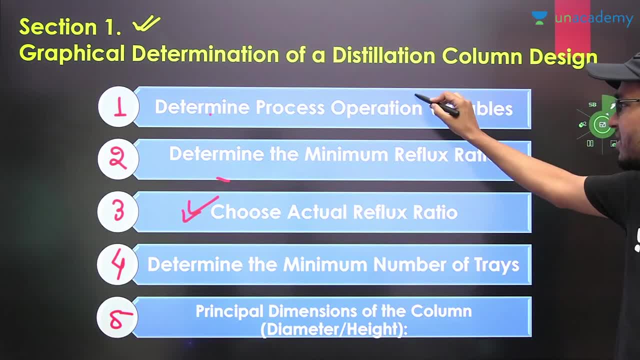 Then you have to work on these five things: First of all, you have to define the operation variable. Then you have to calculate the minimum reflux ratio In the second step, Then you have to calculate the actual reflux ratio. Then you have to calculate the number of trays. You have to take out the number of trays. 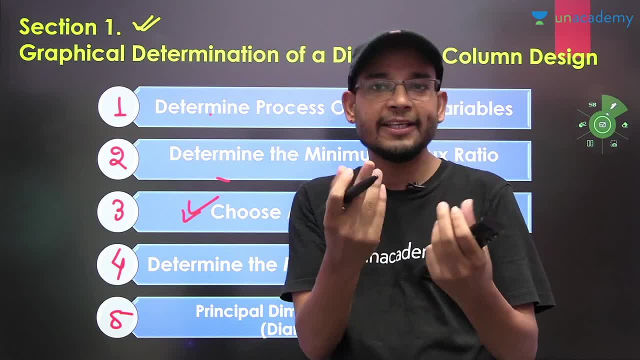 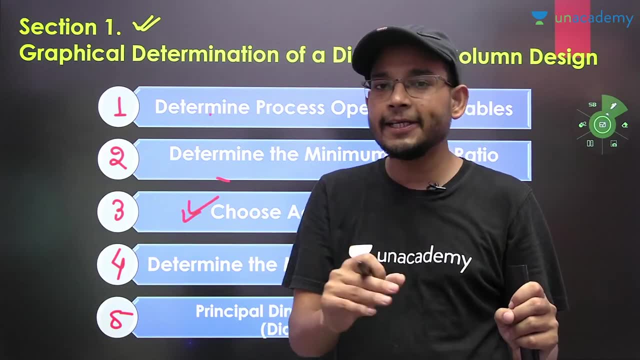 You have to take out the number of trays in the column. The main thing was how many trays will be required For particular separation. If you want to take out the number of trays, You have to take out 80%. How many trays will it take After the tray? 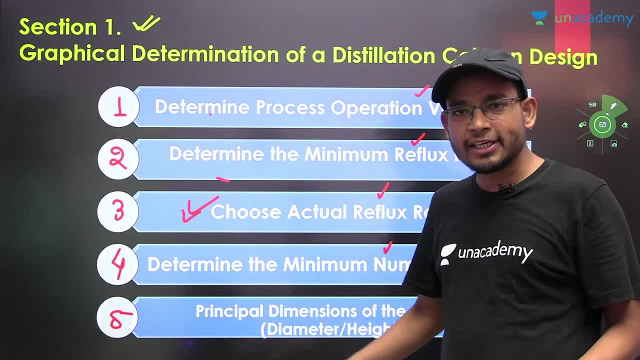 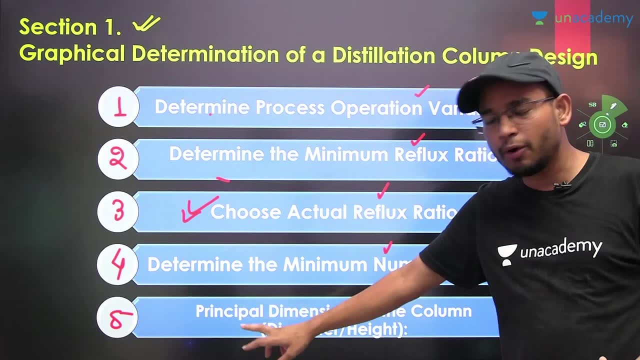 You will decide the diameter and height. In the last part The height and diameter will depend on. Then you will calculate the flow rate. Then you will calculate the flow rate. Then you will calculate the flow rate. Then you will calculate the height and diameter, Then you will calculate the flow rate. 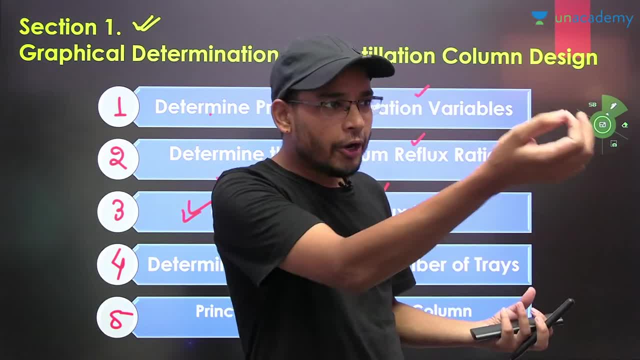 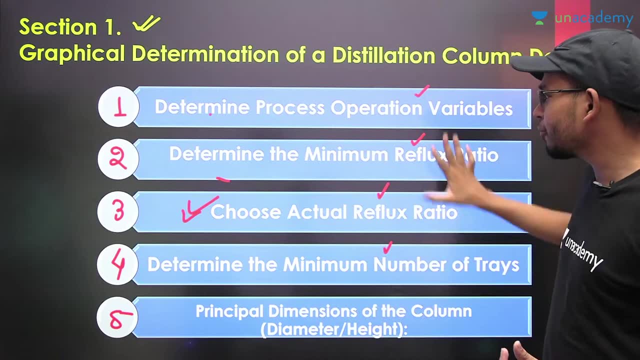 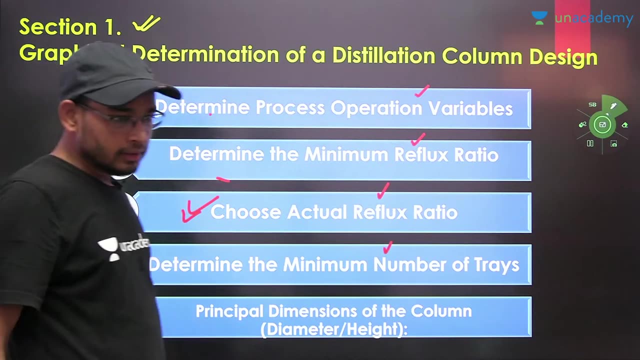 And you will calculate the thickness So that we can calculate the thickness, Because you will know the pressure And everything. So first of all You have to understand the overview, What we are going to do in the whole process. So many things have to be discussed In the first part. 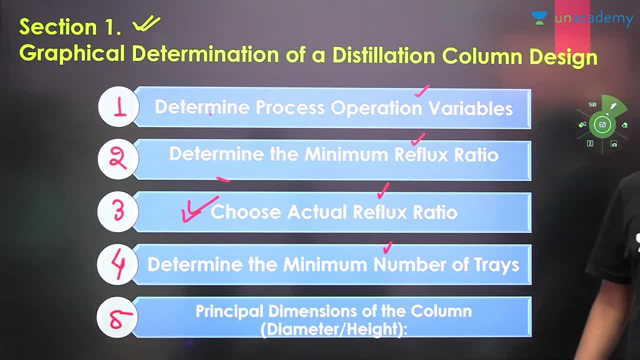 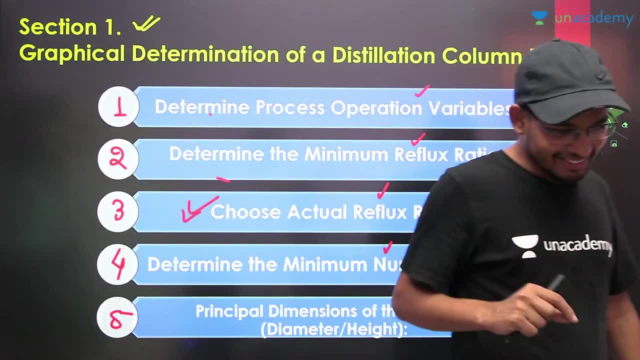 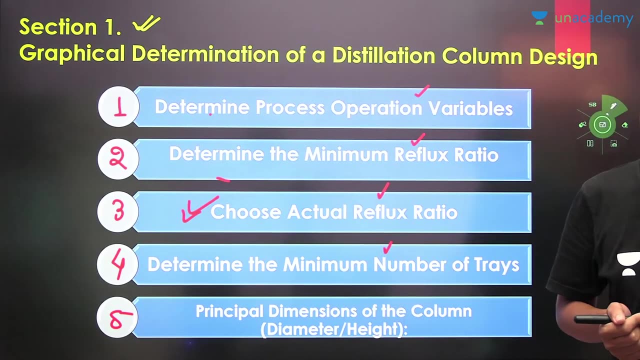 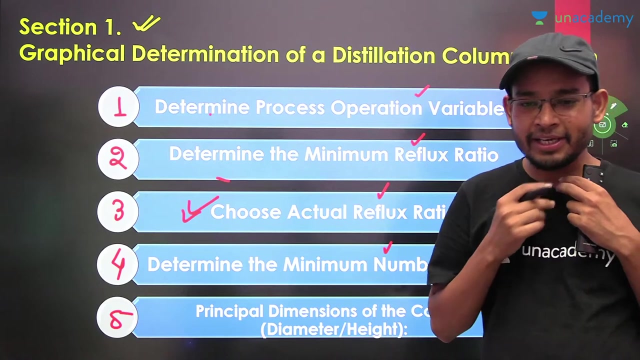 Ritik Rajput, You were from Chemicals. This is not forcibly. you can leave if you are having fun. then you can see the session. Yes, yes, yes, very good. MR100, oh, lovely, okay, is there any problem with the mic? 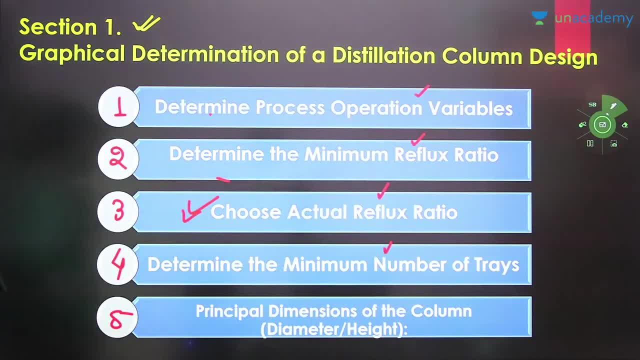 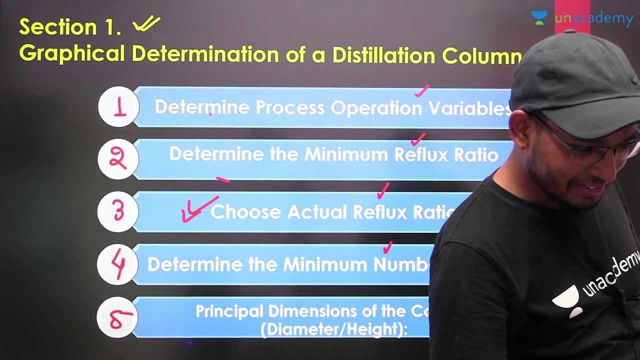 Wait a minute, I am fixing the mic. wait a minute, I am replacing the mic after this: Hello, now see everyone now. perfect, now there is no problem. if you will have fun, then civil people can come. there is no problem. 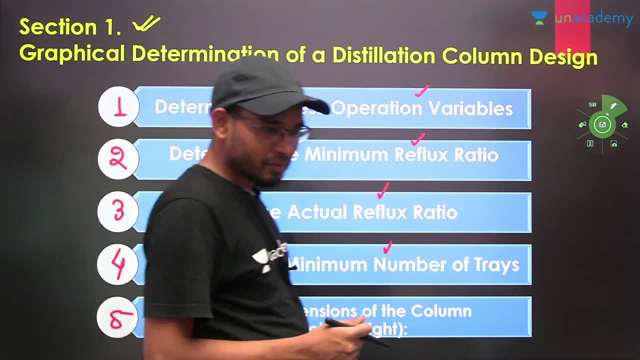 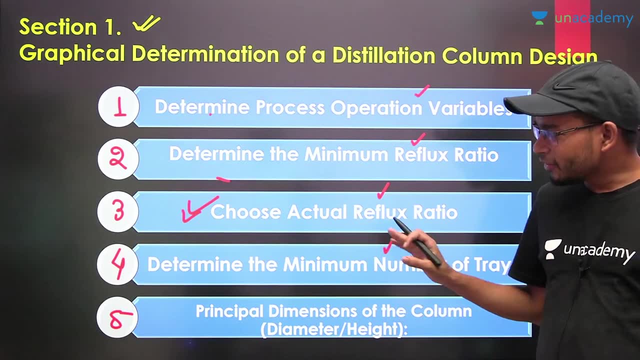 Now see. is there any problem with the mic Right? let's go, So all of you can see the session Now. everyone got this much to understand, right? If we will design any column, then which parameters we will take care of? 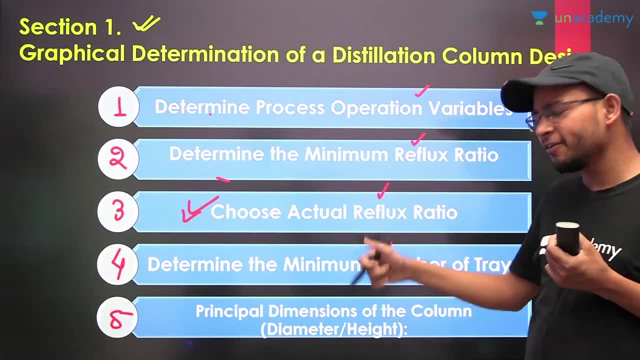 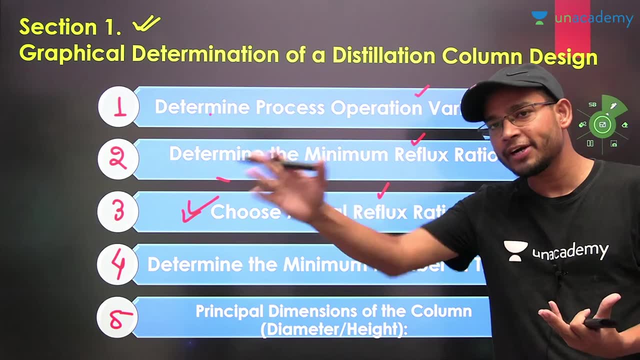 First of all we have to define the variables. then we will calculate the minimum reflux ratio. then we will calculate the actual reflux ratio. then we will define the minimum number of trace. how much minimum number of trace will take for particular separation. then we will define its dimensions. okay, 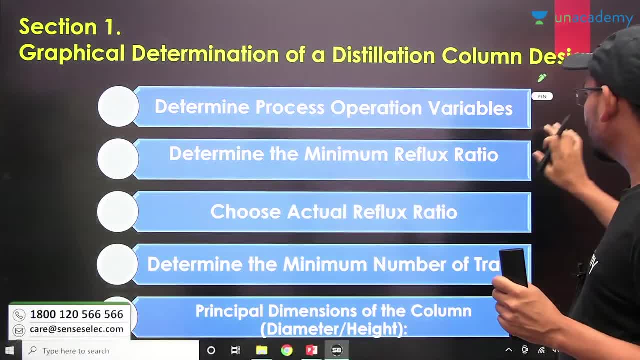 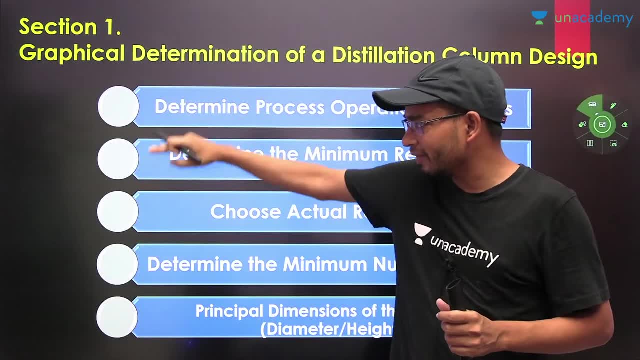 This much we should know first understand. Now I will talk from here. shall I talk from here? Yes, now I will talk after this step one. Now I will talk about each step one by one. I will start talking about these five steps one by one. 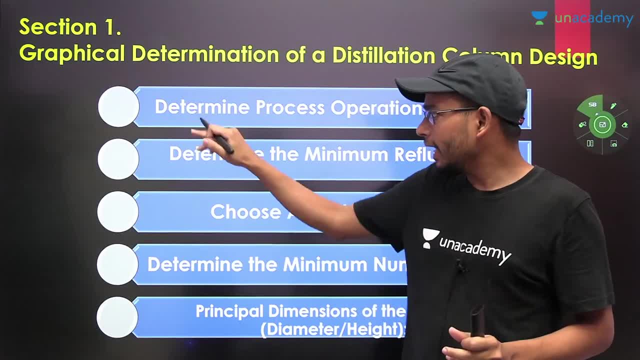 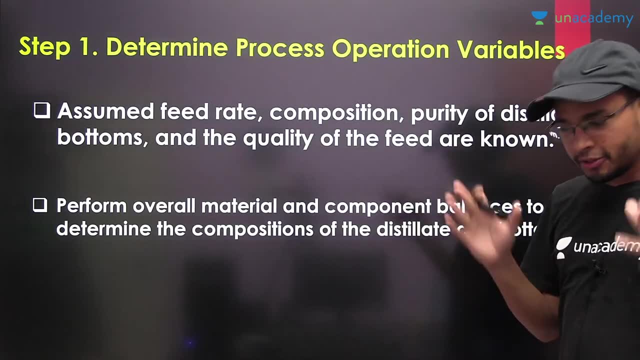 So keep connecting the whole process. Now I will talk about the first step, number one. So what is step number one? Determine the process, operation variables. So first of all we have to define the operation variables. So what will be the operation variables? 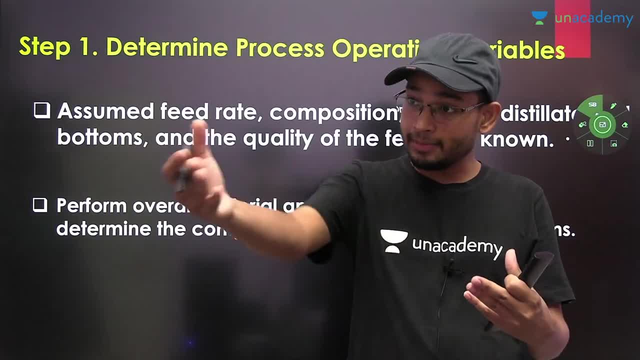 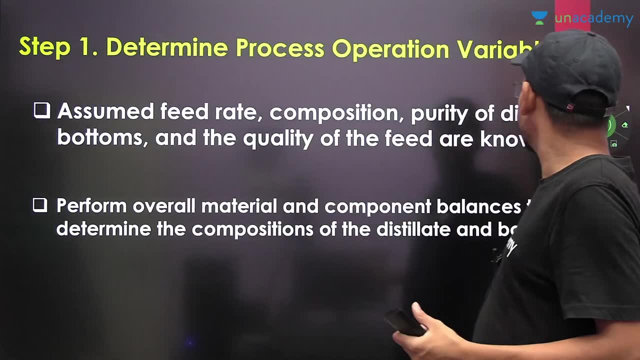 So you will have to say in the interview there He will tell you: tell me a little bit of designing. So first you will say that, sir, we have to define the operation variables. Which operation variables will have to be defined, See, I will tell you. 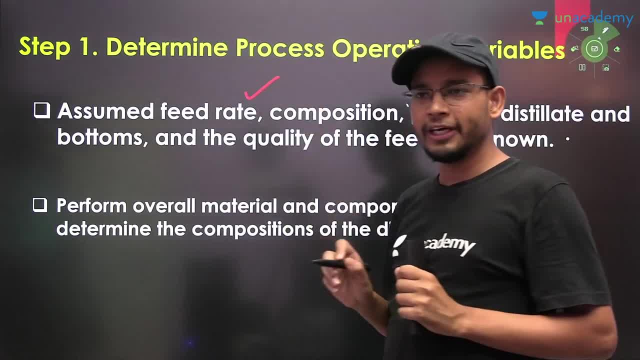 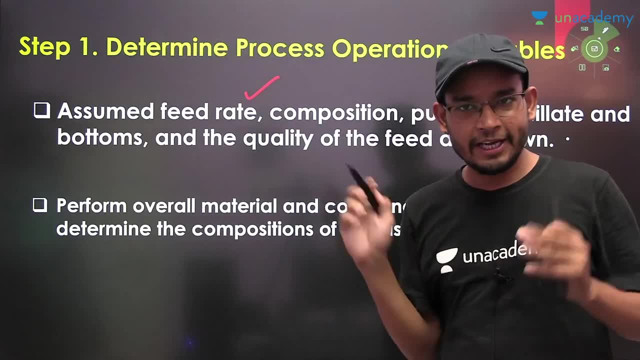 You will assume a feed flow rate You want to send in respect to 100 mol per hour, The rate at which you want to send. So you will define the feed flow rate, Or you can go the other way, In case you have asked someone for it. 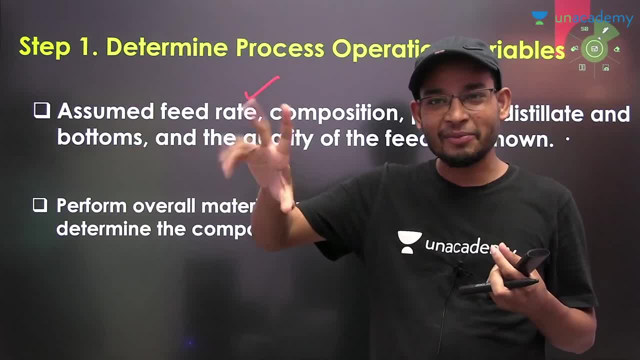 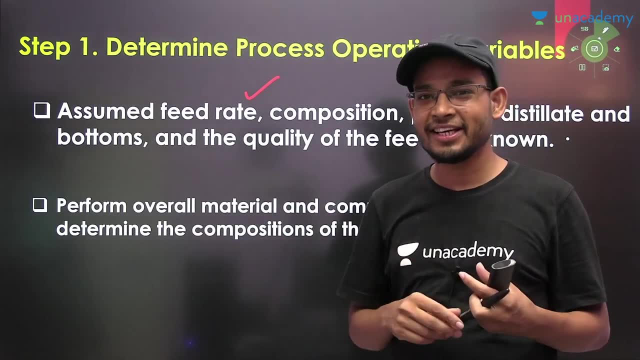 You have asked for columns from ONGC etc. Now the diameter of the column is fixed. Then you will change your feed flow rate. You can also go back. Suppose you have set up your industry And you have gone to ONGC. 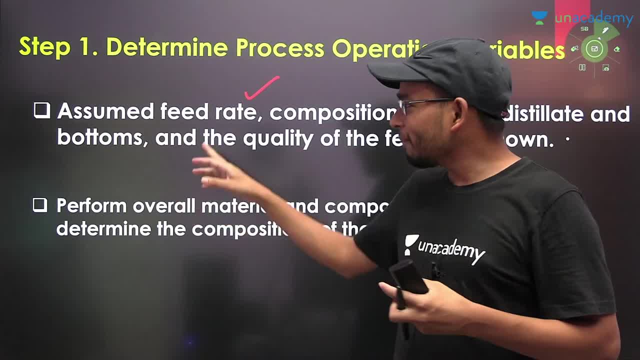 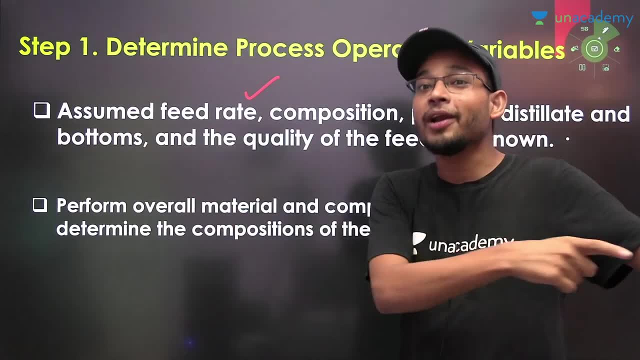 Sir, do you have any old column? Give it to me. So you have brought the column. Then you will not assume the feed flow rate. You will calculate the feed flow rate According to that column. What are you doing now? You will define the column later. 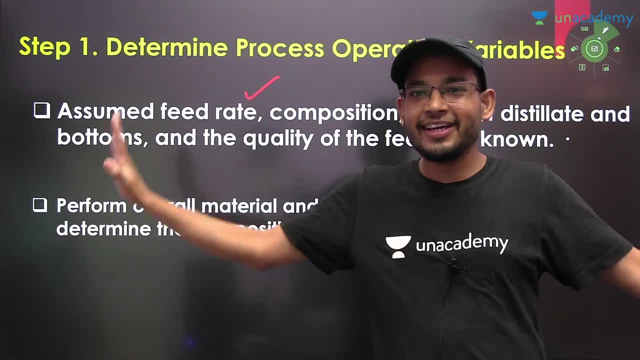 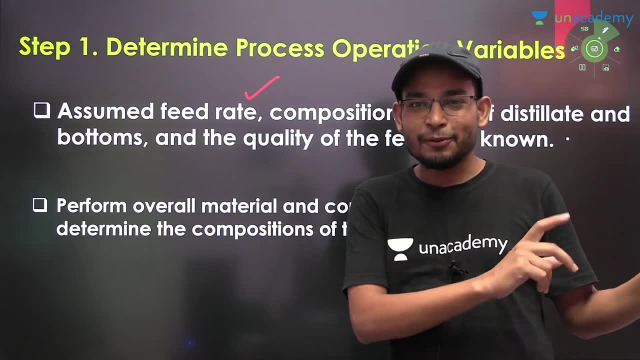 You will define the column later. You have nothing, I am going straight. Then you have nothing, Then you will define the feed flow rate. Feed flow rate is decided by the column diameter According to that column diameter. So we will first assume the feed flow rate. 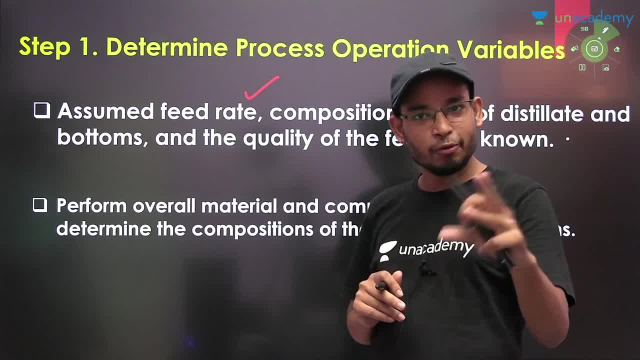 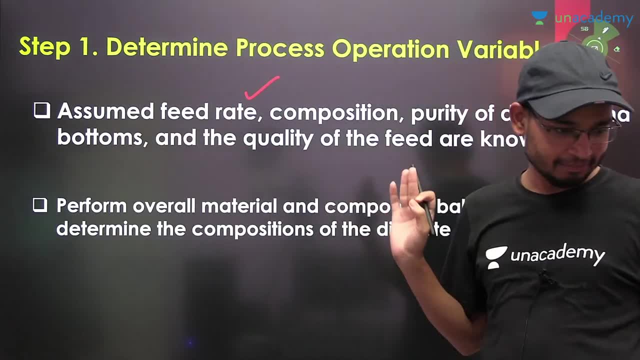 And this can also happen. I have told you this. You can go the other way. In case the column is first, Then you will define the feed flow rate according to the diameter and thickness of the column. It can be done in both ways. 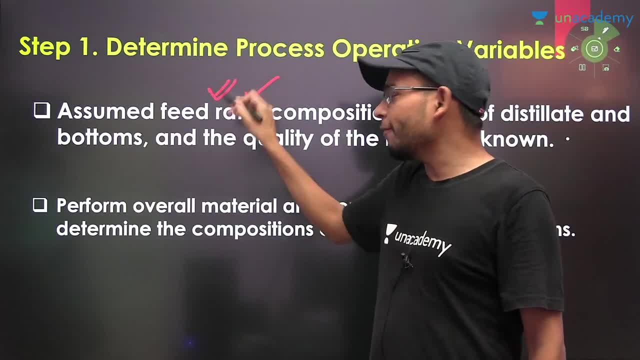 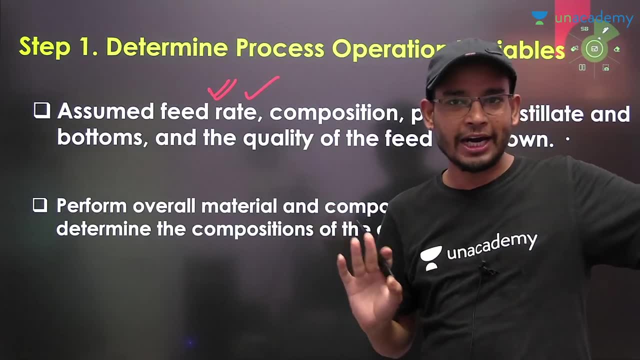 Right. So understand very carefully. So you will define the feed flow rate first, That we have to get entry with this much flow rate. Then you have to see the column diameter, thickness and height. You have to talk about that Then what we have to do. 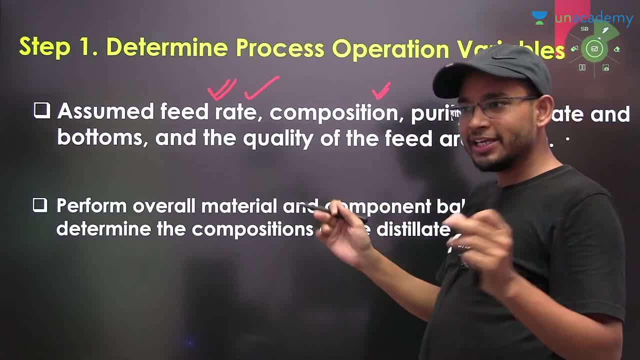 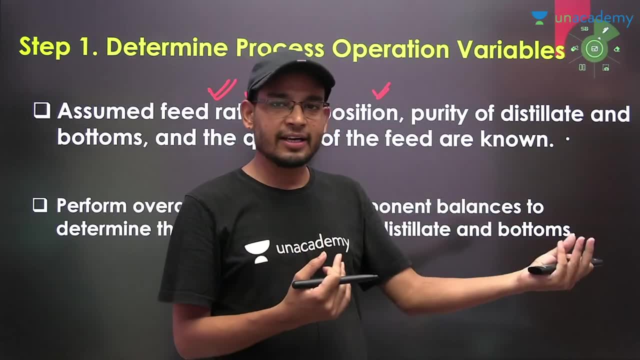 The feed you are bringing. You should know that. the light components in the feed, What are the mole fractions of them? You will measure this first. There are many devices to measure the composition. Okay, So the light components and the heavy components. 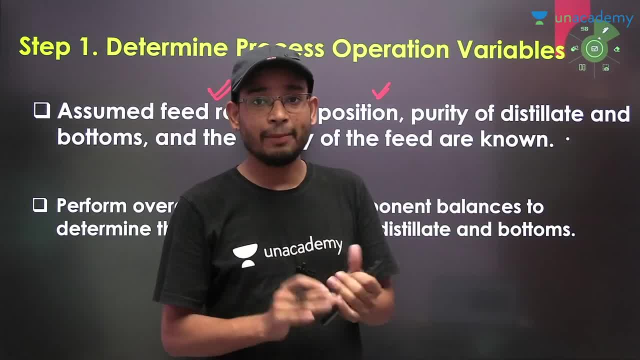 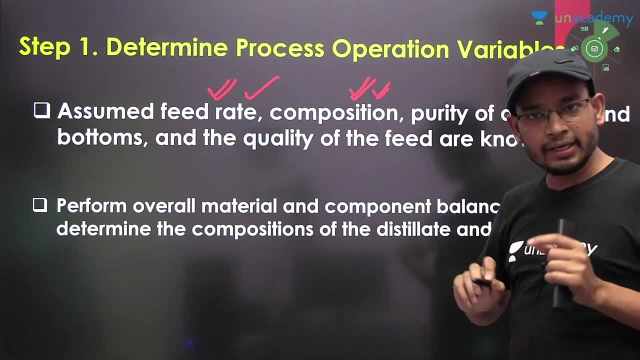 You will know the compositions of the feed, The feed you are adding, Suppose you are adding crude oil. So you will know the compositions of crude oil first. So you will define those compositions. Okay, Right, I am talking about the feed composition. 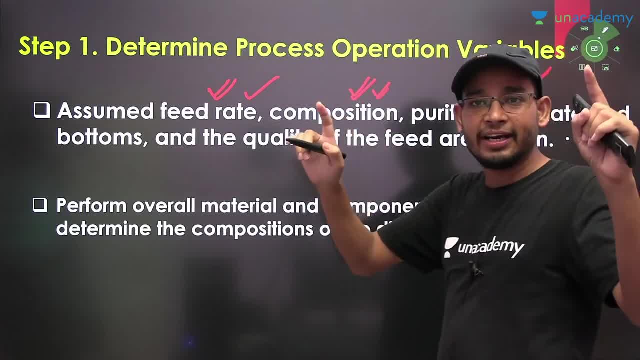 Now You have to see the quality of the distillation Means. what is the demand in the market. According to that, you will design the system. Okay, You will say that no sir, We need 95% methanol, We need 95% alcohol. 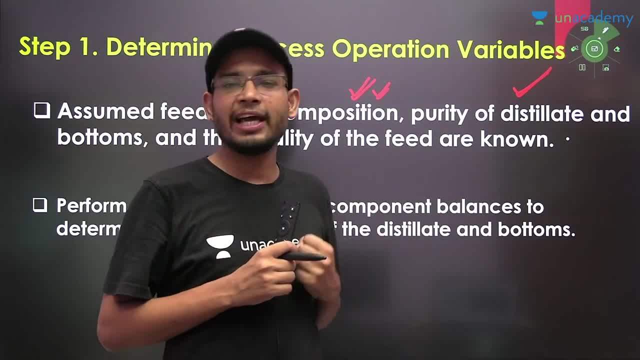 Okay, That much I have to distillate with high purity. Then what will you do? You will define this first, The value of Xd That we need: 95% desire, Okay, So you will define this And how much should come out in the bottom. 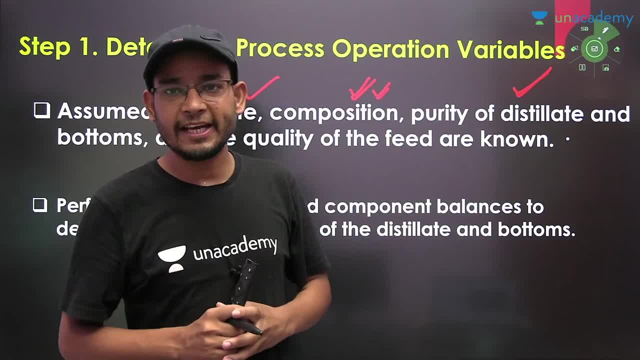 You will set this also: How much will come out in the bottom. You will set that only. If it comes out more, Then you will adjust it with the reflux. Okay, So you will define this And how much should come out in the bottom. 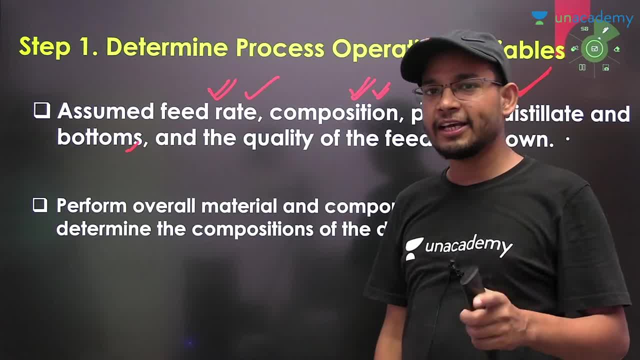 You will set this also. How much will come out in the bottom? You will set this also. How much will come out in the bottom? You will set this also. If it comes out more, Then you will adjust it with the reflux. 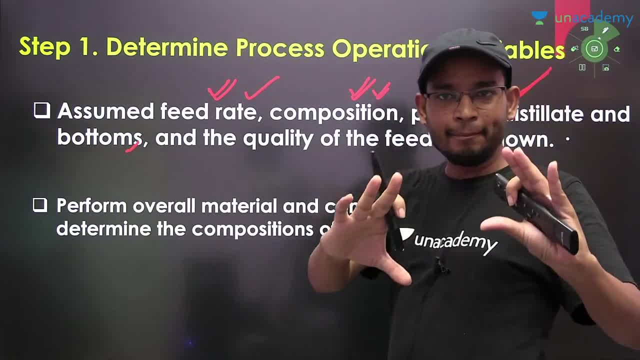 Okay, And when you are bringing feed? So the feed is your vapour, Or is it liquid? Or pure liquid Or is it full vapour? You will have to define this first. Okay, Very important thing is going on here. 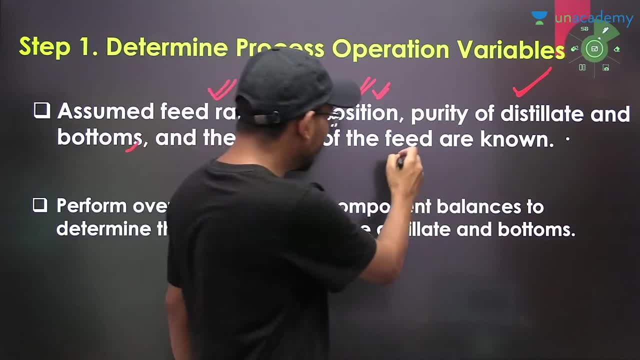 Okay, You should know about feed first, Means, all the information related to feed. You should know What type of fluid are you getting processed. Okay, So first of all, You have to know about the feed, Means, all the information related to feed. 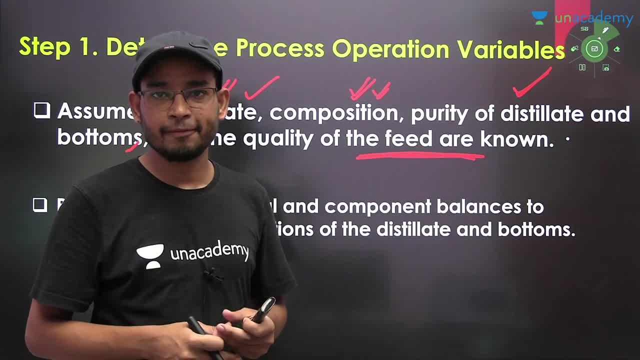 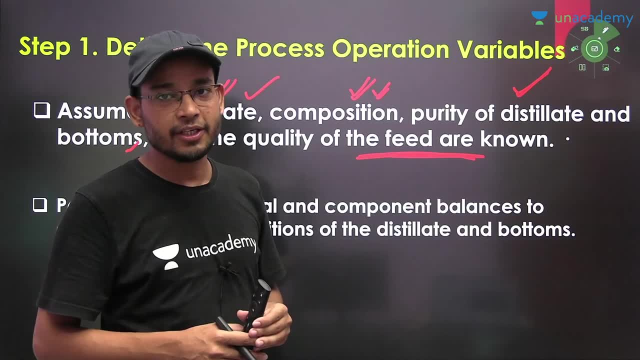 You should know What type of fluid are you getting processed. Okay, So first of all, the story of feed should be clear in the process variables and operation variables. You should know the composition of your feed. What is the quality of the feed? 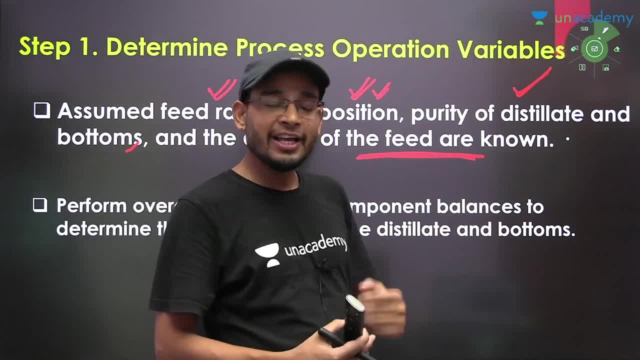 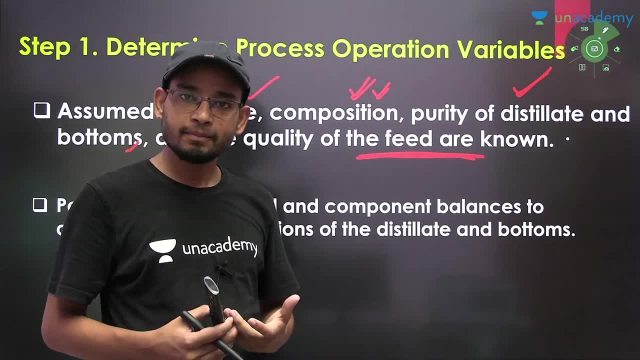 Quality means your feed is full of vapour or liquid or mixture of liquid and vapour. So you should know about the quality of the feed, So you should know these parameters first. only then you will be able to define the number of trays, etc. 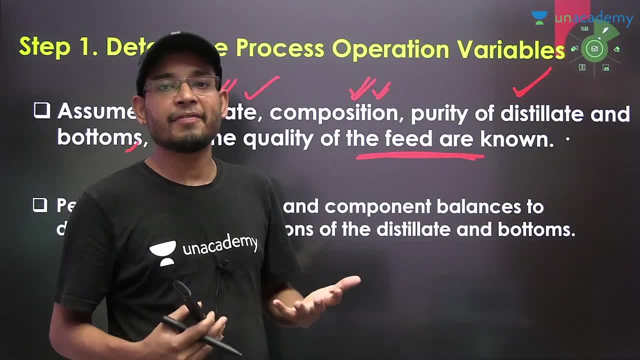 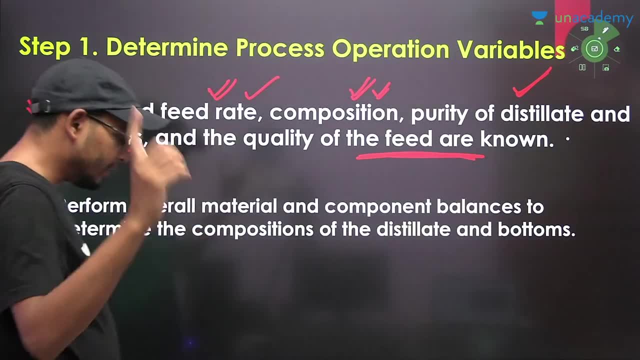 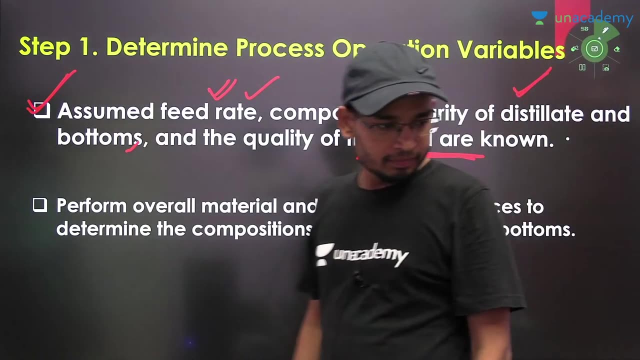 Trays, reflux ratio, etc. only then you will be able to define it First. you should know this much: Did everyone clear the first step? Everyone will tell me once: Did everyone clear the first step? Sir voice, It depends. 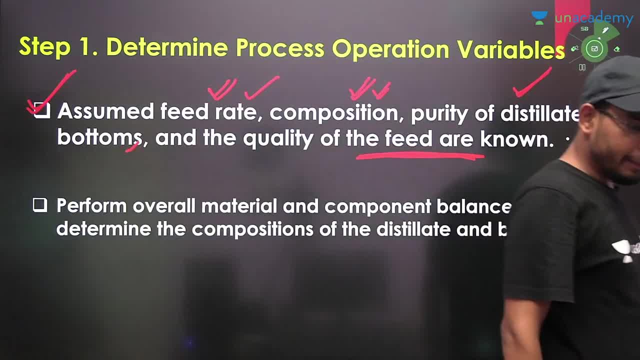 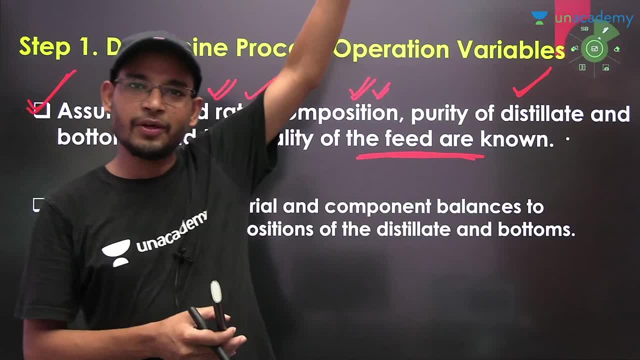 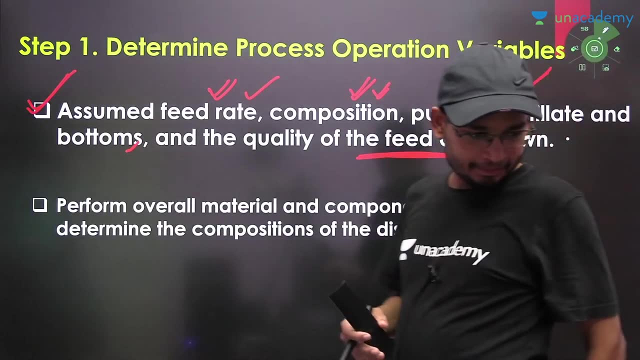 Column is very big. Okay, Did you put chimney at home? You must have seen chimney, etc. You must have seen chimney at home. You must have seen chimney, etc. These are such big columns. Okay, Everyone is clear about the first step. 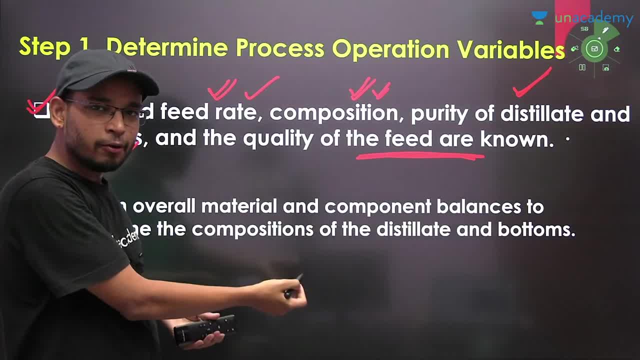 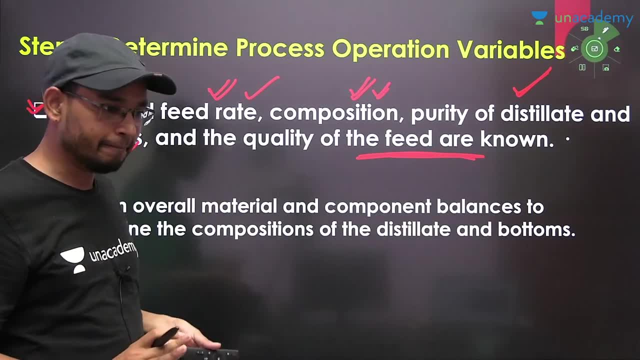 Keep understanding properly And now read the designing in such a way that if there is any question in the gateway of designing and if anything is asked in the interview, then you will define it in a completely concrete way. Okay, So everyone has understood this. 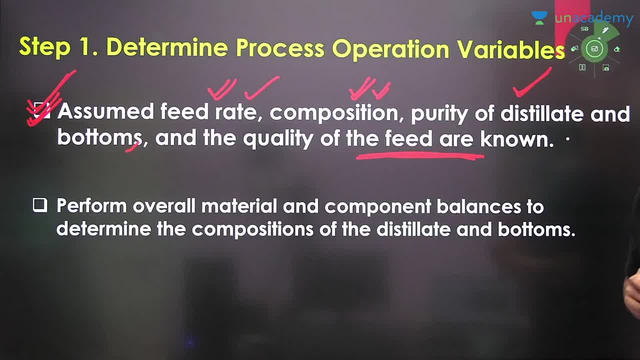 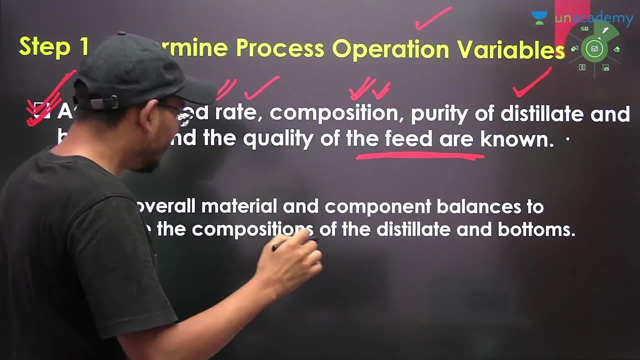 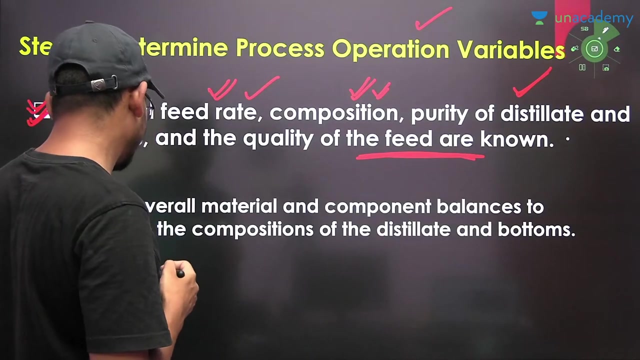 Now I will talk about the second step And what should you know And what will we define After this? the second operation you will have to do is to apply the overall material valence. You will apply the material valence to determine the composition of the distillate and bottoms. 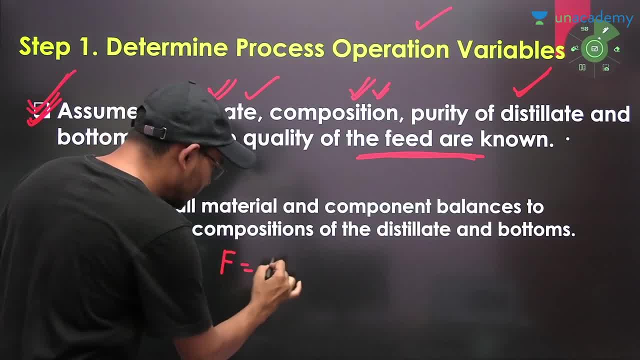 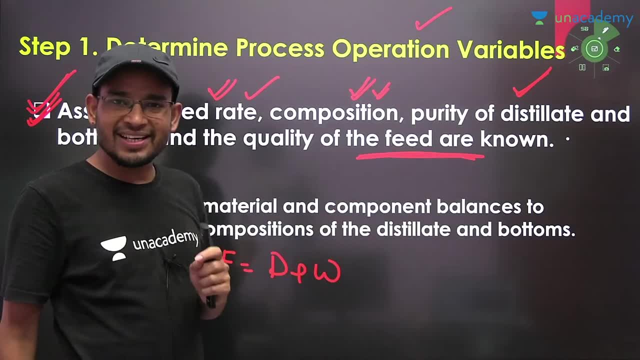 Yes, In case, how will you apply? the overall valence F is equal to D plus W. Okay, In case you know the flow rate. If the flow rate is known, then you can take out the composition. In case you want the composition to be fixed, then you can take out the flow rate. 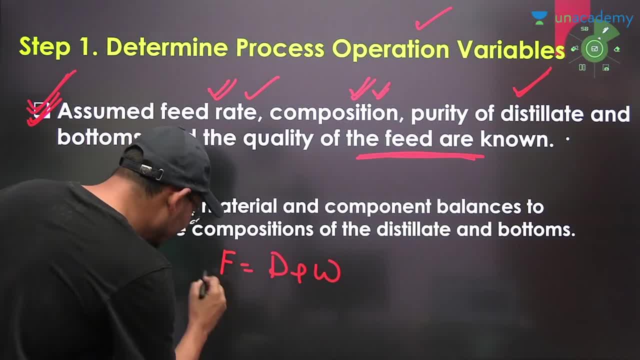 You can do it in both ways. So the component valence of this is the overall valence. You will apply the second one. Everyone will write it here. You will write the second one: F into ZF is equal to D into XD. 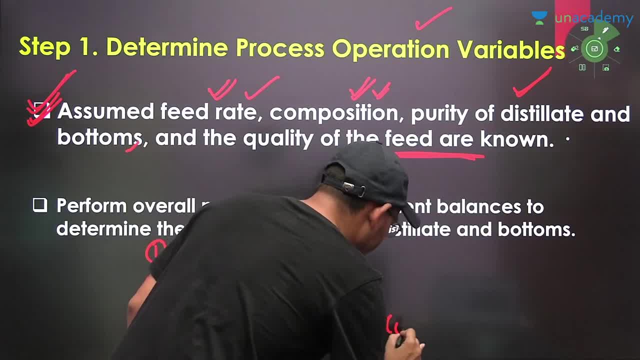 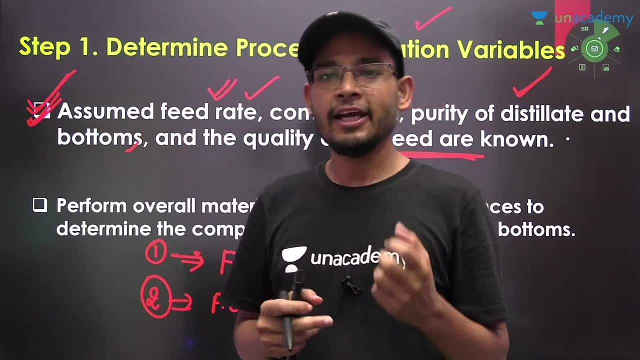 Which I have taught you, And plus W into XW. Okay, Whose composition is this Lighter key? Whenever you read in the distillation column, there is a heavier key and a lighter key. Lighter key is called those which are more volatile. 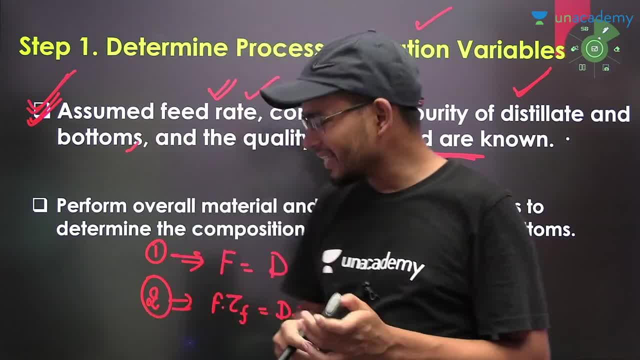 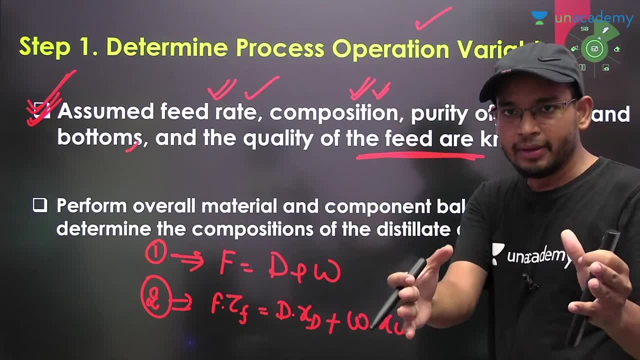 And how are the heavier keys More volatile? Okay, So always remember Whose composition is this Light key? Whose composition is this The light key? It is your mixture. Okay, It is a mixture, So there will be your heavier key and light key in it. 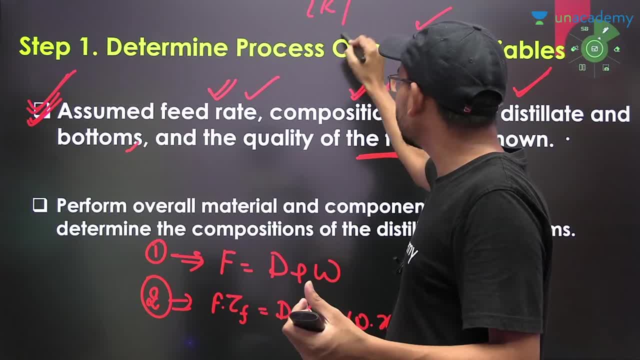 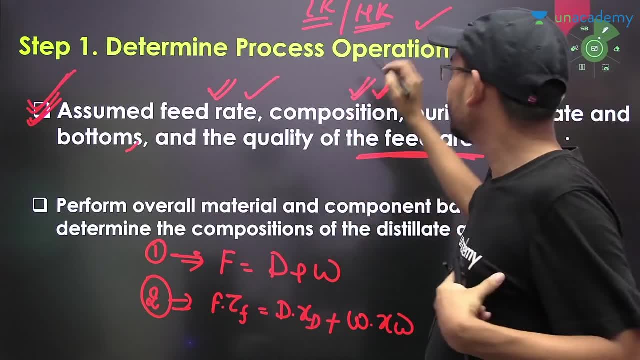 So light key- Write light key also. What is the meaning of light key and heavy key? Understand this. Heavy key means the less volatile component whose boiling point is more Okay. What will this be? Less boiling point component- Okay. 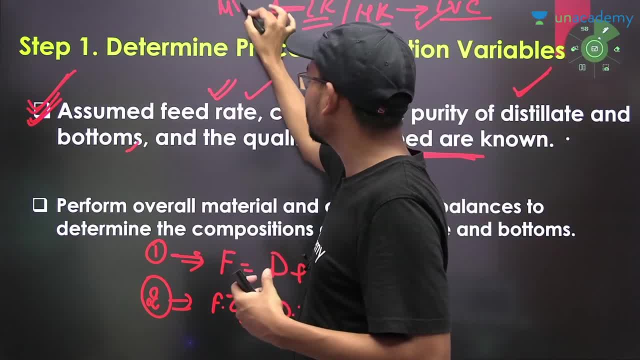 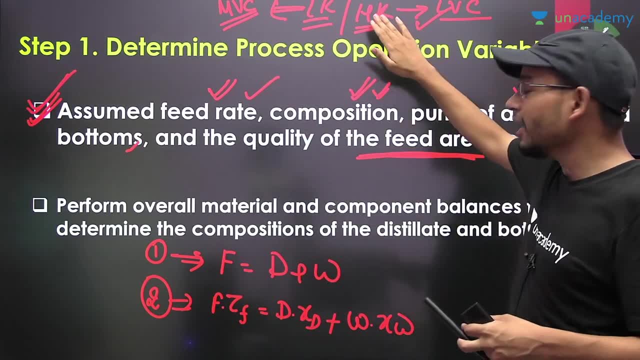 And the lighter key is called more volatile component. More volatile component means whose boiling point is less, Whose vapor pressure is high, Whose vapor pressure is less, and vapor pressure will be less and boiling point will be high. We call them heavy key. 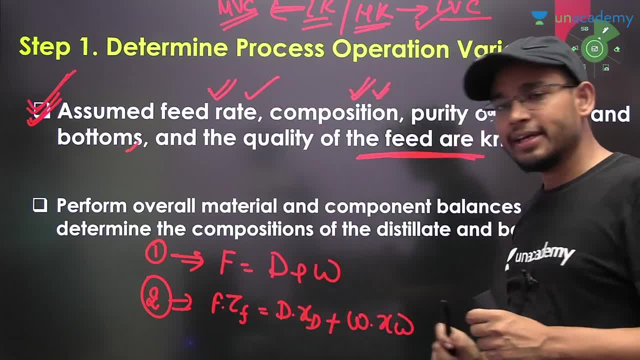 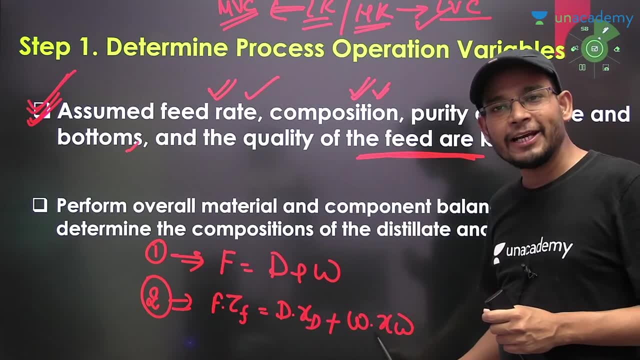 Okay, So the light key is their composition. Whose ZF is lighter key? Okay, It is the composition of the lighter key in the distillate. It is the composition of the lighter key in the bottom. Keep writing it. 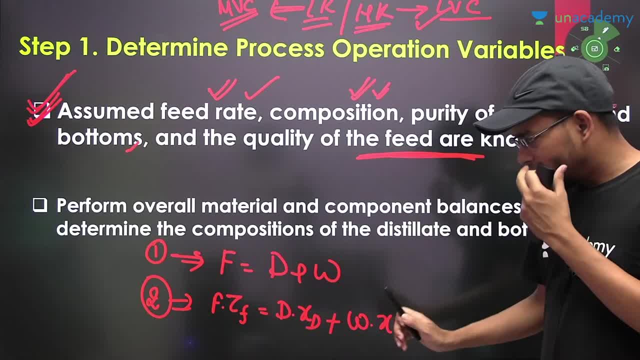 So this is overall balance and this is component balance. Okay, So, whatever things are unknown to you, so by using these things, because you will know the feed flow rate and you have defined DW, So you can find out the composition. 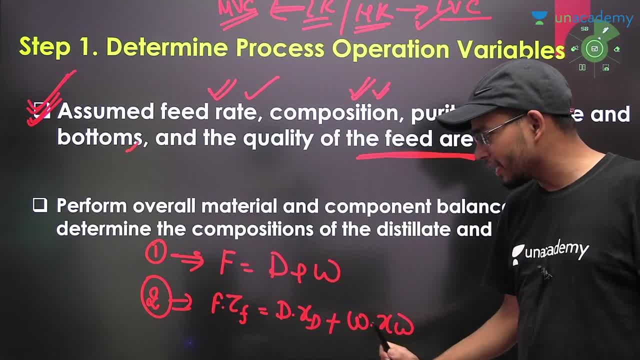 Okay, You will be able to get the value of XD and XW. Okay, In case you have fixed XD and XW, then you will be able to get the flow rate of D and W Like this. So you can write this: 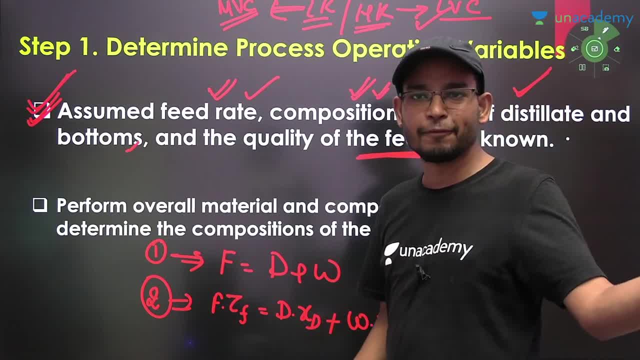 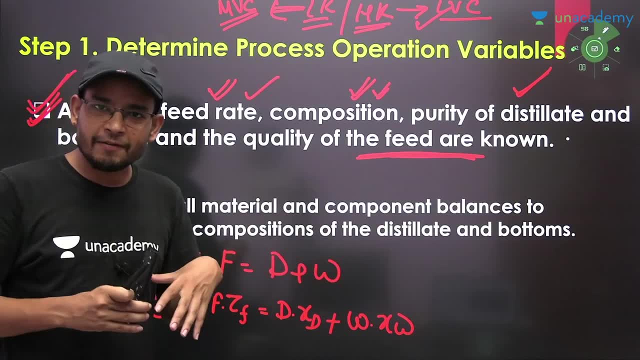 Okay, You will be able to calculate the flow rate of the distillate and the flow rate of the water. You will be able to calculate both things. you just need to know one thing: You will define the flow rate first, then you will be able to find out the composition. 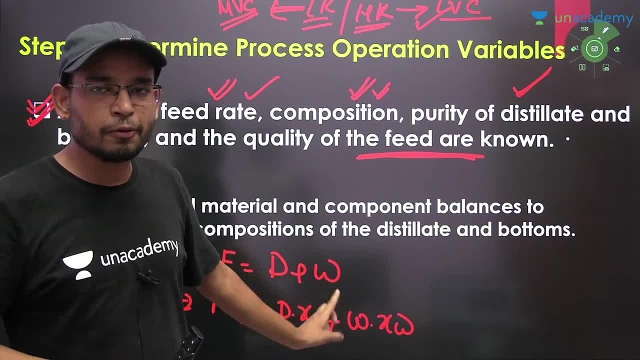 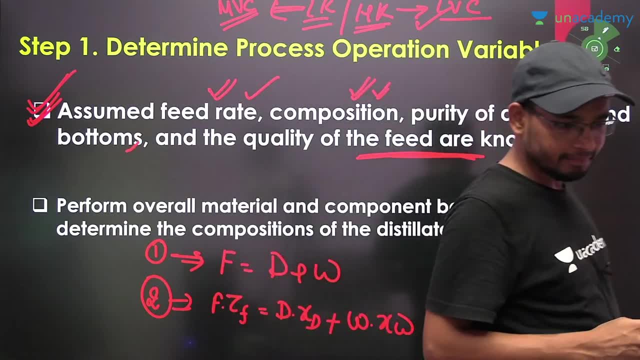 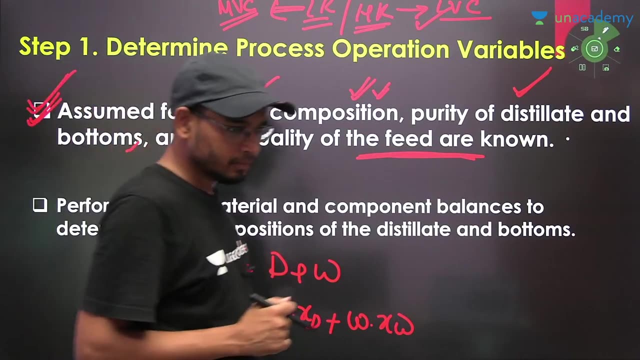 In case you have fixed the composition, then you will be able to find out the flow rate, With which flow rate we have to extract the outlet. Write these two things in a nice way. first, You can extract it by applying this operation. Yes, the quality of the feed will be changed. 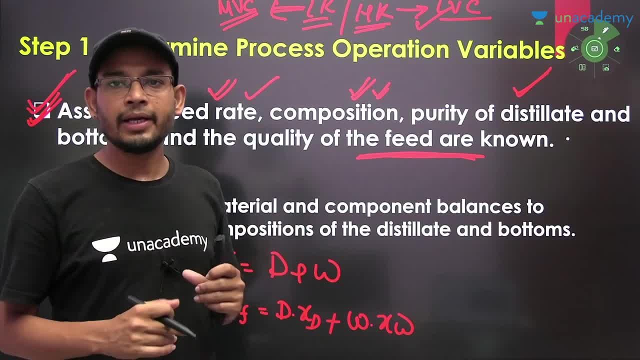 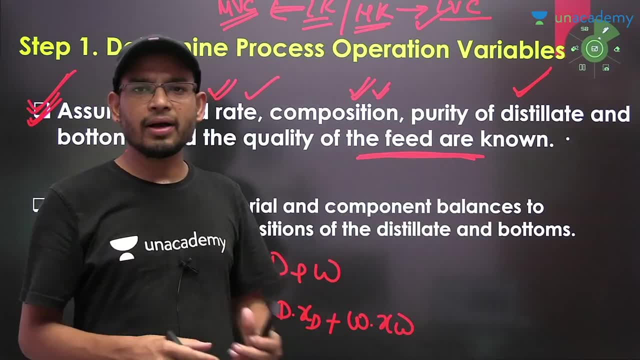 But we try that until one operation runs. the quality of the feed should not change. Whenever you do another operation, you can change the quality of the feed. It depends on how your feed is in it. In case your feed has more lighter components, then you send it like this: 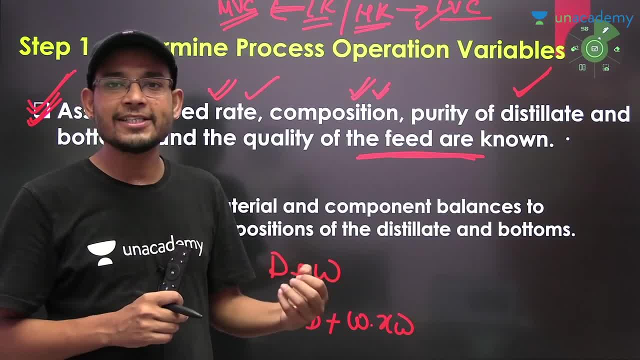 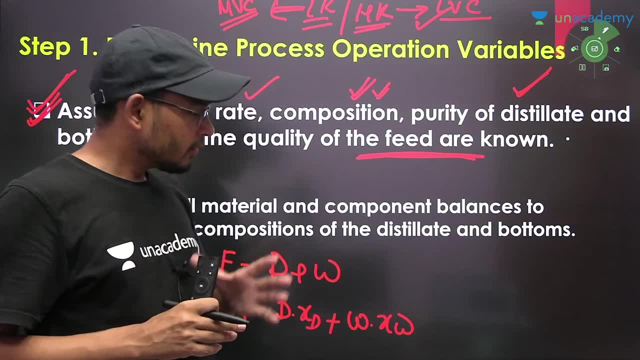 In case there are more heavier components, then you change the quality of the feed. We heat it a little and then we send it So that there is no load on your system. Okay, Surya, It depends on that. How is your feed? 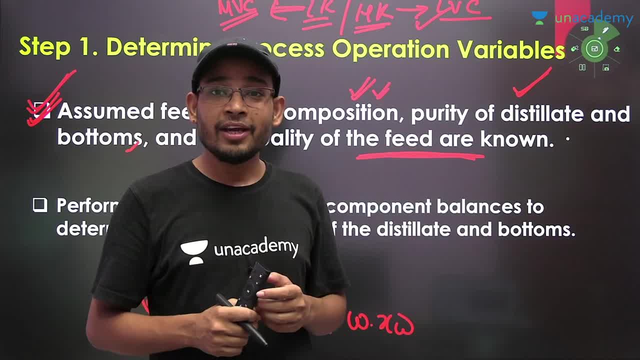 You came to know that you bought a cheap crude oil. What will happen in it? There will be less lighter in it and more heavier in it. Whenever there is more heavier in your crude oil, it does not mean that it is not useful for you. 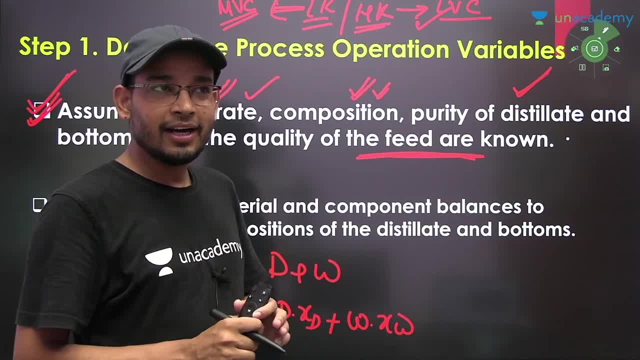 It means that you bought it cheap from the market. Okay, You will have to go to Saudi Arabia. You will buy it from here and there. If you buy it from China, then the Chinese will mess it up. It is also in China. 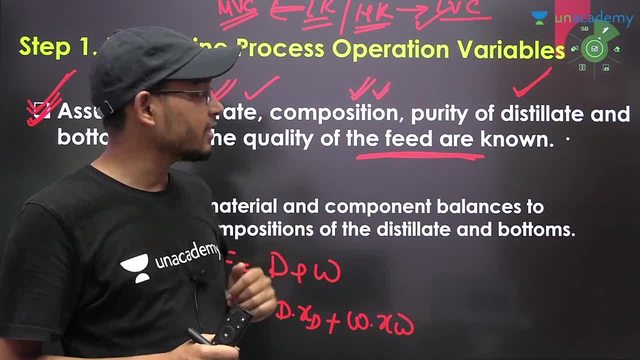 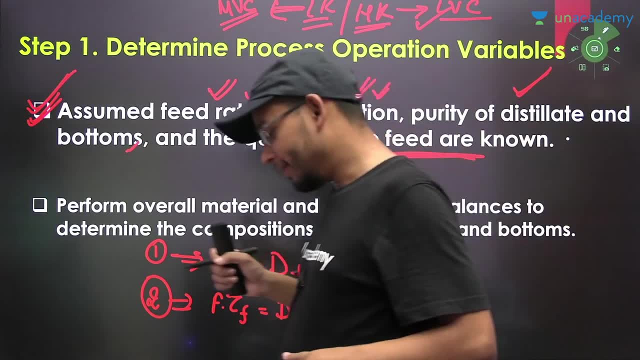 Okay, China does not mess up with India. You go to Saudi Arabia, You get it from Saudi Arabia. Now there is a problem with NGC with Saudi Arabia, So NGC is not buying from Saudi Arabia. Okay, In my time I was in HPCL. 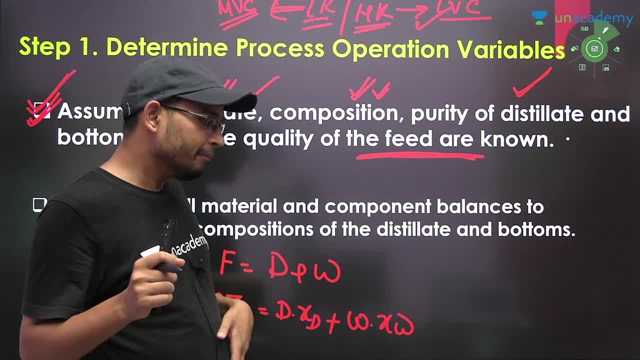 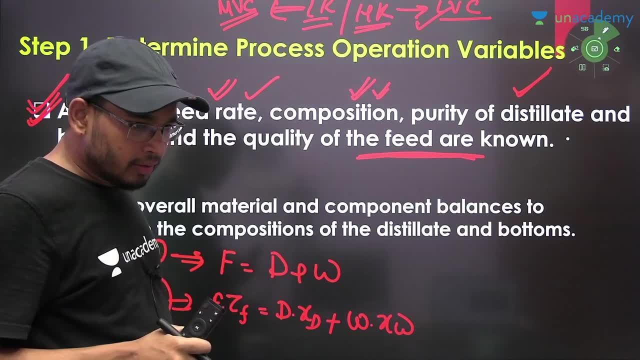 Then HPCL used to come. Yes, Reliance comes from the USA. Okay, So different companies have different crude oil. Go and Google it once. Yes, that is the story of TAN value. That is a different thing. I have already defined it for you. 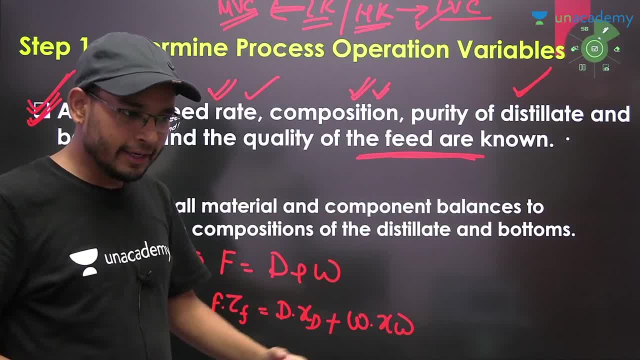 On the basis of TAN value. you buy crude oil in a nice way. Okay, On the basis of TAN, total acid number. I am telling you this Now. the designing part is going on, So I am not going too deep into it. 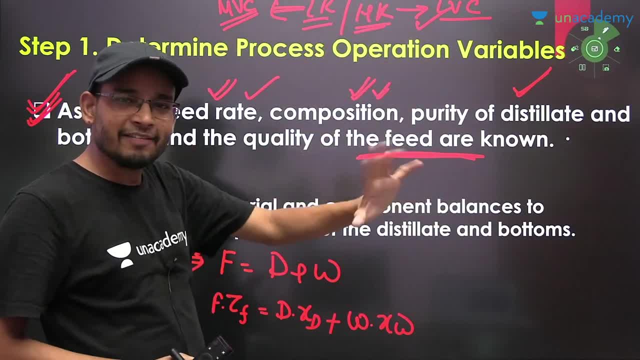 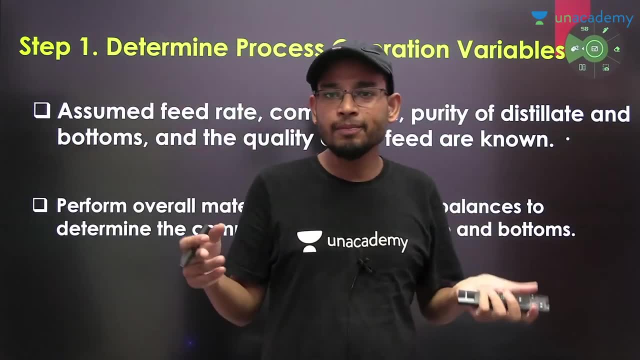 I started talking about TAN value, Then the whole lecture will go on TAN value only. Okay, Come on. So many things have come to everyone's understanding. What will we do Now? I will summarize it completely. First, we will have to define the operation variable of the system. 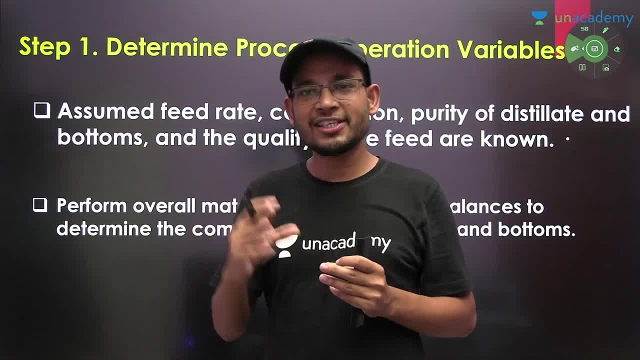 What is the feed flow rate in the operation variable? What is the quality of the feed? What is the composition? What is the bottom flow rate? We should know all this. Okay, After this I will just talk Here. you have applied material balance. 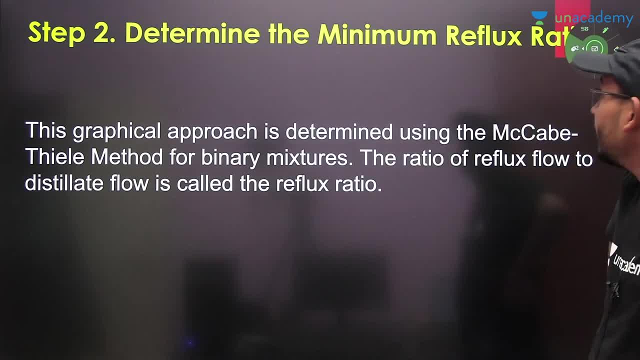 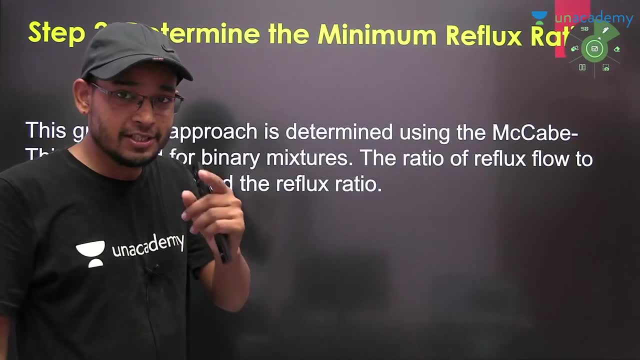 After this I will just talk. Determination is the second step. The second step is the minimum reflux ratio. Very, very important How to calculate the minimum reflux ratio. This is also asked in your gate And this is also asked in the interview. 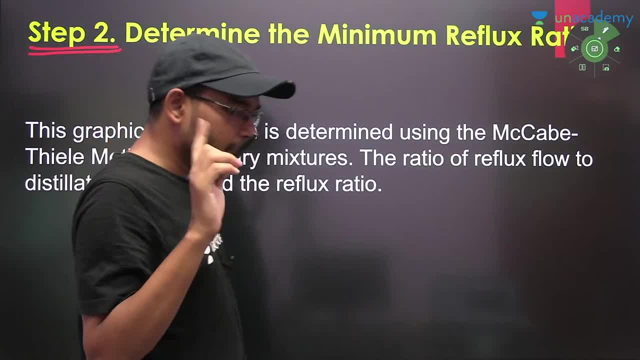 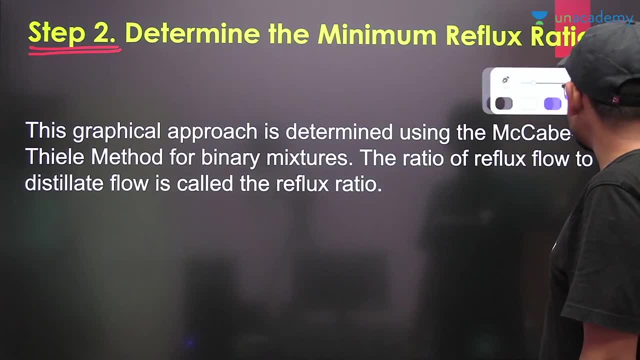 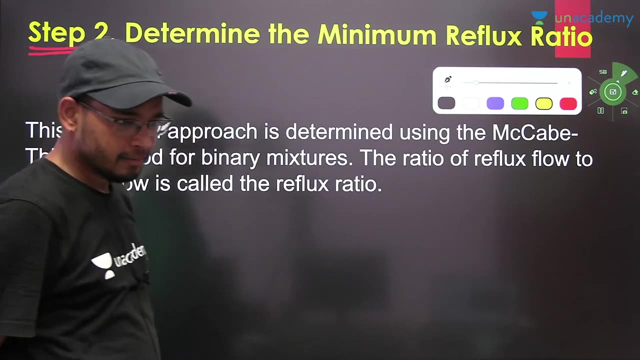 Step 2.. Everyone will write in the copy: Step number 2.. Everyone will write in the copy: Step number 2.. Determination of the minimum reflux ratio. How to calculate the minimum reflux ratio? We will need r minimum. This is also done, but there is not much of lighter in it. 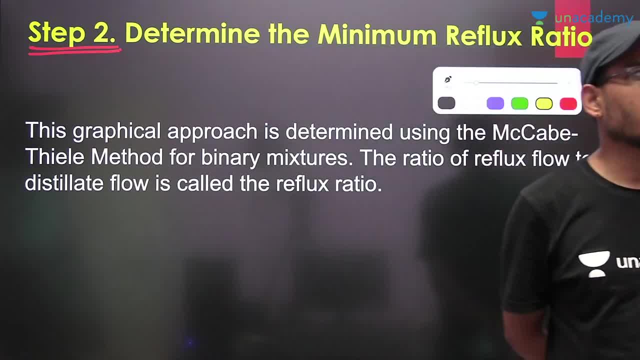 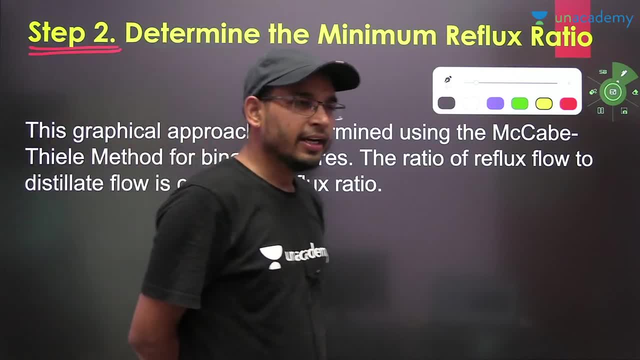 That is also done In it. more of the bottom products are made. Wax is also became more Okay. India also has good But C1 to C5 in it. What do you need? C1 to C5 component: Methane, ethane, butane. 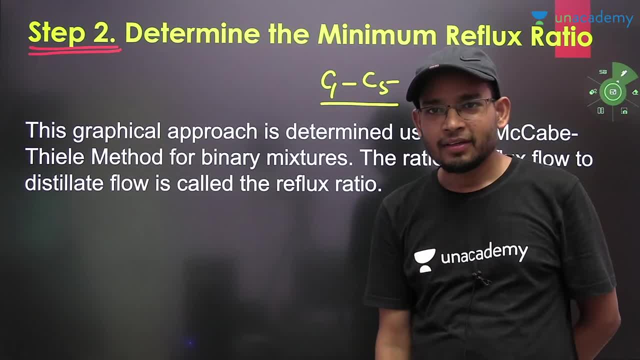 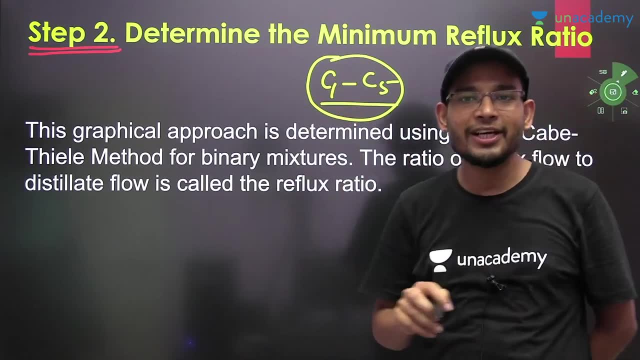 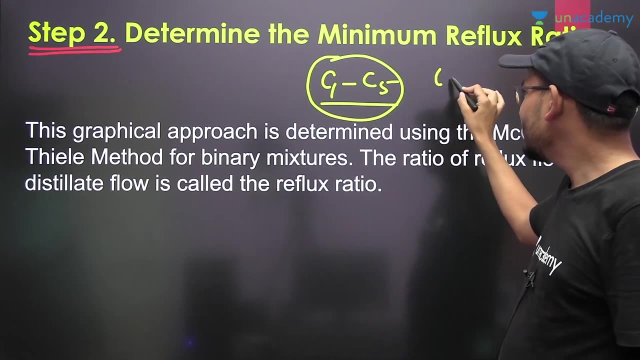 methane, ethane, butane. India's is used more in this gas is used in every house. so you want your crude oil to have C1 to C5 components: methane, ethane, butane components. more it is not more, and in India it is. 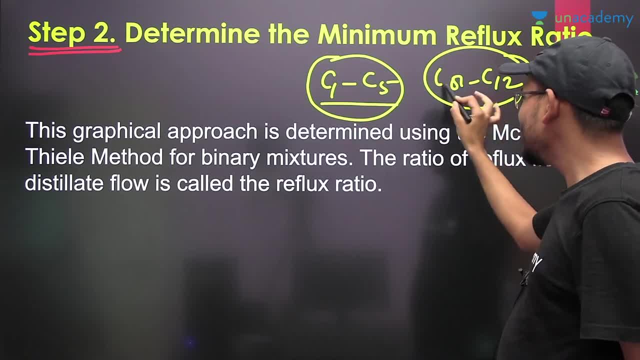 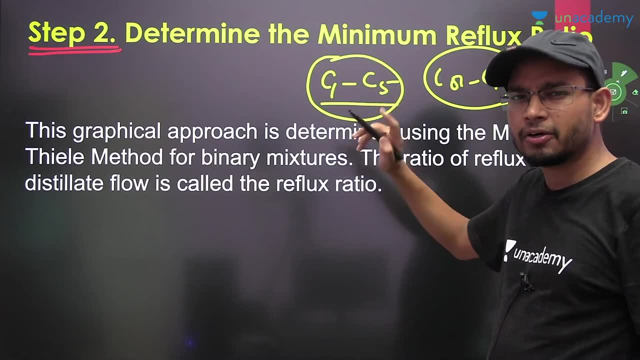 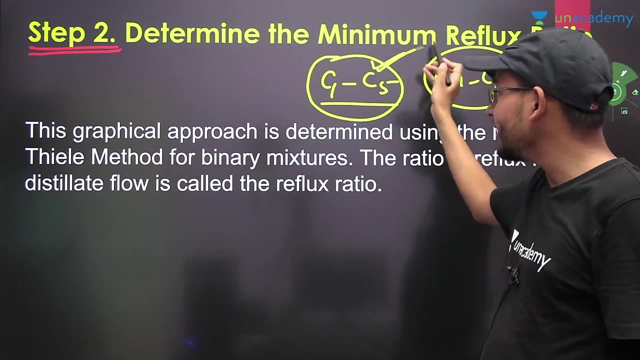 CA2, C12 in crude oil. its quantity is more. quantity is more CA2, C12. after that you can make petrol and diesel. no problem. petrol and diesel will be made, but you have to refine it more. and what do you want? the one which is used more in India. 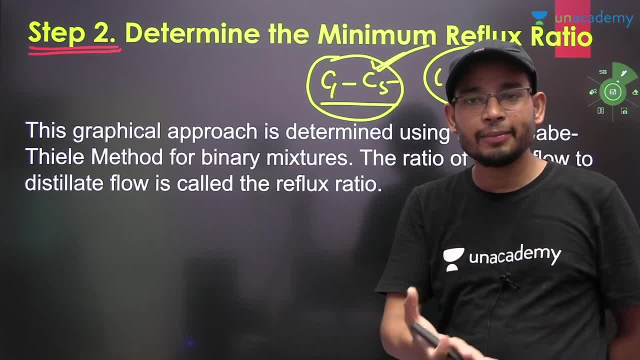 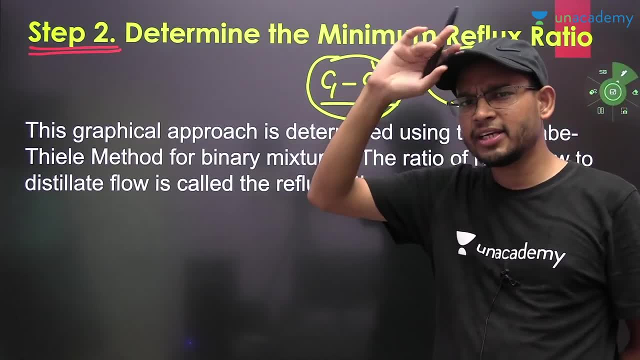 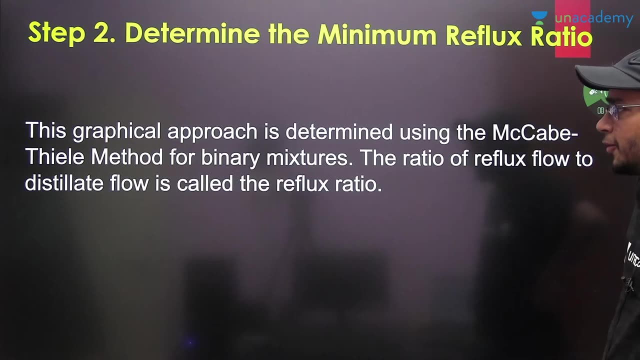 the one which is consumed more: methane, ethane, butane- the one which you eat daily at home. so that should be more. so it comes out somewhere. there are many places in India where it comes out well, but it comes out more from outside. so determination of minimum reflux ratio. 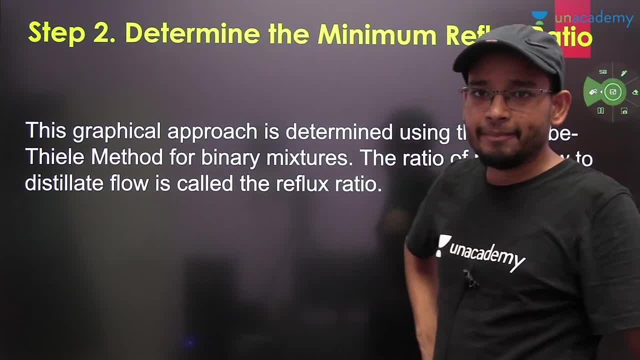 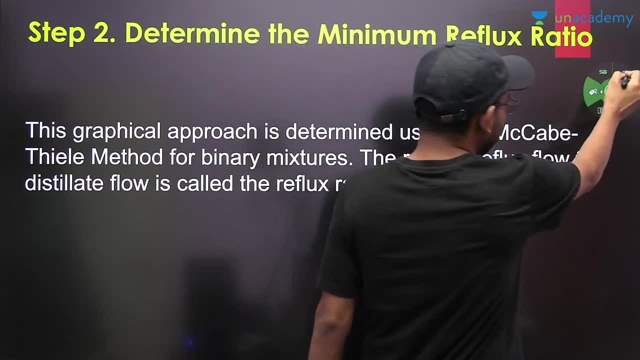 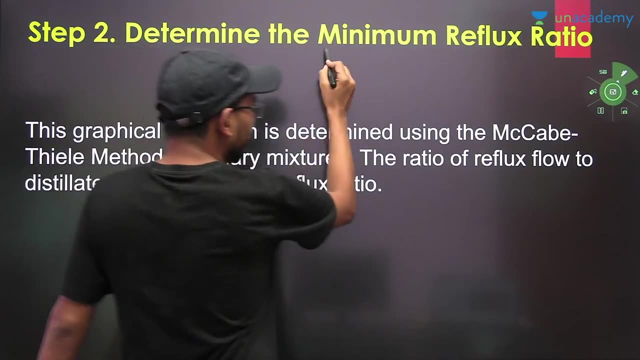 so minimum reflux ratio. there are two ways to calculate it. one is analytical method and other is graphical method. we will talk about graphical method. understand this very carefully. we will talk about graphical method, so we will follow to determination of the R minimum. for R: minimum calculation. for R: minimum calculation. 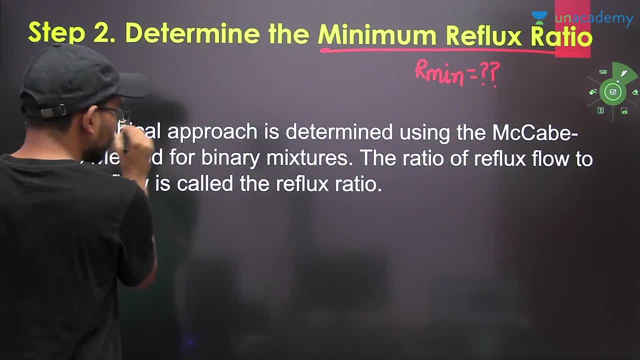 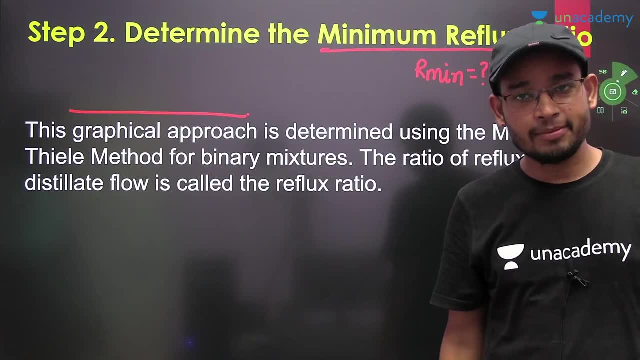 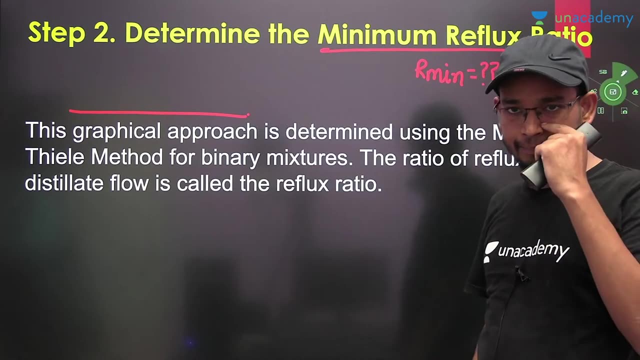 the method we will follow. we will follow graphical approach. now you will ask which graphical approach we will assume, which is R minimum. the method we will follow is Macabre. we will use the Macabre method, which is the Macabre method through Macabre method. 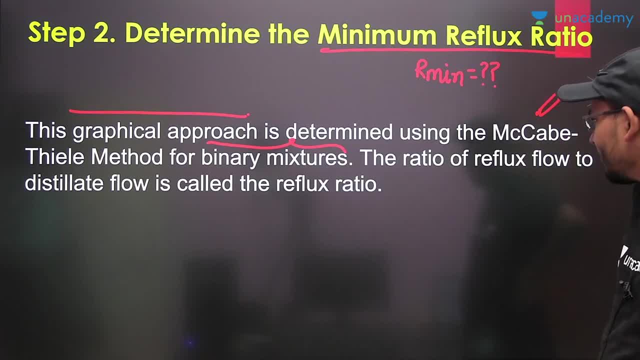 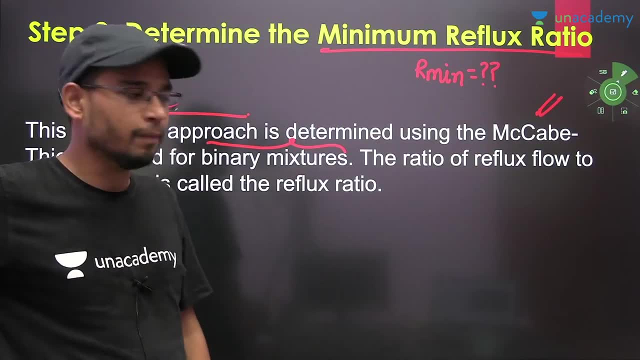 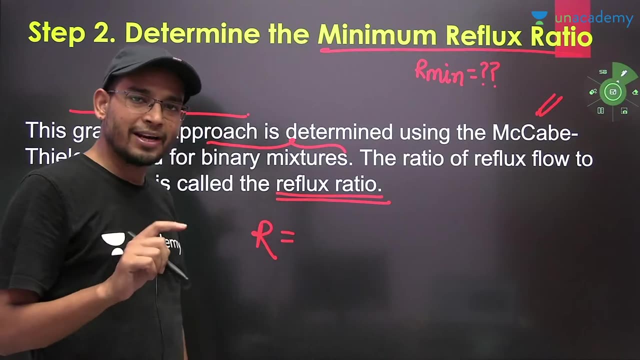 we will talk about whose binary mixture. for binary mixture, we will find the reflux ratio. now the simple thing is, if we are talking about reflux minimum, then first of all tell us what is the reflux ratio. So what happens here is, as you have read it, return upon withdraw. return upon withdraw. 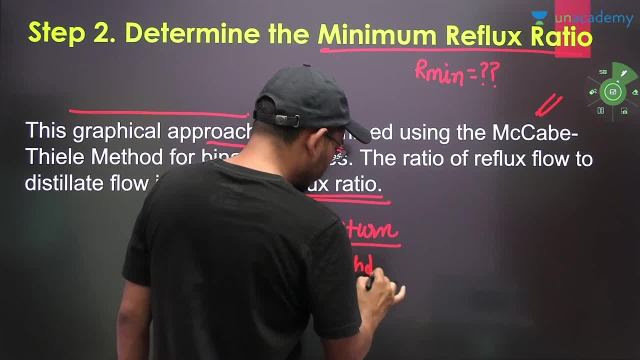 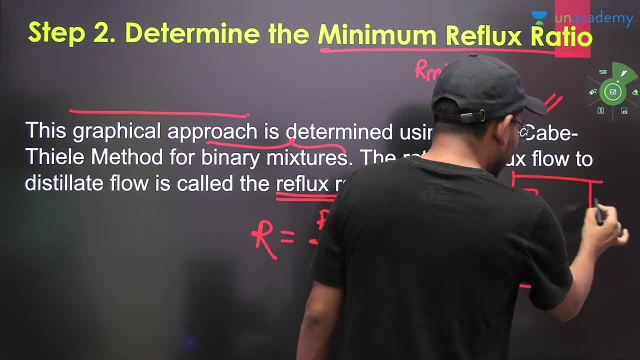 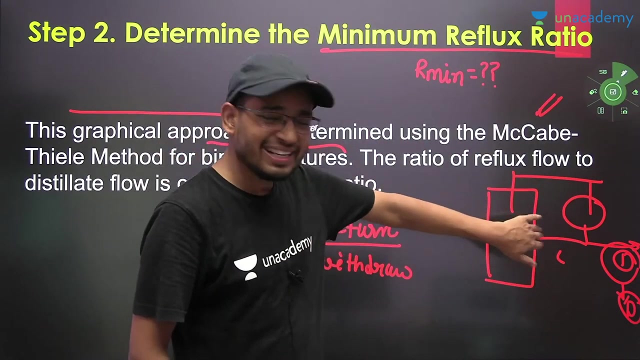 return upon withdraw means this is your column. suppose this is your column. you have a reflex drum here. so how much return are you throwing from the reflex drum and how much you are withdrawing? So how it defines the reflex ratio, The more the reflex ratio it means that you are returning the whole part. 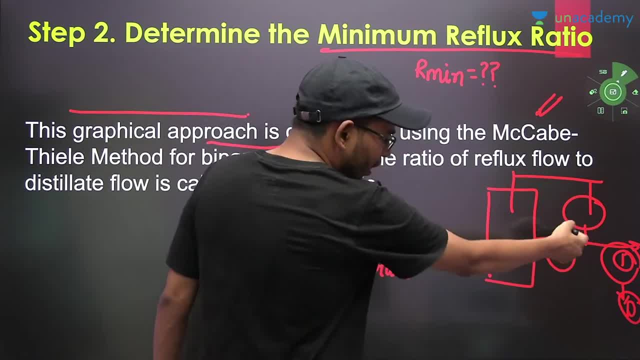 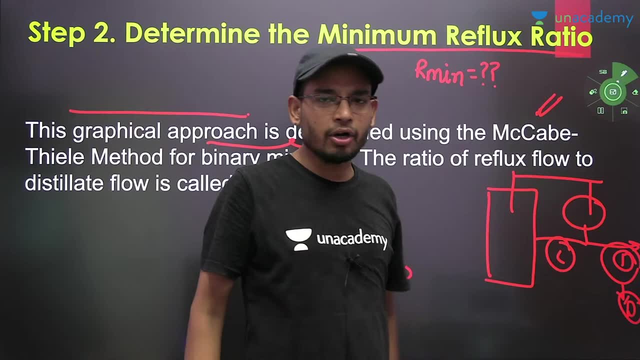 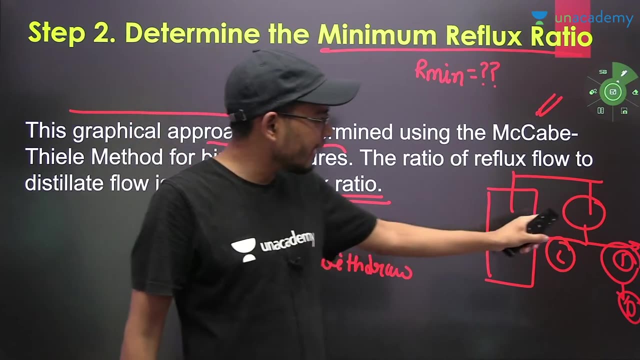 So the maximum part which you are not being able to return and you are not being able to withdraw something. So how much are you returning and withdrawing will define how much the system has of the flat-footed method. So this with which we will do, let's talk about the reflex at first, how much we have. 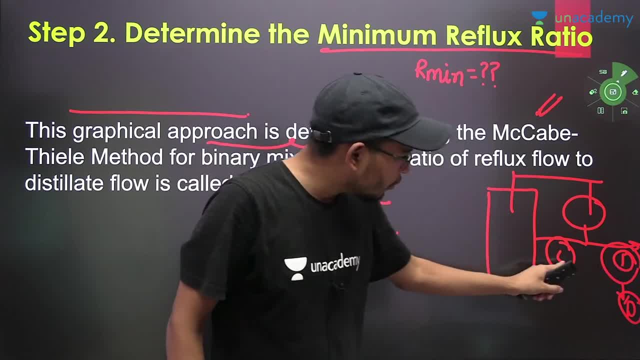 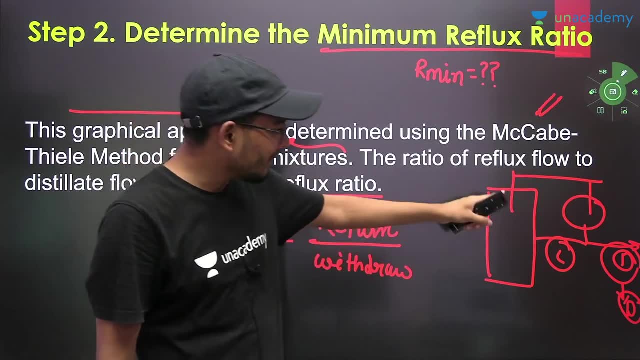 to back off. How much we have to back off. We are going to talk about How much Do we have to back off we are taking out in the outlet. we need to have this knowledge right to define the number of tray. so, according to the number of tray, you will do this work, ok, so we 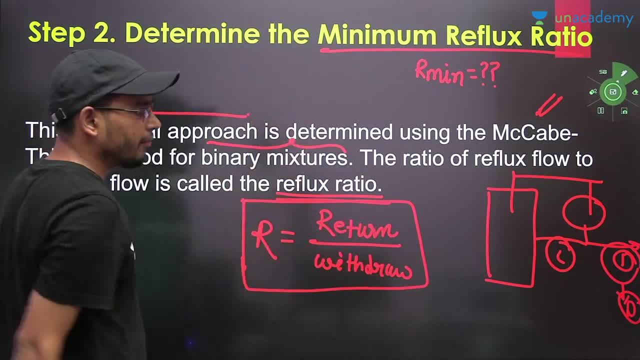 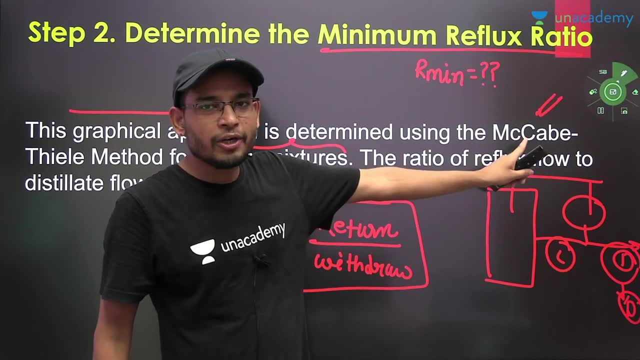 understood this thing. first of all, we have to define the minimum reflux ratio. ok, so now for the minimum reflux ratio. you should know the assumption with the make-up that: what things are you assuming? this is simple. let's ask you in the interview: tell the assumption. 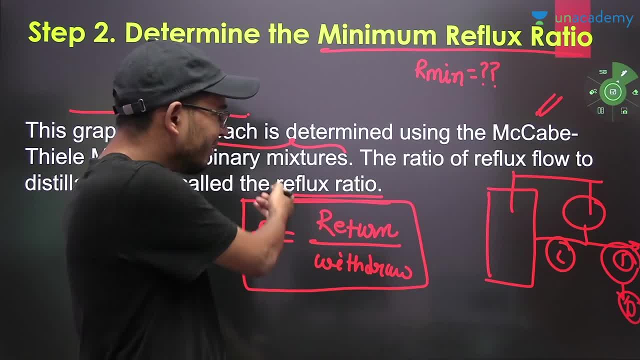 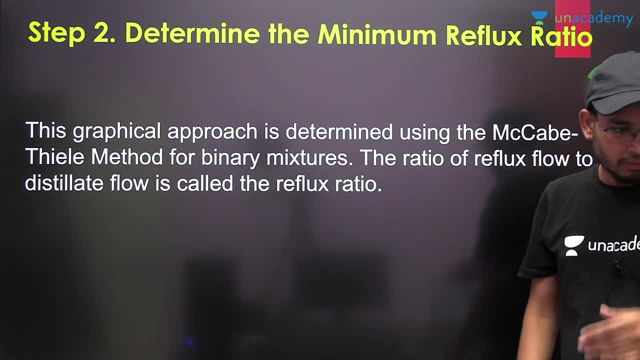 with the make-up. ok, there are 3 to 4 assumptions. first we will write this line this pinch, then I will write its assumption. you have to write that first. write this much. yes, this class will continue every day. yes, you can do cracking in, cracking. yes, your component. 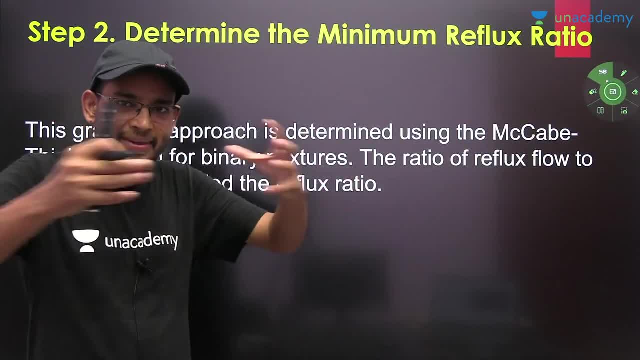 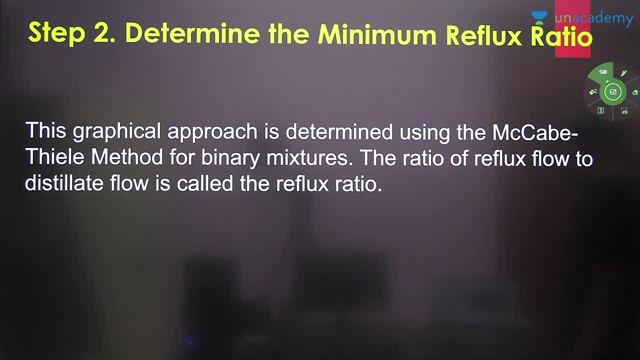 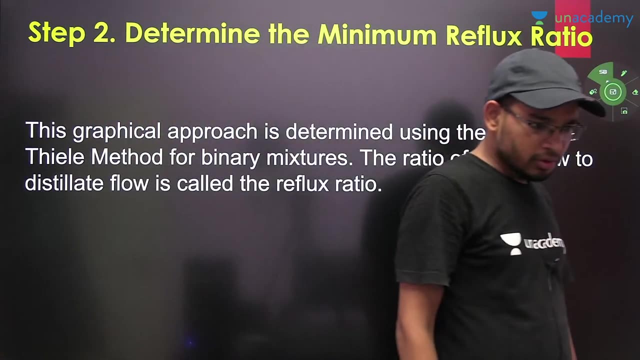 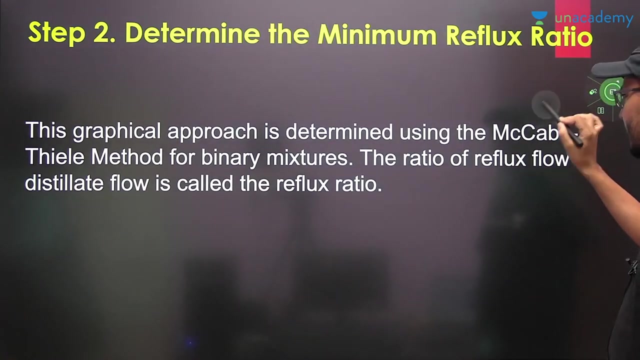 is cracked only after C8,. crack means a long cycle. you have to break that. ok, so you can break it first, write this much. I will talk further. no, no need of pension separate. whatever pension separate is needed, I will tell you. ok, write this much first. now I 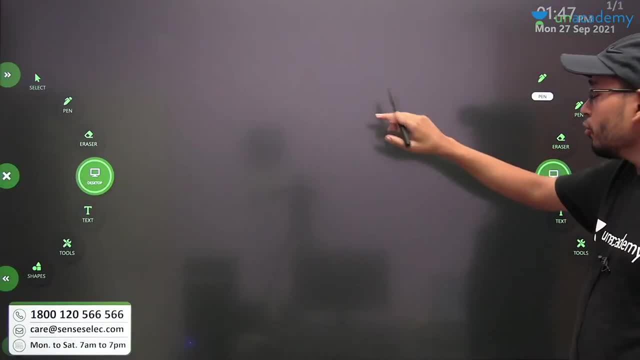 will just talk from here. that simple you have to ask. this is asking in the interview that I said 3 to 4, assumptions: 2%. I have 3% amateurs and 3% amateurs. but I have three thousand amateurs, I have four. 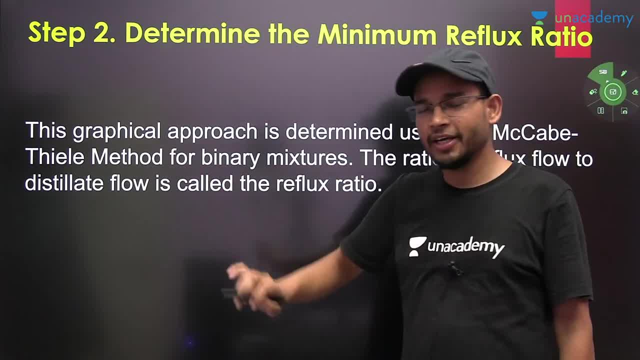 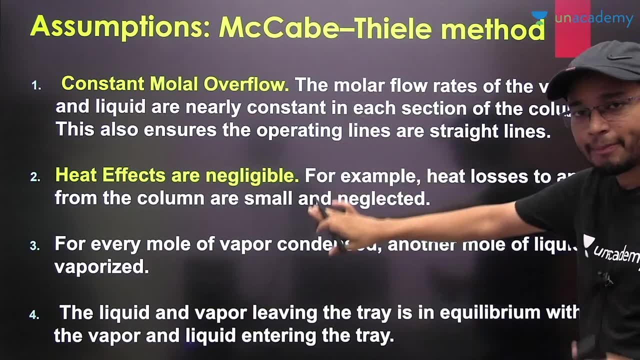 amateurs. I have four thousand amateurs. I have five thousand amateurs. so what am I saying? What is the assumption of Macaphthile? As soon as you use the word Macaphthile, you will immediately ask: what is this? So the first thing about Macaphthile: I have brought it properly mentioned here. 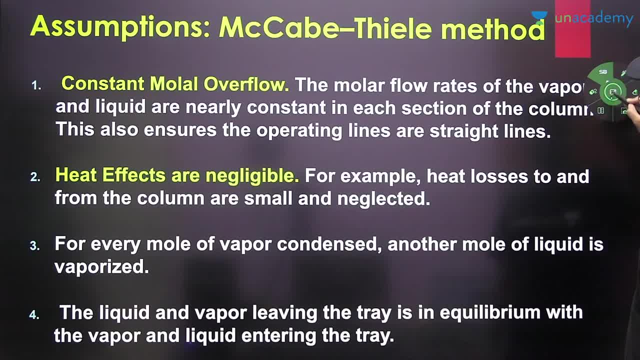 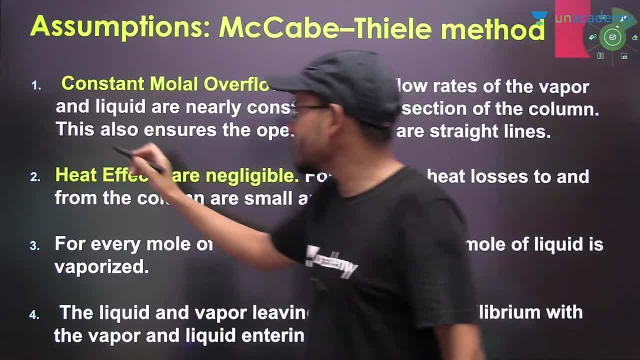 What is the assumption of the Macaphthile? This question has also come in the gate And let's ask you this thing directly orally, So we will write it very well: Macaphthile's assumption, The first assumption. Everyone will write it down. 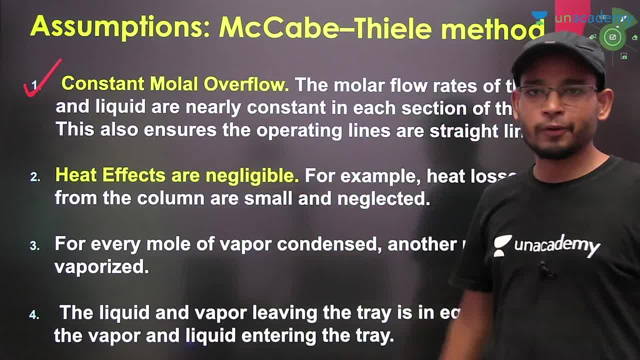 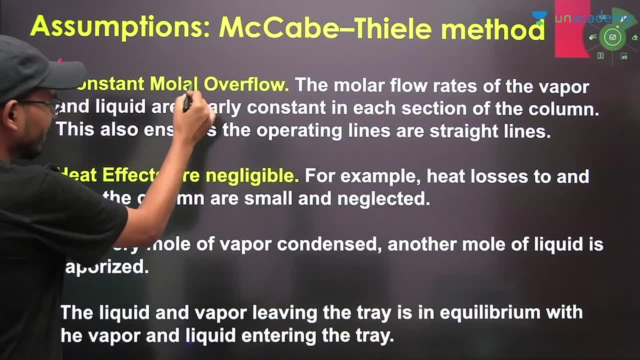 The first assumption of Macaphthile is constant molar overflow rate. Molar means molar flow rate. Write constant molar. Even if you write molar, there is no problem. Write molar- Constant molar overflow. What does this mean? 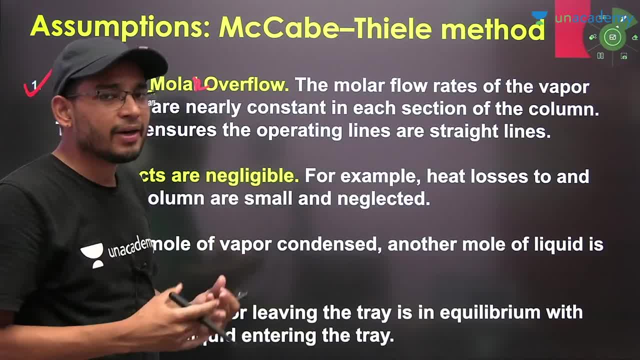 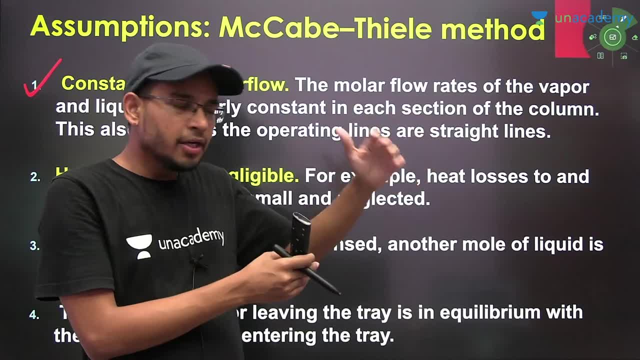 This means that the liquid in the column and the vapor in the column, Their flow rate, is not changing on any plate. Right In case you have a top section. So in the top section the vapor flow rate will be the same everywhere on every plate. 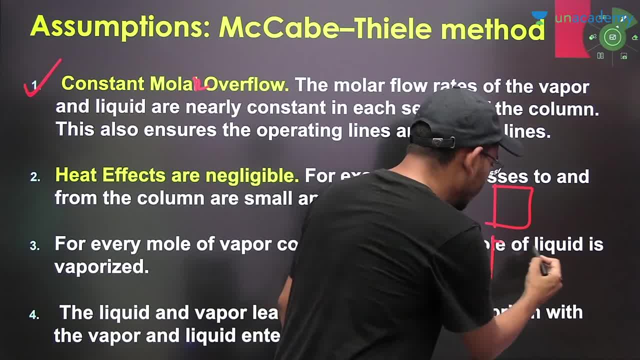 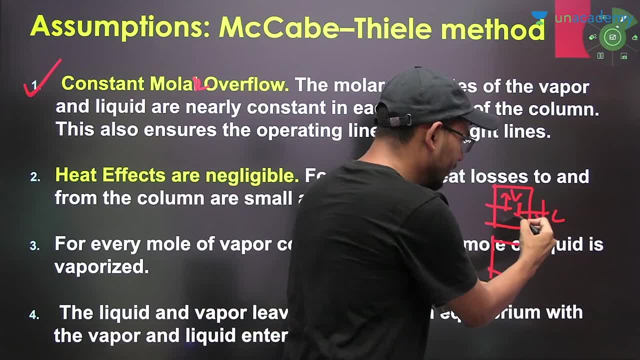 Okay, Look, Just understand. Suppose this is the top section and this is the bottom section. So what will be going on in the top section? Vapor will be going And liquid will also be coming from the bottom section. Okay, What will be coming from here? 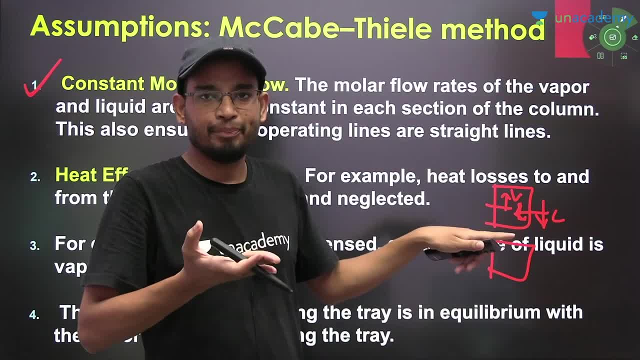 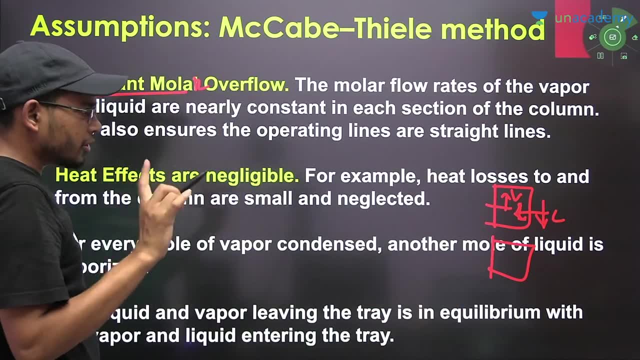 Liquid will be coming Right Now. what will happen? on every plate? It will be the same. Okay. Whose assumption is this? Macaphthile's Okay. So Macaphthile's assumption is that the constant molar flow rate will remain. 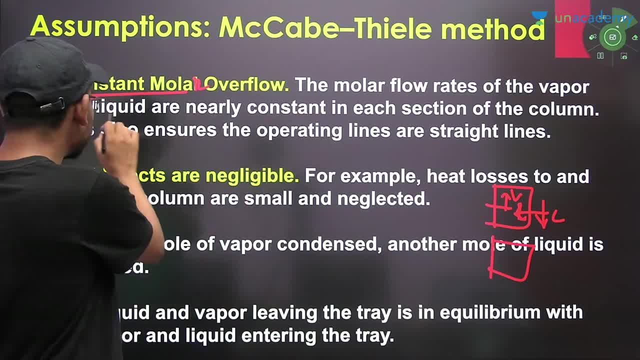 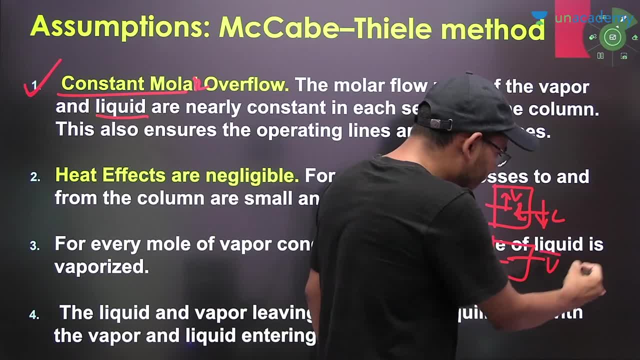 It will not change. Vapor and What is yours? Vapor and liquid, Both In each section. Okay, Now, each Each section means This section will be Here. you have B-bar and L-bar. You must have read some theory. 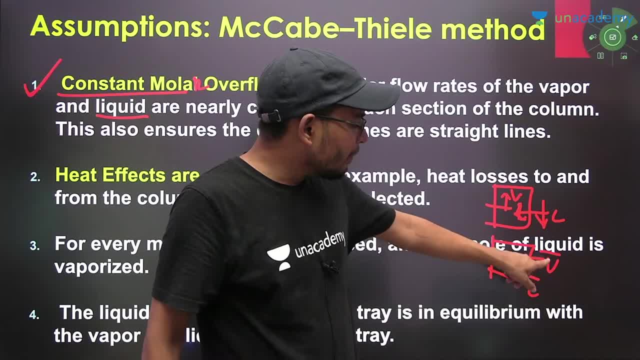 I had taught you L-bar and B-bar, So B-bar will be in the stripping section. You will not change on any plate. This is the first assumption. L-bar will not change on any plate. Stripping section: Yes, L-bar can be different from L. 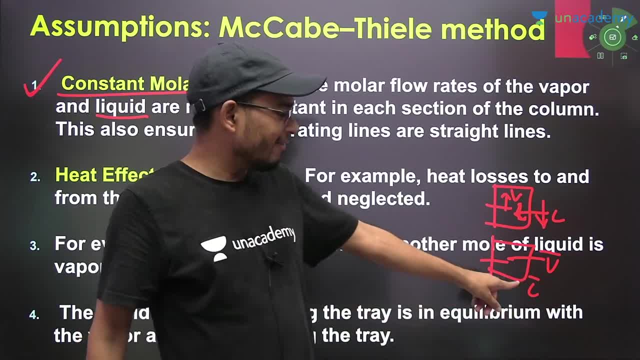 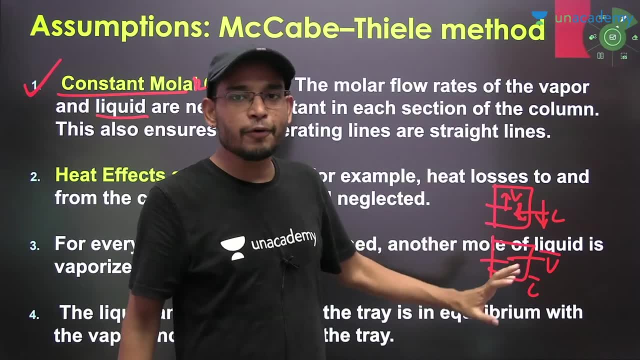 Means What he is saying. What he is saying That these two sections, The flow rate, will not change. in this B-bar The whole column Means In the stripping section B-bar will not change. Okay, So So. 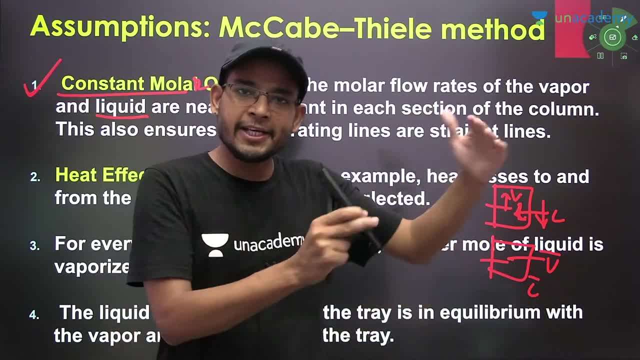 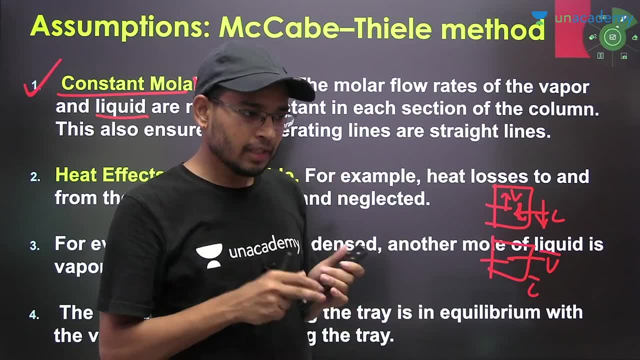 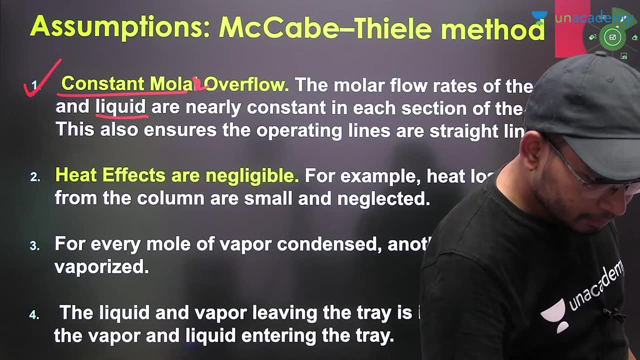 So So B-bar will not change. Enriching section Means Top section. In the top section, B won't change. Are you getting this point? Are you getting this point? Yes, Everyone is understanding the point that I am giving. 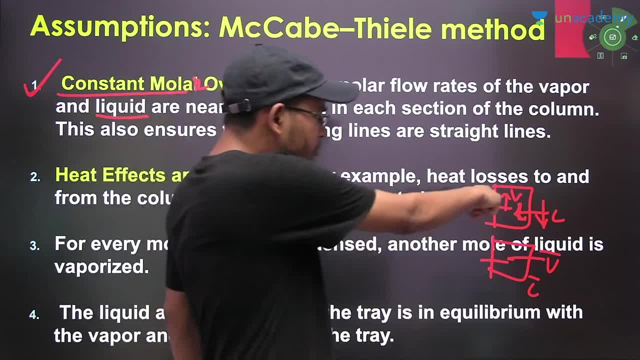 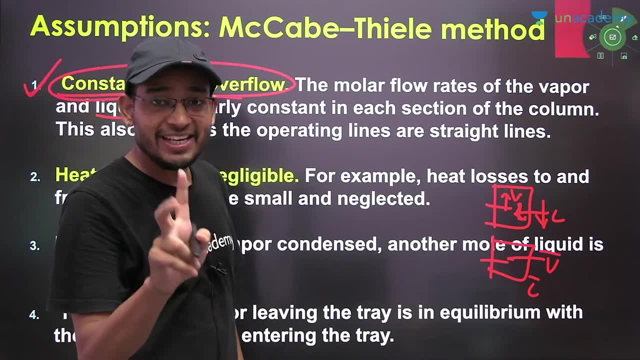 What things will not will be change And what things will be. the change So Means The main assumption means The flow rates. They will not change in column, Each column. Each column means enriching section or stripping section. Okay, 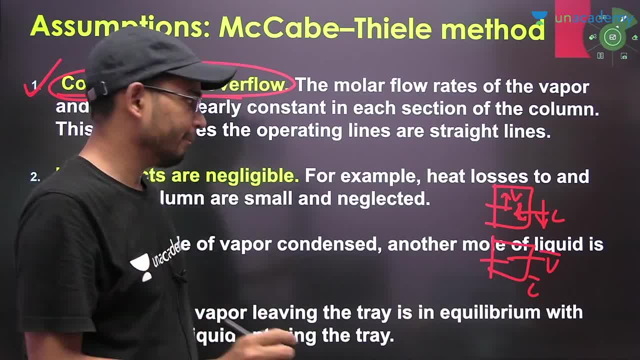 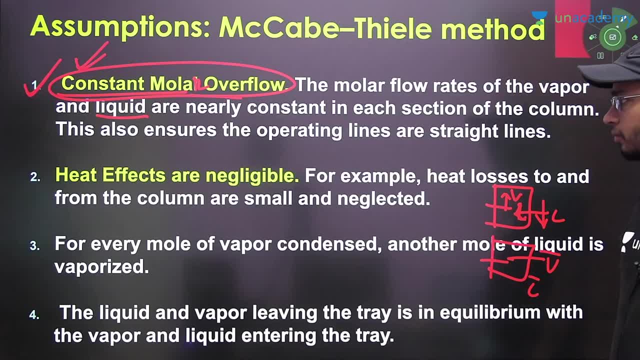 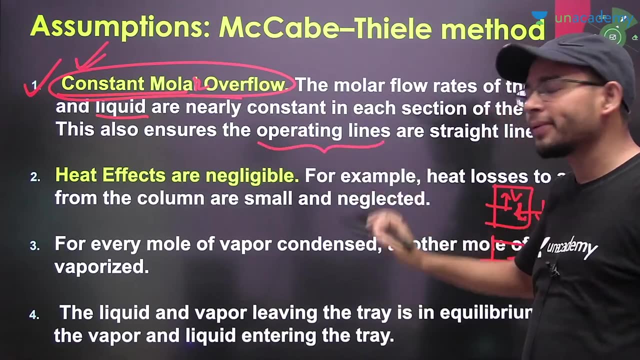 So this flow rate will not change. This is the first assumption of the Mac app. Okay, This is the first assumption of it. Right, And operating lines. Operating lines which are of your top section and bottom section. They will make the form of y is equal to mx plus c. 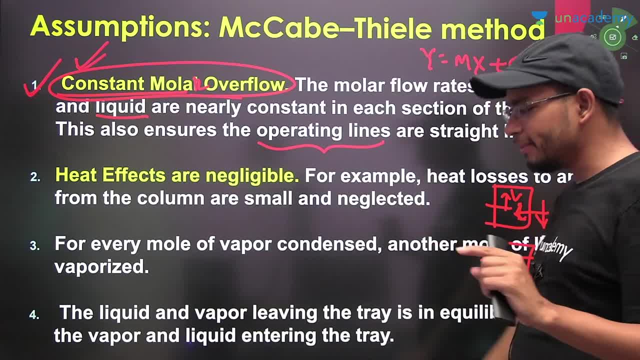 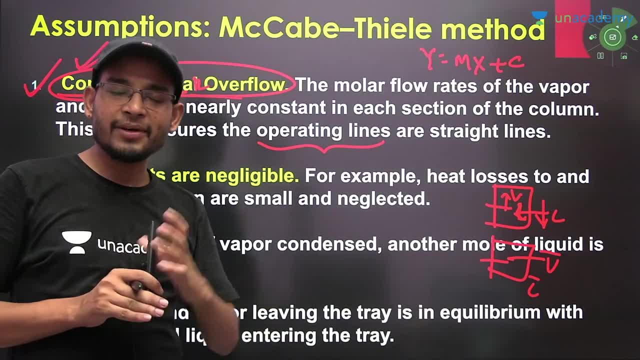 y is equal to mx plus c. You had seen this When you had drawn the equations of operating lines. So how were they? They were linear. You had seen Whether the operating line is of stripping section, Whether it is of enriching section. 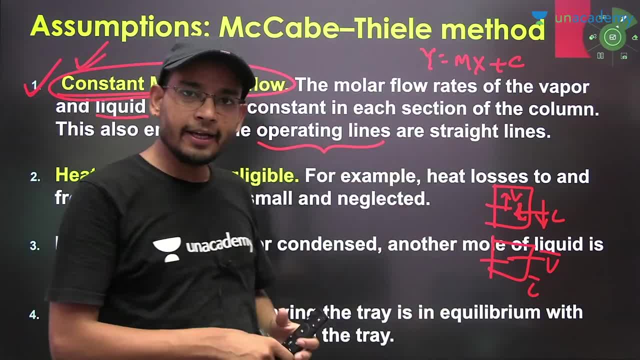 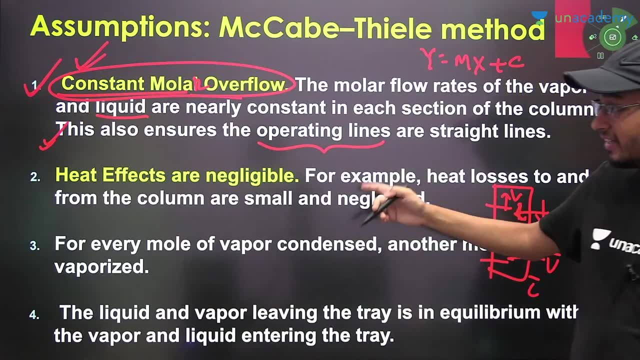 Whether it is of feed line. How were they? They were straight lines. Okay, So this assumption will be written down by all. I will explain the second assumption. They ask this very well, Very, very much, Very important. This is very important for the interview. 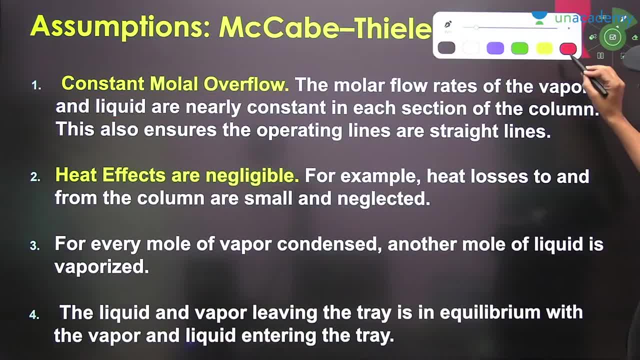 I am telling you, If you will go for interview of work, Then they will definitely ask for Mac app- Okay. As soon as it comes in distillation They ask for assumption of Mac app- Okay. This is important for any interview. 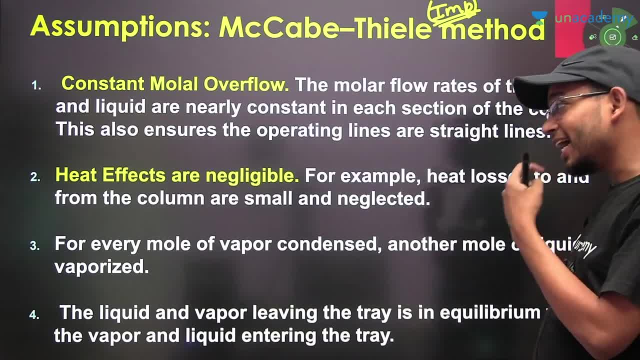 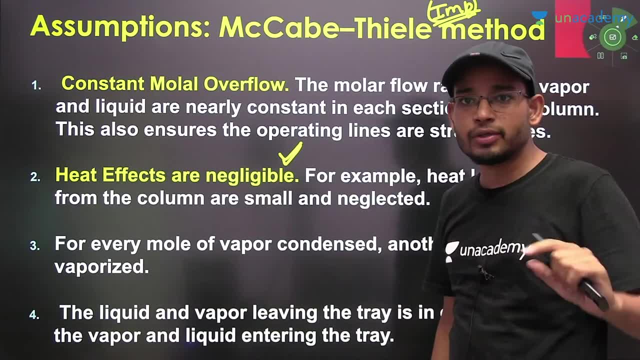 And there is nothing written in gate. also, Now, heat effects are negligible. Okay, What does it mean? The more heat loss will be, The more heat you will gain. How will be the loss? When you See, when will the heat gain be? 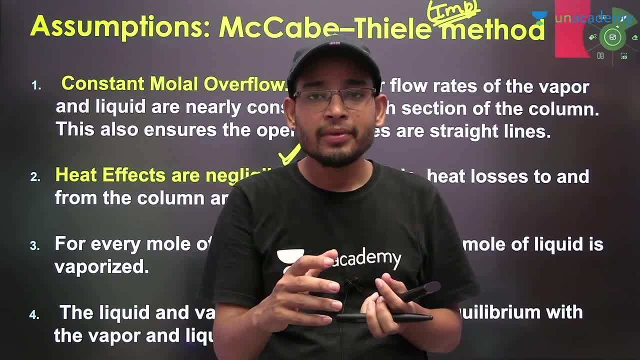 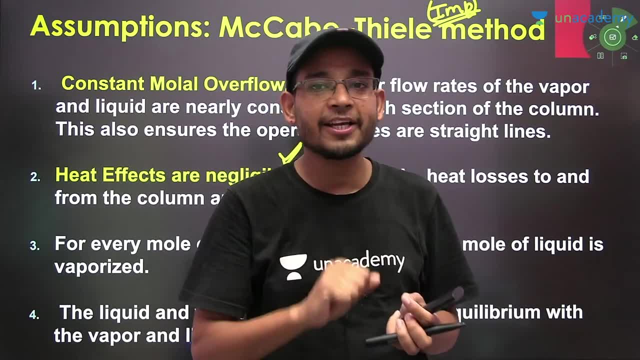 After what it will be. When will you gain? You will gain in the liquid And who is doing the loss? Your, Yes. When your liquid is vapour, Then it will be getting heat. You will supply heat to vaporize the liquid. 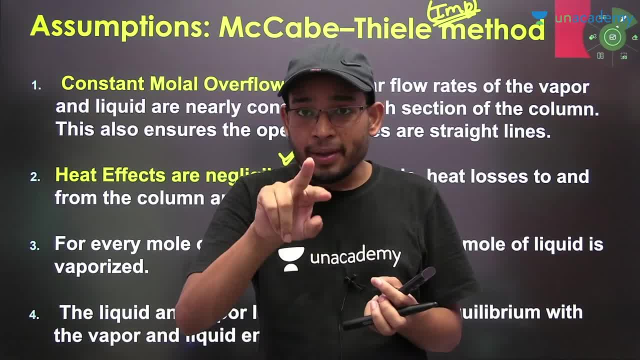 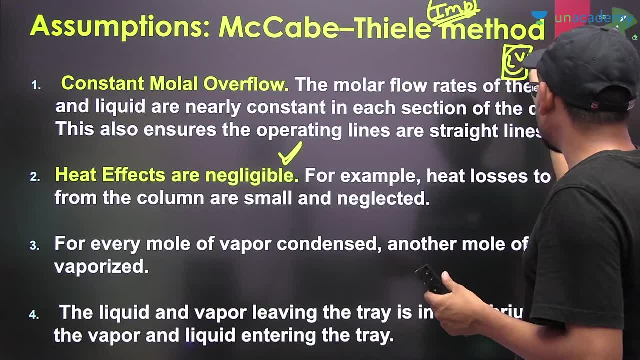 Now when your vapour will condense. So if vapor condenses, then the heat will release. Do you understand? I mean what will be happening? You want that liquid and vapour All time be in distillation column. Then what will happen to the liquid? 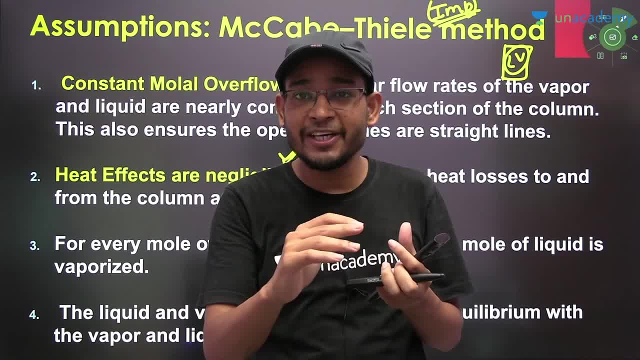 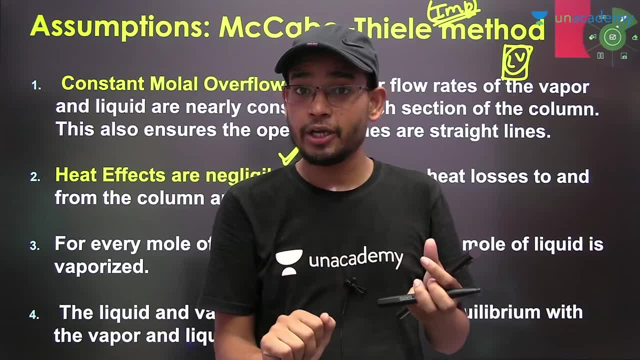 Vaporizing will happen. Vaporizing will happen The liquid. If you vaporize the liquid, then you will give the heat to the vapor. Now the vapor coming from above will also be condensed. Now it will be condensed, which means the heat will also release. 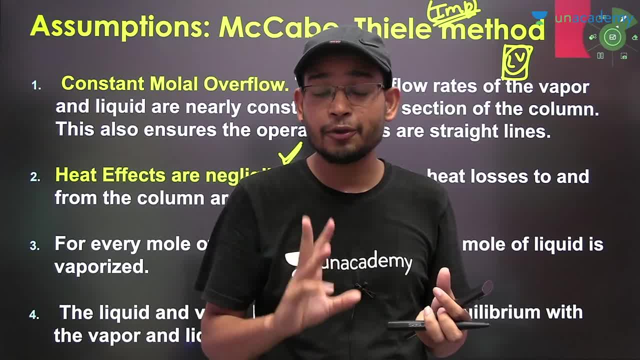 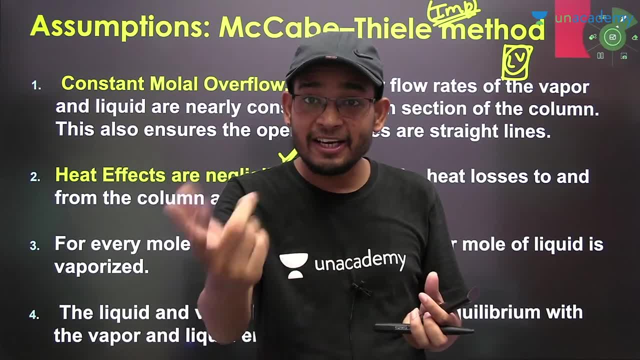 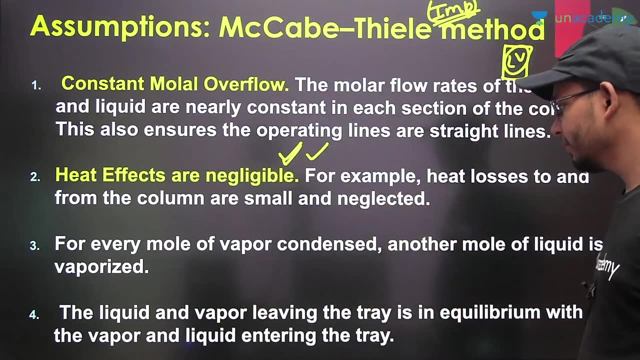 So vaporization and condensation will run parallel. So the more the heat vaporizes, the more the heat will release when one mole of vapor will be converted into liquid. So heat effects are negligible. Yes, this is what is written in the third point. 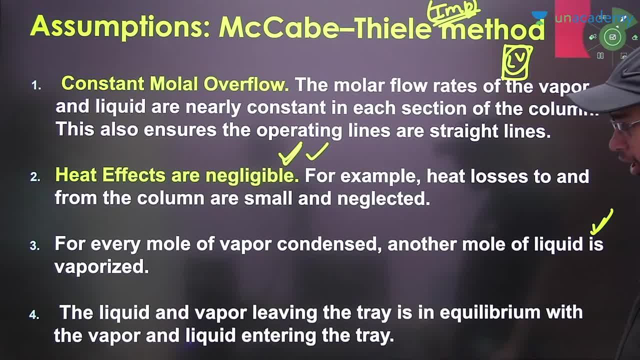 Tick Yes and understand the fourth point. everyone Understand the fourth point, which means the tray. What will be going from here? Vapor will be going And your liquid will be coming from here. So the vapor that is going in the tray, the mole fraction of your light component, will be there. 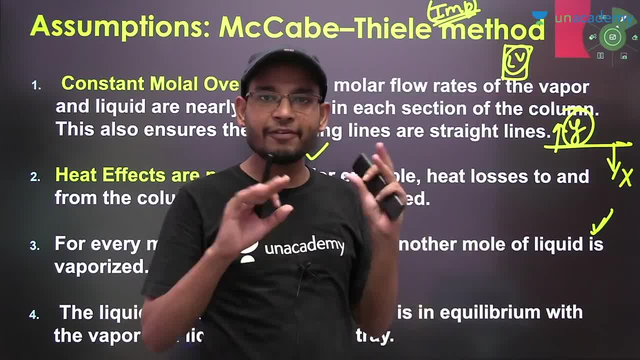 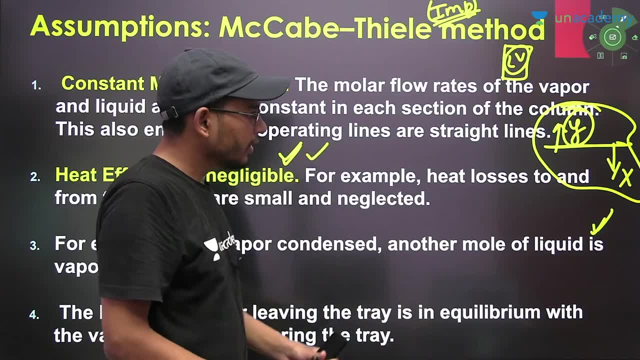 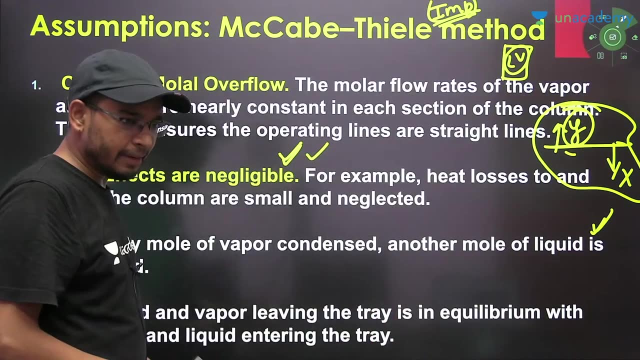 And the mole volatile component that is leaving on the particular tray. Both of these Vapor will be in equilibrium. This is the last assumption of the Macabre theory. Vapor and liquid will be in equilibrium on every tray. Tick. Vapor will be in equilibrium on every tray. 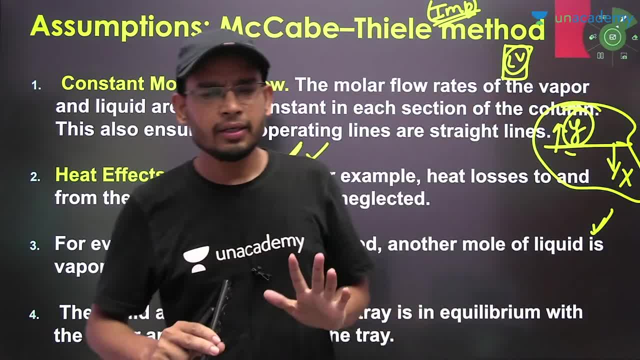 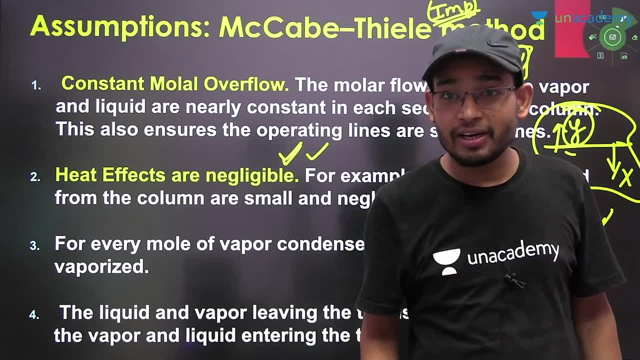 Read it. read it. What is private? Read it properly. It will not be private, Don't worry, But read it. Don't think about all this. Think about what is going on right now. You know, sitting in this circle, it will become private. 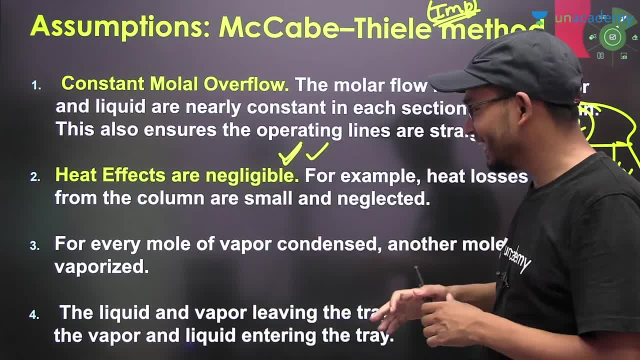 It will become private. The things that are going on right now. you will not understand this. That heat effect are negligible. It will not have any meaning. Then you will understand. Okay, You don't have to think about all this now. 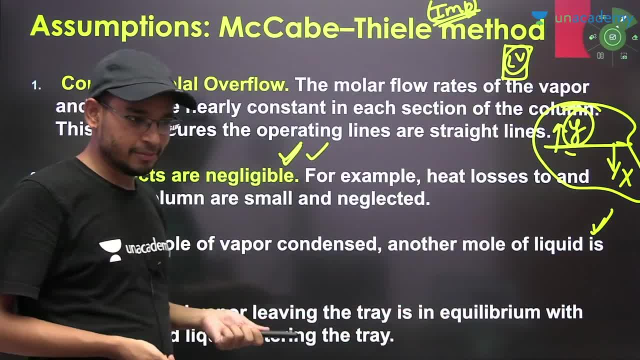 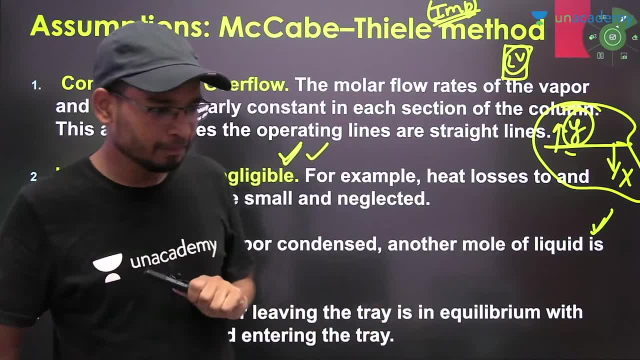 Yes, There is an equimolar diffusion in this. I had taught you about diffusion. Okay, So you don't have to think about this theory. Follow the current process, nicely, No one will get it done privately, Okay, Don't worry. 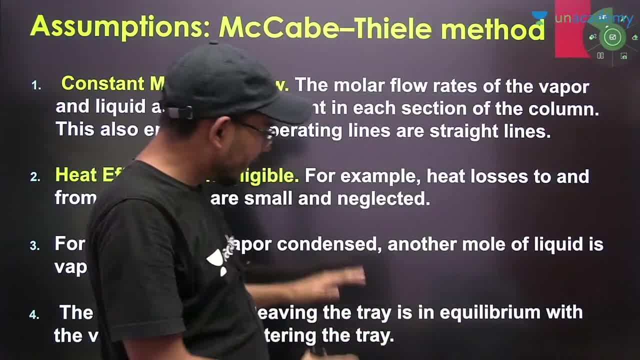 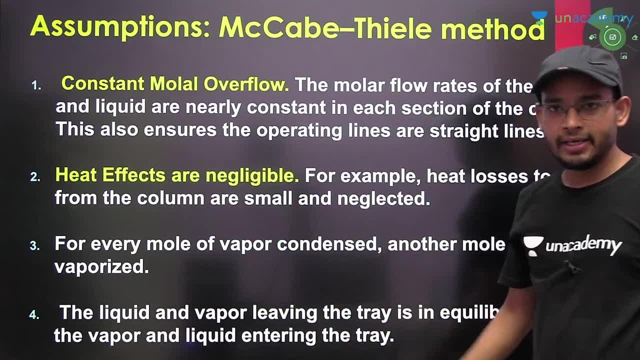 Come on, Write it down All of you properly- Its assumptions- In such a good way. You will not get it in a hurry. You will note it down from here. I have written it down at one place and given it to you. 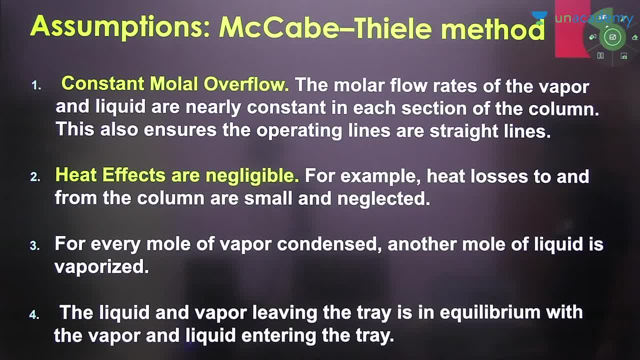 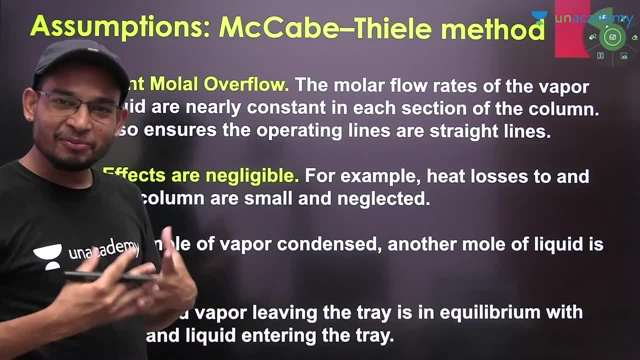 No, no, no, no. This is not the meaning of the equilibrium. I am telling you right now, MR 100.. You are Okay, You are. So it is very important for you to tell. See, I am telling you right now. 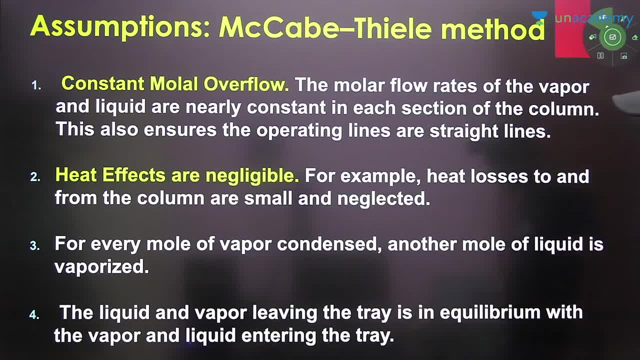 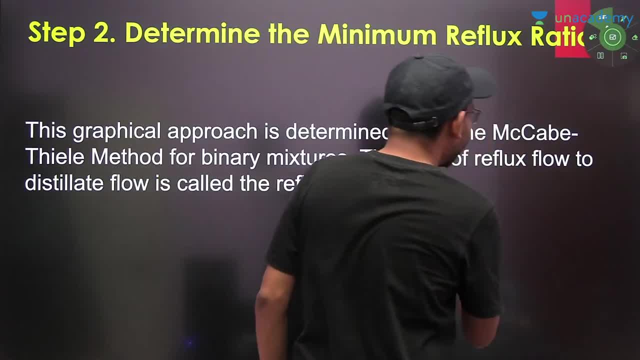 I am telling you MR 100 right now. Don't worry, See, the equilibrium is coming. See, what does the meaning of equilibrium mean? Not composition is same Equilibrium. Equilibrium never means that the composition is same. Temperature previous. 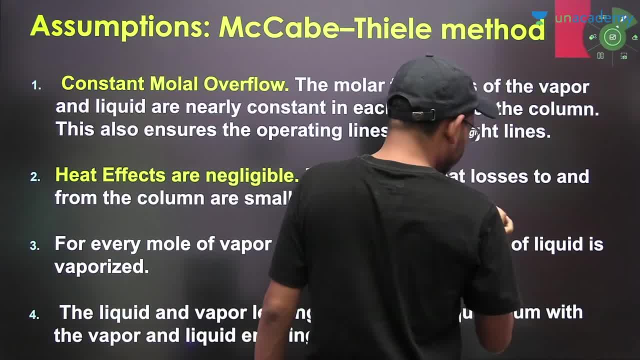 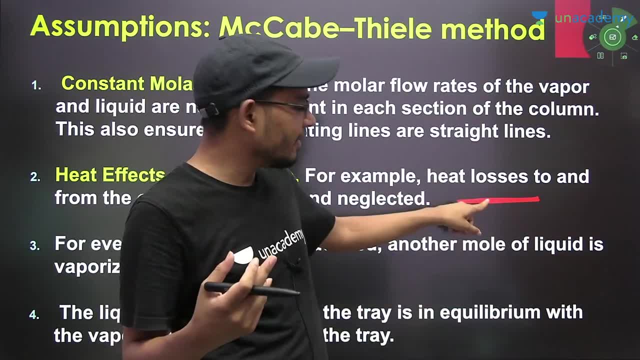 See what the meaning of equilibrium means. Suppose this is a tray. It is a tray, Okay, The equilibrium that will exist, That is the separation of vapor plus liquid, It will be on this tray, Okay. Vapor plus liquid, That is the vapor going from here, will be X. 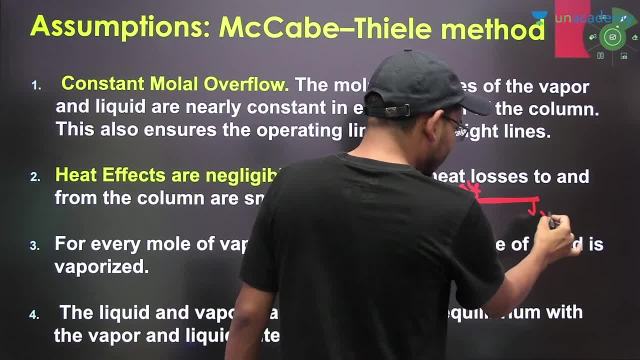 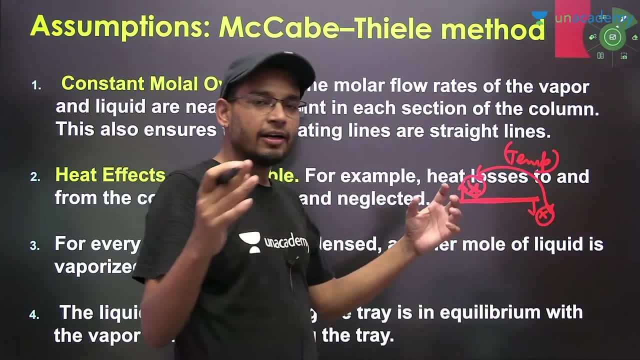 And the one going from here will be Y And X. Its temperature will be. Its temperature will be. What will be the both of them? It will be the same. What is the meaning of equilibrium? Temperature of the system or the temperature of the surrounding will be same. 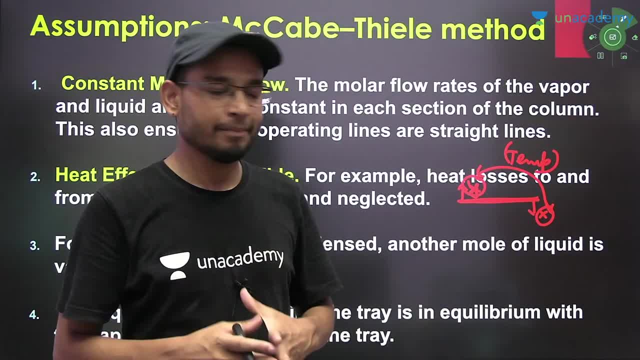 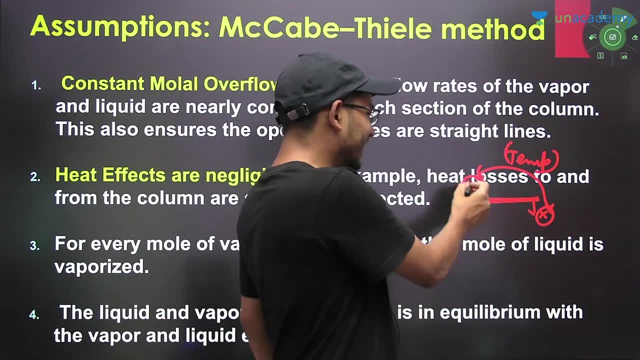 What does it mean? How will the system be? Equilibrium, Gifts free energy is the same. What will be the Gifts free energy of this system? It will be same Right, So always keep this thing in mind. So what will happen? 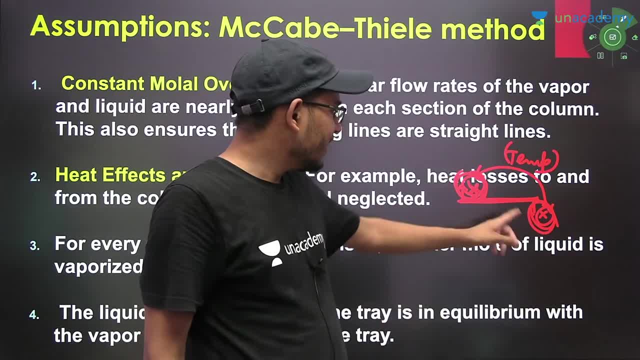 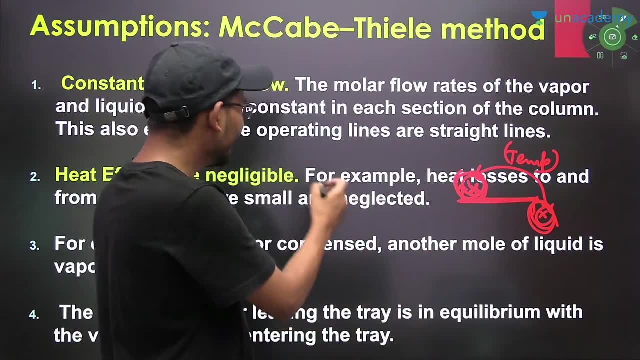 Your Y and X is different. Right, This is liquid, This is gas. The composition will not be same. Okay, The composition will be same. So, dude, then there must be separation here. what is happening on the plate? there must be separation. 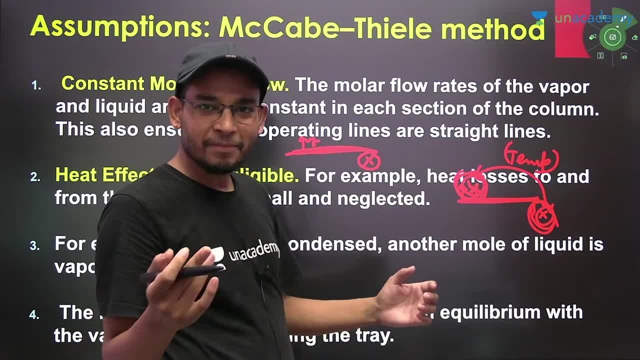 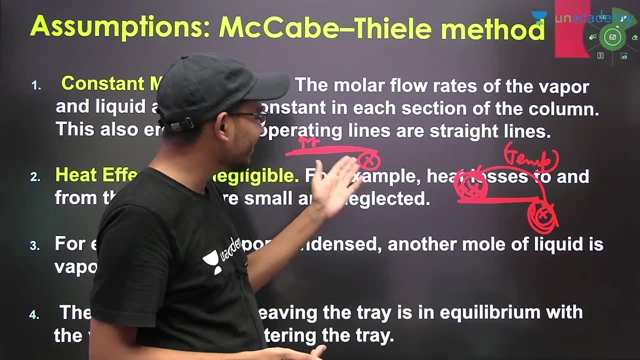 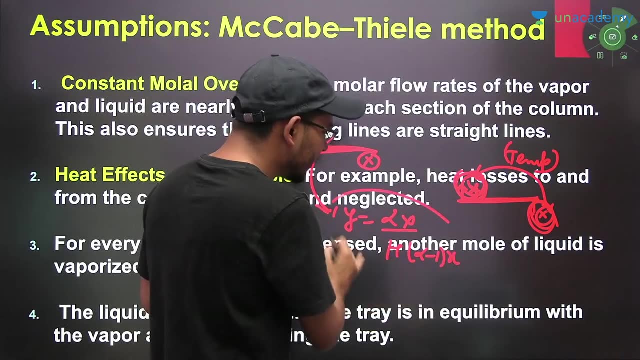 there is y and x. this means there must be separation. this is a tray in case the composition will be same, then there will be no separation. for separation there is equilibrium. this means, whatever data will come, y is equal to alpha x upon 1 plus alpha minus 1 x. 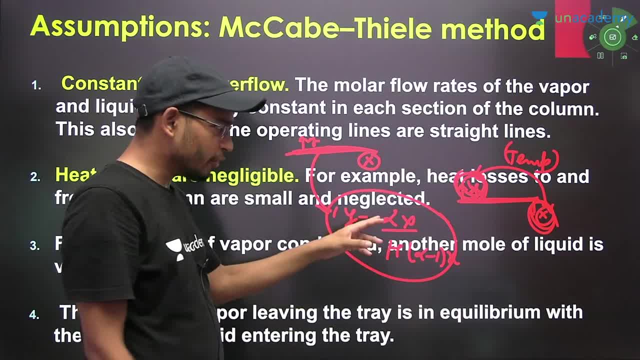 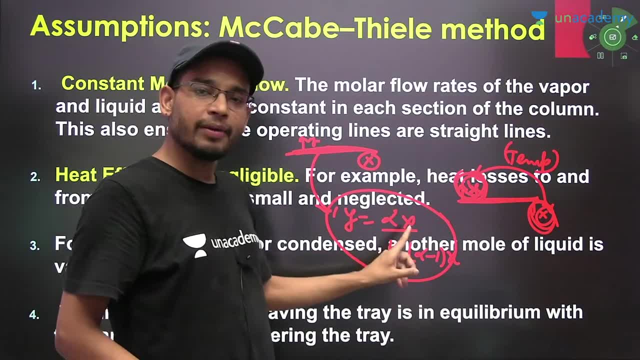 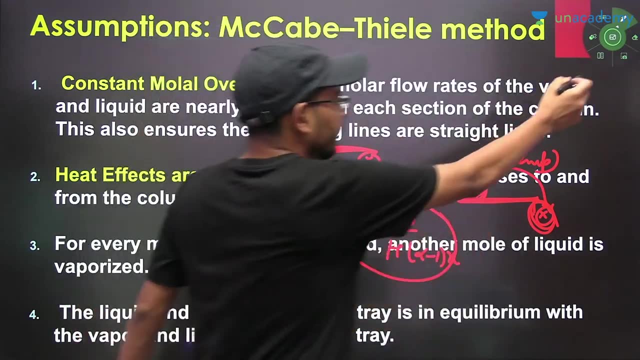 from here you will get equilibrium? from where? from here you will get yx. this is not from operating line. you will not get it from operating line equation. you will get it from equilibrium relation. you will get it from experimental data. ok, never think that they will be equal. 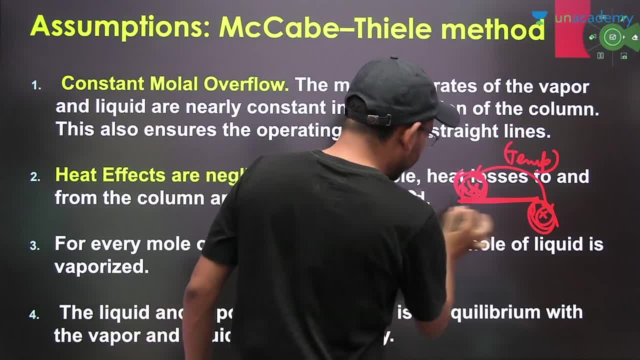 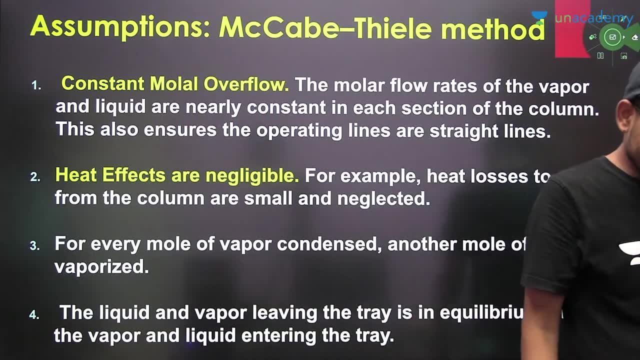 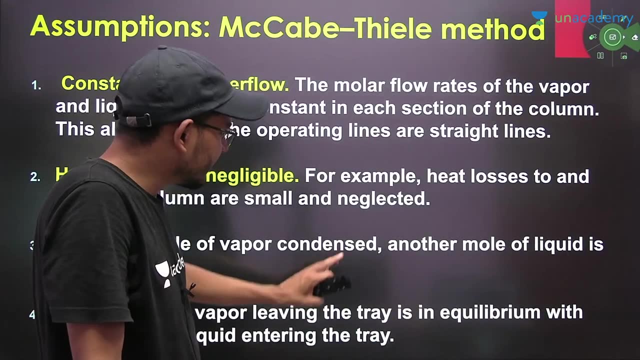 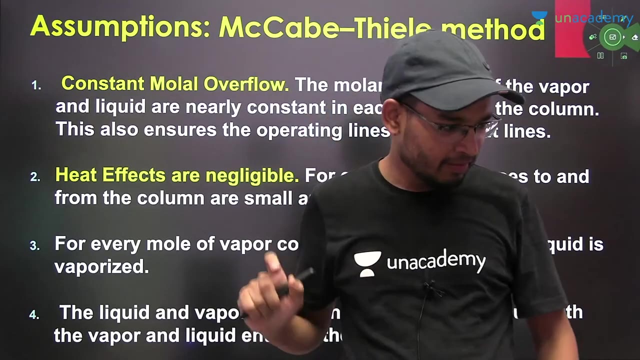 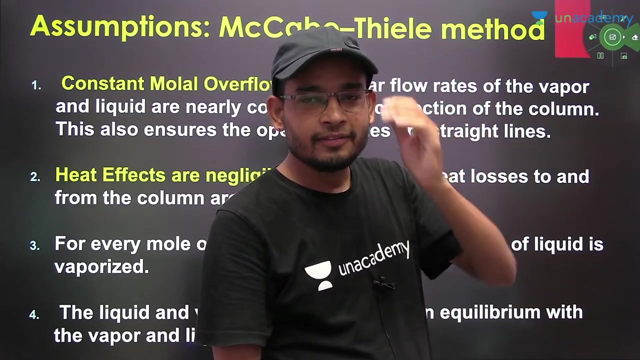 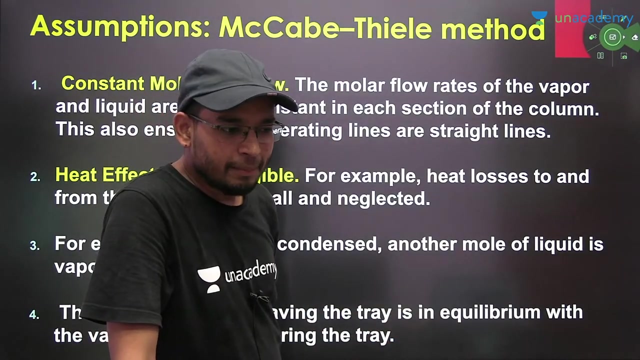 I am rearranging it. you have noted it done, ok, I hope you finished. ok, done, then I will talk. what is your objective? people tell me what is your objective first. you tell me will process or not. now people comment: what is your objective in film? what is the purpose of? 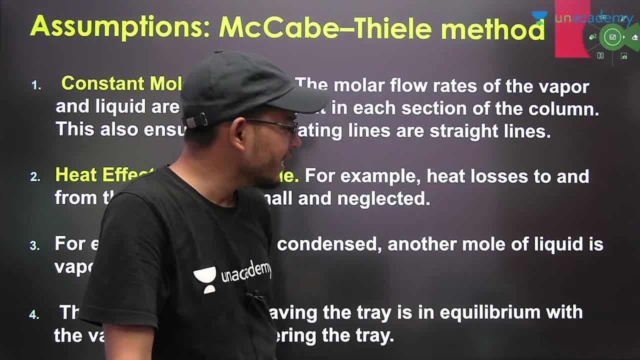 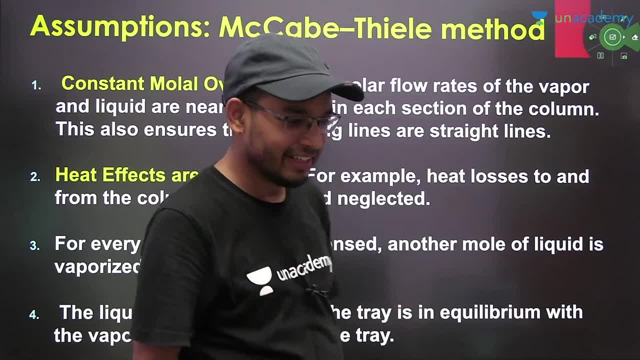 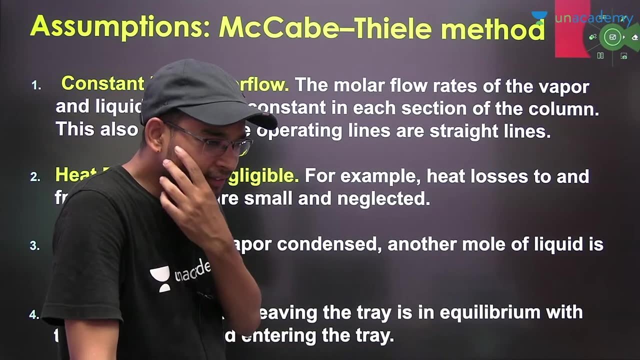 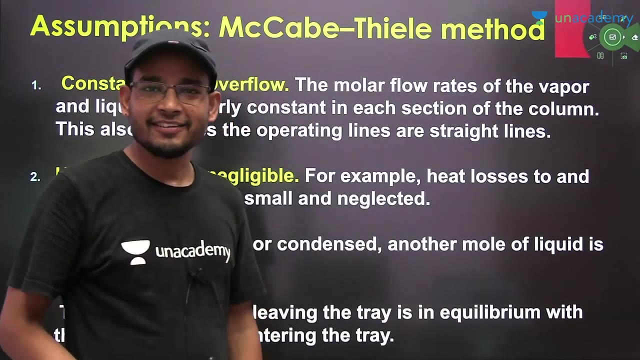 the process for what we are doing. all this separation is fine. now what is the objective for a particular thing? minimum reflux ratio. very good, siddharth. the story of minimum reflux ratio is going on. to find the minimum reflux ratio, you have to go to the graphical method. 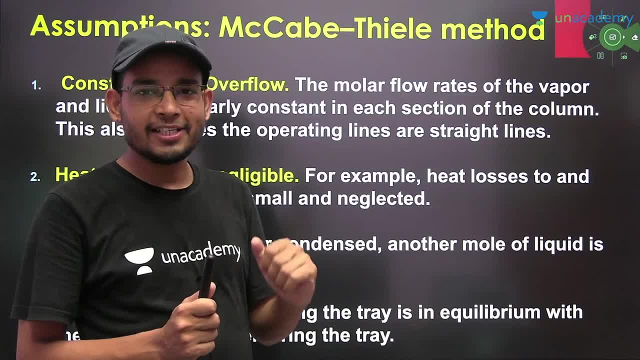 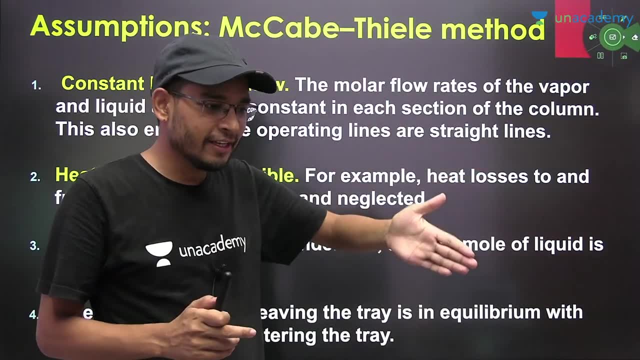 when will you make the graph? when you will take many McCabe's assumption, then only you will make the graph. so now, whose calculation is going on minimum reflux ratio's. so be careful about that. whatever you are talking about is going on with minimum reflux ratio. 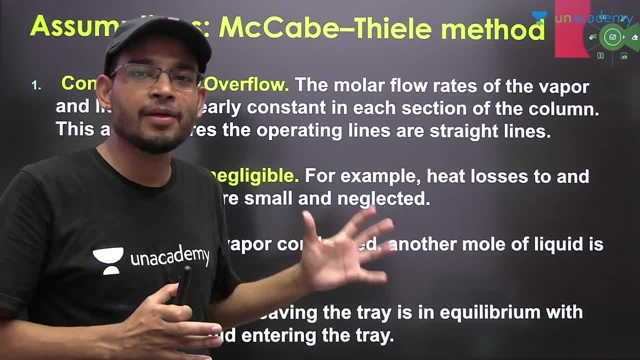 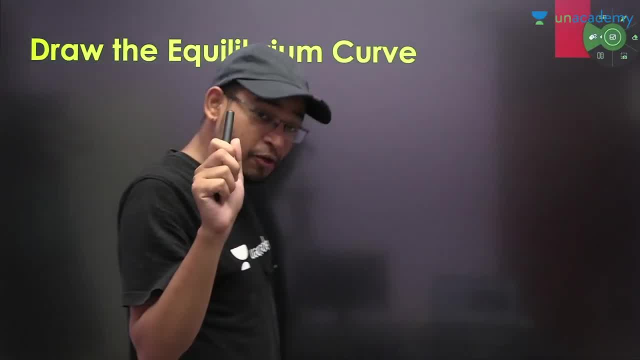 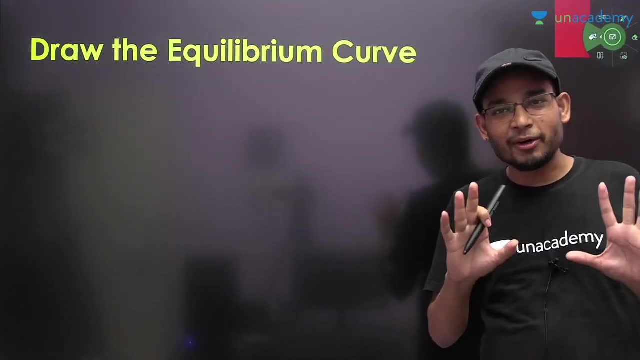 right, your work is going on with minimum reflux ratio. to calculation of the minimum reflux ratio. fine, yes, now come now. reaching to minimum reflux ratio is not so easy. to reach to minimum reflux ratio is not so easy. It is not that easy to reach the minimum reflux ratio. first, you have to work for 2 days to reach the minimum reflux ratio. 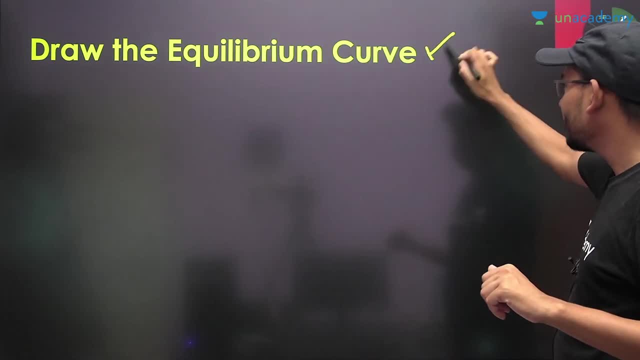 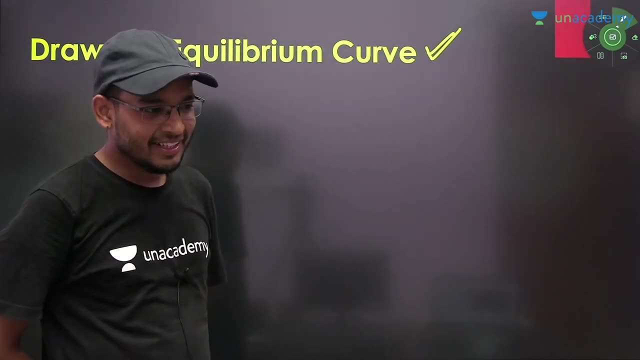 To reach the minimum reflux ratio. there will be an equilibrium curve on the way. So now you have to draw the equilibrium curve to find out the minimum reflux ratio. You have to define the equilibrium curve Now. to define the equilibrium curve, this is a whole lecture in itself. 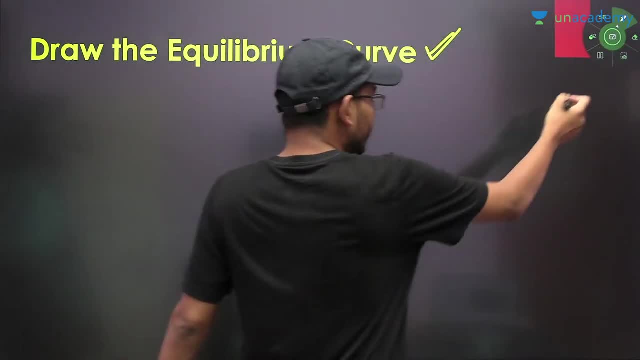 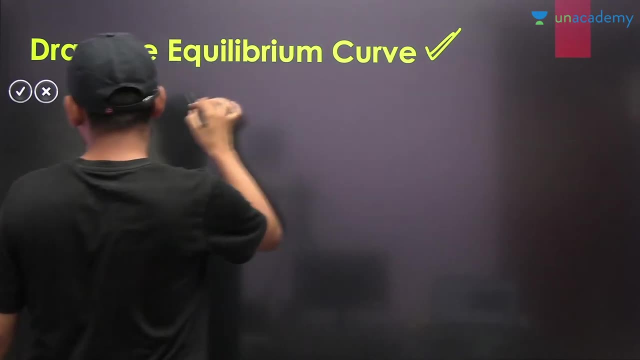 It is a whole lecture to define the equilibrium curve, Right? so all of you will add the heading equilibrium curve. I will give you a little idea. all of you will add the heading equilibrium curve. All of you will add the heading equilibrium curve. 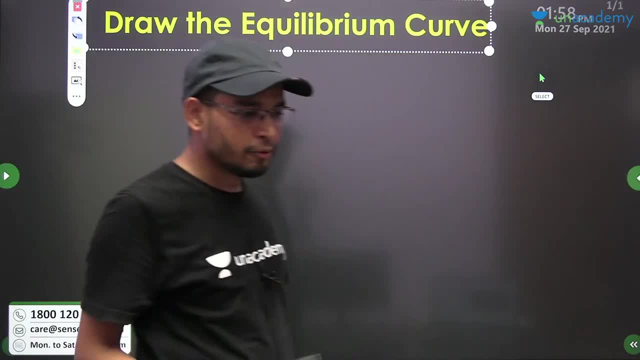 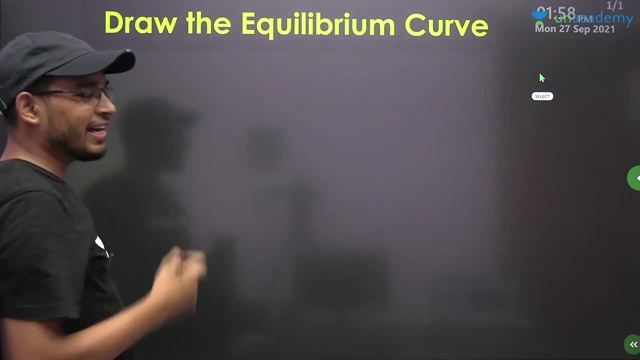 They ask questions in different interviews on this. They ask questions in different interviews on this. on the equilibrium curve: This is a different discussion. I have taught this in at least 4 or 5 lectures on YouTube. Go and watch it. I have taught it in at least 4 or 5 lectures on YouTube. 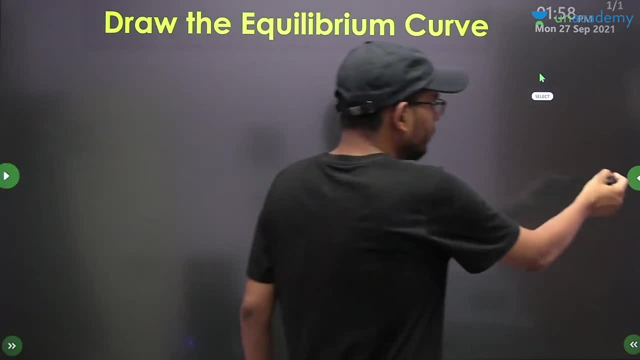 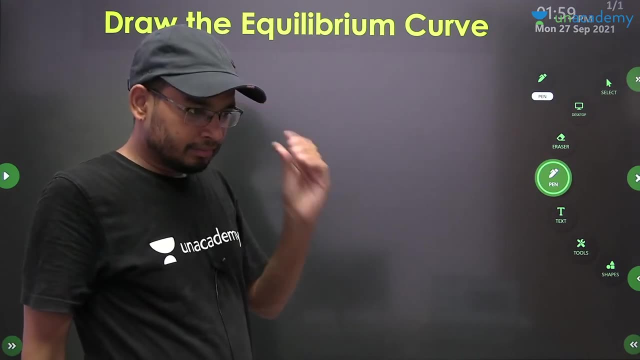 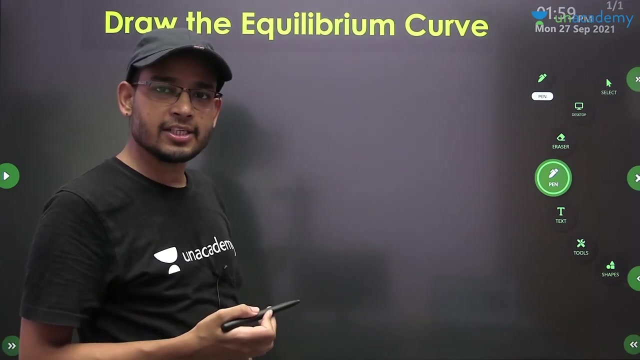 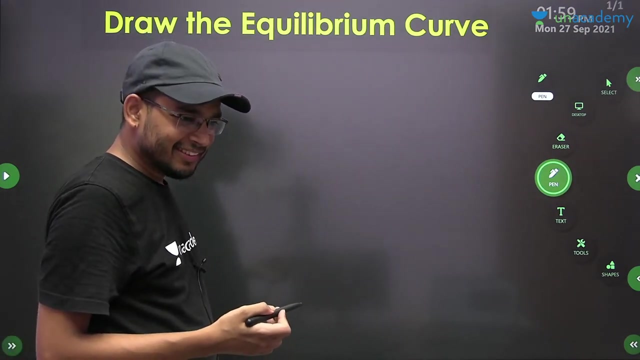 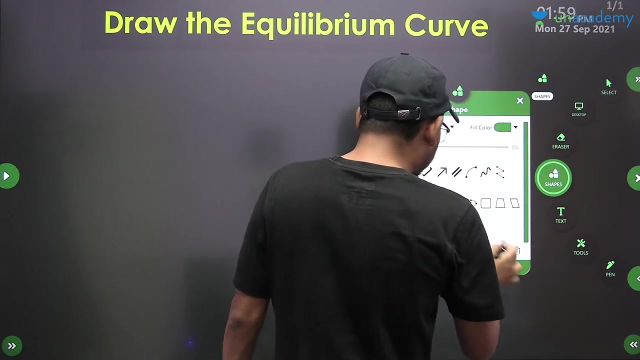 I have taught it in at least 4 or 5 lectures on YouTube. There will not be an end to it for a short while as there is a lot more in it, but if you have covered it here, then in interview you will be asked question from any distillation column. 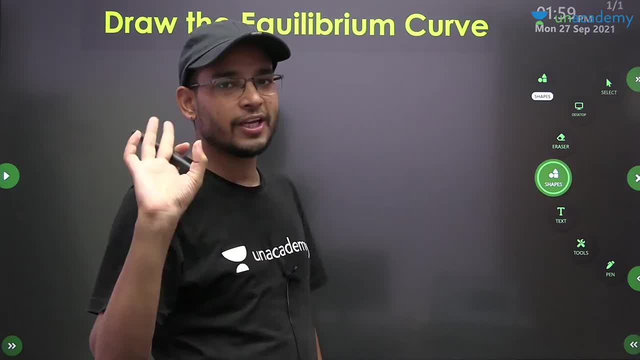 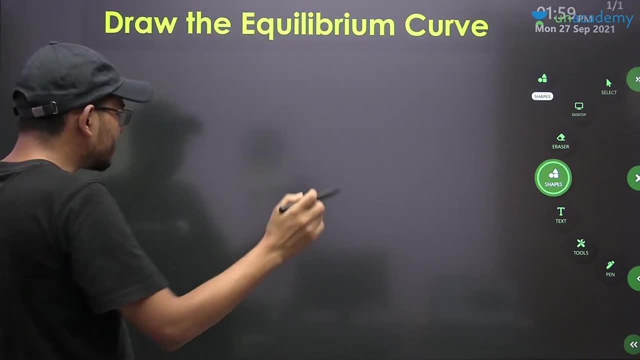 and in mass transfer. you will be asked question from distillation column, so you will definitely give its answer. i guarantee you this much. you should understand properly. draw the equilibrium curve. so first of all we have to define equilibrium curve. now, how can equilibrium curve be? you may have forgotten. 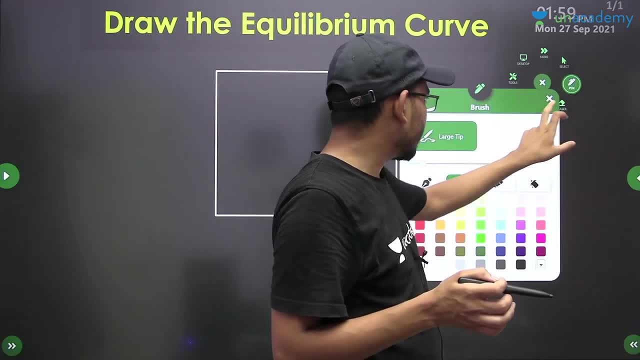 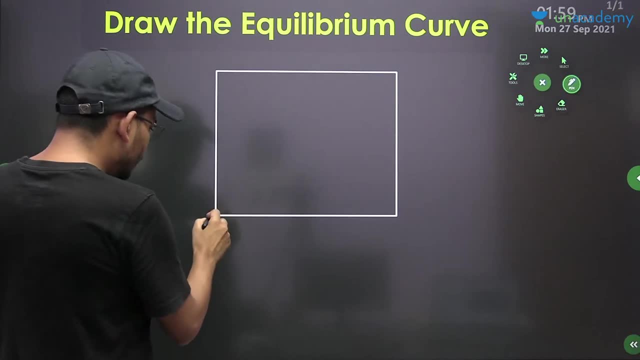 so i will give you some idea so that you will be able to connect properly, in case you have some idea. ok, if you remember equilibrium curve. so here you used to take less volatile component: xb is equal to 1, xa is equal to 0. and here you used to say: 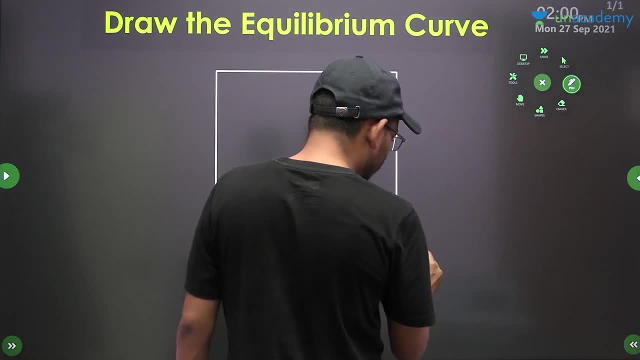 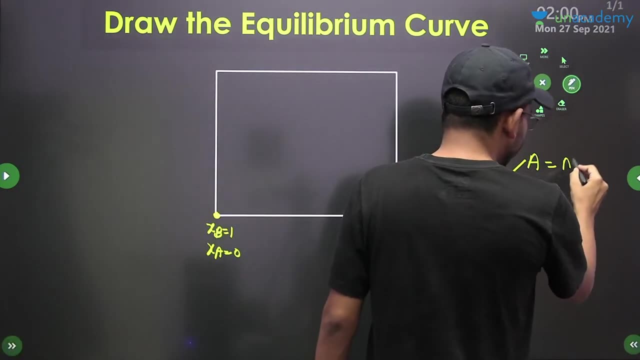 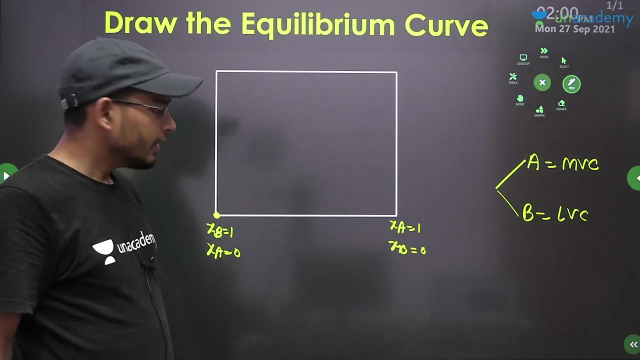 more volatile component. xa is equal to 1, xb is equal to 0. ok, what is a more volatile component? a is the more volatile component and b is the less volatile component. right, b is the less volatile component. you may remember, we have also known its pure boiling point temperature. 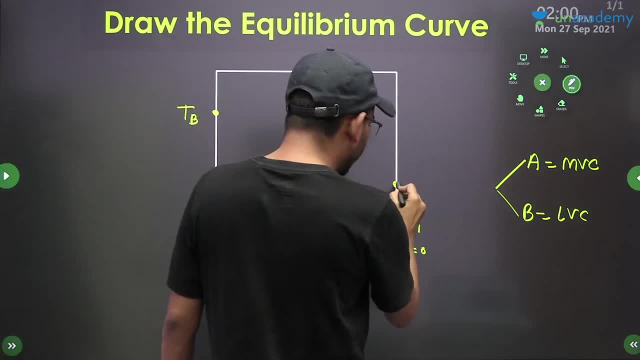 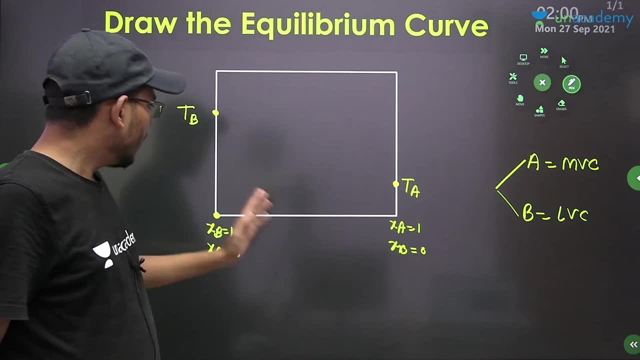 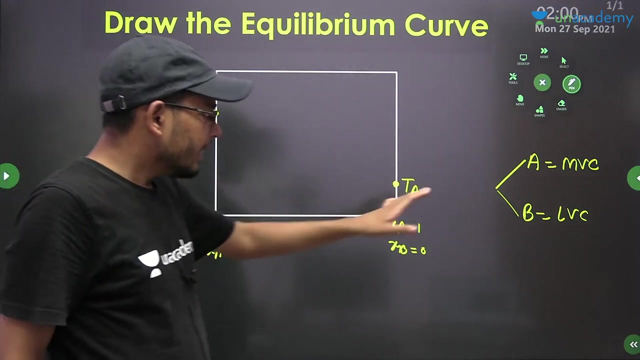 Tv and we have also known its pure boiling point, temperature, Ta ok. its boiling point will be less because its more volatile component is here and on this line. its pure is less volatile component, so its boiling point will be more right. this thing everyone understands. so the more volatile component. 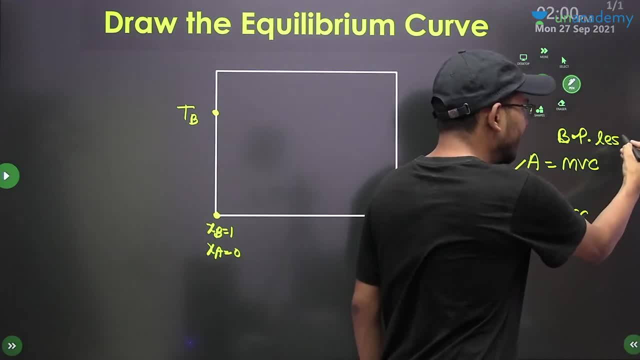 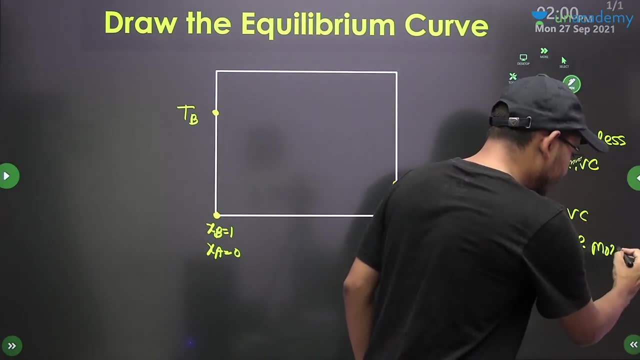 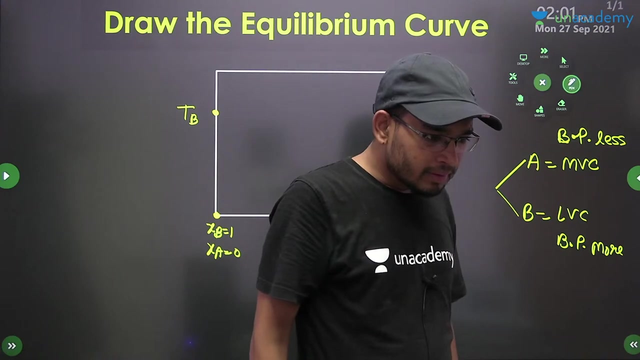 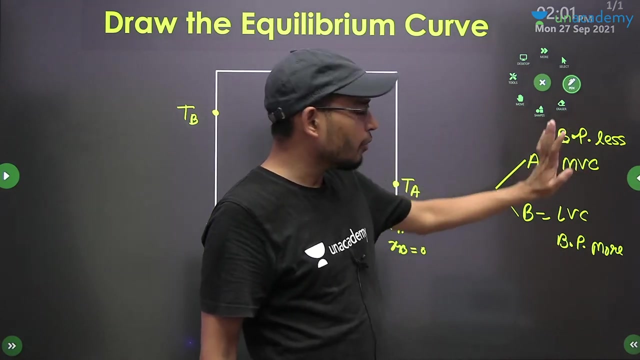 its boiling point will be less. comparatively less: boiling point component and its boiling point. its boiling point will be more. keep writing everyone very well. yes, Txy diagram. yes, so what will happen? boiling point will be more and its boiling point will be less. ok, so how we would have come up with this. 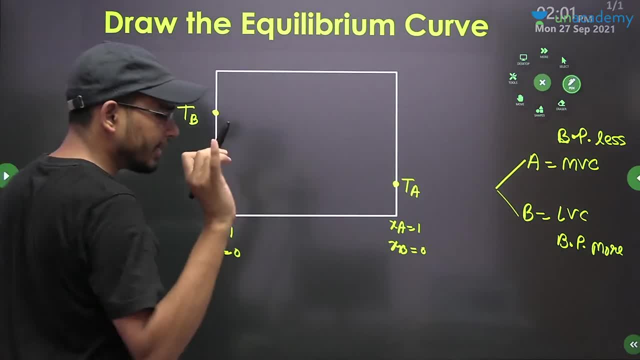 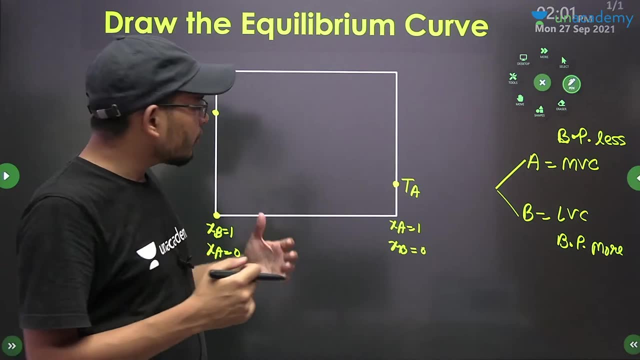 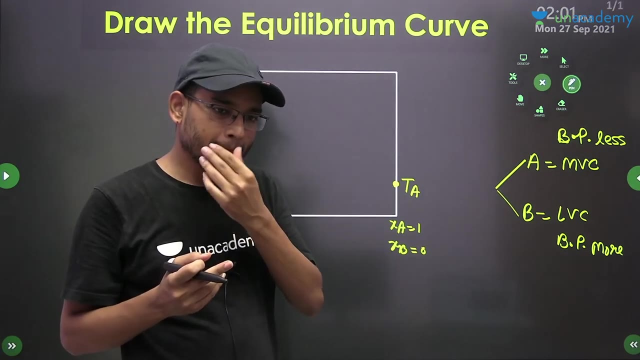 if you recall so, how to be the calculator of Tv and Ta, can you please tell me once? can you tell me once again? let me recall you how to be the calculator of Tv and Ta, how we would have calculated. do anyone remember? please tell me quickly, only then. 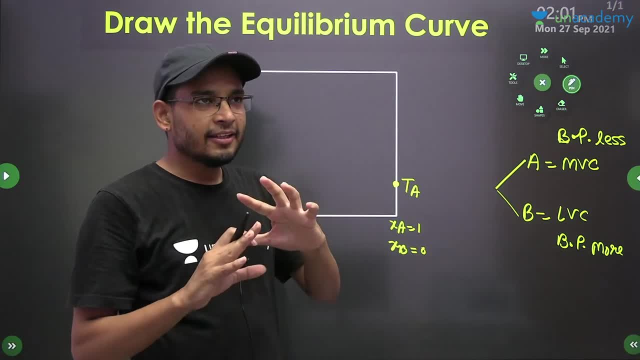 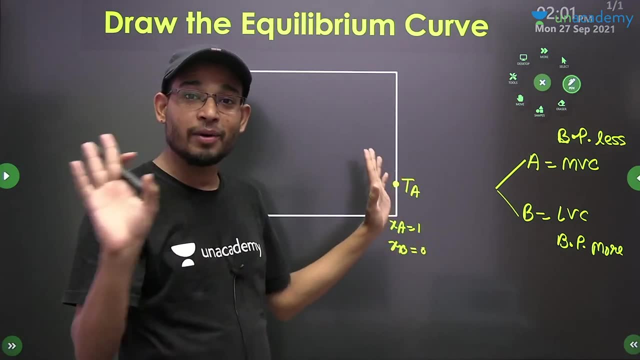 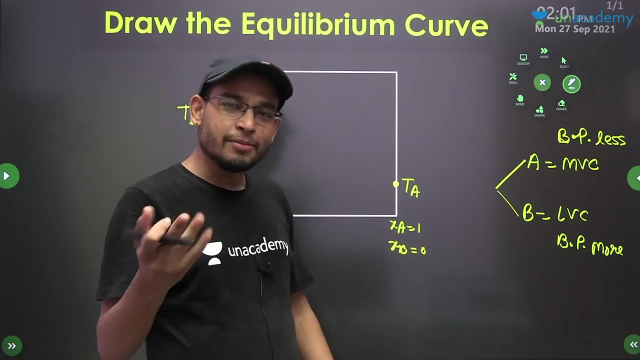 the system will be fun only then. it will be fun. otherwise, and i will teach you how to do it- you will see two kids and i will teach them. i have decided that i will teach them. well, but i will leave it later. you will see it, yes. 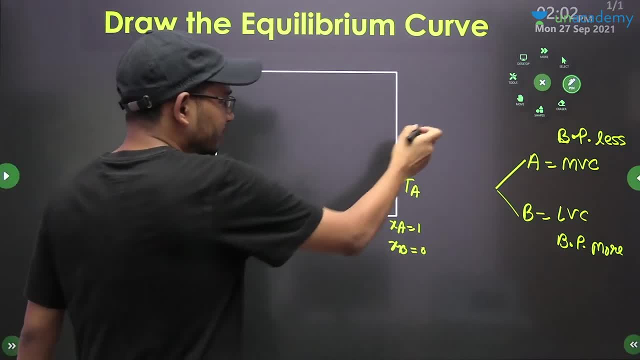 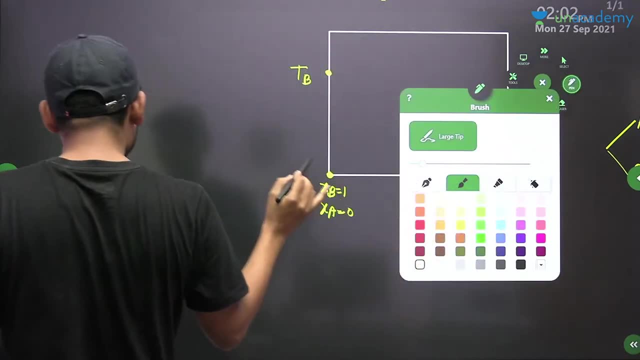 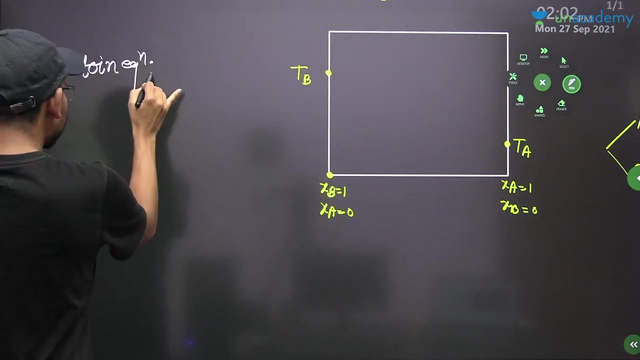 from antoine equation. very good, from antoine equation. from where? from antoine equation come here. what was antoine equation? everyone will keep writing: what was antoine equation? yes, very good. what was antoine equation? ln p set. let me talk about p set. 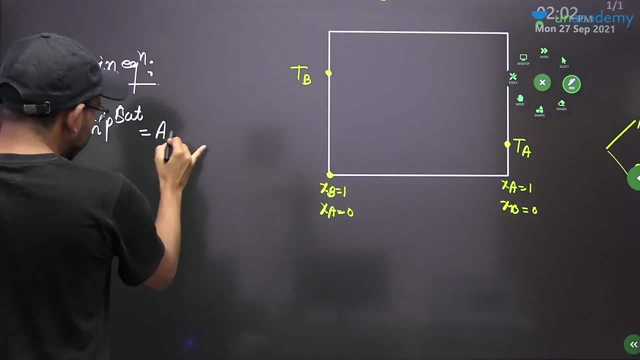 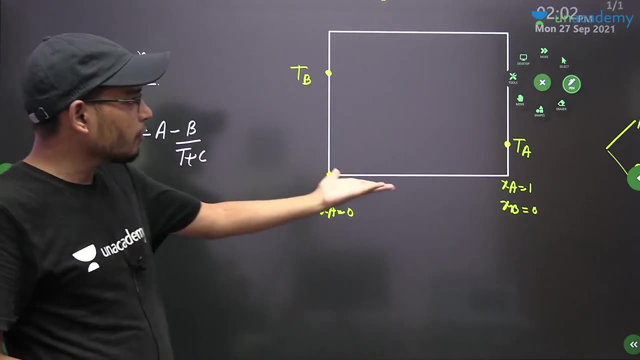 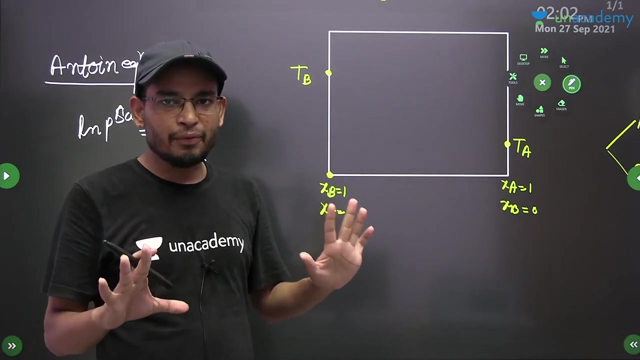 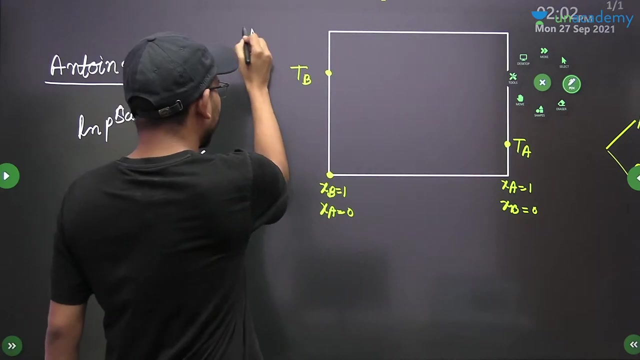 p set is equal to a minus b upon t plus c. this was antoine equation. so, whatever column we are operating whenever you are defining the equilibrium curve. so you have to fix one quantity, you have to fix the pressure or you have to fix the temperature. so this diagram will be: 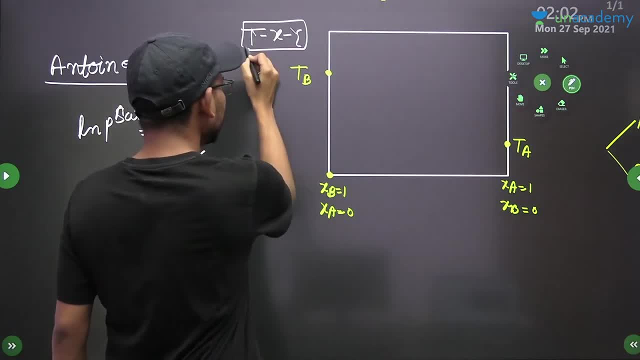 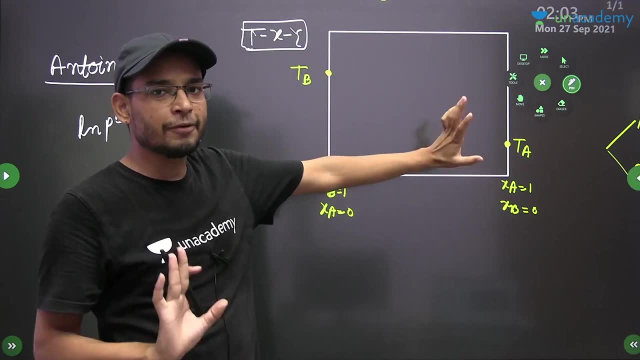 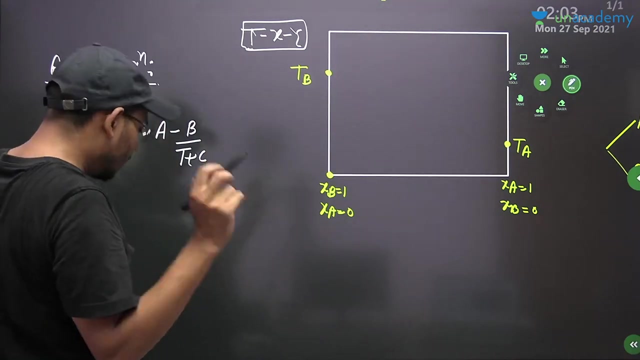 we are talking about txy diagram. so txy diagram means we will fix the pressure here: 1 atm, 2 atm, whatever it is, but the value of pressure will be fixed. ok, now what do we need? tb. so understand the concept very carefully. how will we find tb? 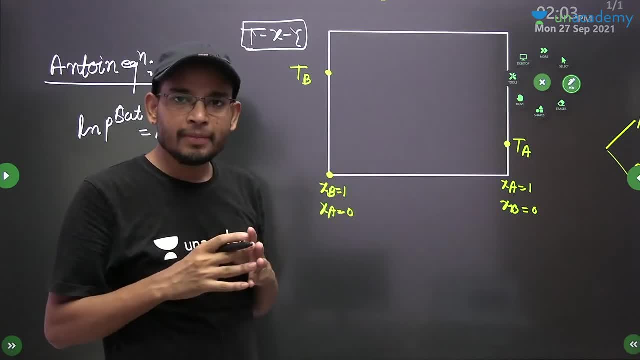 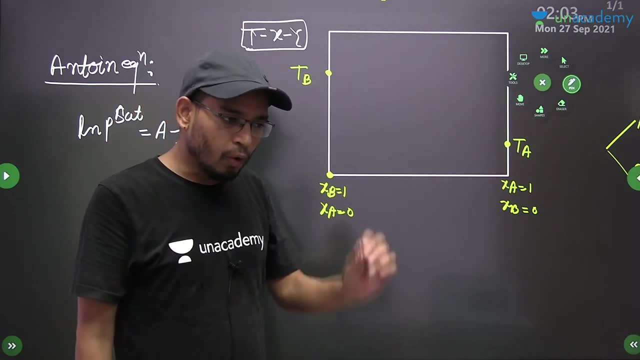 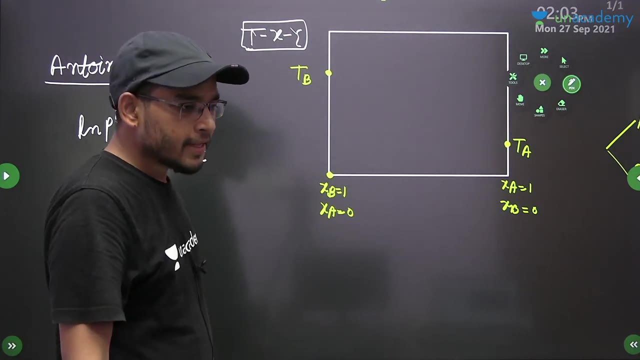 what is tb? it is the boiling point of the b component. now, what is the concept of boiling point? someone will tell me here what is the concept of the boiling. what is the concept of the boiling, will everyone tell me? the lecture of the students who are studying on plus is going on. 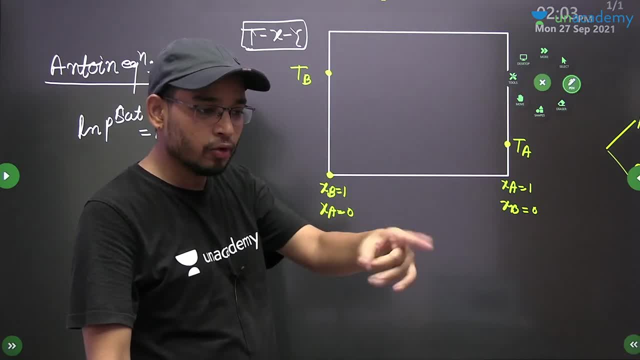 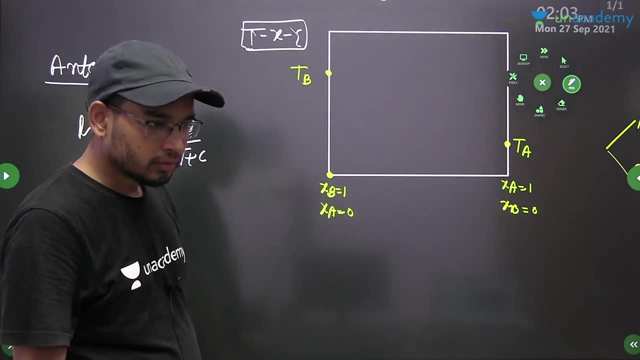 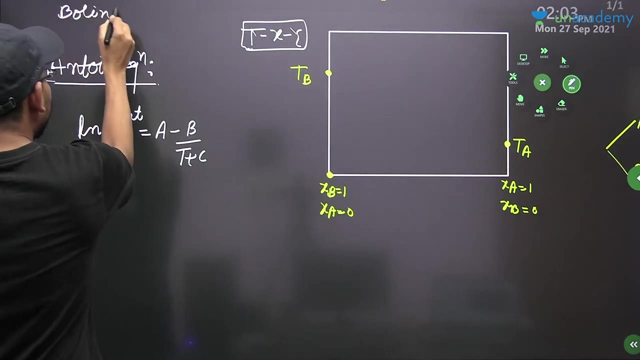 ok, it is over. in the last, very strong- whoever is a plus student will be smiling. p total is equal to p set. ok, p total is equal to p set. very good, so what is the meaning of boiling? what is the meaning of boiling? p total will be equal to. 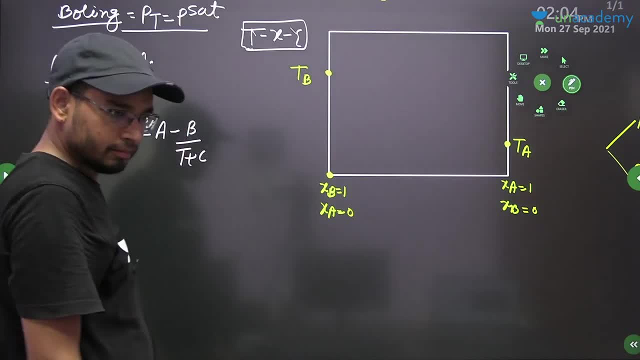 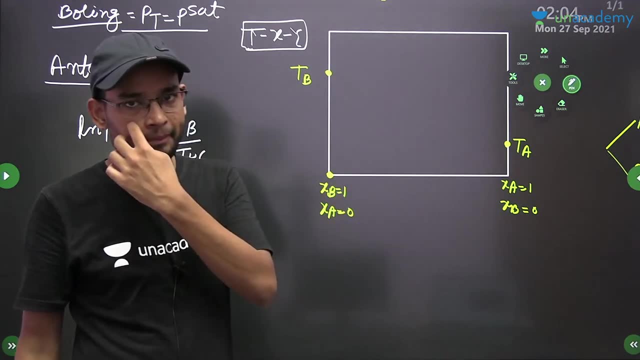 p set. you have read this in the 8th class. ok, just like. saturation, pressure will be equal to total pressure. what will it mean? boiling will start. what is boiling? evaporation is a surface phenomenon. evaporation is different, but boiling is different. what is boiling? 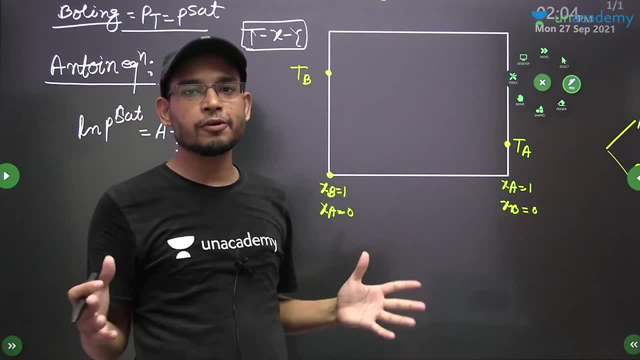 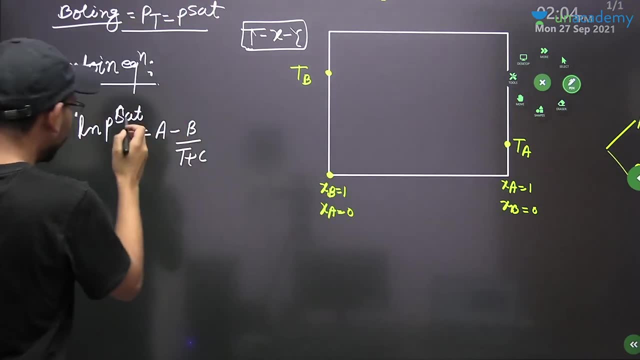 in boiling the bulk moves, in evaporation only the surface molecules move. ok, so boiling will happen. so boiling means total pressure is equal to saturation pressure. so your pressure is fixed here. what is your pressure? it is fixed, you will keep the pressure here, p total. 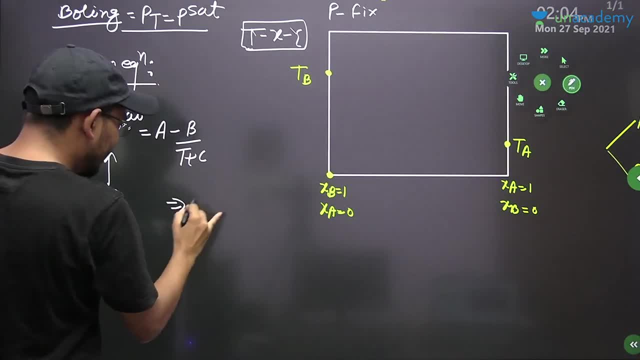 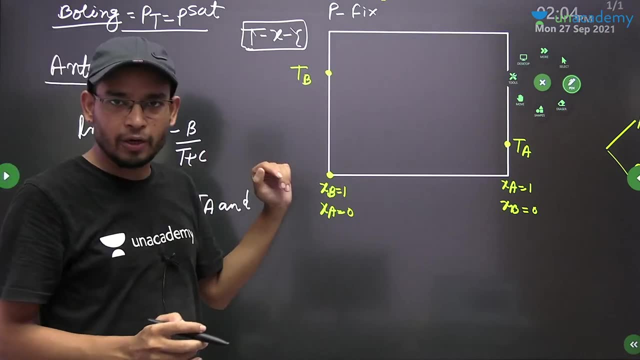 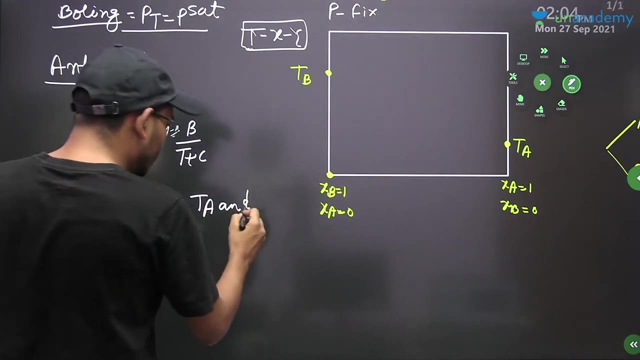 ok, so what will be calculated from here? here your calculation will be TA, similarly TB, because ABC component will be different, for TB will be different for A component and for B component ABC will be different, so the value of ABC will be different. so from here you will calculate: 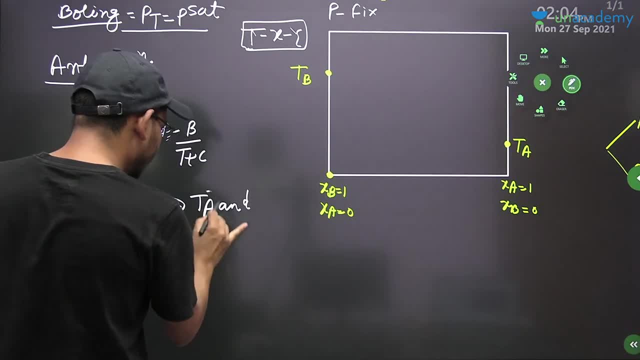 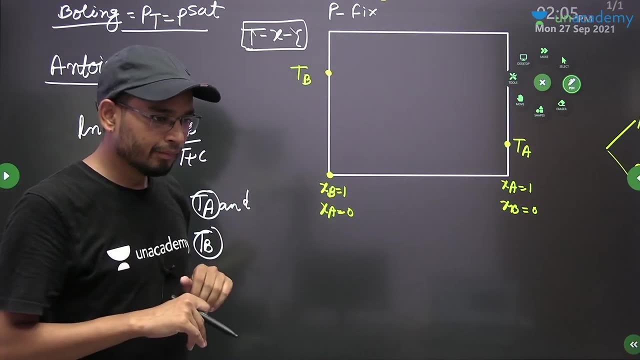 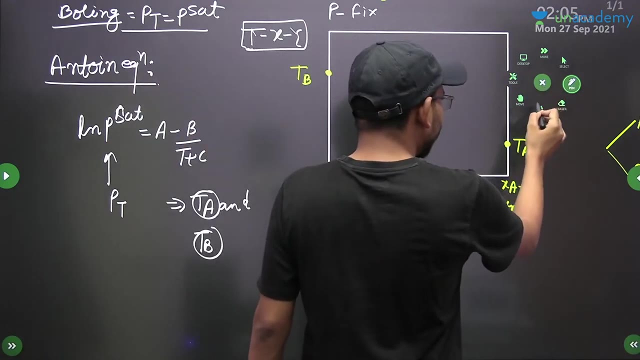 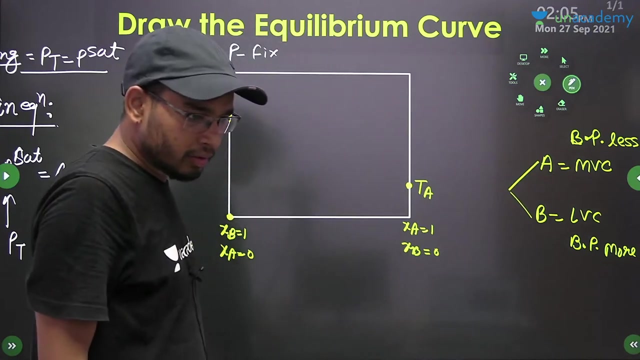 TA and TB. first of all, everyone understood this: how to calculate the value of TA and TB. everyone understood this. yes, boiling will occur, not boiling point. boiling will happen there. this is the condition of boiling. this is the condition of boiling. ok, MR100, this is the condition of the boiling. 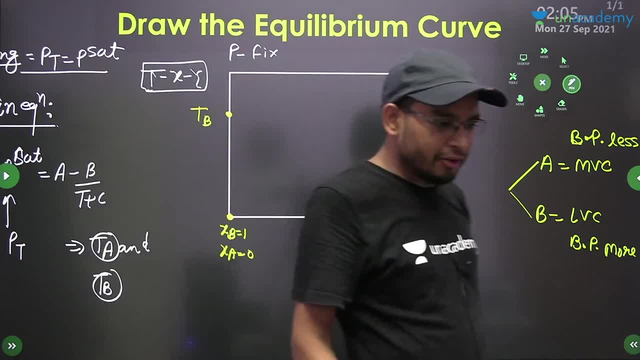 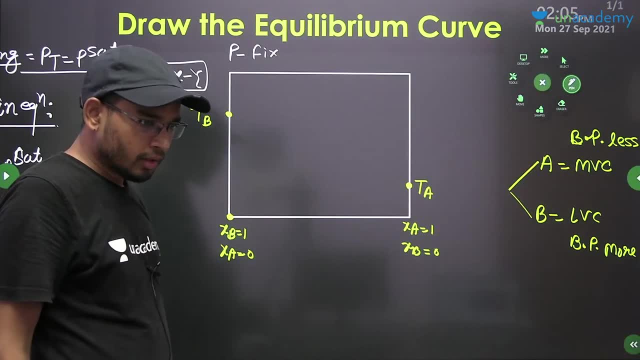 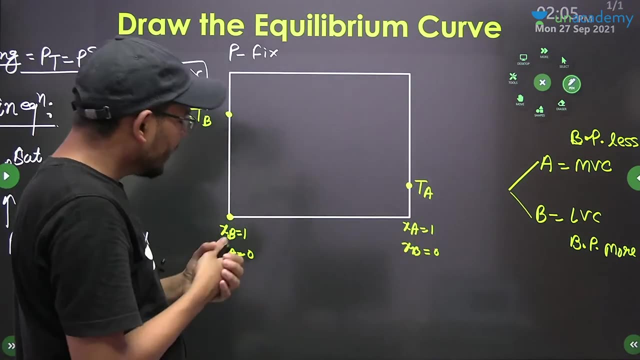 everyone understood TA and TB. everyone. everyone reached TA and TB. everyone reached TA and TB. tick. now, what did you do? what is this? this is the range. this is the range, ok, so let me take a mixture. let me take a mixture of A and B. 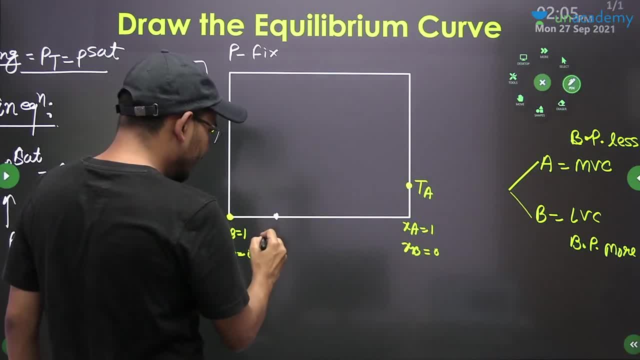 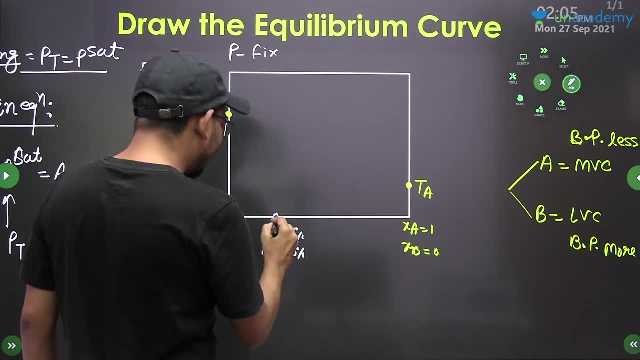 whose composition is: B is 60%, B is your 60% ok and A is your 40% ok. so what did you do? you started heating the system. you got the first point. you got the first point in the same way you used to talk. 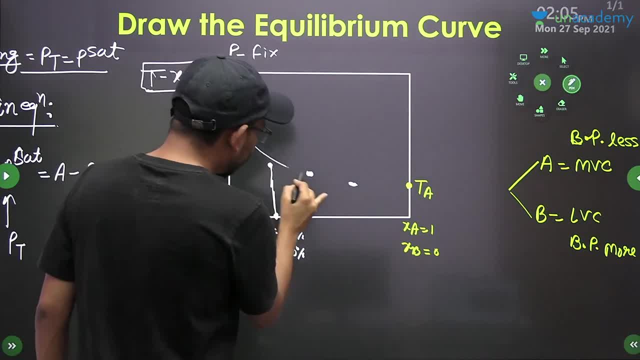 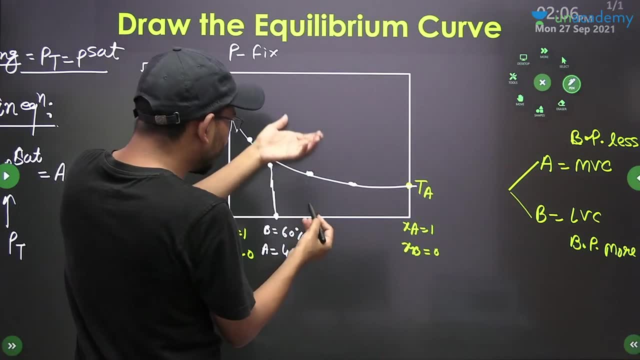 does anyone remember a little? does anyone remember in this way you used to get these points and similarly, you then: what did you get? this was your liquid, this was vapor, liquid plus vapor. then you used to heat, then the last drop of the liquid vaporized. 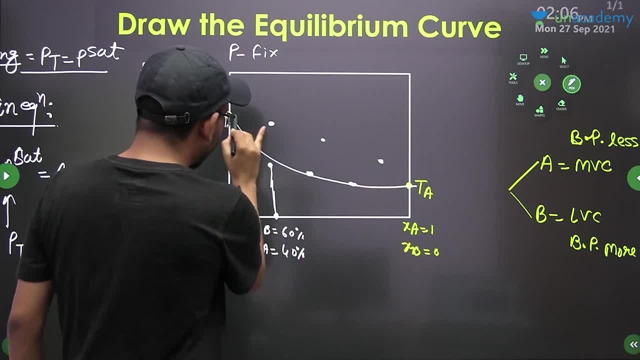 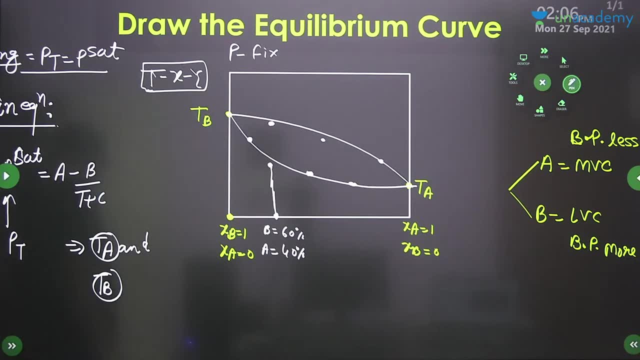 then you used to get these points, then you used to get the last drop of the liquid. similarly, what did you do to them? you used to join them. similarly, what did you do to them? you used to join them. ok, so what did you do to them? 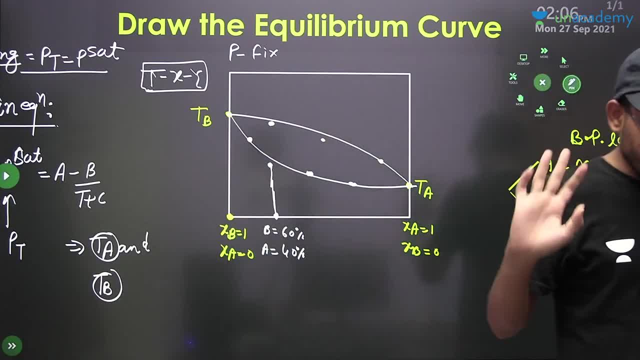 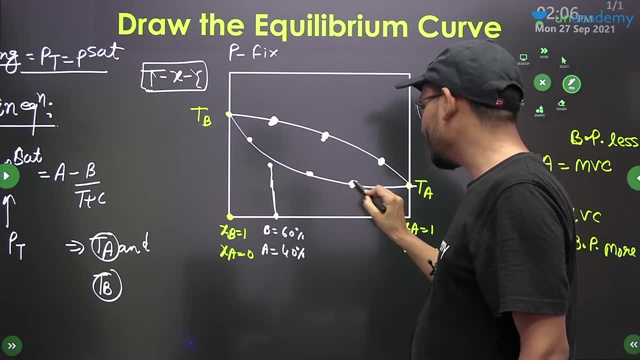 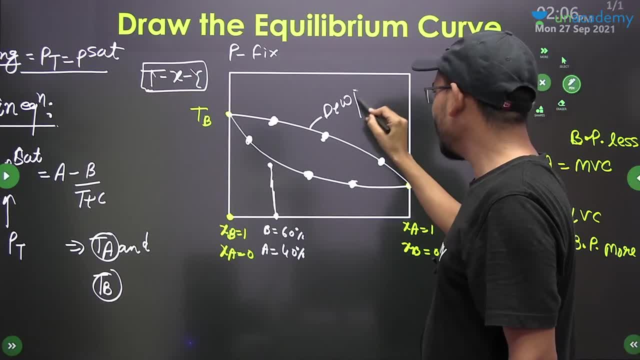 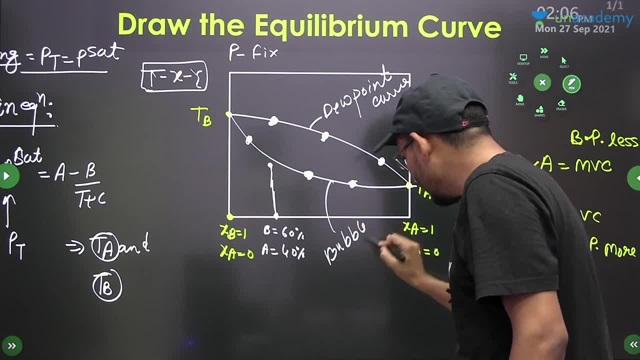 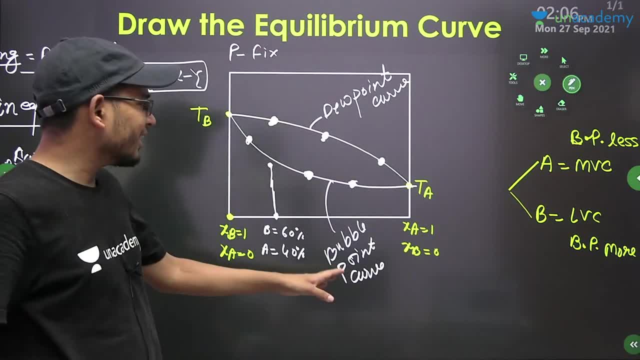 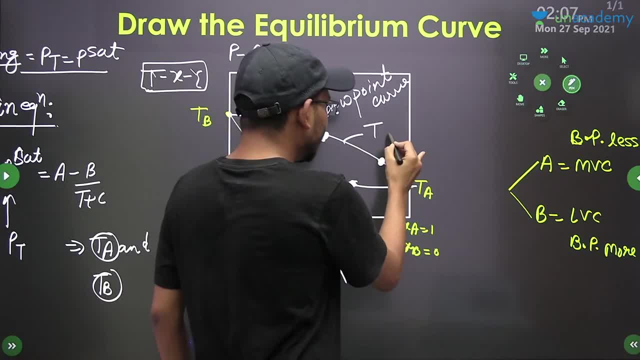 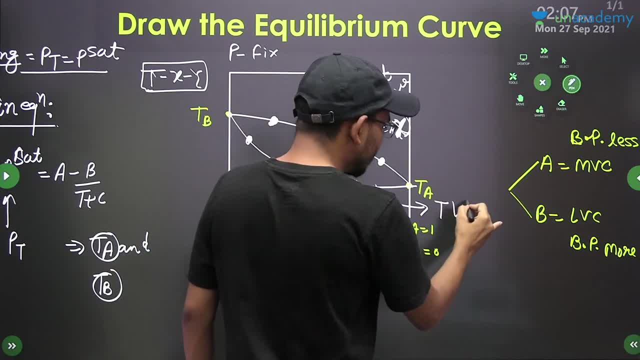 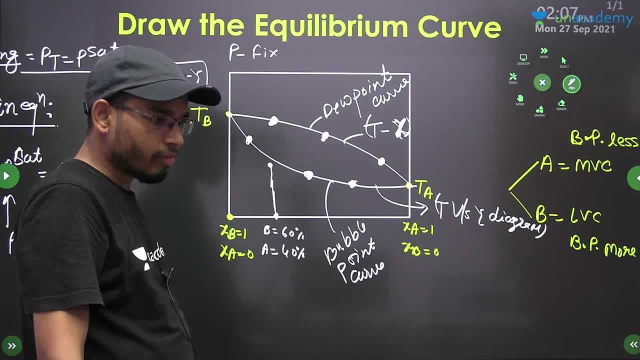 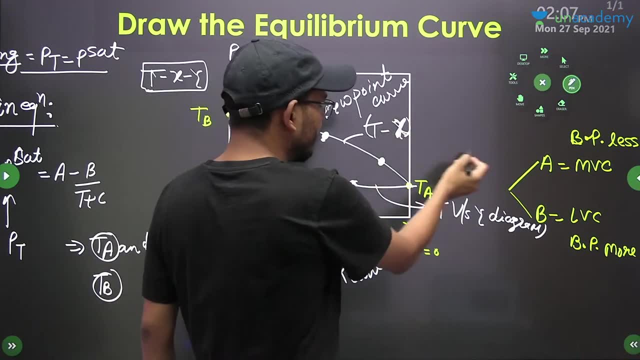 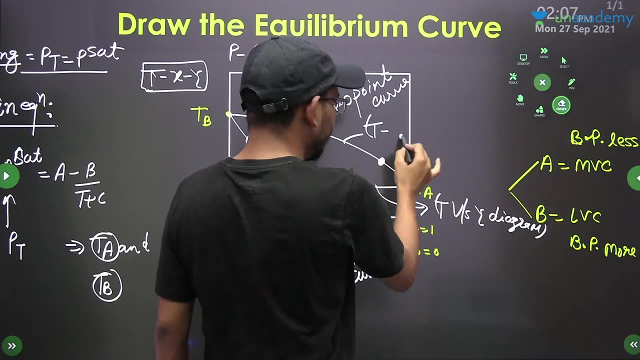 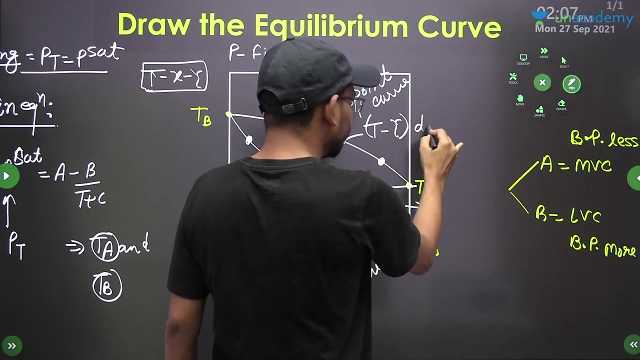 this is the dew point curve. Yes, this is ty. it's a little upside down here. fix it a little. fix it here. this will be ty, this will be tx. this is the ty diagram and this is the tx diagram. 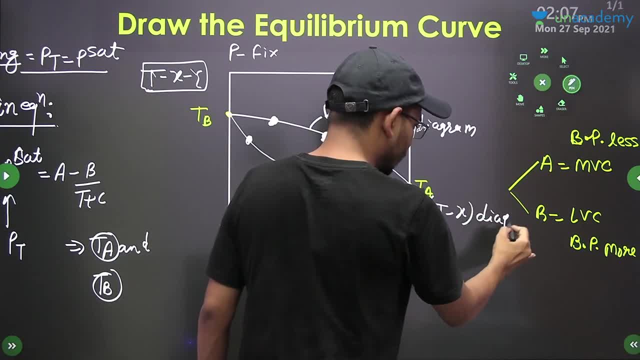 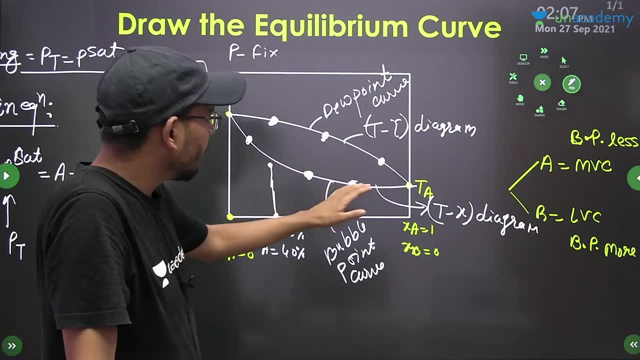 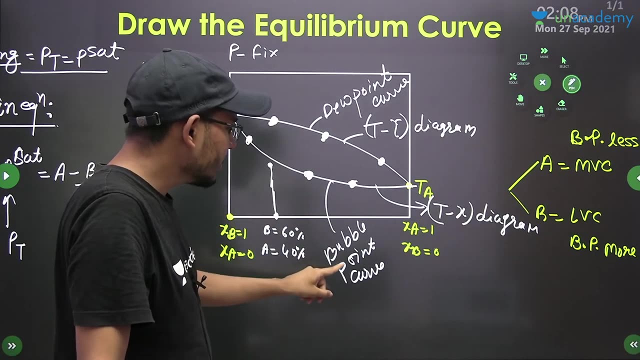 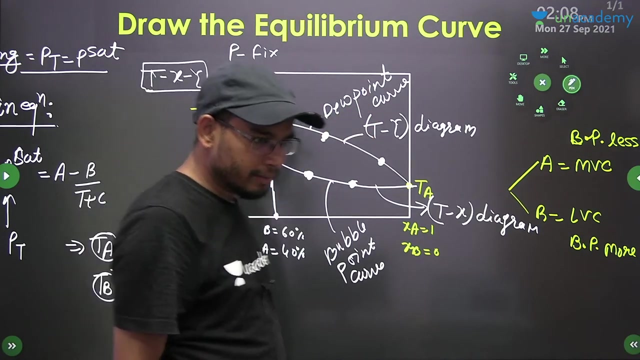 Yes, locus of the all the bubble bubble point. this is called bubble point curve. locus of the all bubble point is known as bubble point curve. locus of the all dew point is known as dew point curve. fine, sure Done. 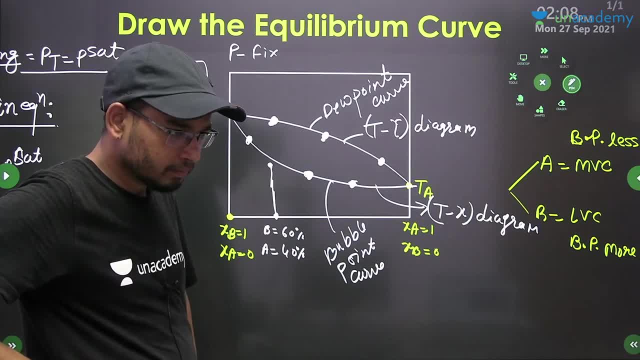 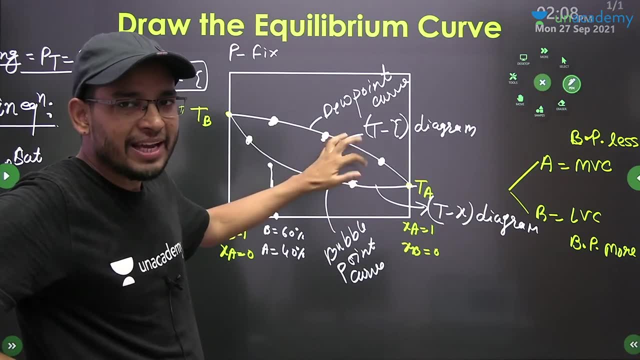 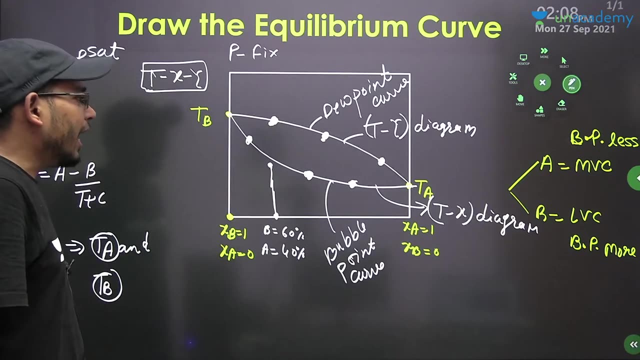 Perfect. you guys write down enough here. See, i just showed this, as a graphical method means experimental method. It's actually an analytical method. you guys will also learn that one. Now we have to make a xy diagram First. we got a about this much already understood. 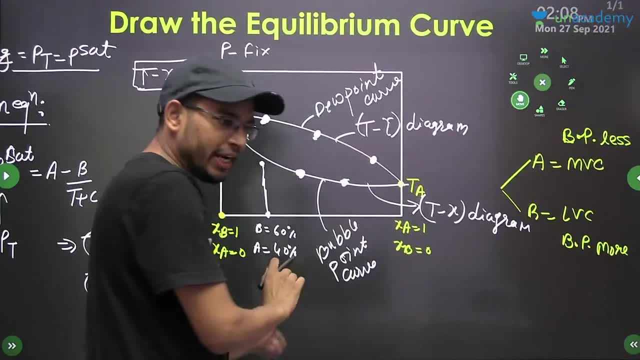 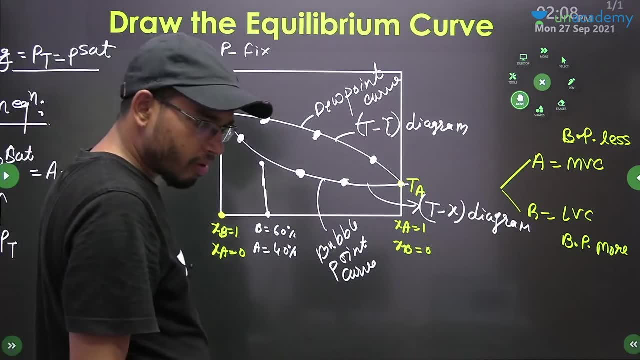 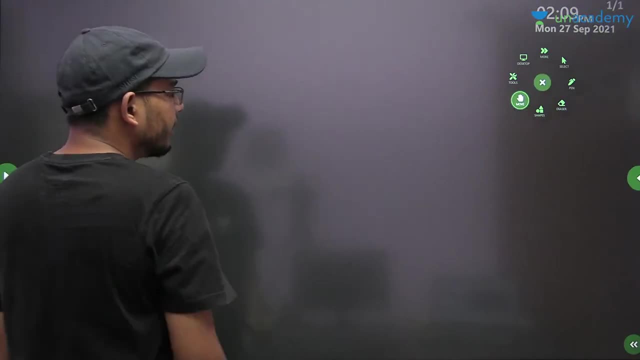 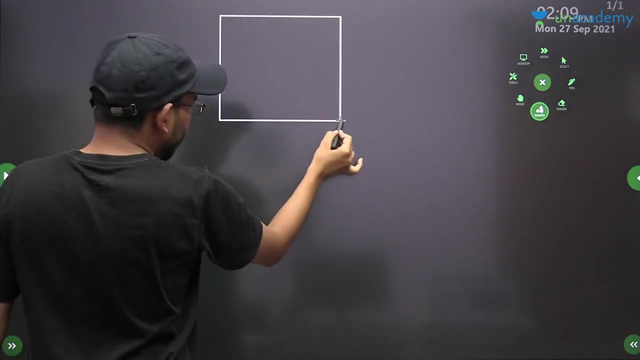 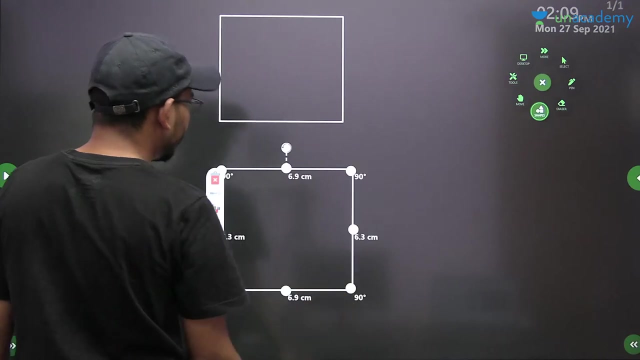 Now i will draw it very close to the first line away. Now I will talk about the xy diagram. so see very carefully: now you make two figures. you have made the txy diagram. now you have to make one more xy diagram. now I will talk. 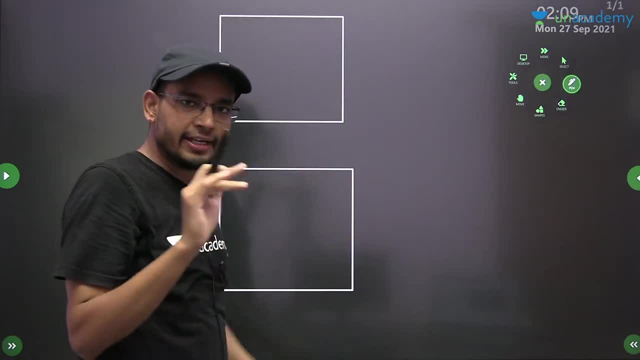 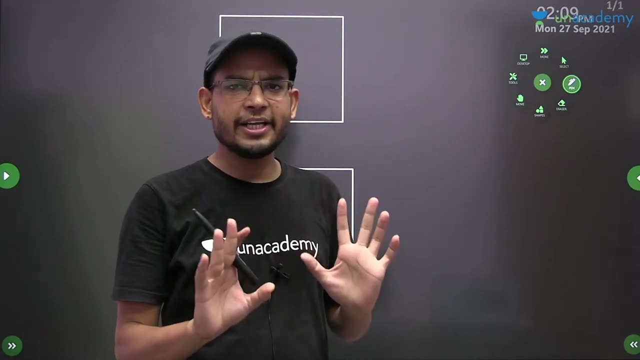 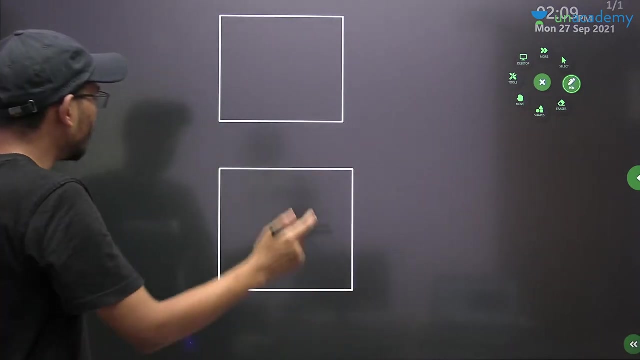 about the xy diagram. you have learned the xy diagram. who wants the txy diagram in very detail? go to youtube. all my sessions are there. I have taught the txy diagram in detail. tell me one thing: how will you keep a point I have told you there? okay, you can go there. 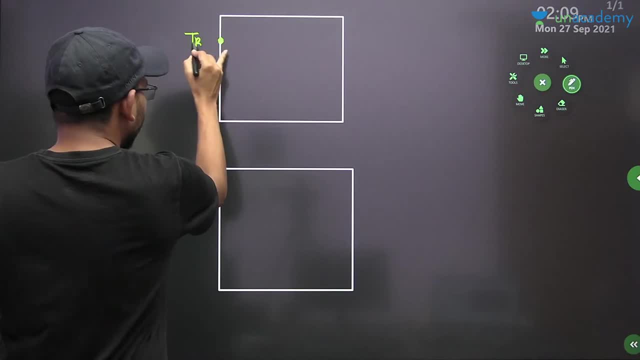 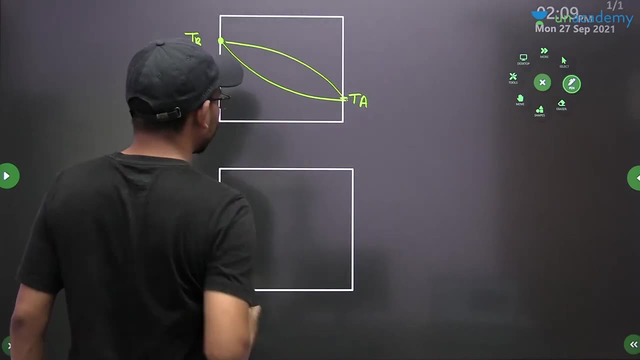 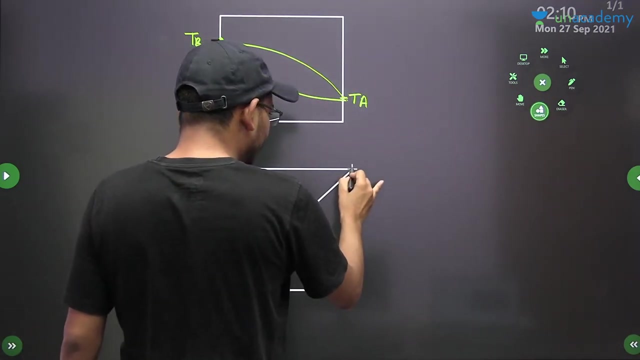 and see. so this was your tb and this was your ta, right? a child also made such a nice figure of it and sent it in excel. it's very good, okay, and this will be yours. txy, this is your diagonal 45 degree line. okay, this is the 45 degree line. now you have to make. 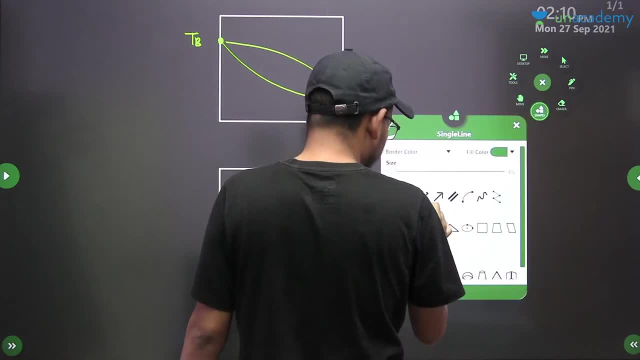 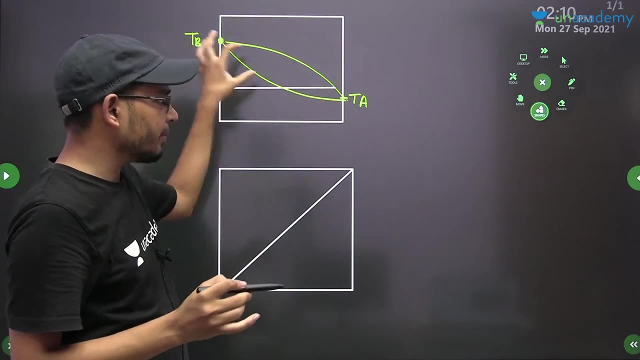 this xy diagram. so understand all of you at once again quickly what we will do. we will go to a particular temperature. suppose you go to this temperature. you go to this temperature. okay, any middle. have you to bit medium temperature? okay the thing. 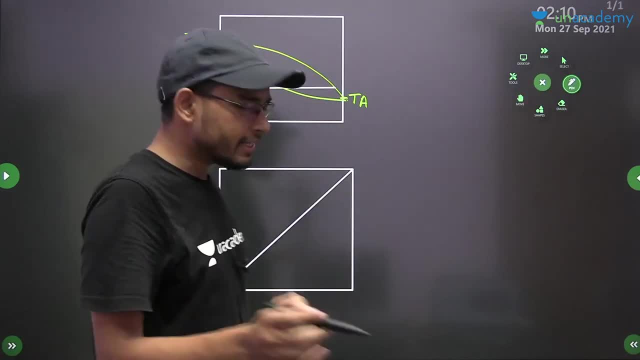 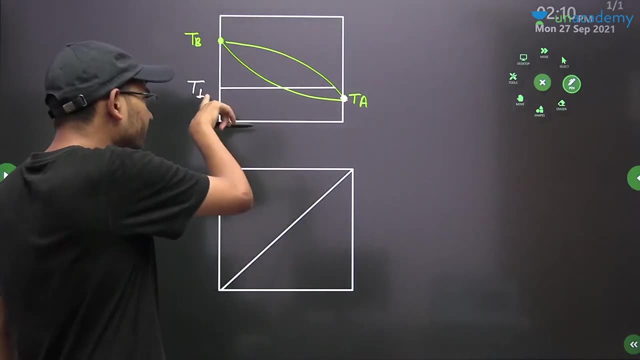 happening in designing. We choose a temperature between a town with whom the meeting between possibility and tb, between which any of the greatest intermediate t1 temperature has to play. okay, now, whatever intermediate temperature should choose then, what will that liquid plus vapor will do? 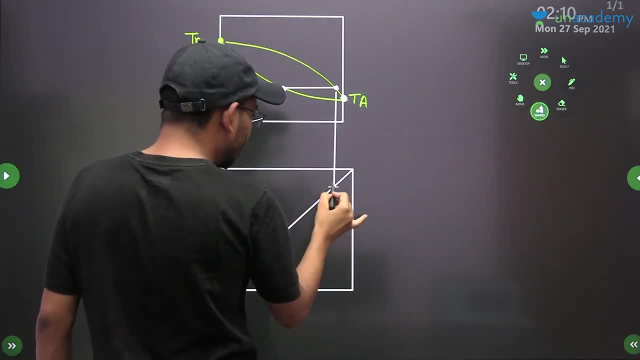 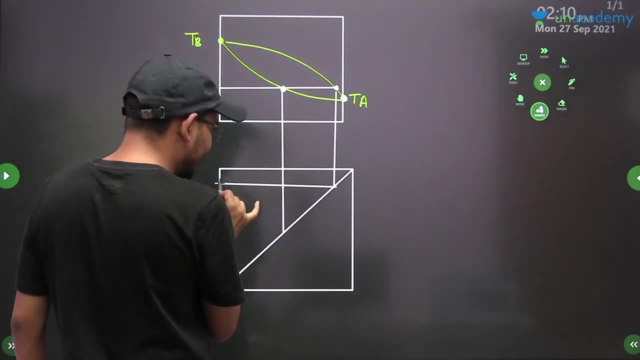 will separate it. then he will do it in liquid plus vapor will separate it. then you put the paper here on the diagonal, on the xy line, and do it even with X line. okay, and what to do with it? parallel to the x-axis. right, Let me make it from the dotted line. Let me make it a little. 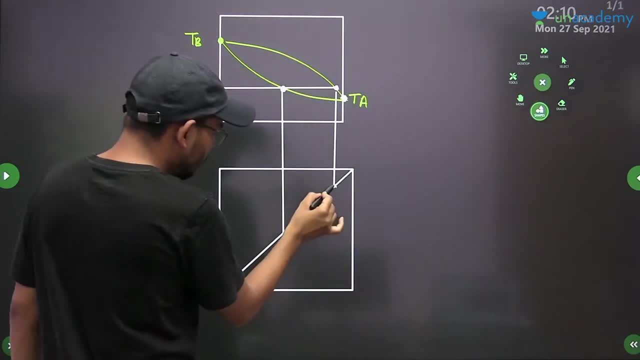 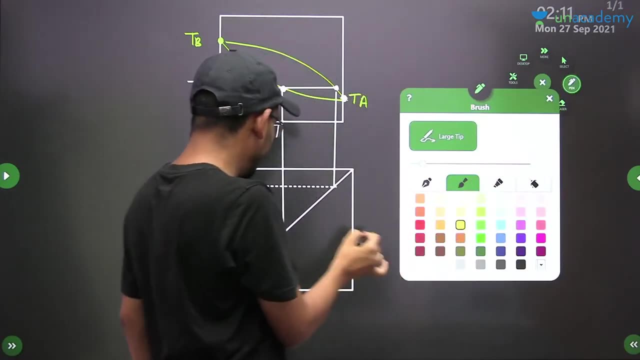 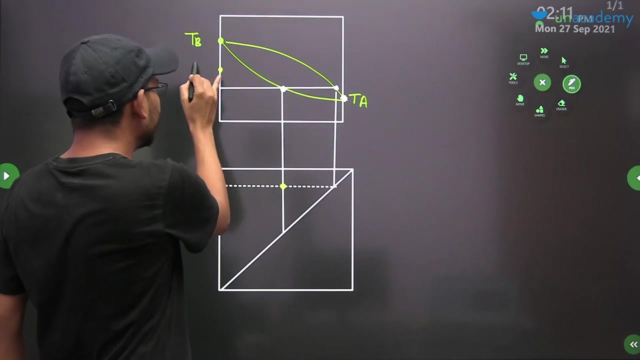 dotted line. This is how you do it, Right. So which one did you get? You got one point. this one, This one. You got one point Right. Then what will you do Then? choose another temperature. Then you choose another temperature: T2.. Okay, You choose another temperature for this. 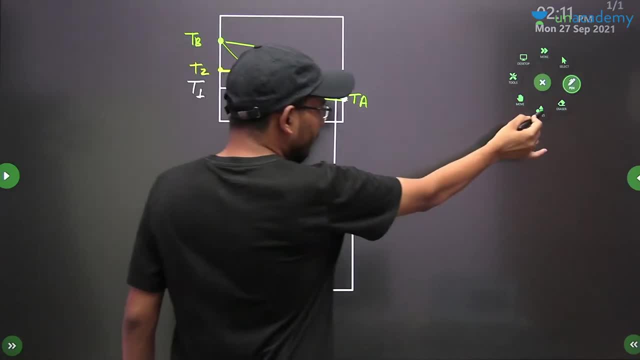 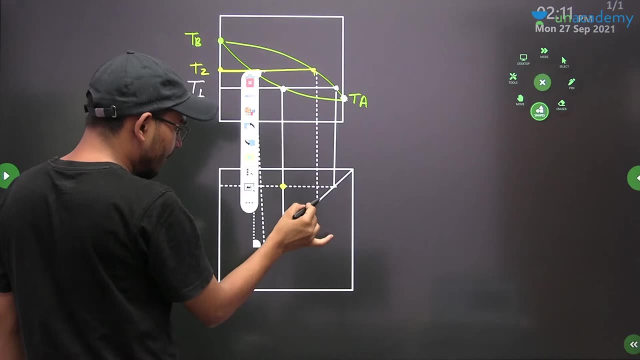 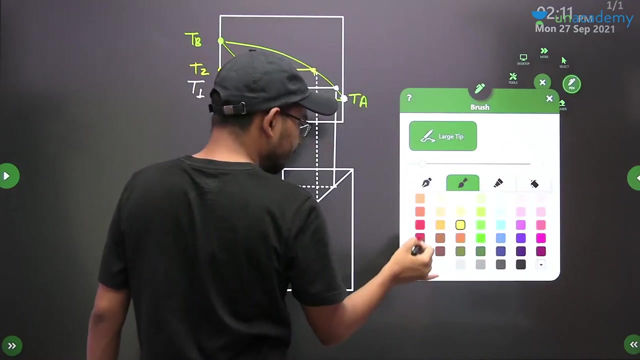 Here also. you got y and x. Okay, What did you get? Your y? Everyone understood right. Again, you got your y and this is your x. Okay, And you moved it horizontally again. So you got another point again. You got one again. What is the second point? Okay, You got this point. 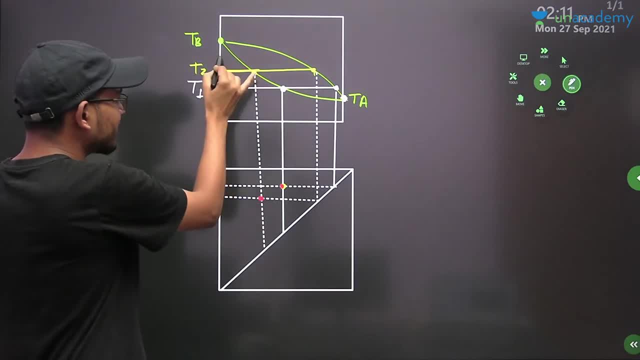 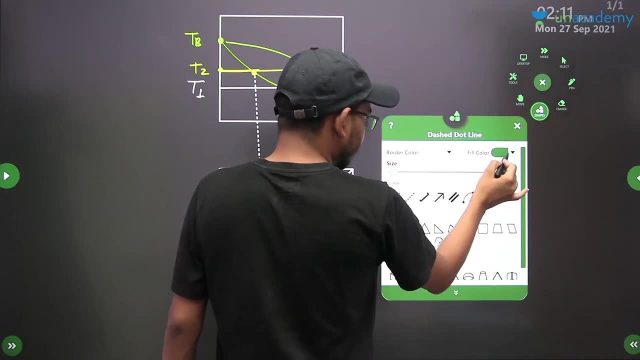 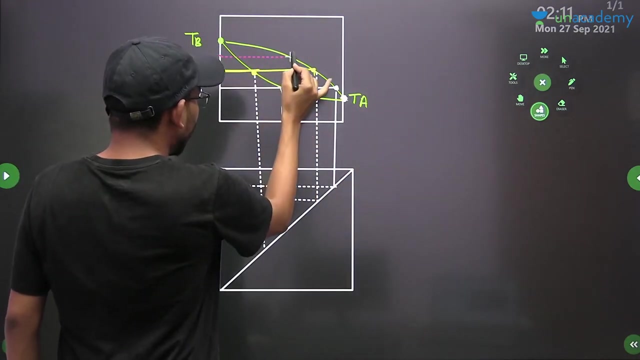 You got this point: Means T2.. Again, you chose a third temperature. Again, you chose a third temperature. So I am changing the color. Okay, Look very carefully. you chose a third temperature, All right. Again, you got your x and y data. x and y data. 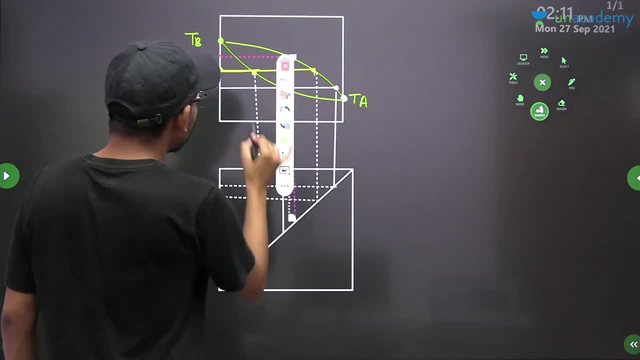 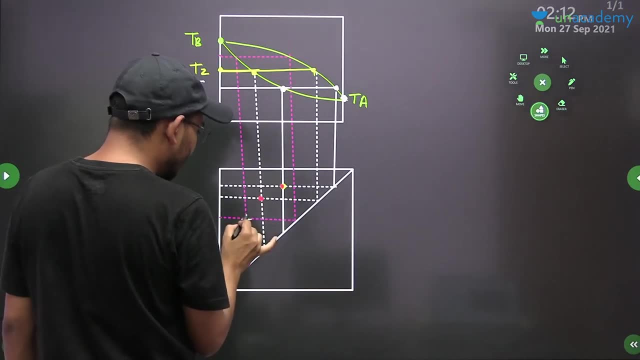 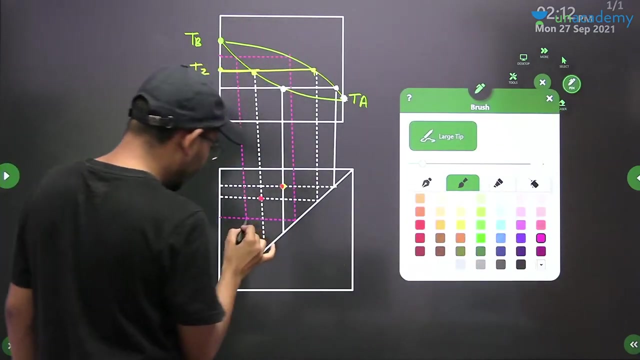 You can directly sign it below. And you got liquid data from here, Right. And then you moved this forward again. So, again, you got one point? Which one? This one, Okay, You got this point. Fine, You got this point, All right. So you got this point as a point, All right Now. your paper is called liquid data, then that is what we will do. Next, we will do the prior second point In the following on the 3rd time we have to remember the point a little. All right, So in the following: once again, you have the information we had. so we will get the data. Okay, You will get the data. It will be because of this. it is the point. Okay, You will get a point again, So you 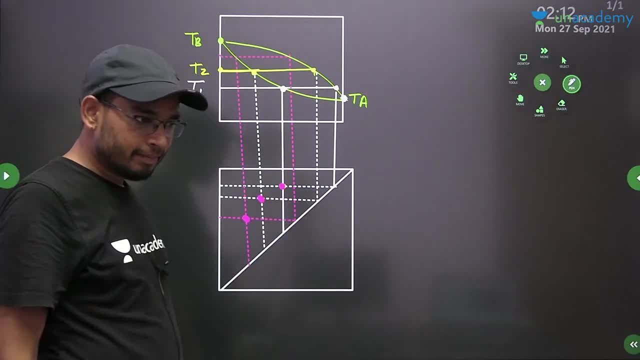 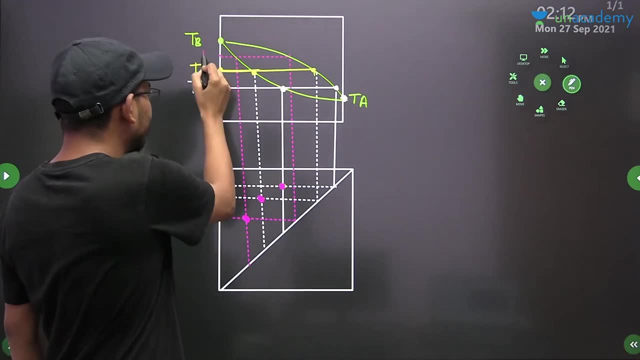 what will happen. everyone will understand. this is coming to everyone, as much as your tie lines will be. you will get that much points. one tie line, two tie lines. this is T3, then T1, T2, T3, then what is the temperature of T1,? what is the temperature of T1,, this one? 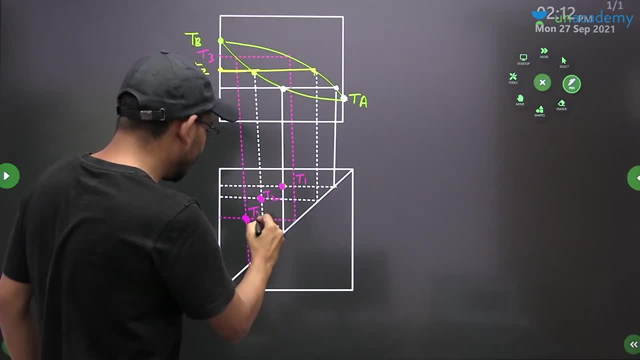 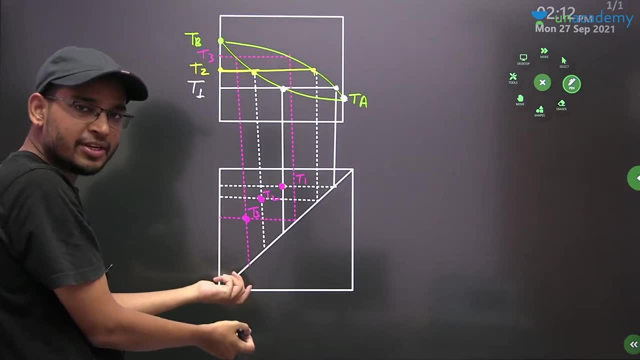 T1,. what is this temperature? T2, what is this temperature? T3, ok, as you will increase, then it means where the temperature is increasing top to bottom, then what happens in the bottom? what happens in the bottom? the temperature is not much, you are seeing, and what will? 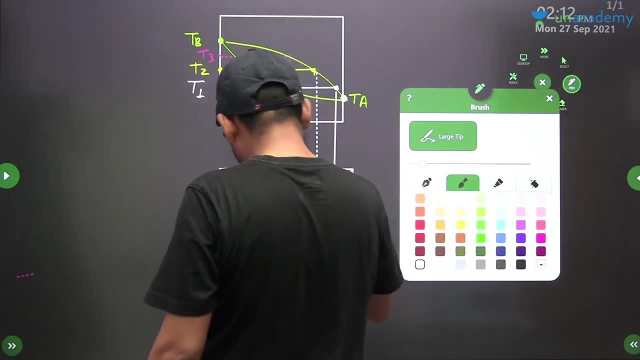 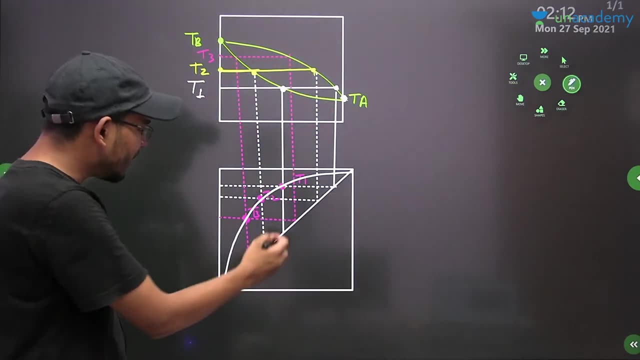 you do? you will mix them. what will you do? you will mix them properly. ok, you will mix all these points properly. this way, your equilibrium will be formed. ok, you will see where the temperature is increasing in the bottom side, because see which one was your. 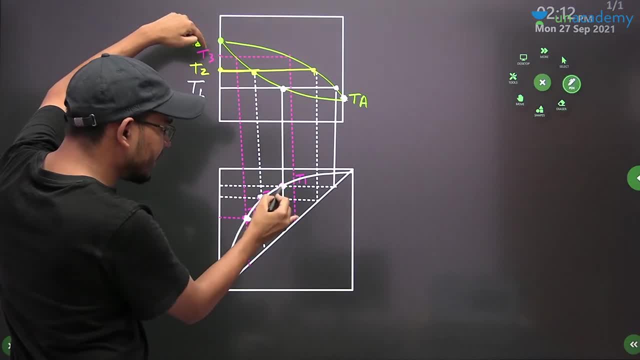 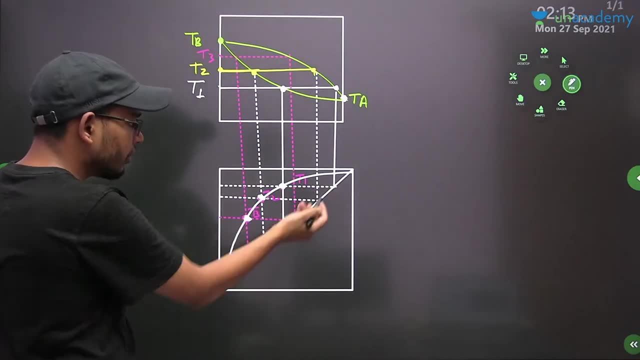 T3, this one? ok. which one was T2, this one. which one was T1, this one? so T1 was less T2, then where is your bottom? here you get XW. where is XD in the top? ok, so what will? 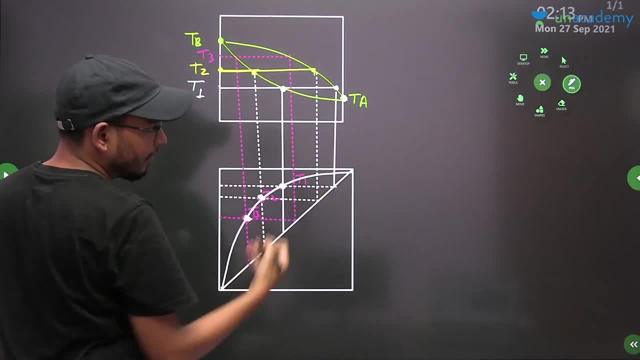 happen in the top. you will have to do more here. If you take a minimum temperature here, then you will get a point here. ok, so in this way you get T1, T2, T3, so if you mix them, then the temperature in your diet. now what? 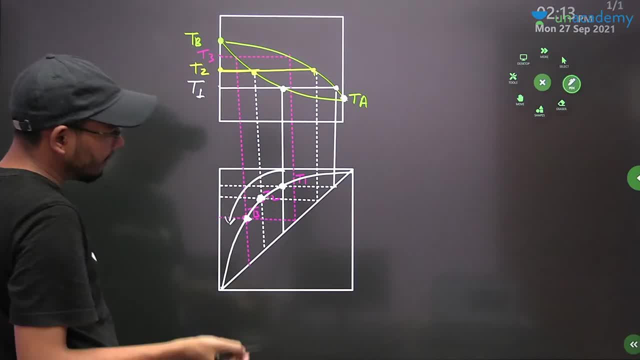 will happen to you. you will see: this is T3 temperature, this is T2, this is T1 temperature. ok, this was T1, this was T2, this was T3,. you will write properly: this is the equilibrium. 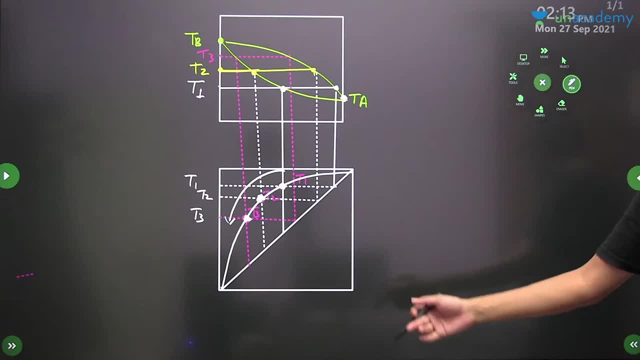 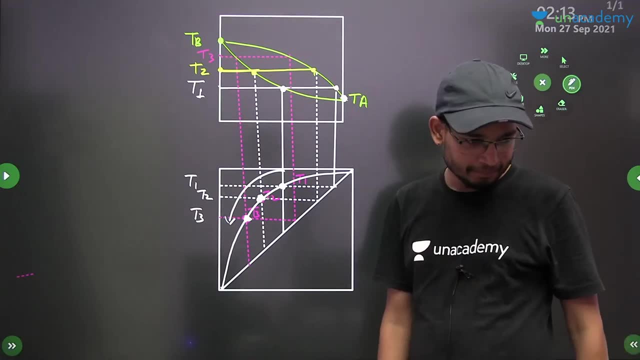 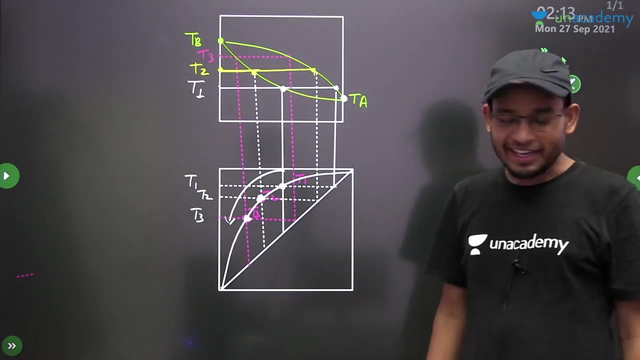 curve. you will understand it very well. this is a very qualitative representation. it is not so easy to make it. Then you will have a very good practice. then only you will be able to make it right. otherwise it does not make it right. tell me, I do not know which one to mix, then there will be. 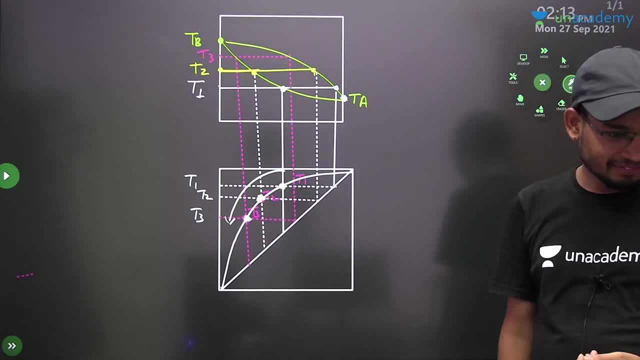 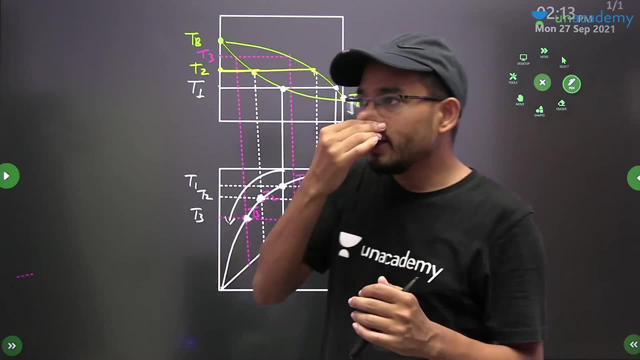 very good concepts, then only you will be able to make it. ok, then make it very well. one or two people taught me on plus, so people know what they have done, which is their graph paper and excel. one child made it on graph paper, one child made it on excel and sent. 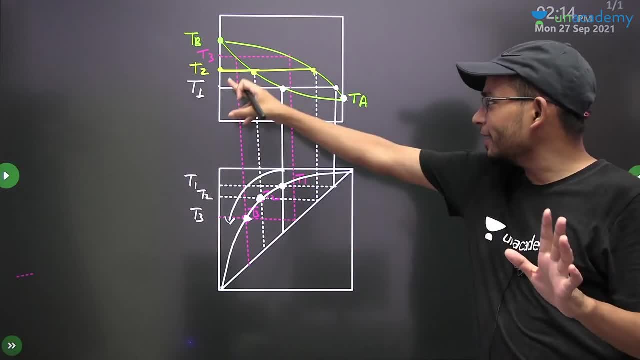 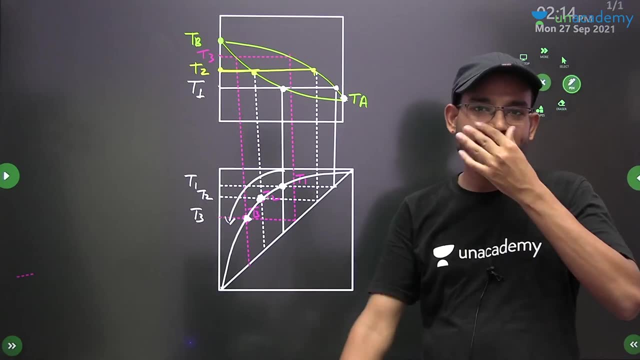 it to me. Take all these points properly on excel. Ok, So it was a question of designing. he did it properly. first it was a question of three to four pages only, which used to come in your btech. ok, he took the temperature properly. 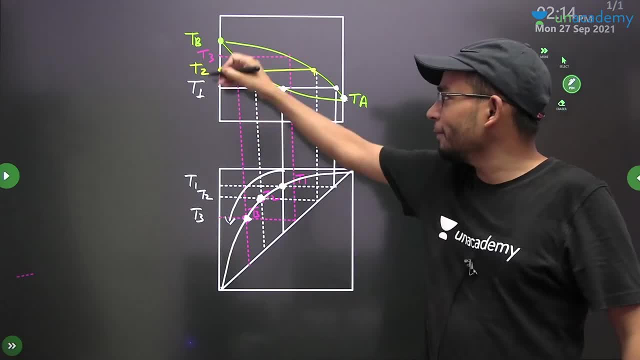 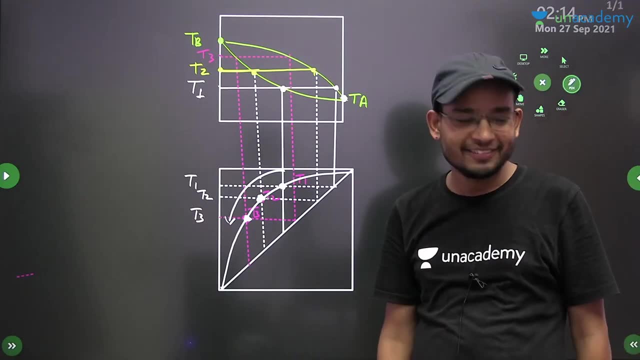 between them and took the point properly and made it on excel. ok, I put his work on the group too. you must have seen it on your group. I put it on the whole group. some people must have seen it, must have enjoyed it. so this is very interesting. I have put it on the. 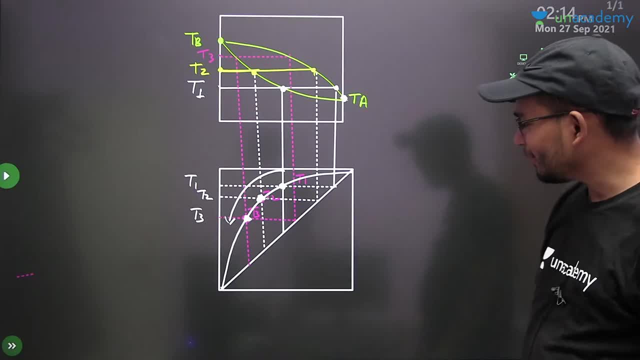 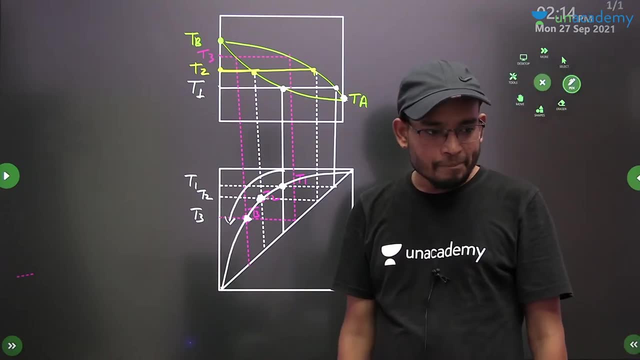 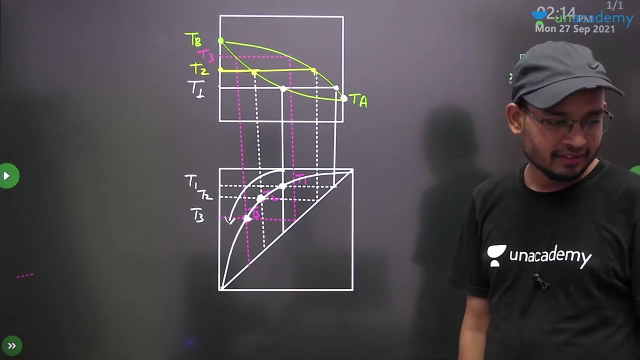 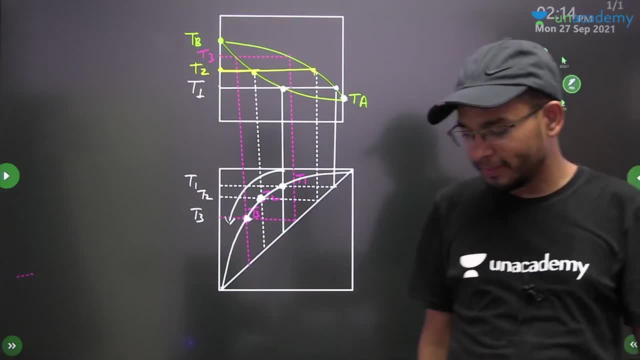 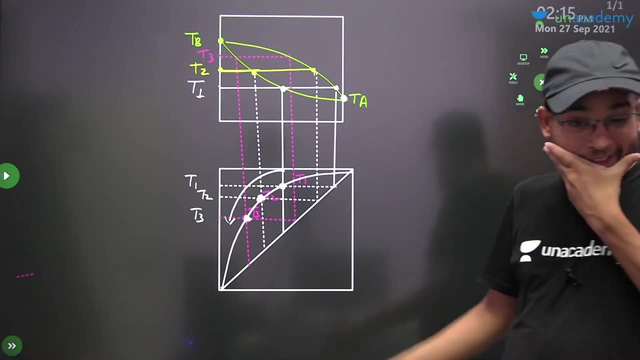 curve. see, this means if you want to get a real feeling, then you have to make it like this. see, understand the second method of this. yes, Very good, Very well. he knew. he made it and sent it. he knew very well. 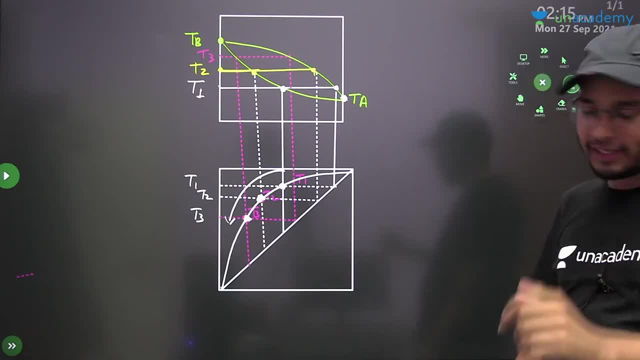 Ok, Yes, I put it on the group. Very good, This is done. Now look at its second method and third method. Just understand, like this And its method. This method one has come to everyone's understanding. This is the method one To draw. This is the actual method. This is an interesting 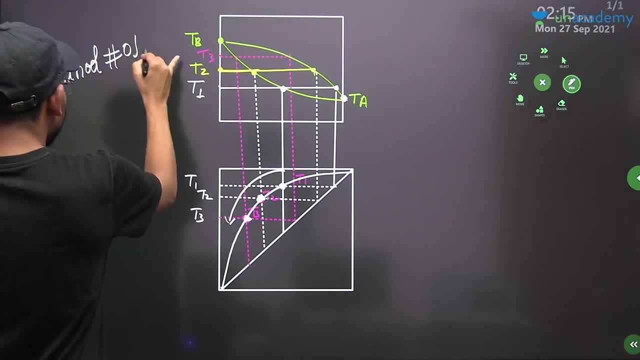 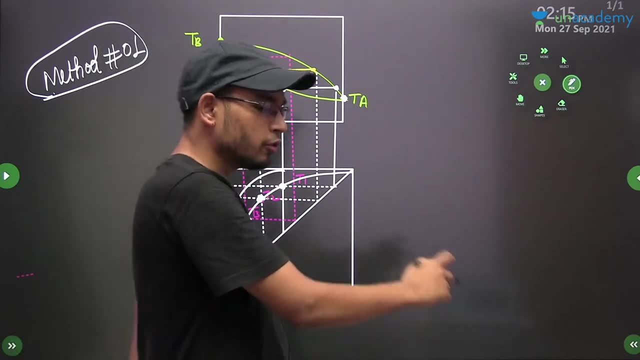 thing. Method one: Okay, This is the first method. This is the first method. What is the second way to represent it? Understand that Done. You have made it. All the points have come to everyone's understanding. How did you draw? This point has come to everyone's understanding. Come on this. 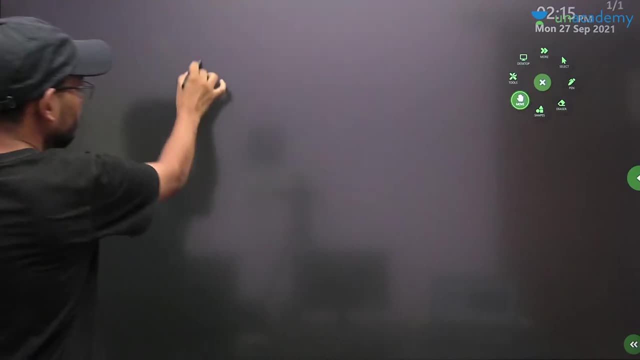 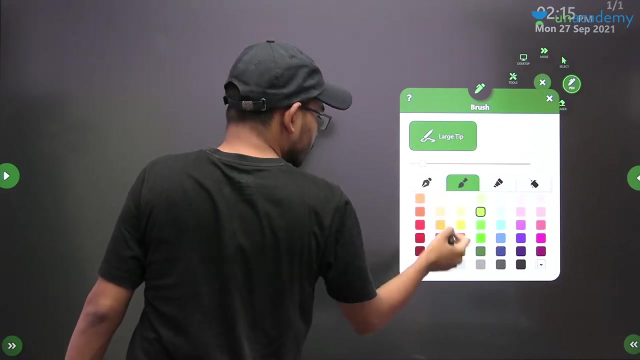 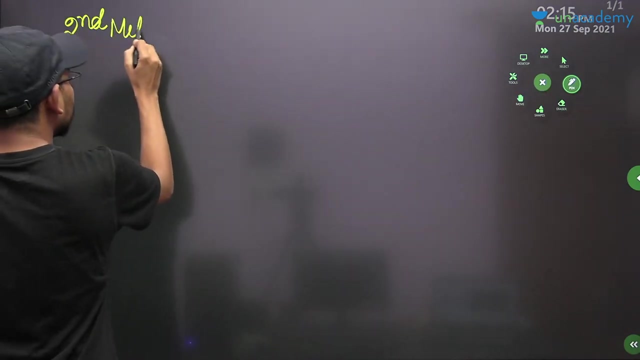 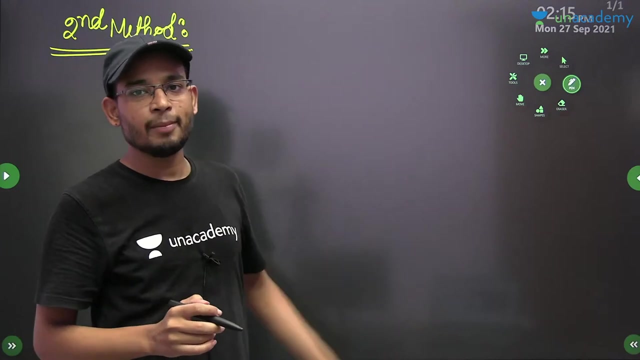 point. This point is important. Come on now. understand the second method. What is the second method? Look at its second method. Understand everything. well, Second method: Now, the ultimate thing has to reach the reflux ratio, And to reach the reflux ratio you will have to go through all these actions. 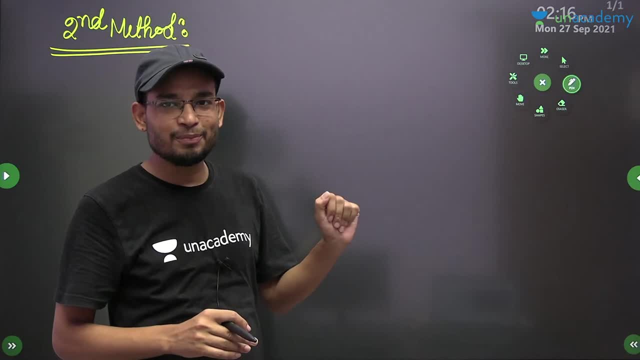 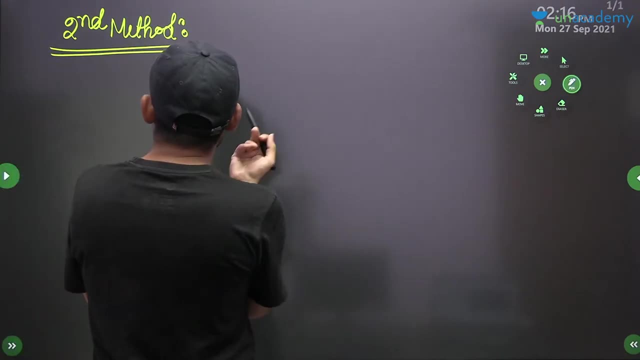 Okay, Who has to talk Of reflux ratio? So all these things will have to go through all these steps. Okay, Then you will get the reflux ratio. You will not get it like this In designing. you have to do all this. 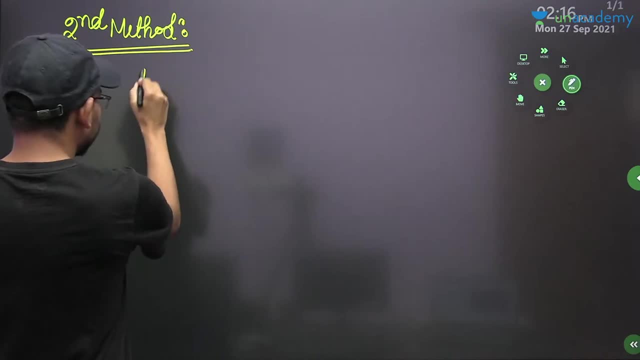 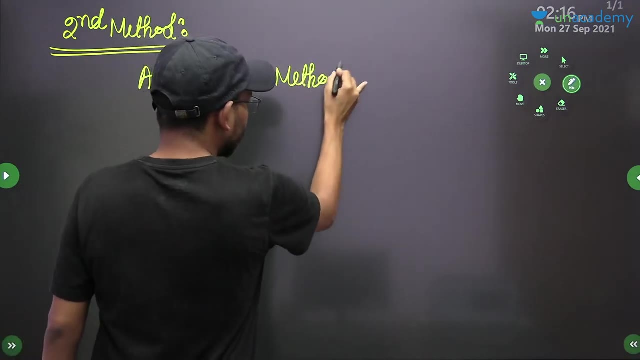 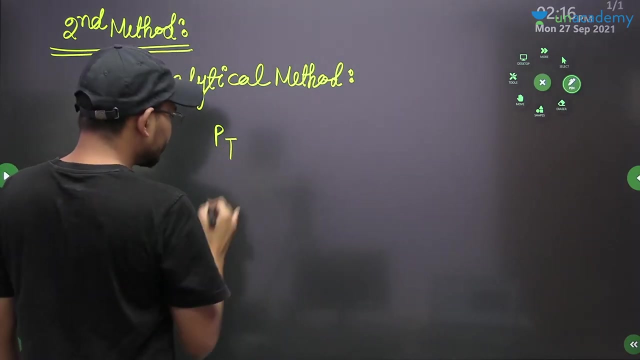 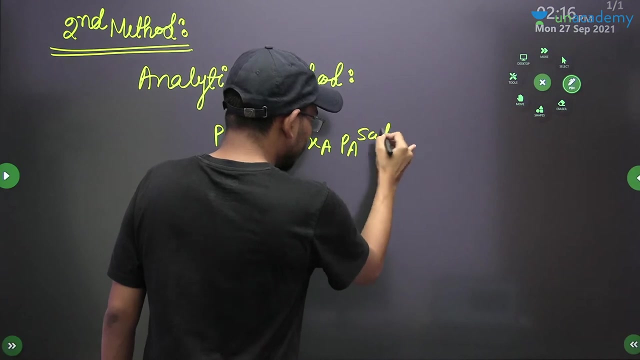 Now, what is the second method? Analytical method, Analytical method, Analytical method. What is the analytical method? Everyone understand very carefully. Everyone understand the concept. What is our p total? Let's see a little closer. let me tell you a little more closely. This is our p total. 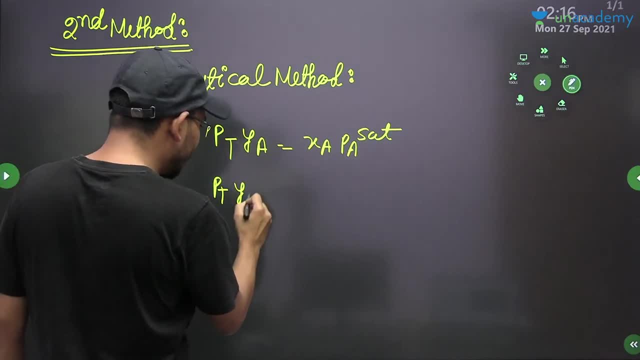 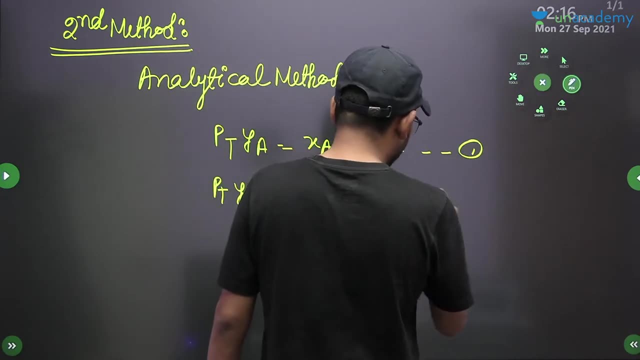 Right, This is 20,000 here. Let's see 30,000 here. okay, 134 plus 25.. We have so many Xs. This is R Soul, isn't this Okay? It would have entered the same. 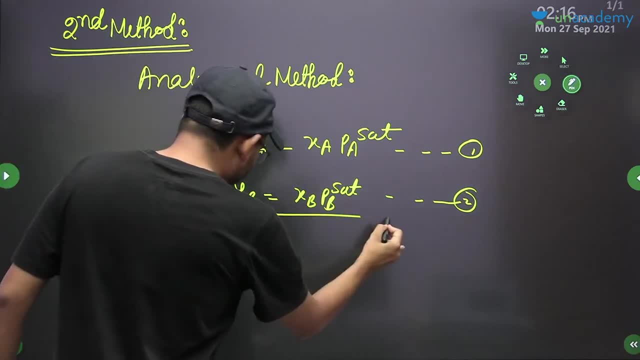 number than before, so that one can also go over that. Okay, Where are they? Okay, 가지 bitte kal мне. or do one more. Wait, Please wait. Will you wait? Please wait. If you do it one, then you can see when to. 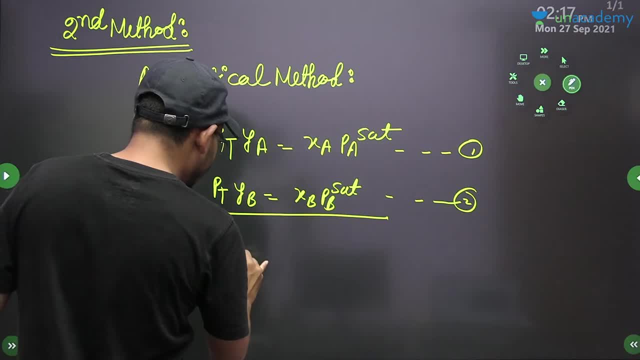 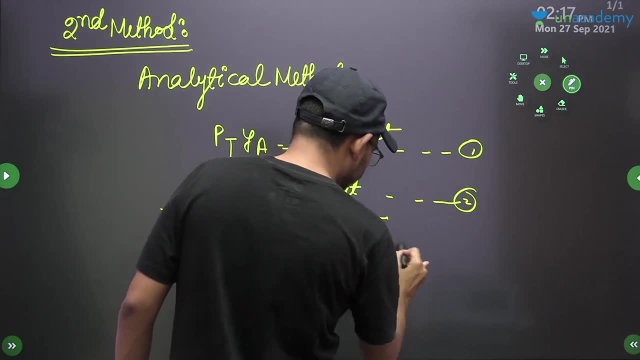 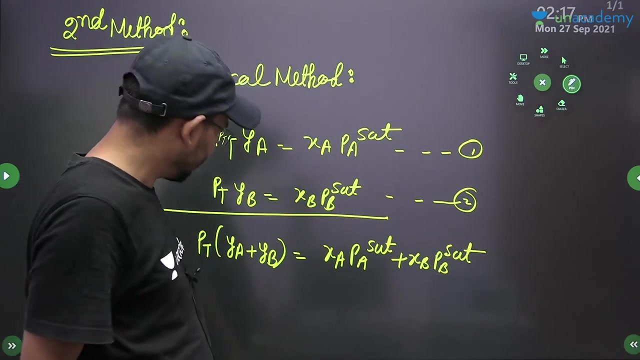 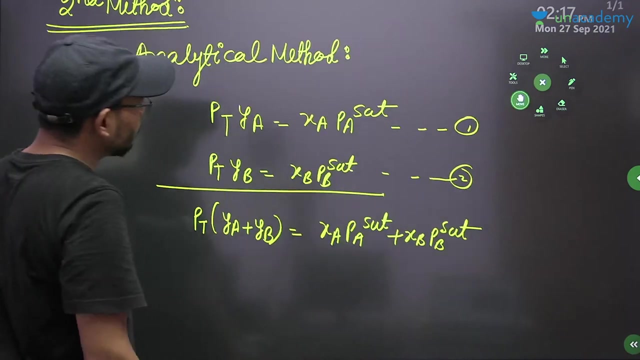 this second perofi, then you can also tying then this secondello kalu록 to that one. So say: here you will have ya plus yb, and here you will have xa pa set plus xb pb set. you understand now what is ya plus yb? it is 1, so how much is p total? understand this carefully, i will. 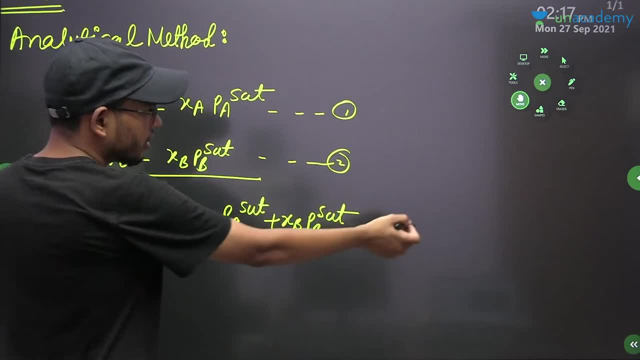 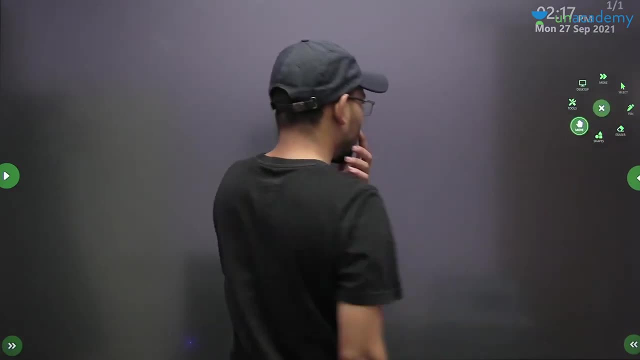 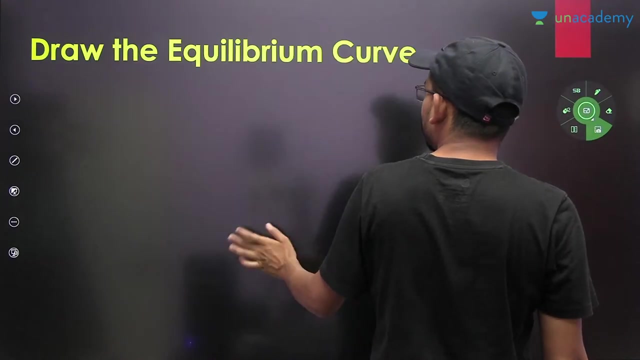 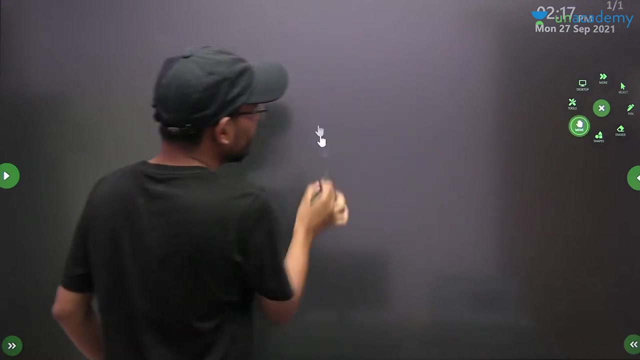 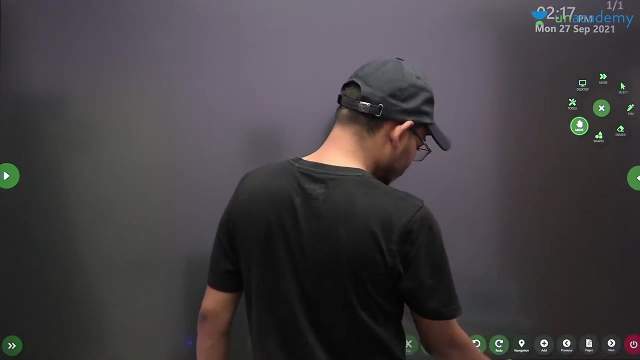 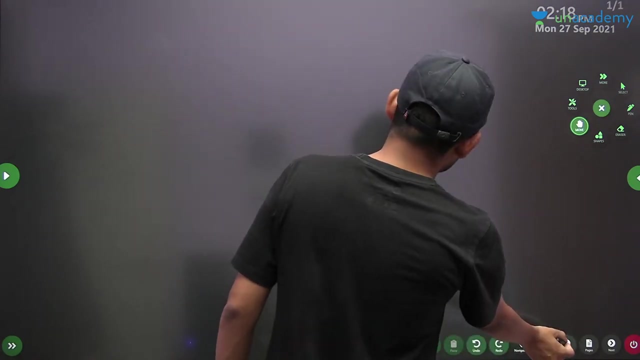 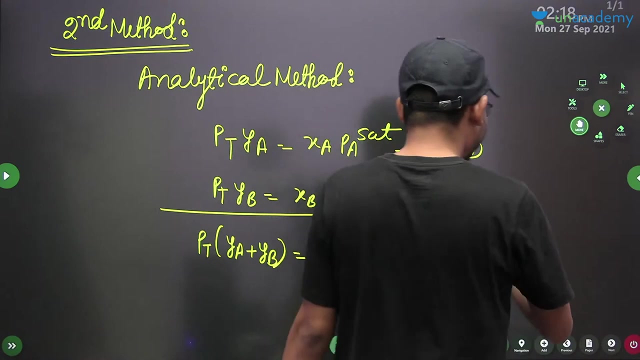 do it from the side. i will do it from here. also. i will use it where it went. did it get erased? one minute? it will come here. one minute. it came here. okay, i thought i will have to write it again. fine, understand this much. so how much is? 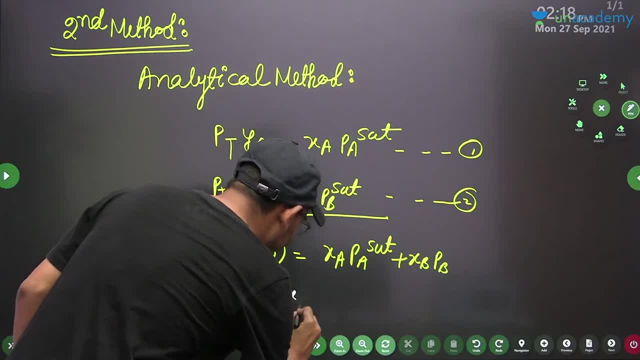 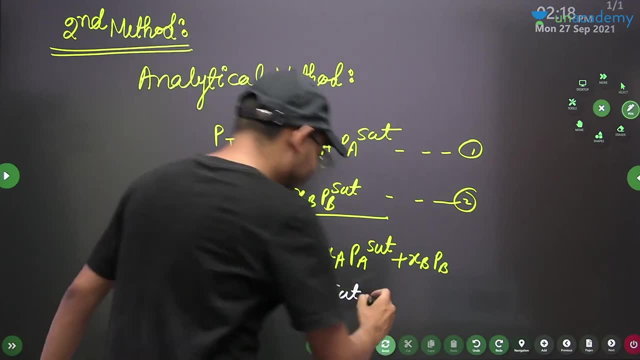 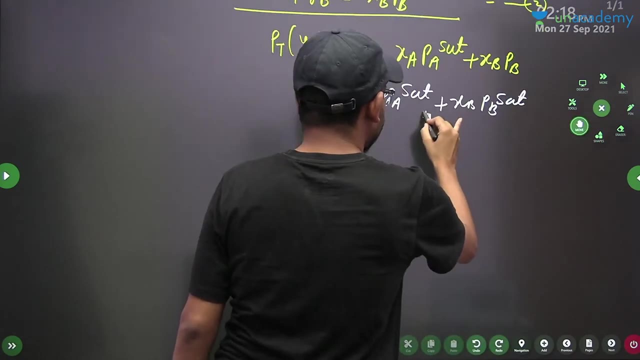 p total equal to 2? p total equal to 2 is xa pa set. sometimes technical things are not easy in many things and sometimes they irritate too. plus xb pb set. now it is very fast. on the first day it was going very slow, okay, so now to make it rough. the biggest problem: 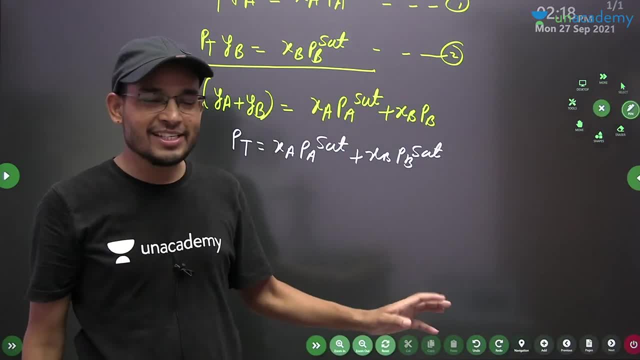 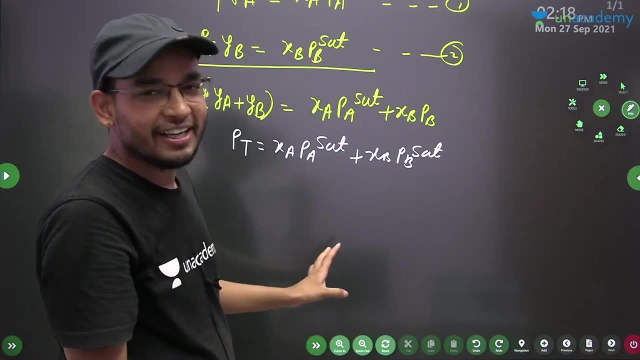 used to happen, so i used to teach offline to make it rough. i used to think like this: i will hire a candidate and tell him that, brother, you have to do like this whenever i write it. then you have to make it rough. this is the worst situation in the board to 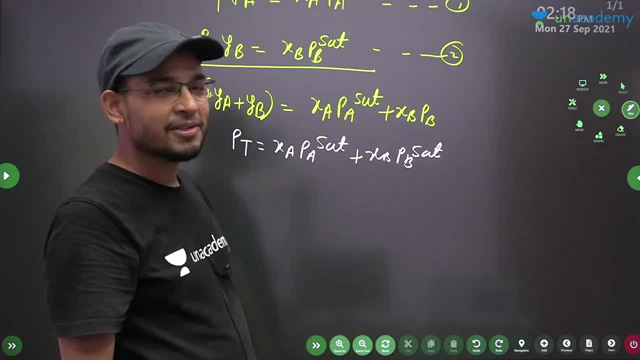 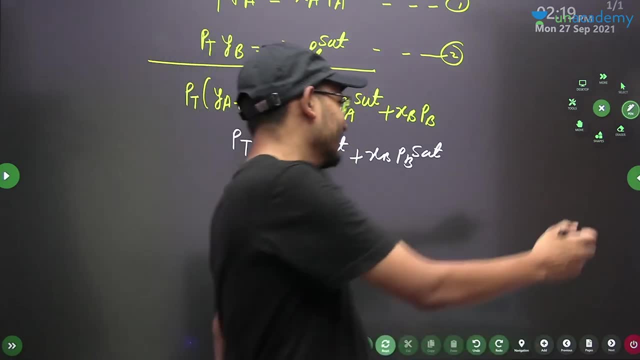 make it rough. okay, since then this board is like this. see, since then this board came. since then i said: no matter how much anything happens, you must have seen that earlier our board was there. we invested, we said: do it, brother, this board should be there. okay, i got to know that half of the energy is going. 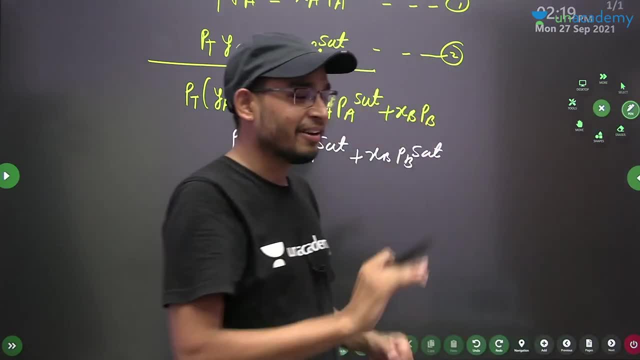 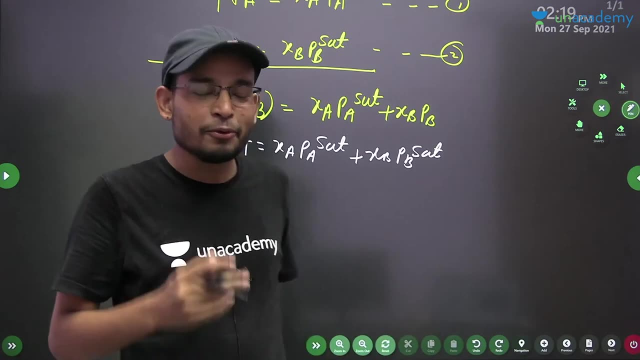 into that. only half of the energy is going into making it rough. now i got to know that one was our lazy teacher. let me tell you, one was our lazy teacher. he didn't want to make it rough at all now. he had to teach them something new. 3 okay. 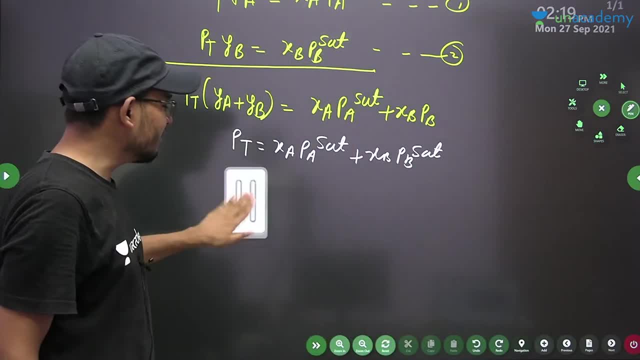 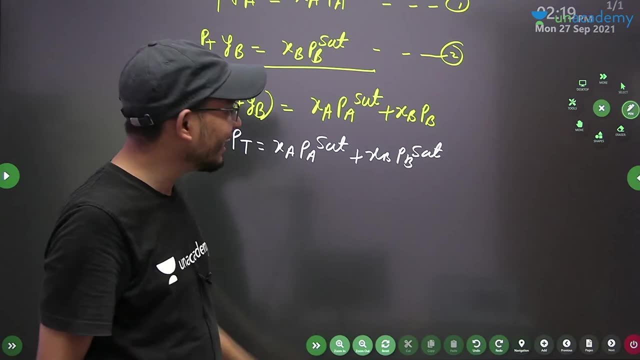 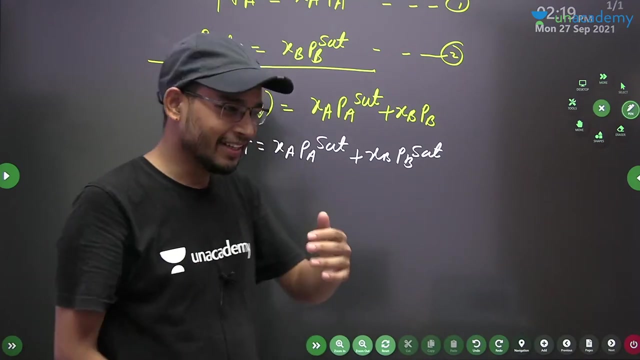 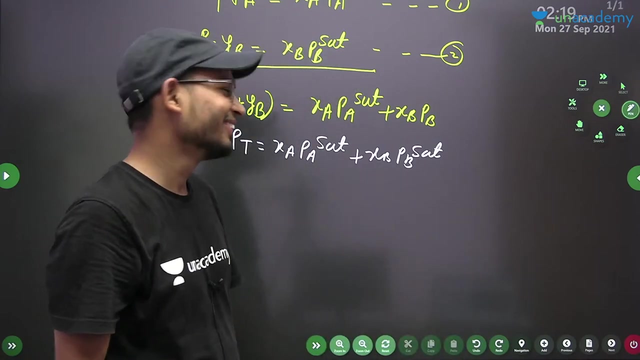 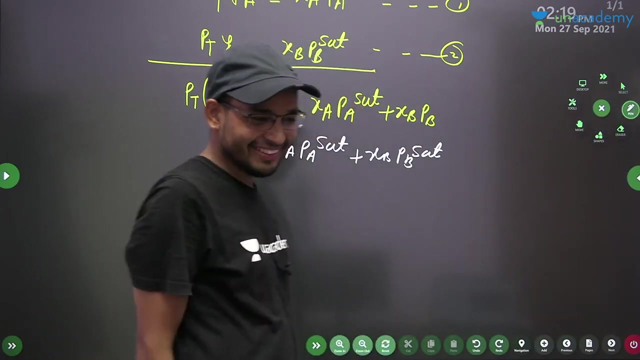 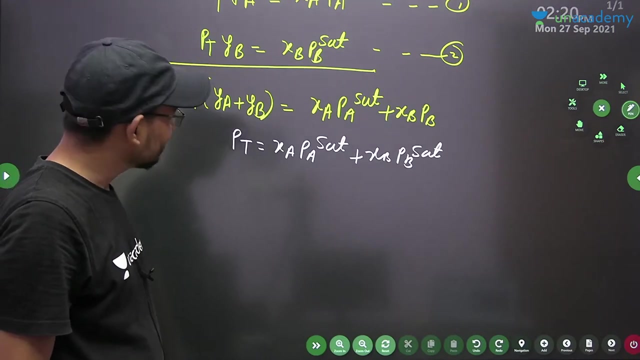 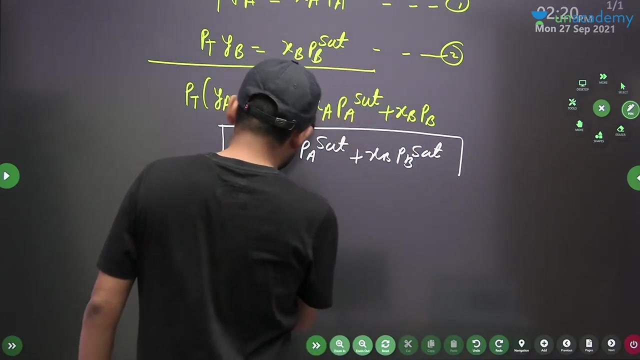 2, 3, 2, 2, 2, 2, otherwise he was going to show the board. he was going to show the board in 2: 7. So this is what we got. we understood that Pt has reached here. Let's understand the analytical method: how to draw a graph. 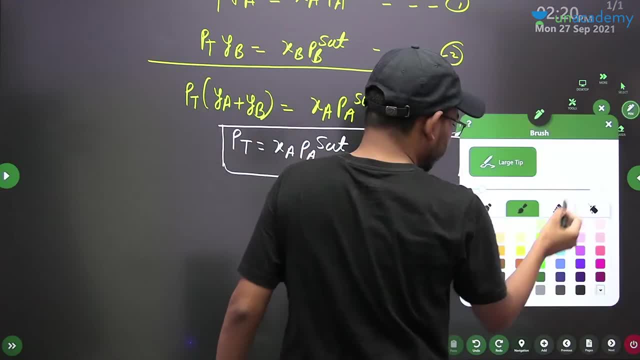 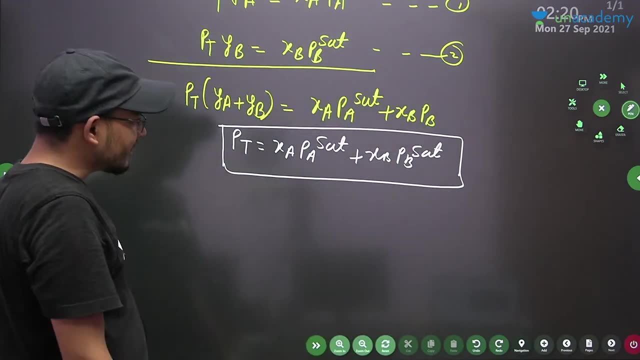 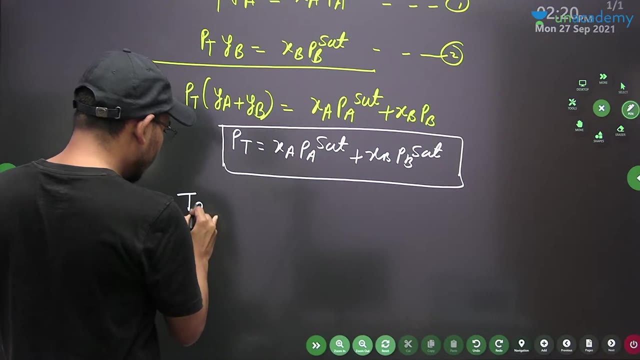 Pt has reached here. now look very carefully. Now I will choose a temperature in between, because we know Ta and Tb. Ta and Tb are boiling points of a pure component. Suppose this is 400 and this is 200 and this Tb is 400. 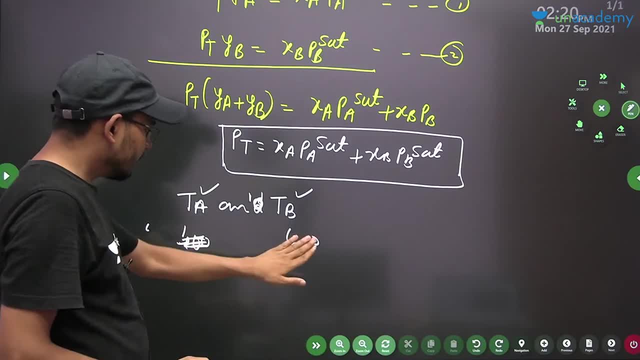 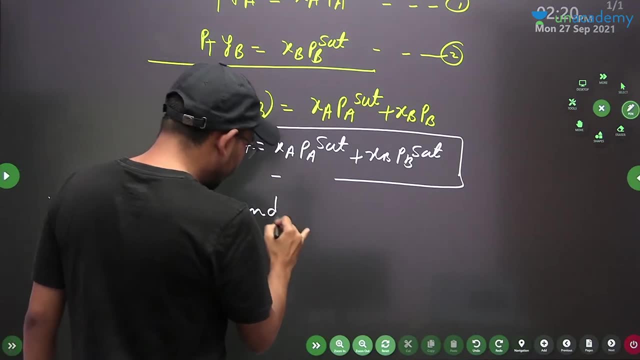 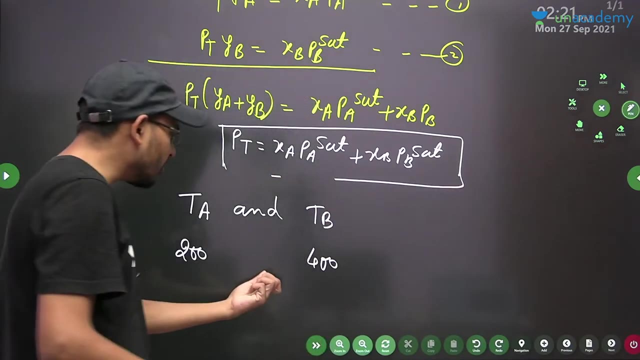 Tb is 400. and how much is Ta? Wait a minute, How much is Ta? Listen, this is Ta and Tb. This is less volatile, so its boiling point is 200 and this is 400.. Now I have chosen an intermediate temperature. 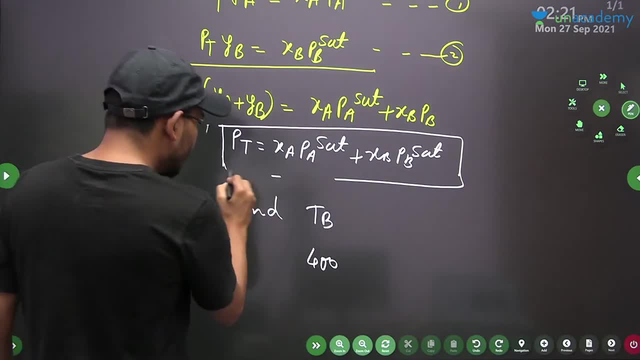 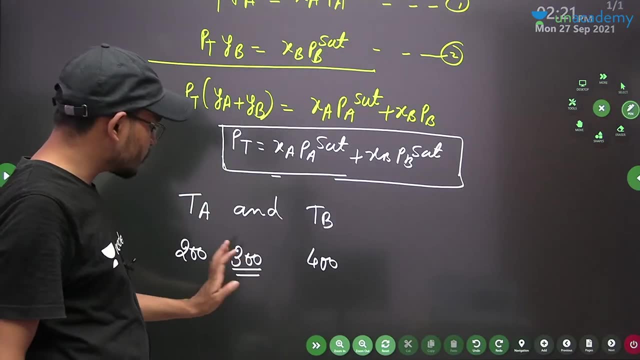 You have to choose it from your mind. Whenever you have put such questions in BTEC, you must have chosen it from your mind. Suppose I have chosen a temperature of 300.. Now, at this temperature, will we get Pa and Pb set? 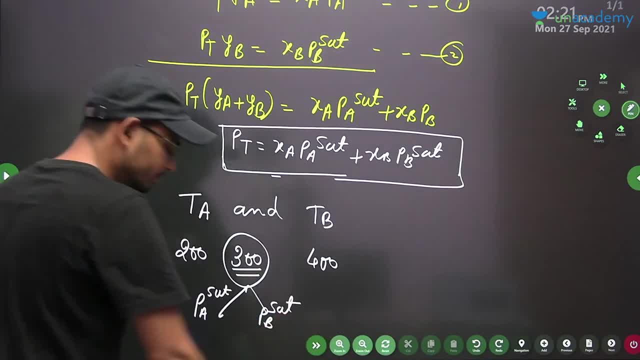 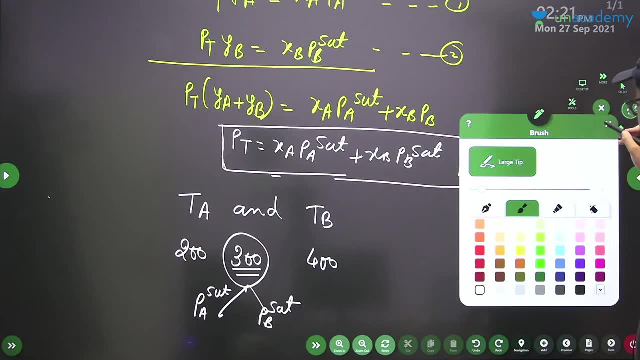 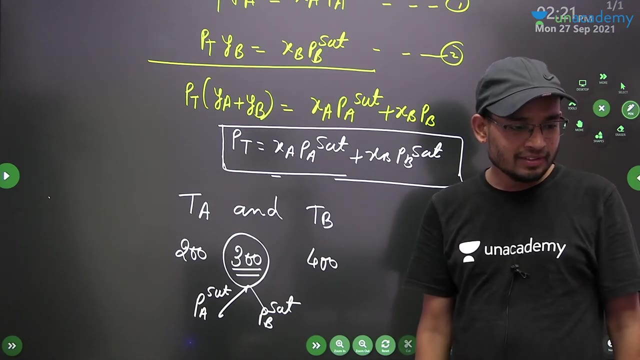 Everyone will get Pa and Pb set. Everyone. At this temperature, everyone will get Pa and Pb set easily. There will be no problem. There can be no problem in this. Say yes or no, Everyone will get Pa and Pb set, Yes or no. 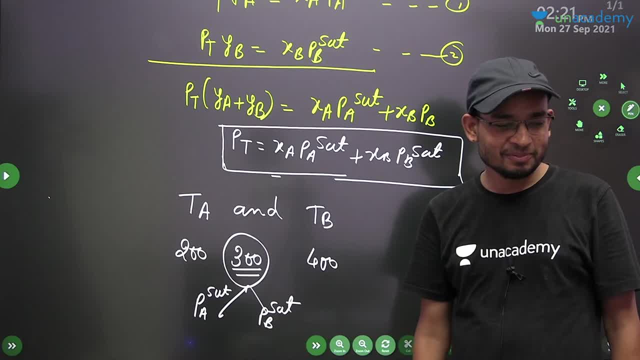 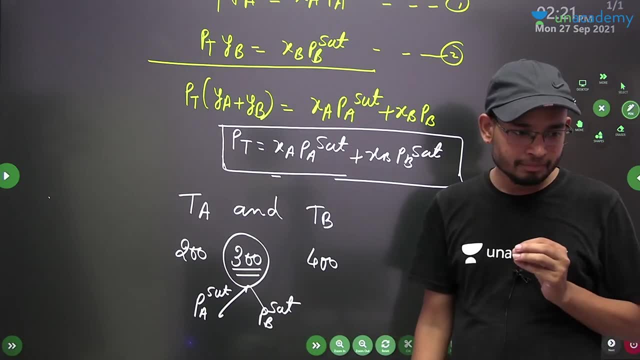 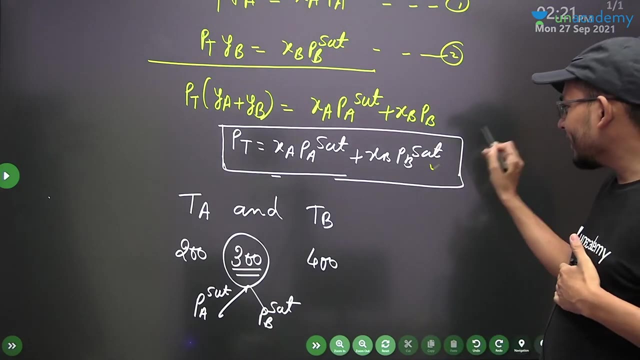 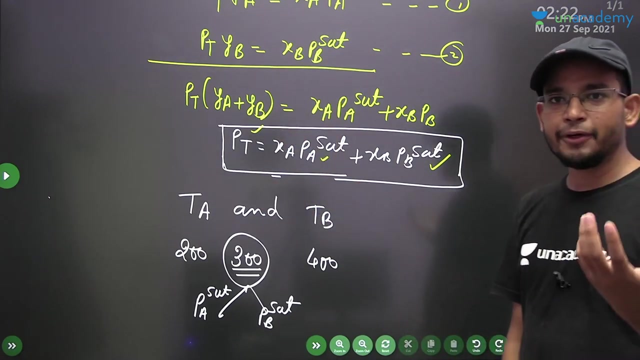 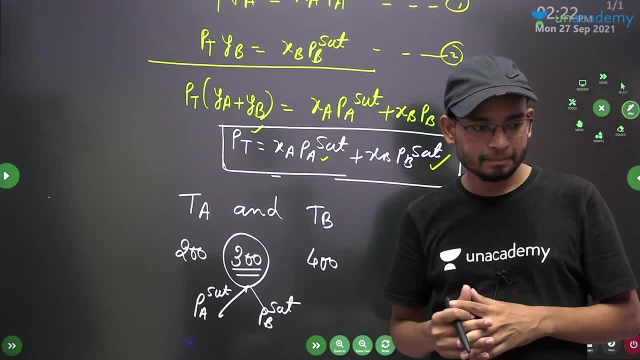 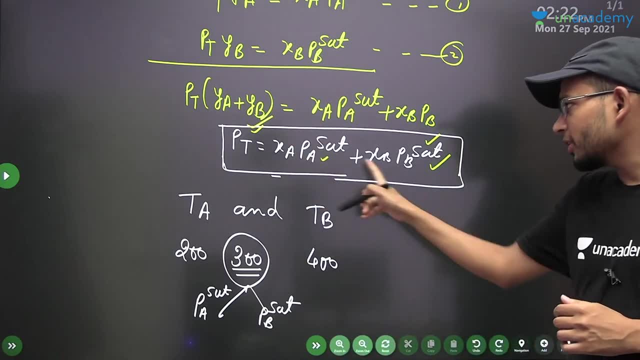 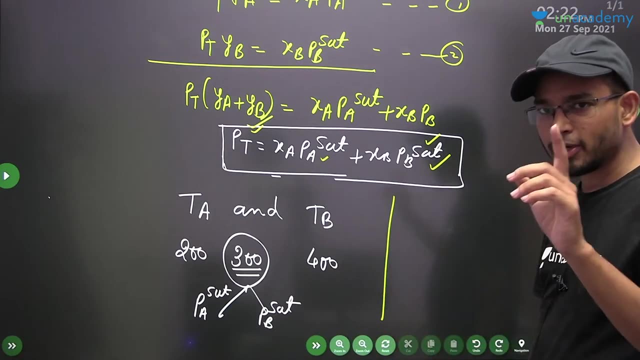 Everyone will get Pa and Pb set. This is the end. You already know the total P. You have taken Pt constant of the entire system to plot Txy diagram. You know Pt total. how will we write xa? we will write 1 minus xa. 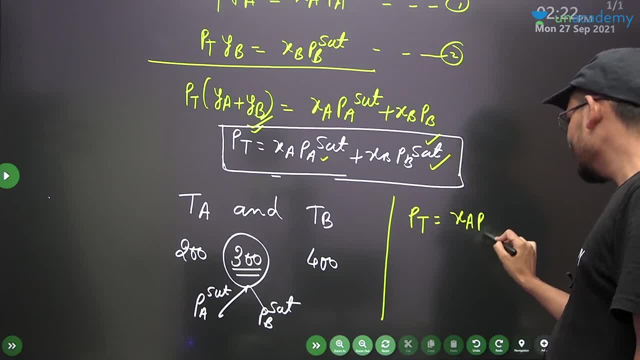 p total is equal to xa pa set plus 1 minus xa pv set. we can write like this: because in binary system xa plus xv will be 1, so tell me, will xa reach here? p total you know, pa set you know. 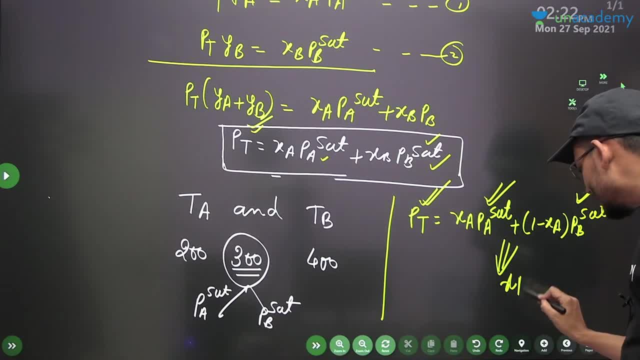 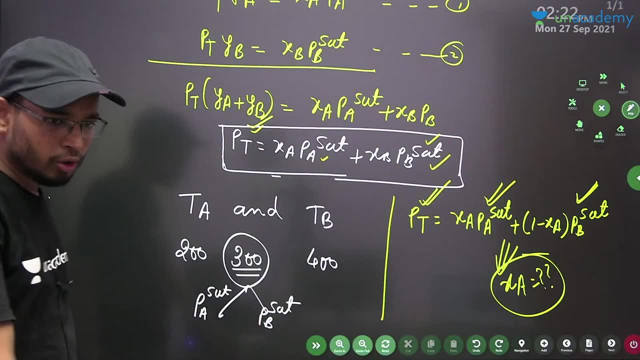 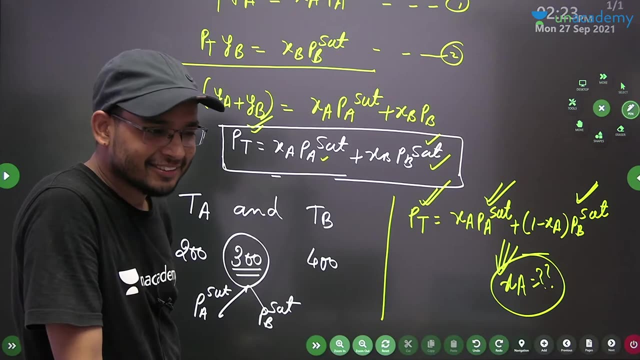 pv set. you know, everyone will be able to write xa. yes or no? yes or no, tell me, nupur. yes, I have made you do all this, ok, yes, very good, will xa come now? tell me if we put xa in the first line. 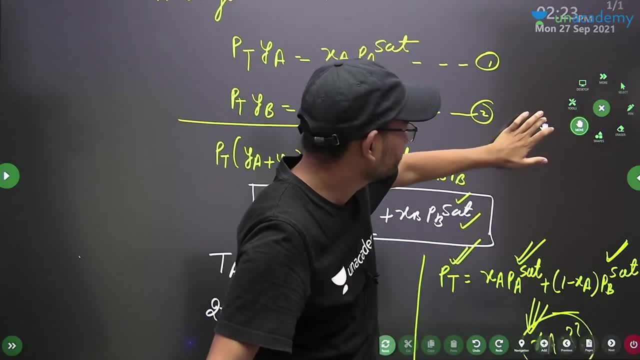 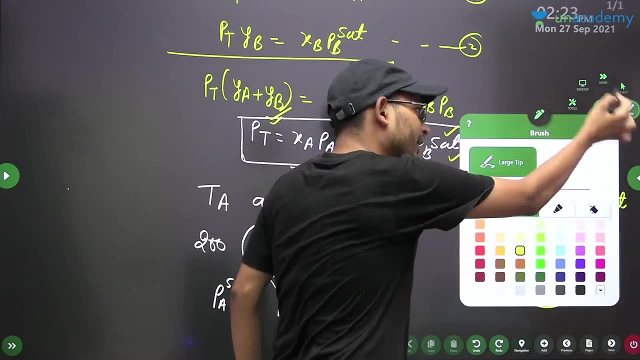 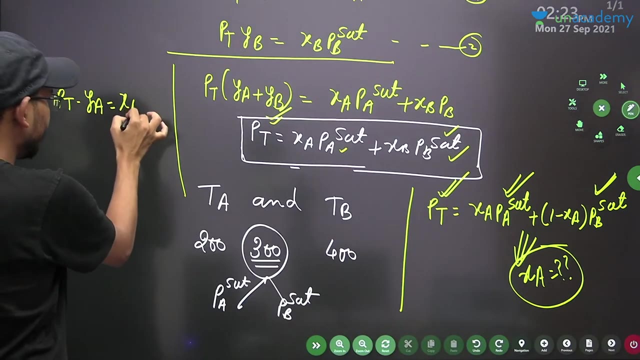 then will ya come or not. tell me, will xa come here? we will keep it here. ok, I will write it. if you put xa in the first line, then will ya come or not? p total into ya is equal to xa pa set. so xa you know, pa set you know. 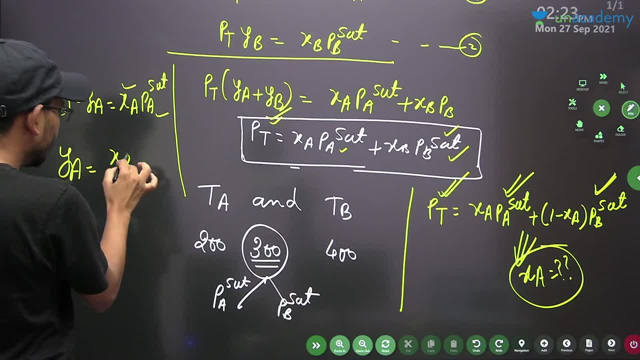 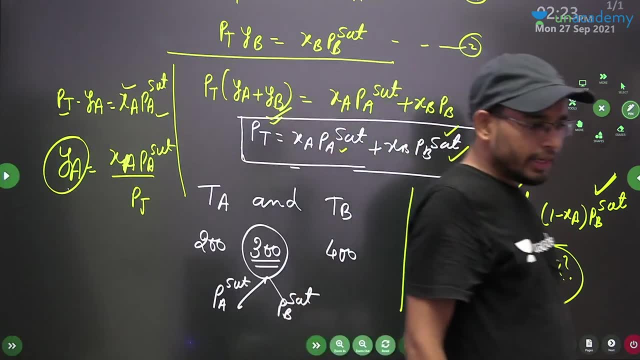 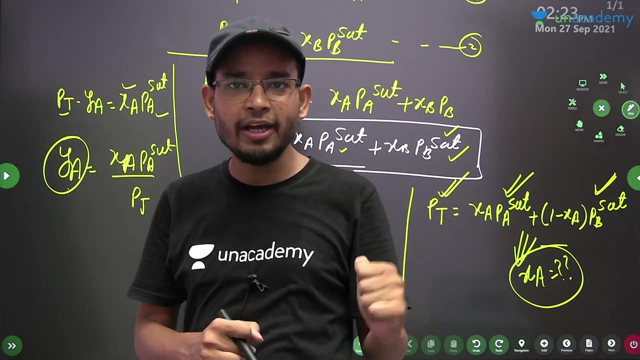 p total. you know, so won't ya come. xa pa set upon curve p total, so tell me, will ya come or not? you just need this xa ya. xa ya will come and you know the different temperature. you will plot txy and also xy diagram. 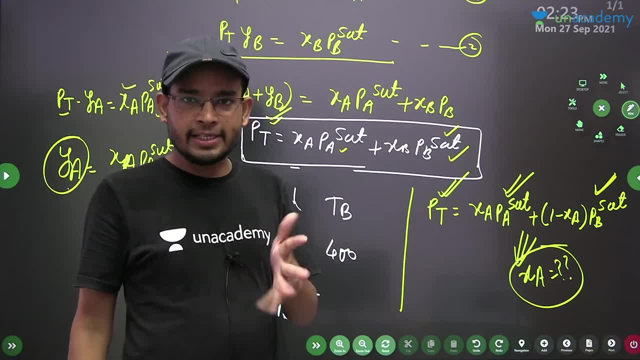 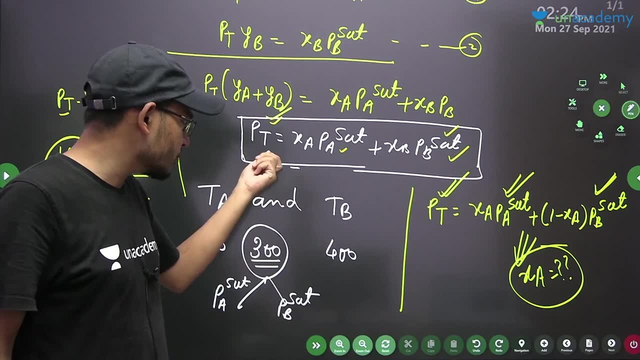 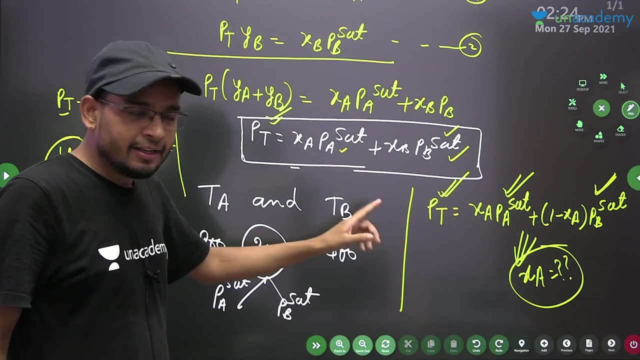 yes or no? xa ya, xa, ya also know. then you will plot txy diagram because you have one temperature. so you got txy diagram. you will choose an intermediate temperature, then you will get xy diagram, then you will get point, the number of temperature you choose between this. 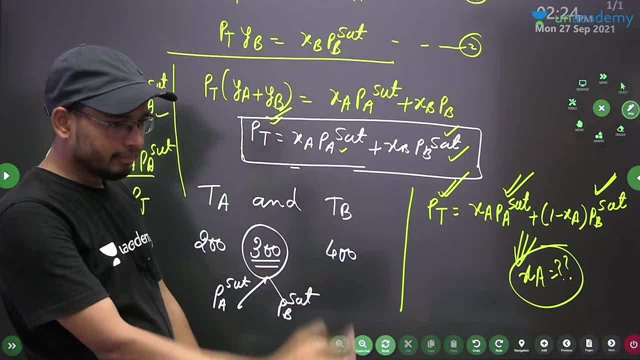 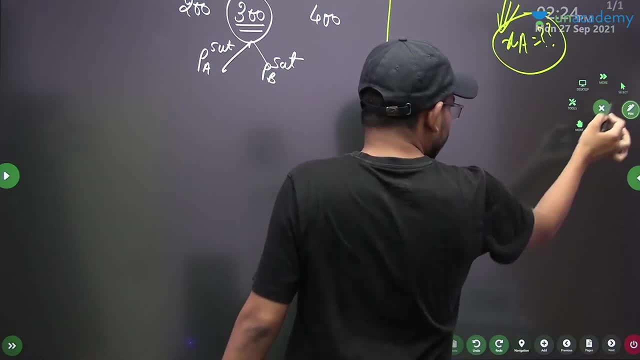 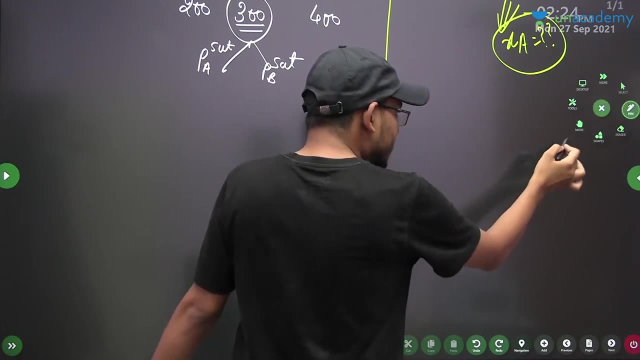 you will get a point, okay, so in this way, you will plot, I will make a sheet of it. I will make a sheet of it in a beautiful way. understand all people. these things are very useful, very useful. after studying, you will be able to collect these things so easily, which we are talking about. 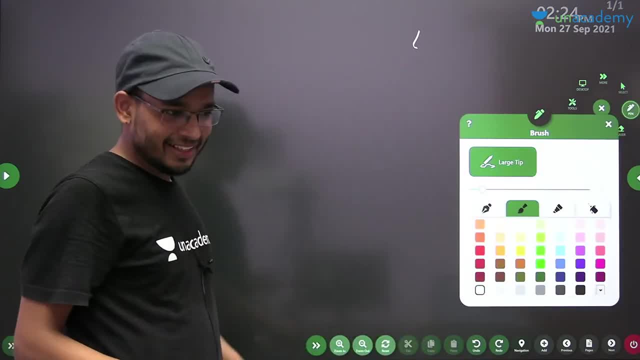 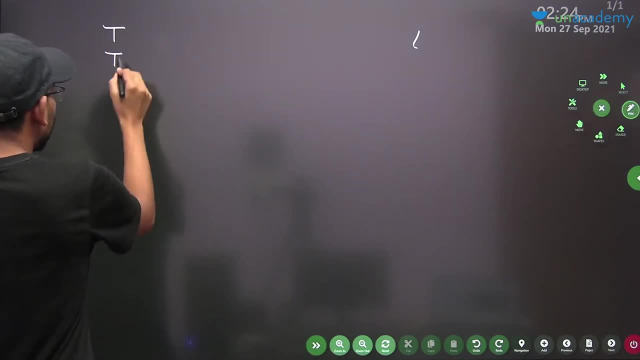 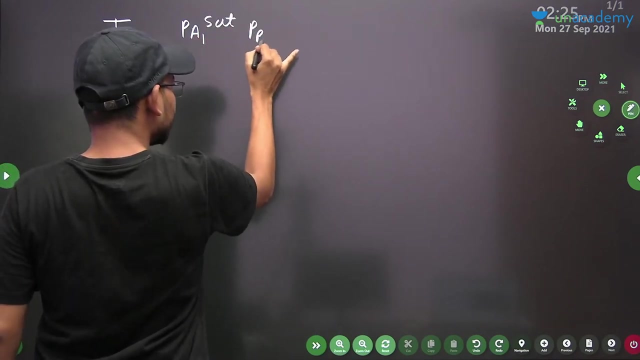 things are not so easy in the beginning. see, if you do a lot of work, then these things will be very concrete, clear. so what do we know? we have chosen a temperature- t1- one temperature. you have chosen t1- one temperature. you have chosen t1 on t1. what you got? pva1 set and pv1 set. so from here you got. 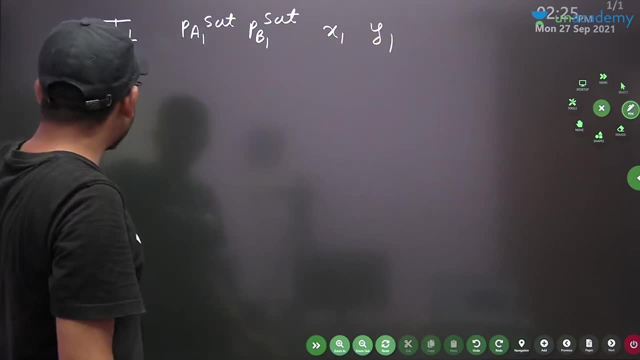 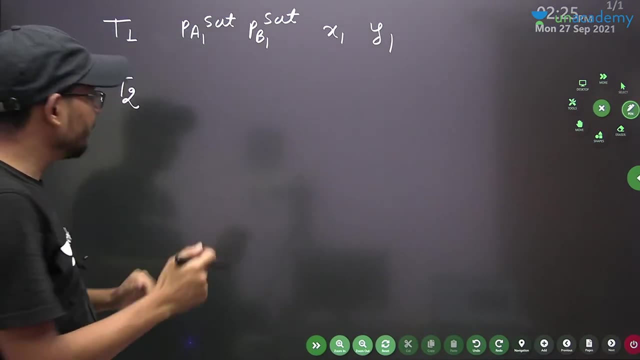 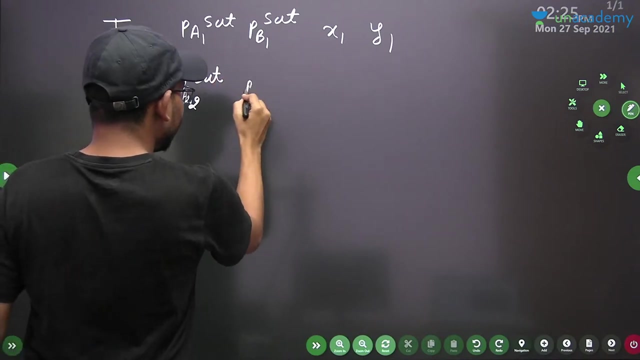 x1 comma, y1. one point. then you have chosen an intermediate temperature, t2, which is the temperature between them. okay, it will boil on it. so you will put the temperature of the beach again in the equation. so you will get p2 set. from here you will get pb2 set. from here you will get x2. from here you will get y2. 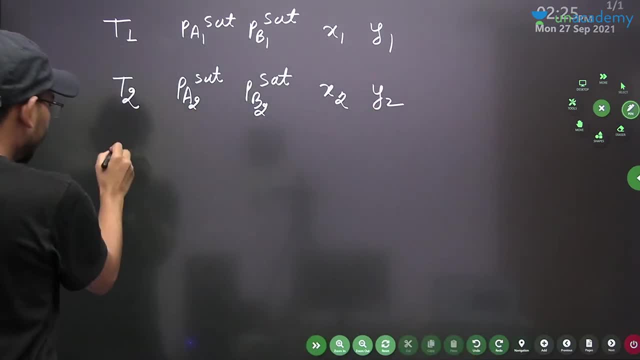 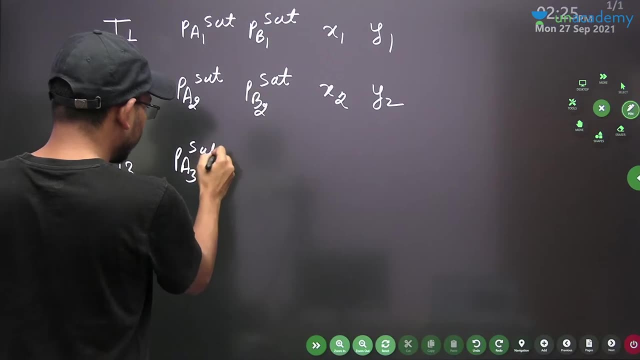 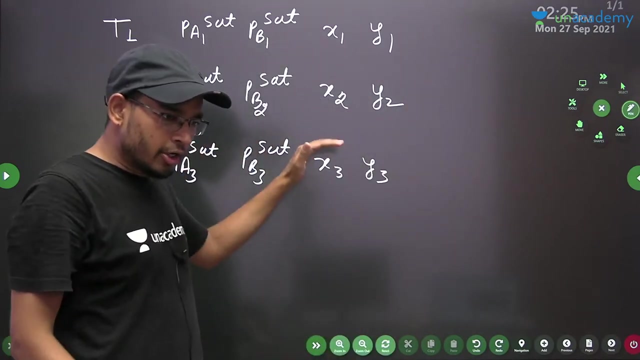 similarly, you have again, again, t3. as I have also told, the procedure you have to follow the same. so you will get p83 set, you will get pb3 set and from here you will get x3, y3. see whatever points you have to find. 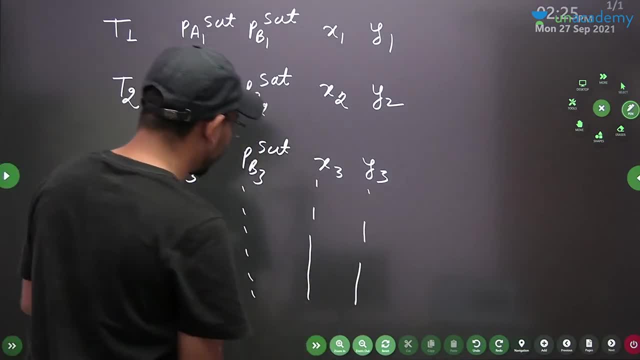 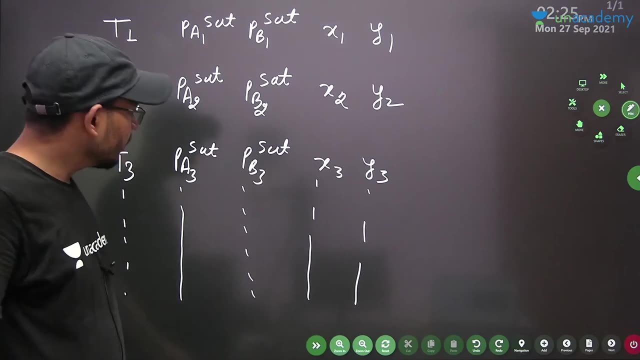 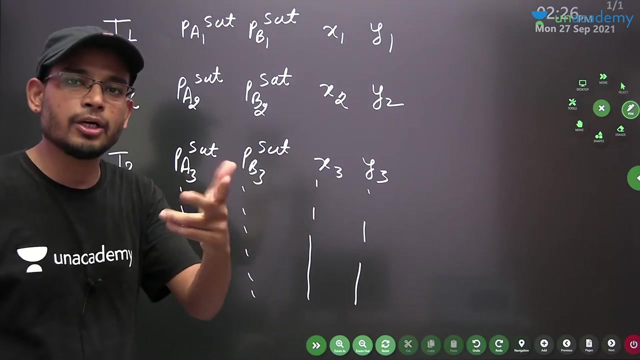 whatever points you want, the more accurate you are able to plot the graph, the more accurate you put the plotter, the more points you have. with so much accuracy, your graph will be played right. so this was yours. you will also plot the tx- y diagram and from here you will also plot the xy diagram. this was method number two. 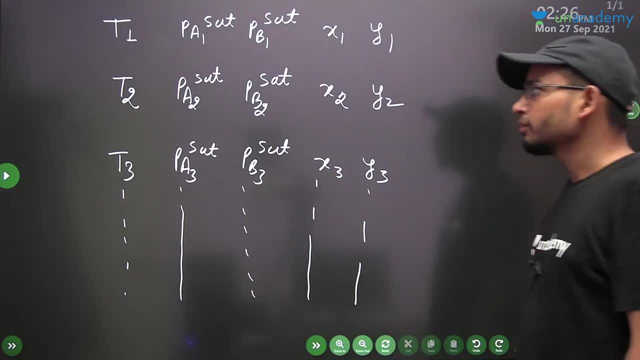 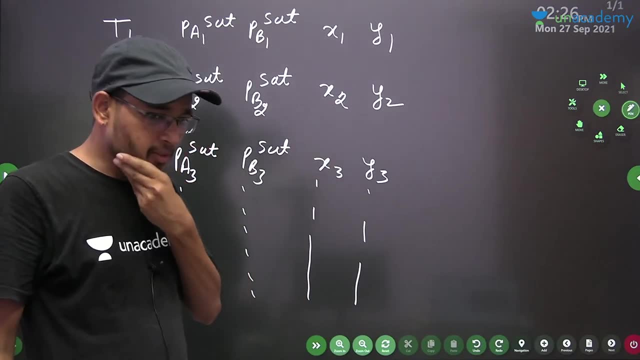 did you understand? this was method number 2, 2, deter 2.. method number two: to determine like this, This method. This was method number two To this method: draw the equilibrium curve. did you understand, yes or no? 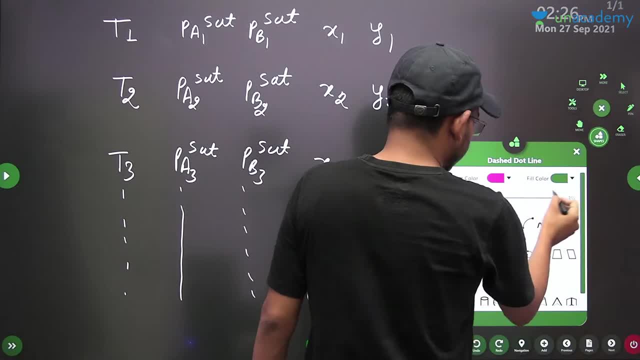 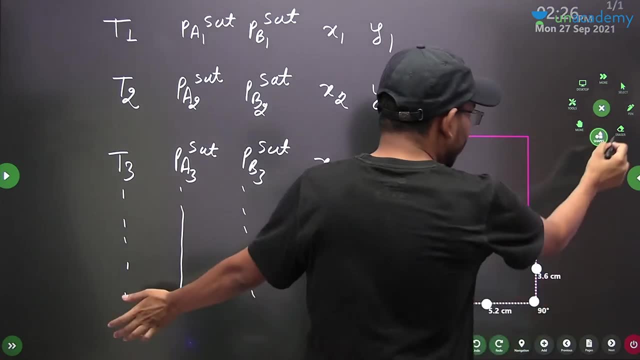 if you have this data, then you can plot it with a smile. if you have this data, then you can plot the xy diagram, and if someone asks you to plot the txy diagram, then you can plot it. you have the point there. this is the analytical method. 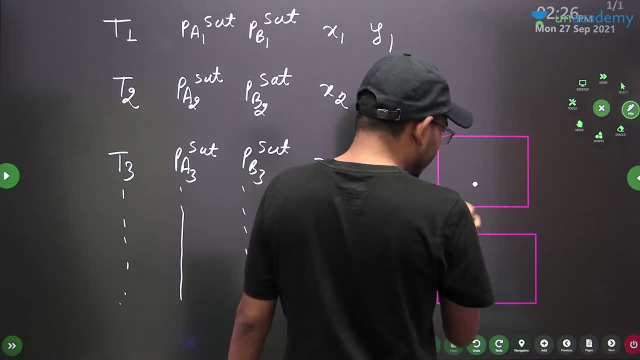 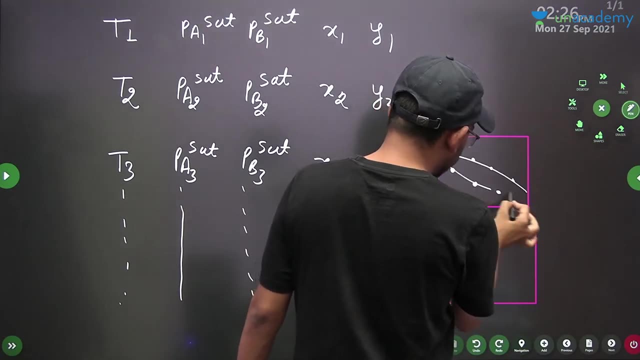 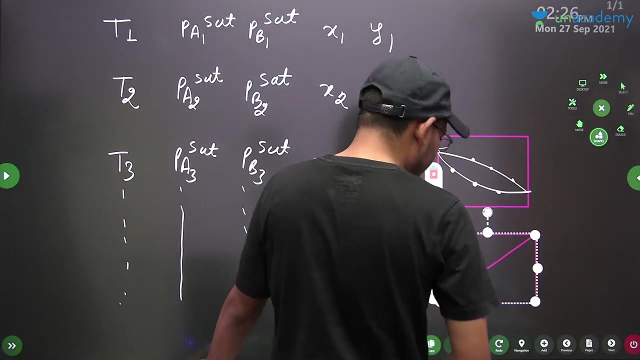 you know the temperature: x and y. this is the point. you will get t versus y, t versus y, t versus y, t versus x. this will be your plot. similarly, you know the diagonal line. you will know this: 45 degree without thinking. 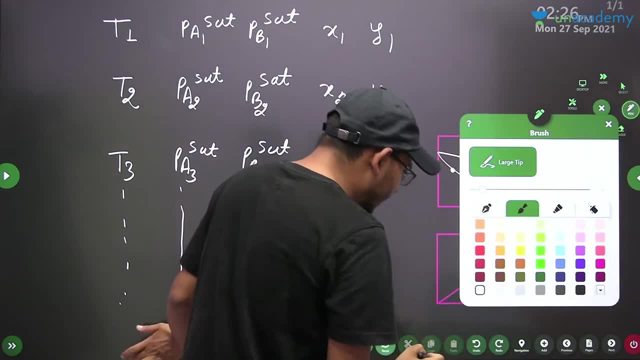 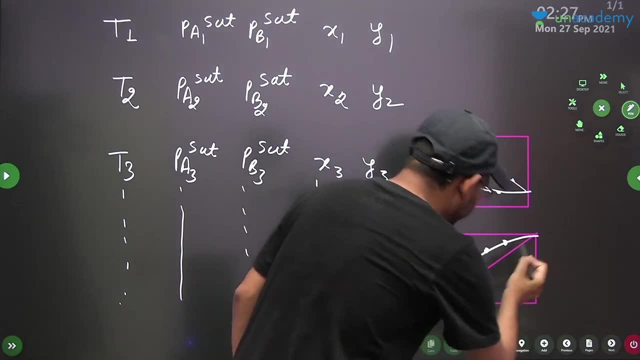 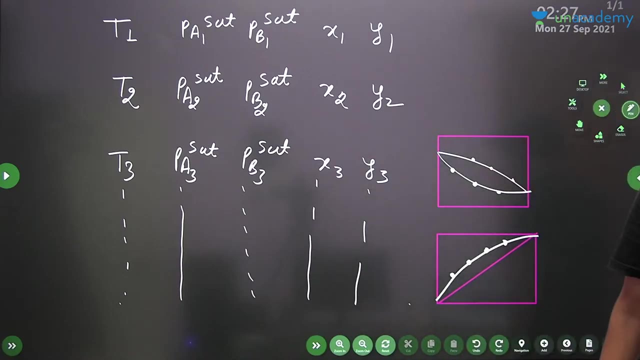 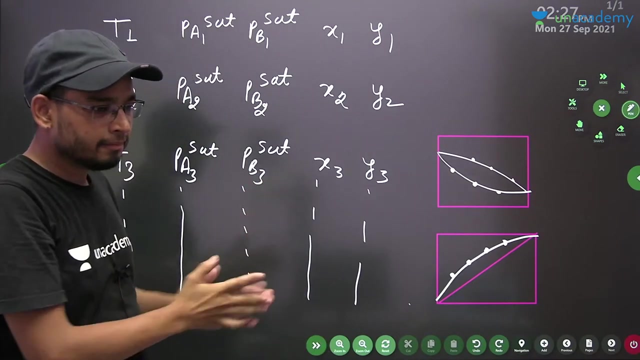 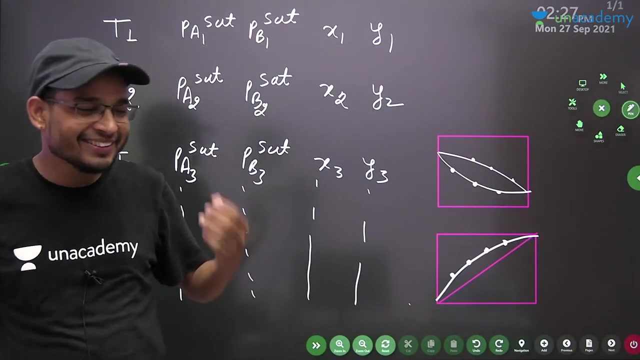 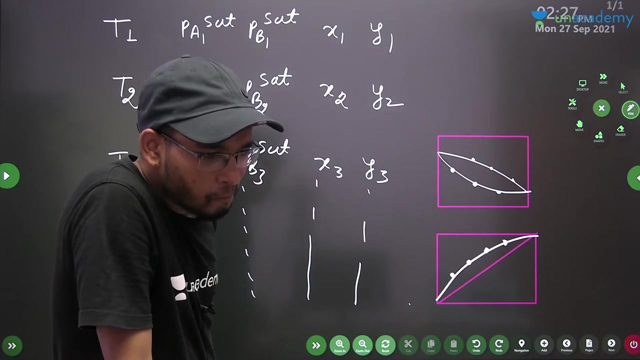 and you know x and y, you know x and y, you know x, y, x, y. you will know this at a particular temperature. you will get this and this. you will get this and that. next we are going to discuss the AUTOMATICUS. 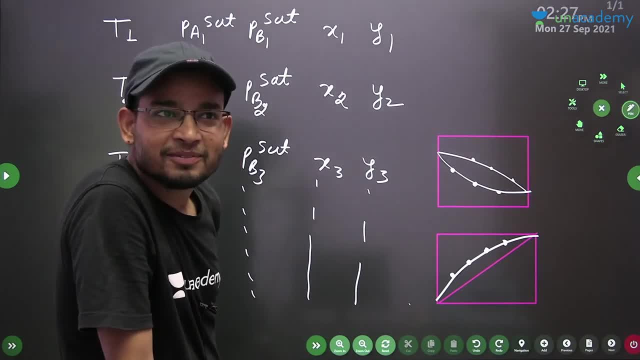 and we are going to discuss the INCREASING TEMPERATURES, INCREASING TEMPERATURES, INCREASING TEMPERATURES, AND YOU WILL FIND OUT THAT INCREASING TEMPERATURES. I will start the discussion with you, Then you will see. 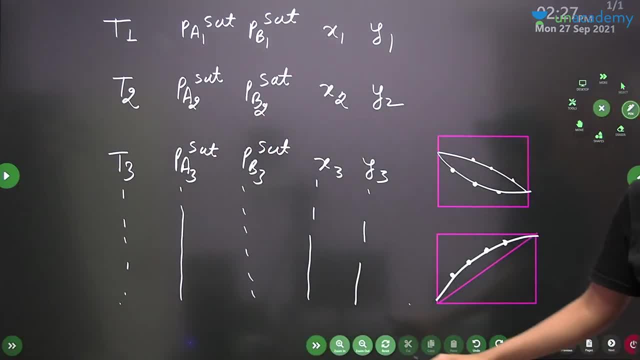 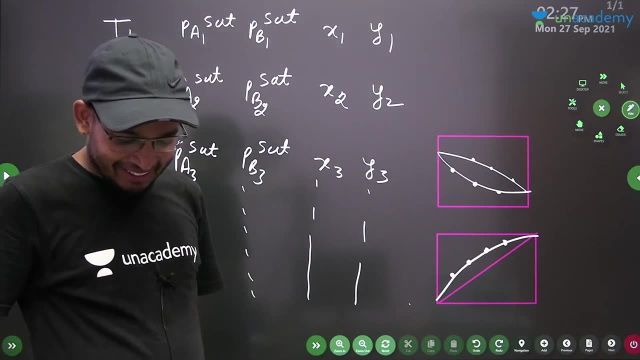 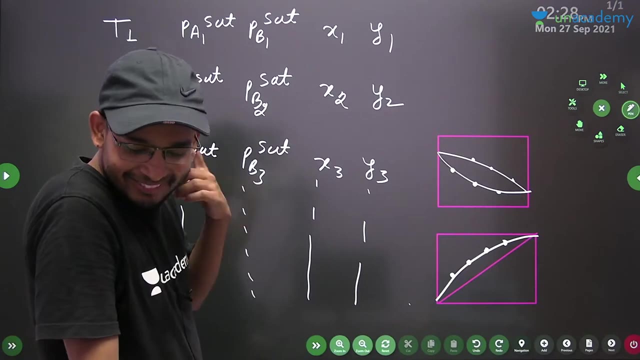 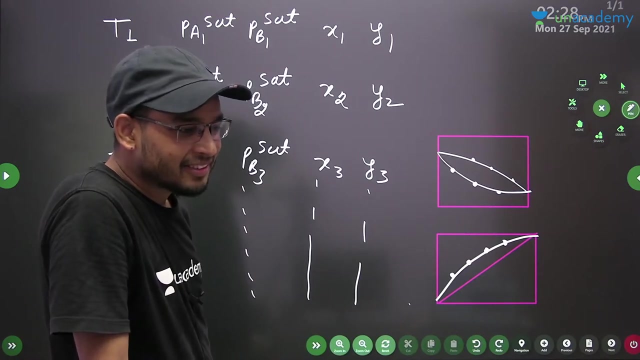 Always read like this: Don't go to give interviews, Bring more interviews. Bring more interviews, Then you will enjoy more. You should have this much subjective knowledge. You should have this much subjective knowledge. There are many students like this. They have good knowledge. 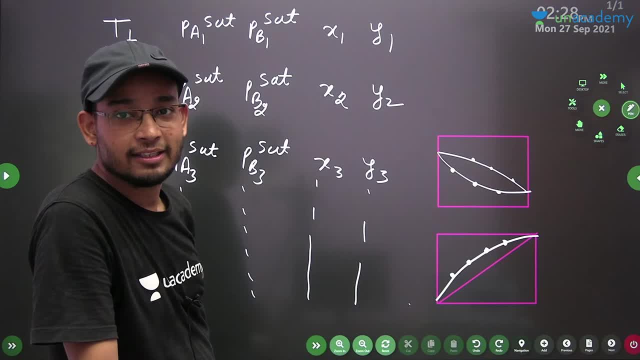 They go to interview and they learn. They go to interview and they learn. It is not necessary that they have reached a good institution. It is not necessary that they have reached a good institution. They have done a good job. Sometimes they reach. 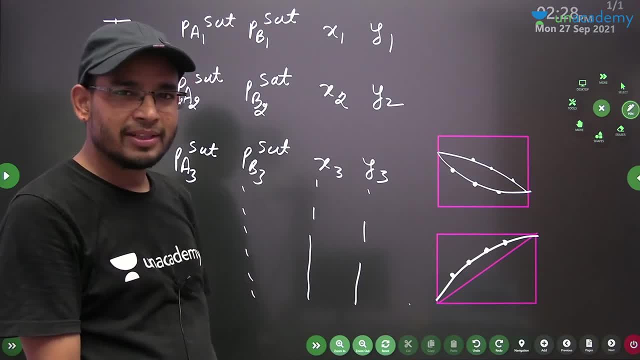 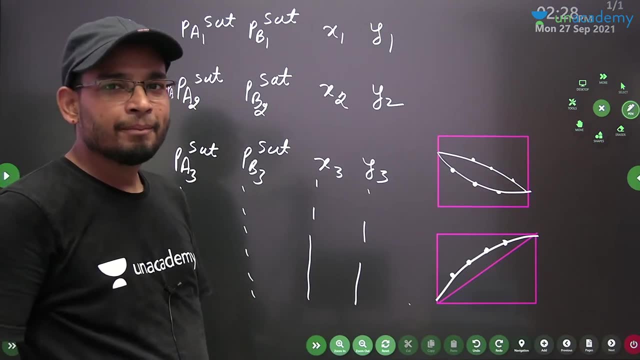 In GATE 8, the rank comes. It does not mean that there is no need to be a knowledgeable person. So the rank came, The rank will come. You can put questions. You can put questions. There are a lot of people in the KSU. 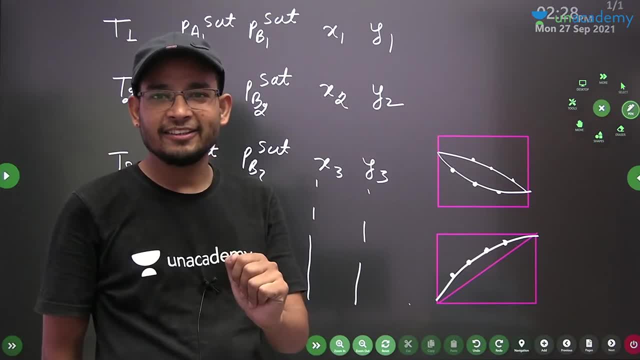 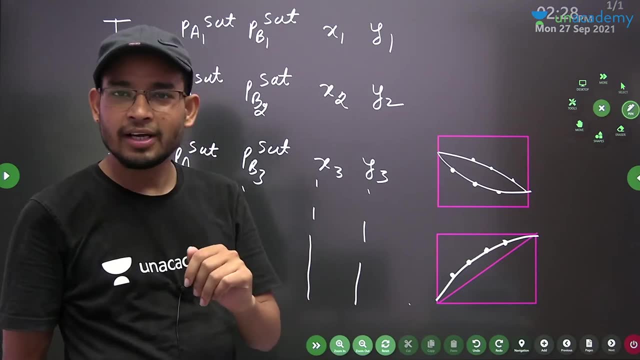 And many people who are not able to do good in three hours. What is the game of GATE? It is a game of three hours. Someone has done very well in three hours And your three hours was not good. It does not mean that you are wrong. 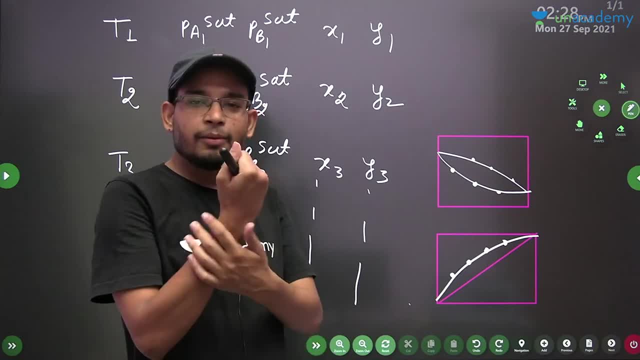 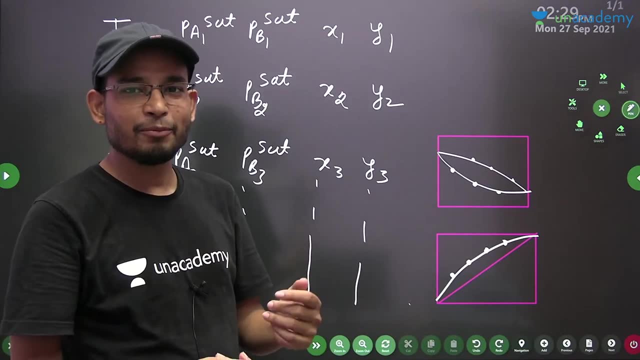 No, You are very good man. It will be useful to you. It is that he played well in three hours. Rohit Sharma tell me Sometimes it is not working. It does not mean that the work is not going. He was not able to perform at that time. 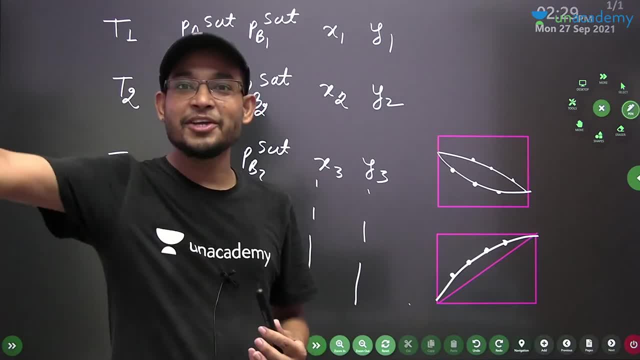 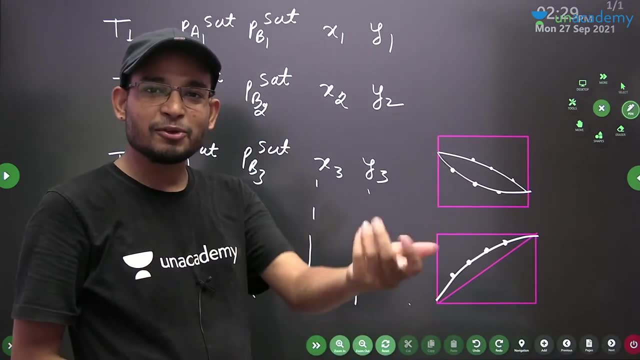 You must have seen him hitting long sixes on the net One day. you must have seen that he was looking for the ball in some bushes. He was not able to do it there. It turned out that a small bowler came and got up from the IPL and bowled him. 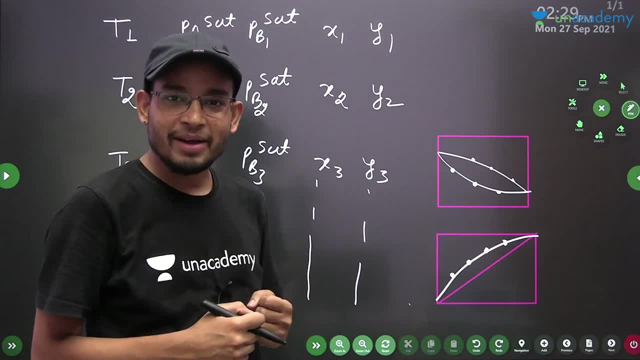 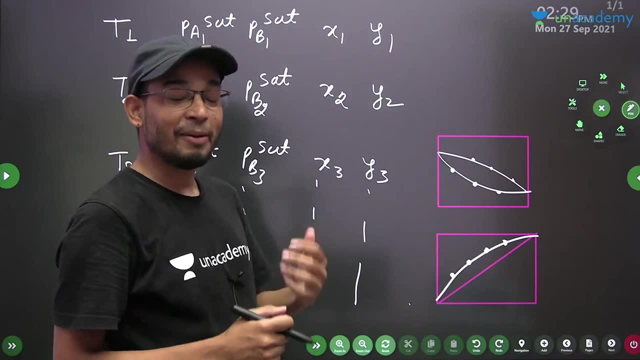 Okay, So now he didn't think of himself. I am everything. He hit the Malinga's long sixes in the World Cup. Okay, You IPL people don't have to bowl and fix your collar. He hit the Malinga's sixes in the World Cup. 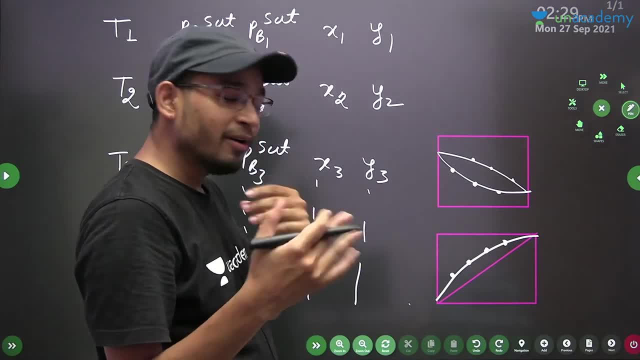 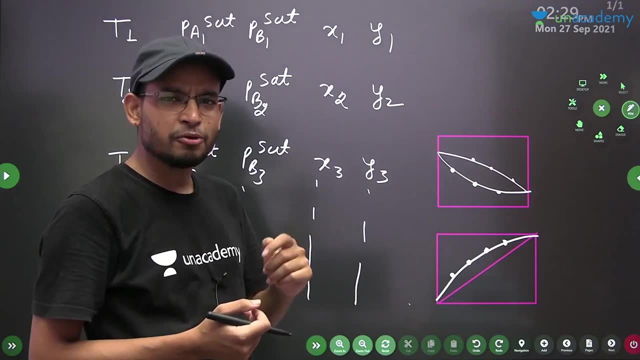 Okay, This is IPL, So it's a matter of time. Someone's three hours went well, So he made a run. Your three hours didn't go well, You couldn't make a run, So this doesn't mean that you are not weak. 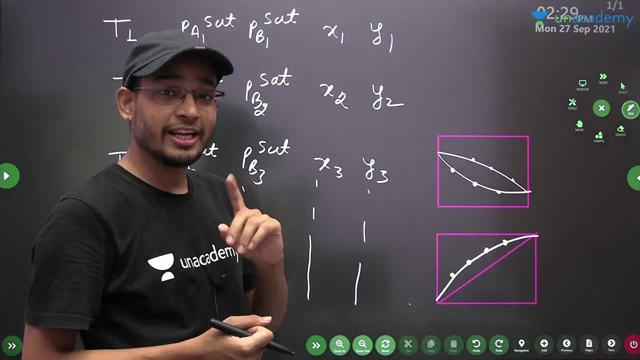 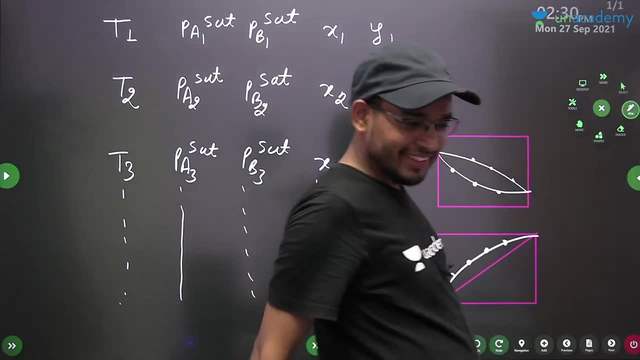 Okay. So the next time you hit the long sixes, it will look far away. It's a matter of time. One day, our time will also come. Okay, Our time will also come Right. It's a matter of time. 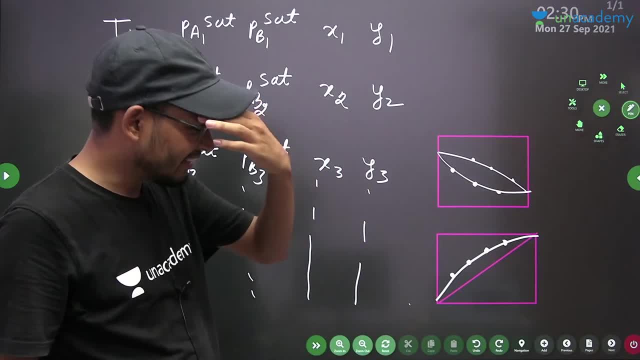 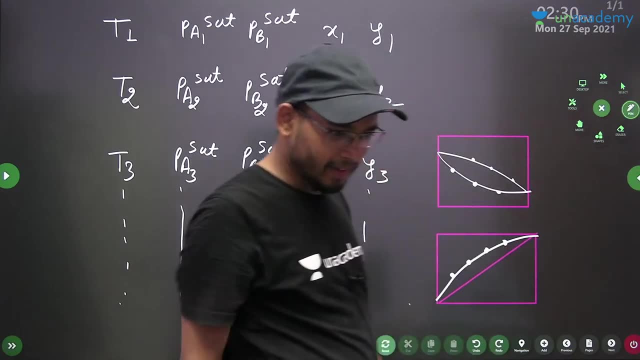 It's a matter of time. That's it, No problem, Our time will also come very fast. The time will come fast Once we get down on the ground. we will hit the long sixes like this. Okay, But keep the confidence of the strong. 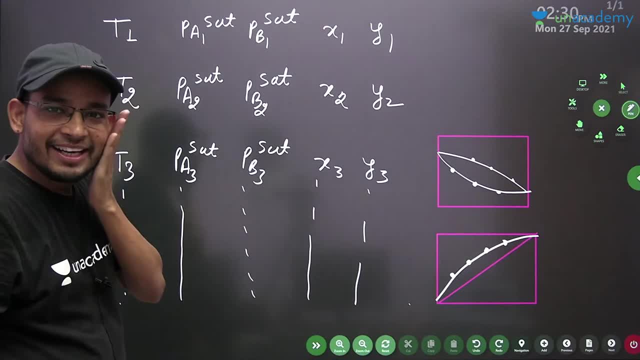 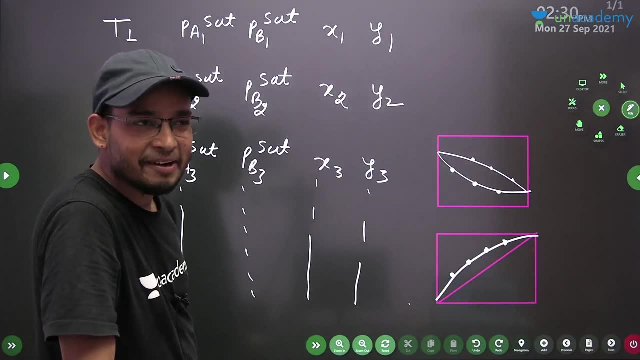 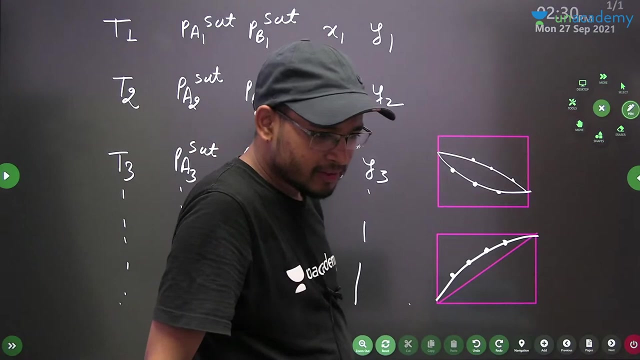 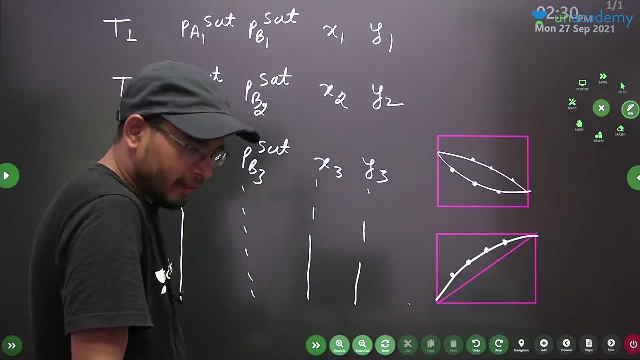 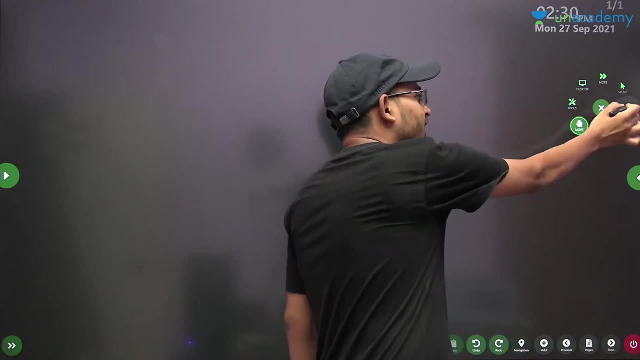 See, I will now tell you the third method with confidence I have not told you until now. See, See, I will tell you three methods of equilibrium curve. This is method number three. Come, If you want to talk. please talk on equilibrium curve. 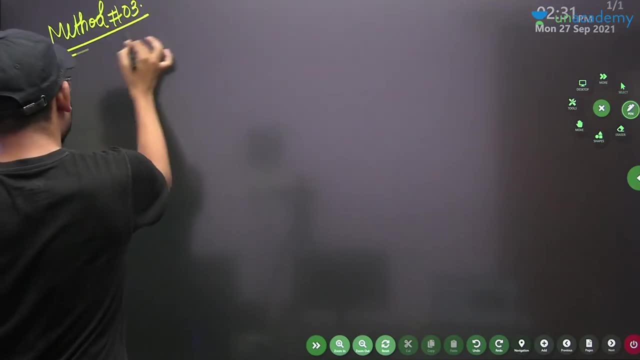 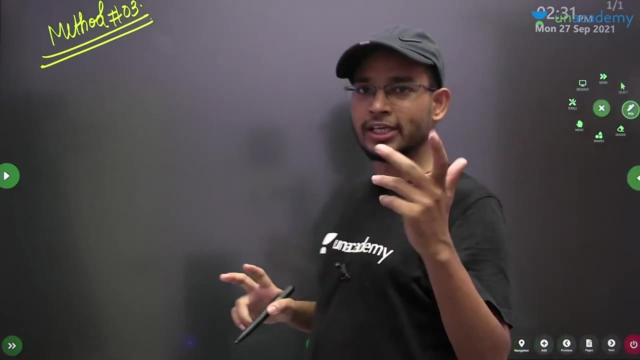 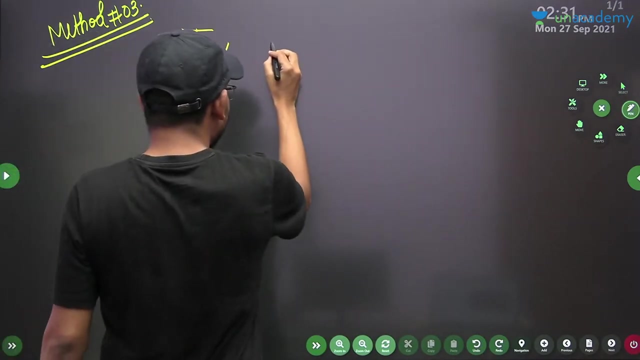 If you have one now, you focus on this. For example, this is the whole unit of balance, Right? the second method is analytical and the third method is also analytical, but in a different way. in case you know the temperature, you know the temperature. so what you did? 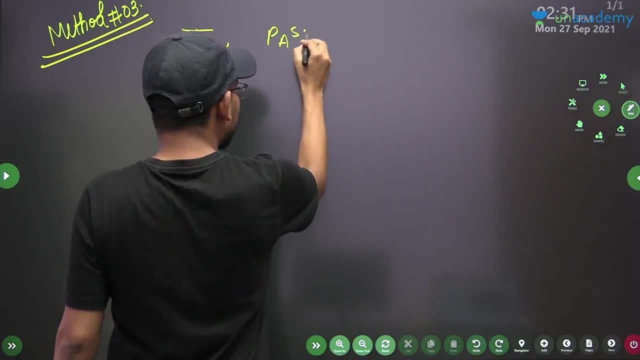 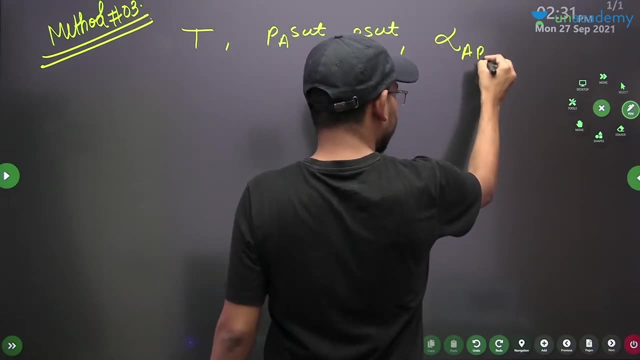 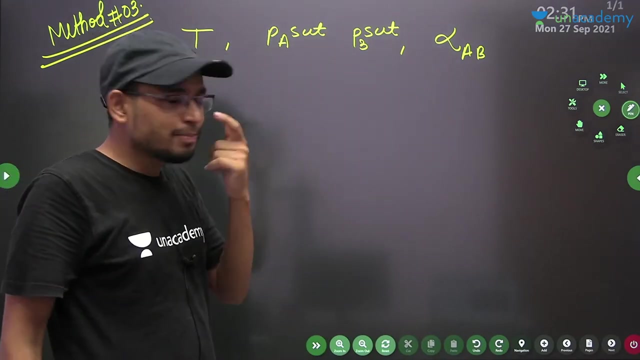 you got the saturation pressure, you got the PA side and you got the PV side. ok, and according to this, you got the alpha AB. ok, you got the alpha AB right, you got the alpha AB. now, in case you know the alpha relative volatility, then also you can smile and 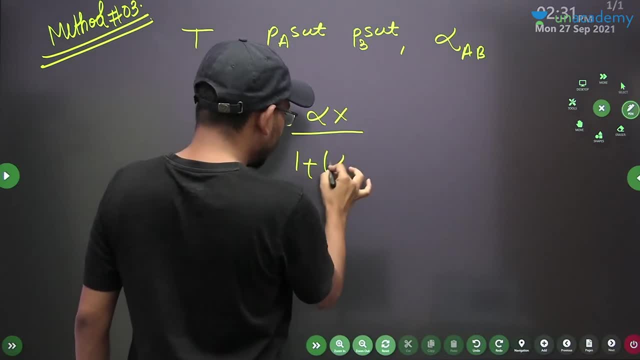 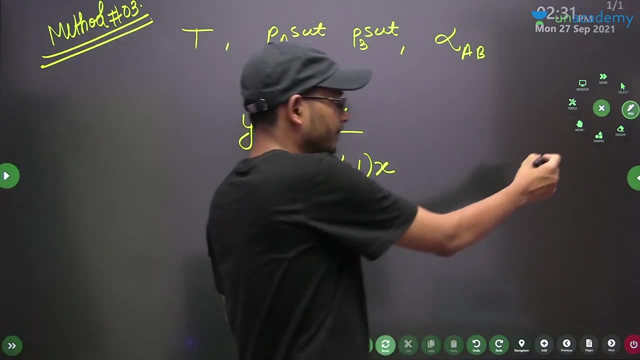 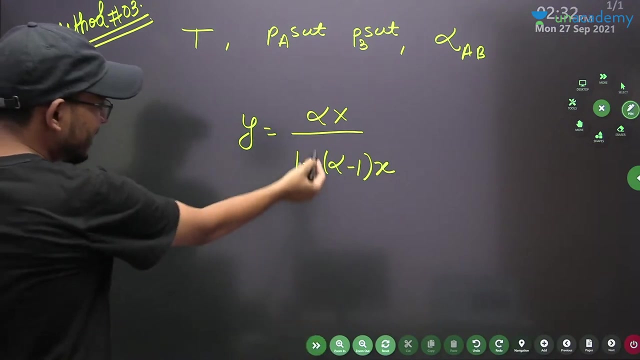 y is equal to alpha x upon 1 plus alpha minus 1 into x. ok, with the help of this equation, you will be able to make the equilibrium curve. you will be able to make the equilibrium curve, ok, now, as you keep on keeping the alpha value. 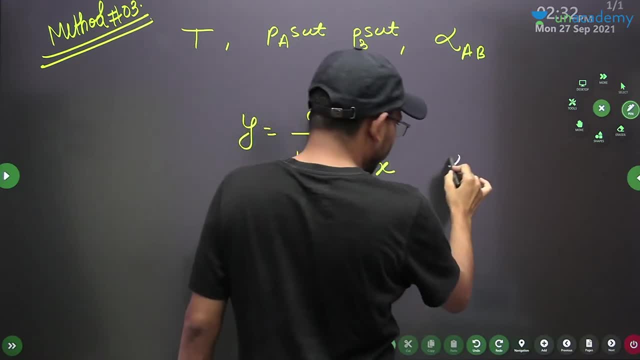 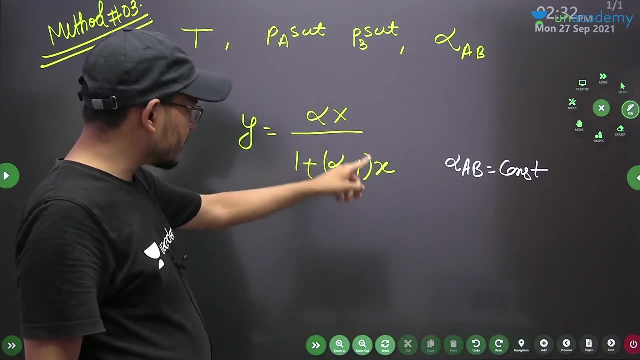 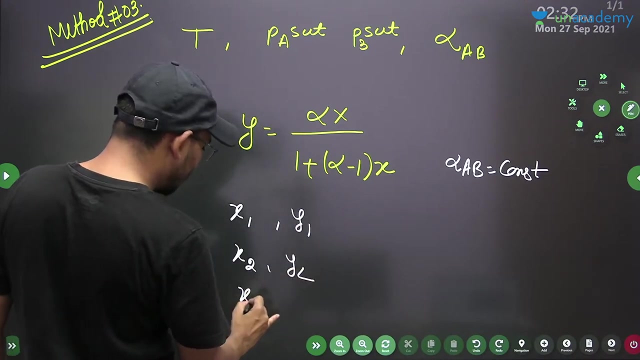 as you keep on keeping the alpha value. suppose your alpha is constant. alpha AB is constant. alpha AB is constant. ok, suppose, throughout the system, your alpha is constant as the x changes. on x1, you will get y1. on x2, you will get y2. on x3, you will get y3. 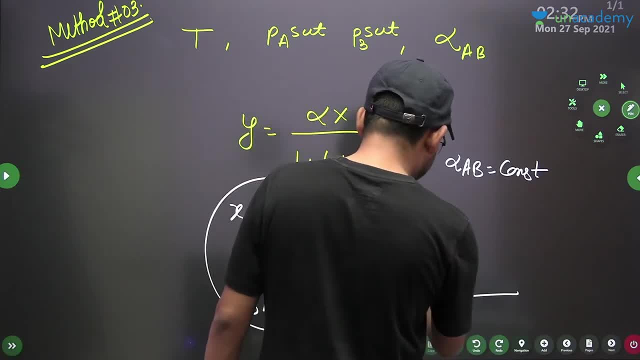 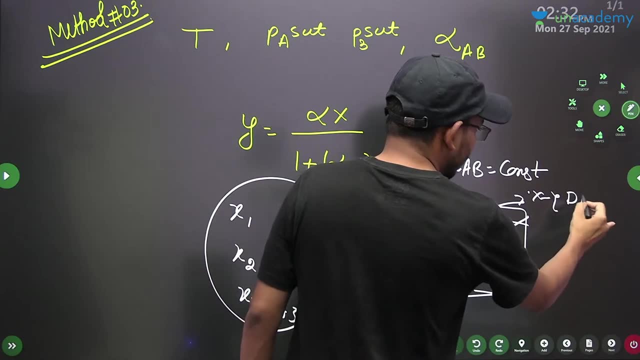 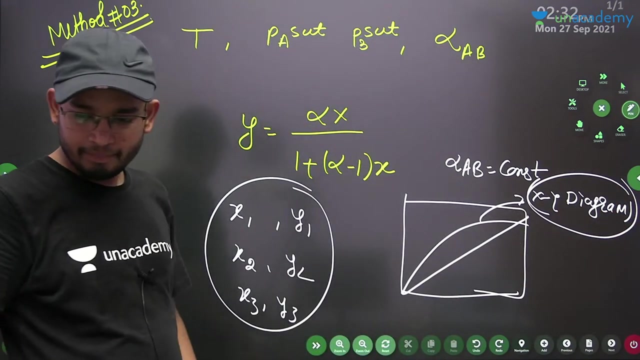 ok, you also got this point. and where did you put this? on xy diagram. you put this on xy diagram, so this is your xy diagram. ok, xy diagram. this is the method number 3. if you won't write x in this method, ok, you will also find x Greek. 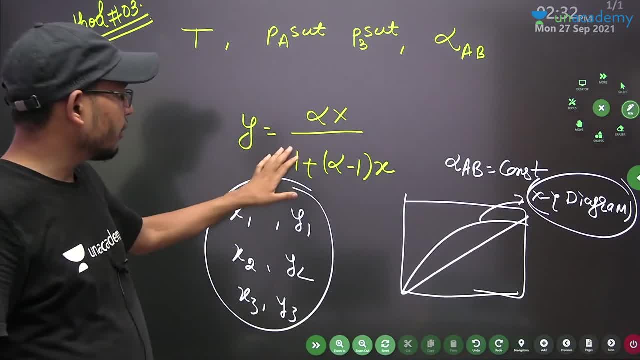 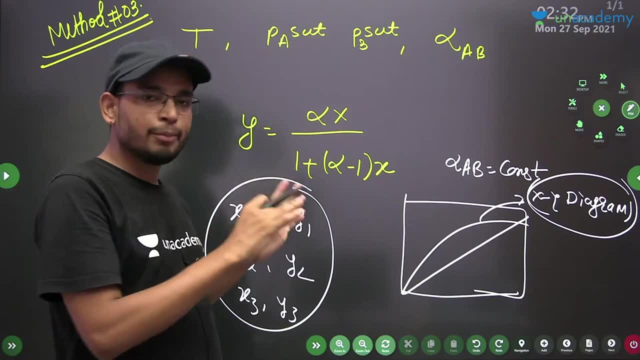 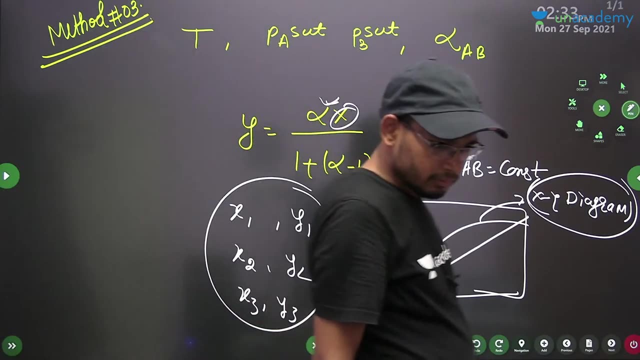 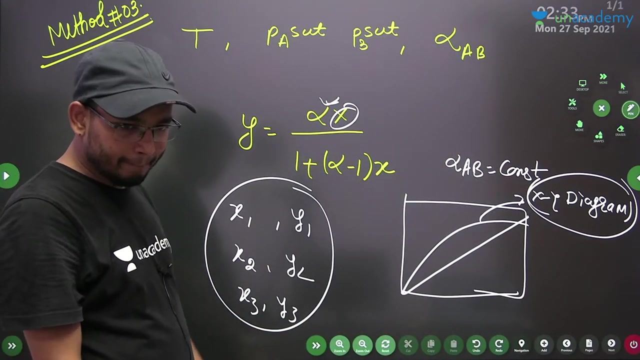 you will find x and y diagram as well. this way you will also find x and y diagram if you backside along with the same, taken a example term, we will also do the same: x and y diagram. we will also take xurea diagram, fine, so this is method no.3. 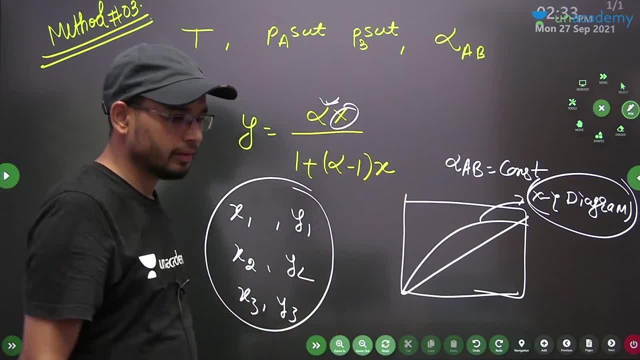 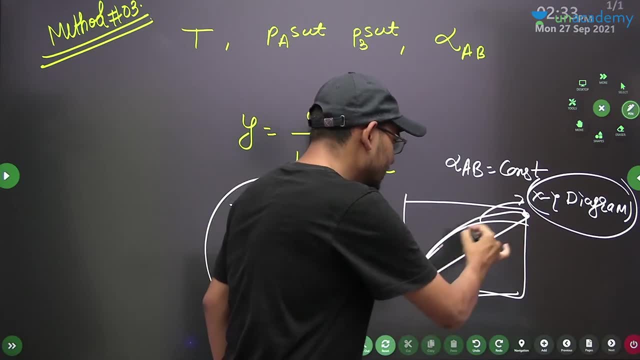 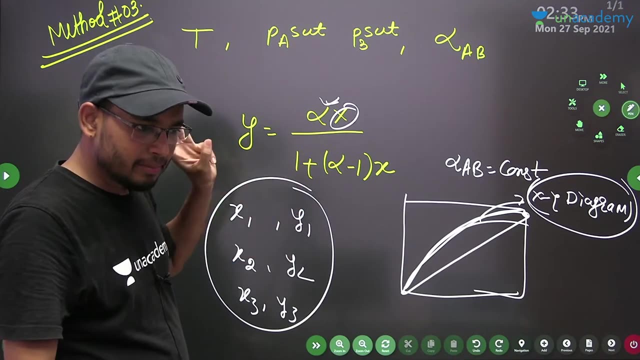 so this is also your xy diagram, this one perfect. so in this way we will get it in diagonal. you will make a beautiful figure. i mean, i just explained it to you, right? so what was this txy diagram, which has 3 methods? so now you have covered a small part of that step. 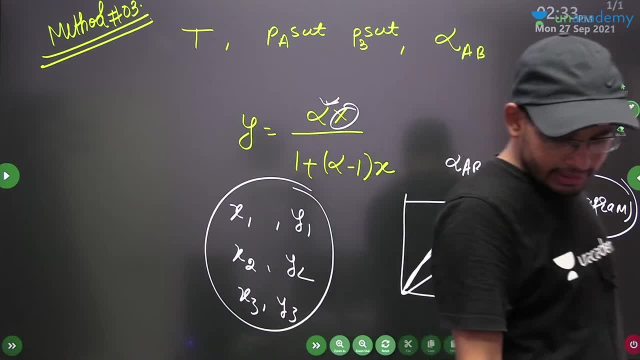 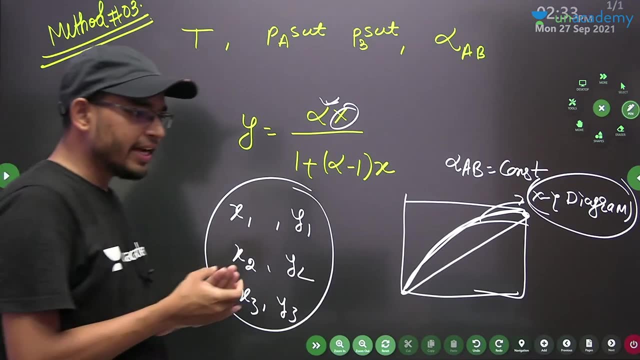 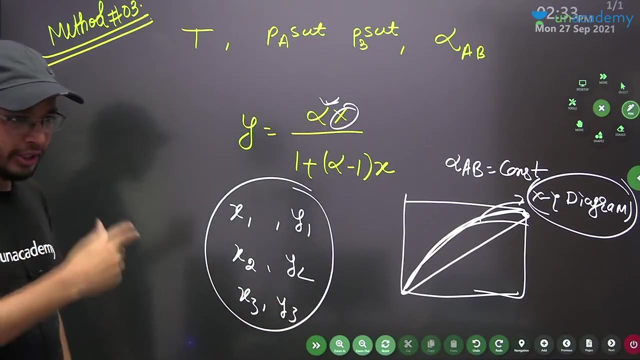 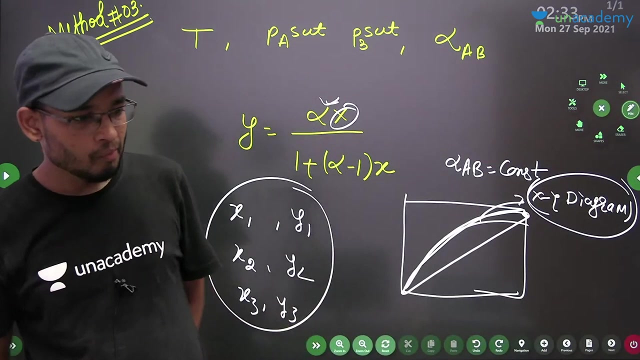 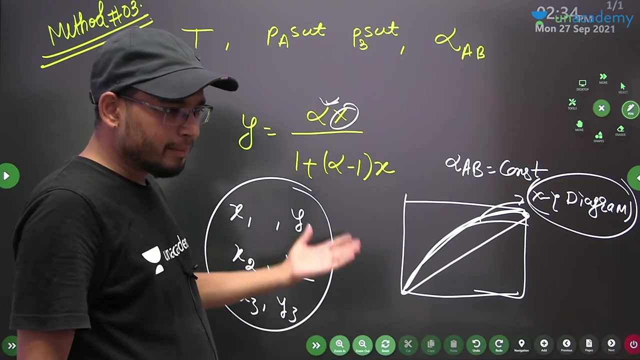 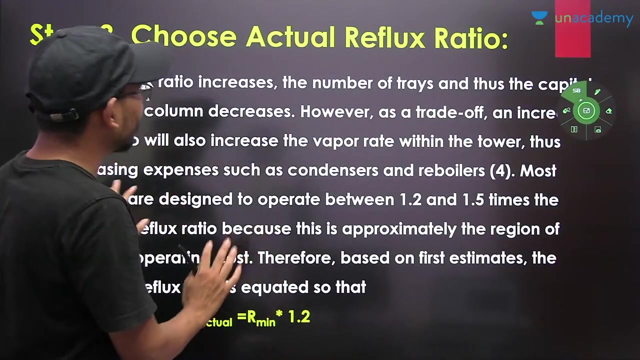 till here, everyone understood, yes or no. everyone understood equilibrium diagram, right. everyone understood equilibrium diagram right. tell me, do equilibrium, fine. till here, everyone understood. till here, there is no problem. i have explained it to you. now. see again, this was in the middle. if your equilibrium curve was in the middle, 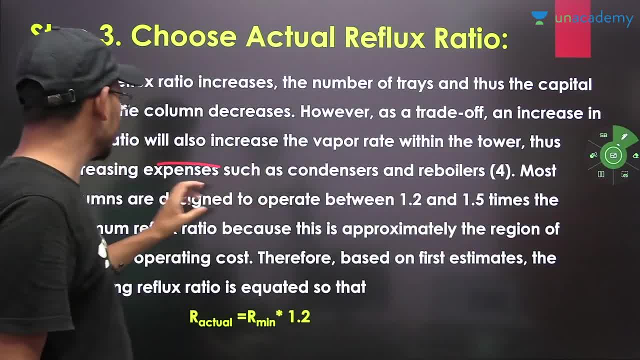 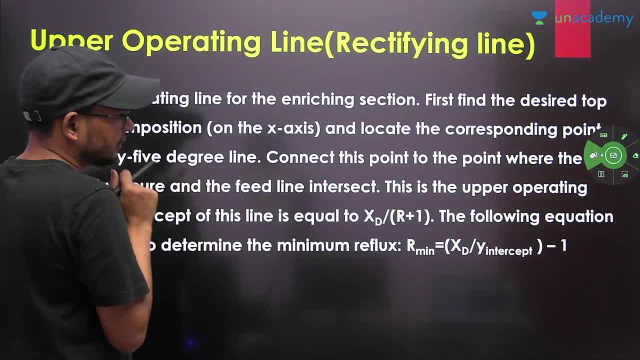 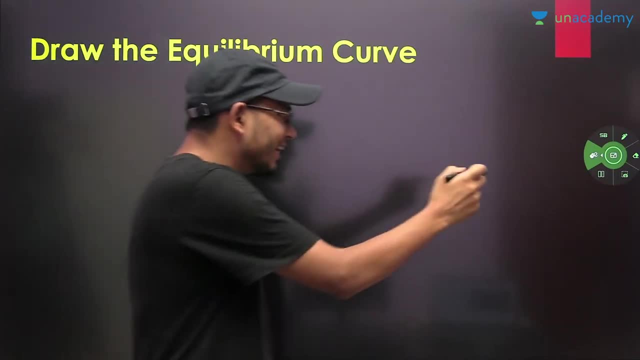 i have explained it to you in detail now. this is passing through the path, the draw, the yes till where we have reached. we have reached. draw the equilibrium curve till this part we have reached. you will have to know equilibrium curve first. you should know the equilibrium curve. 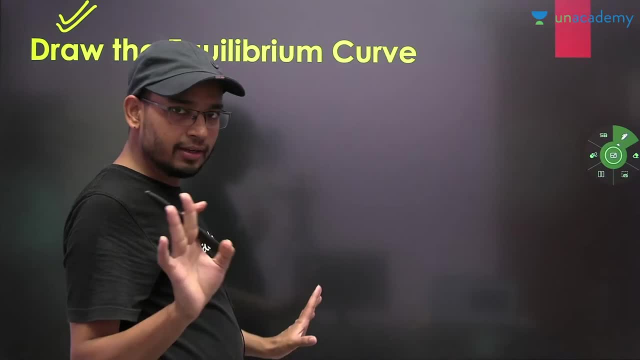 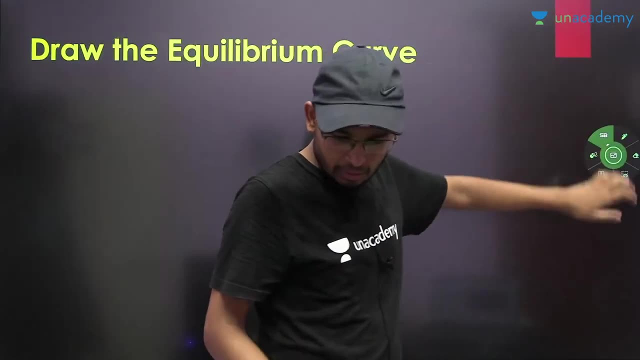 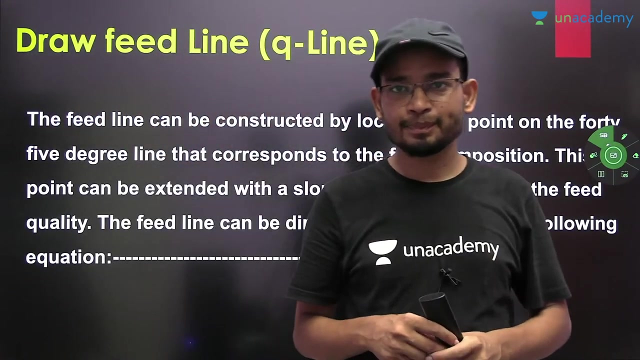 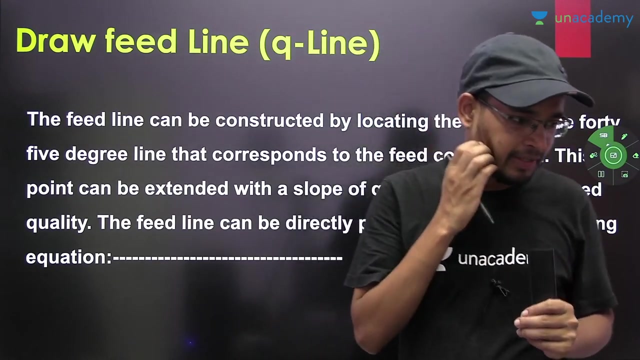 how you will draw it. you have done it fine. now the next step. next step: i will talk from here. i will talk from here: draw the feed line. now you have to draw the feed line. where, on equilibrium curve, on equilibrium curve, what you have to draw, what you have to draw on the equilibrium curve, you have to draw the feed line. 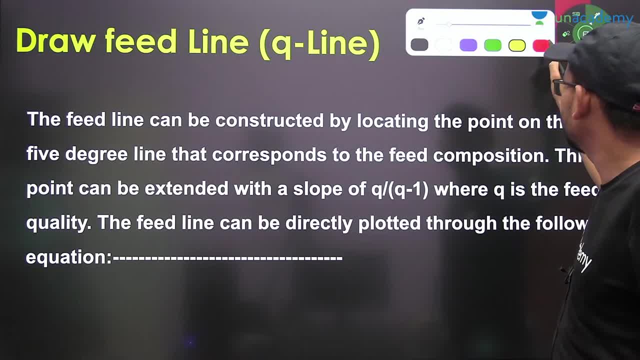 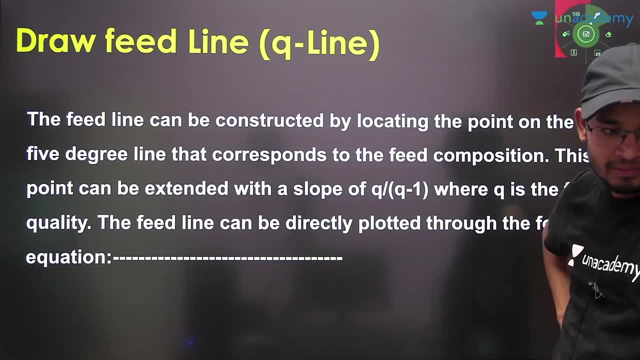 means Q line. Q line means you have to draw the feed line. will you draw it? what you need to draw the feed line, first of all, what you need to draw the feed line, tell me you have to draw the feed line. so what you need, Q and Q. 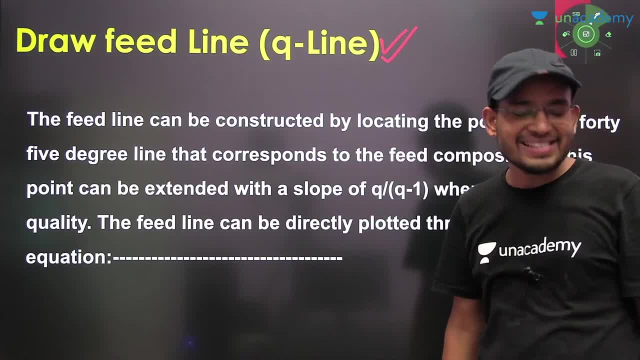 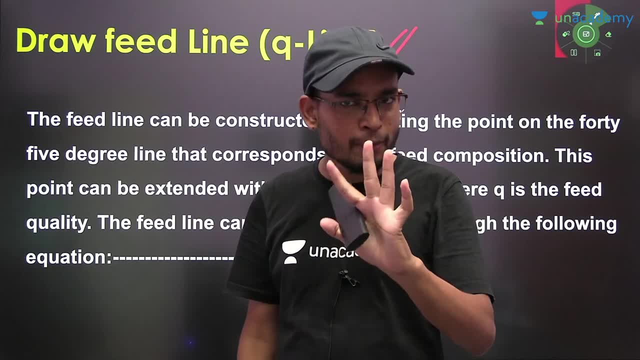 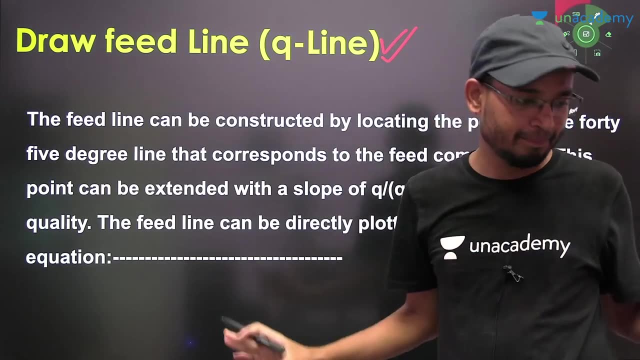 you have to know this in the first step, because you already know what kind of feed you are using, right, what kind of feed you are using. Q is known to you. Q is known, Q means what kind of feed you are using. you know everything about feed, feed condition. 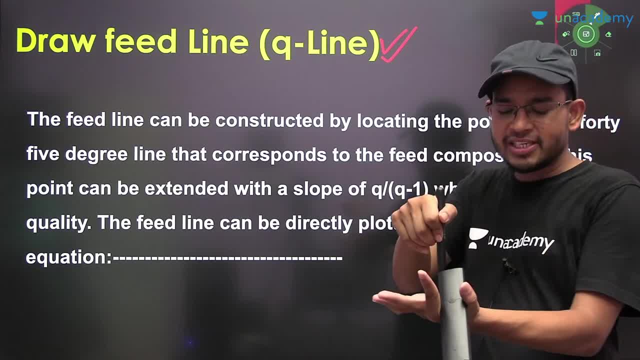 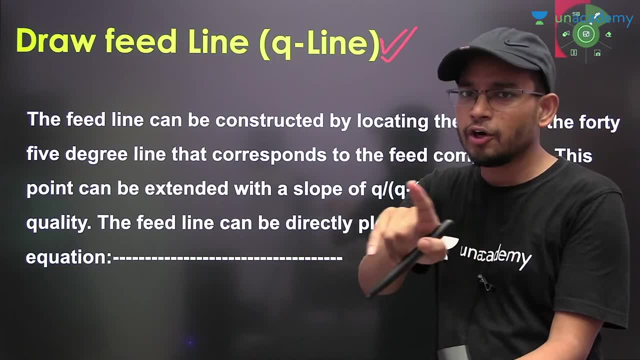 Q and XF. this is already known to you. you have to draw the composition in the first step. Q is the feed condition. you know, in the first step you will not need any other thing. you will need the equilibrium curve. you have to work on it. 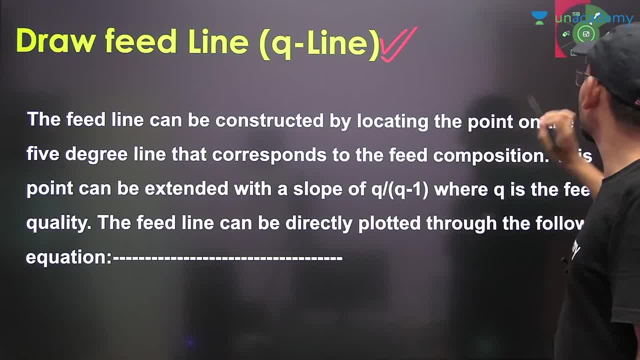 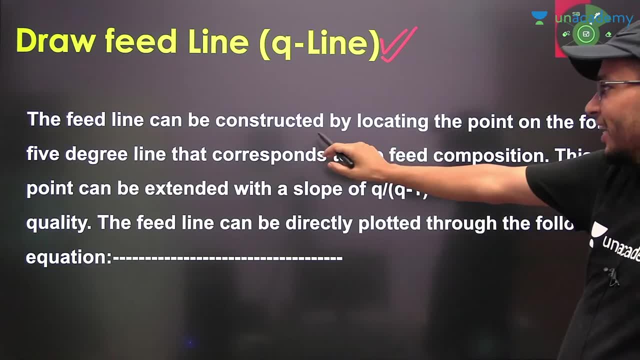 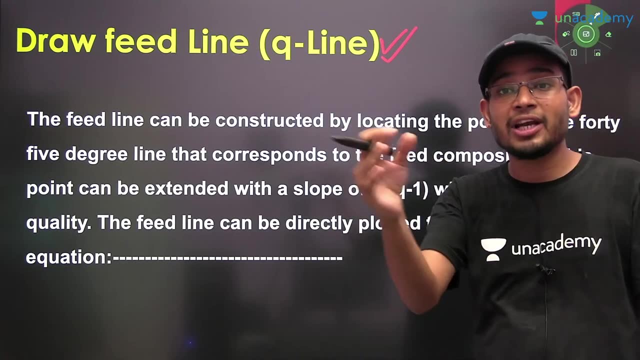 ok, now draw the Q line. so you have to draw the Q line. to draw the Q line, first of all, feed line can be constructed by locating the point of the 45 degree line. 45 degree line means the diagonal line at the corresponding of the feed composition. 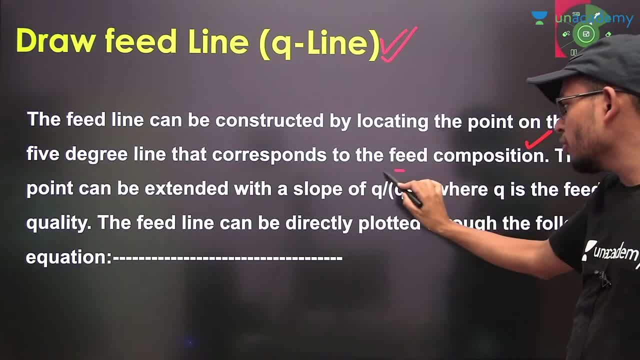 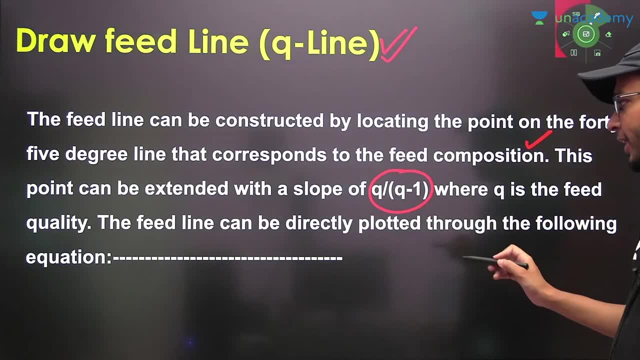 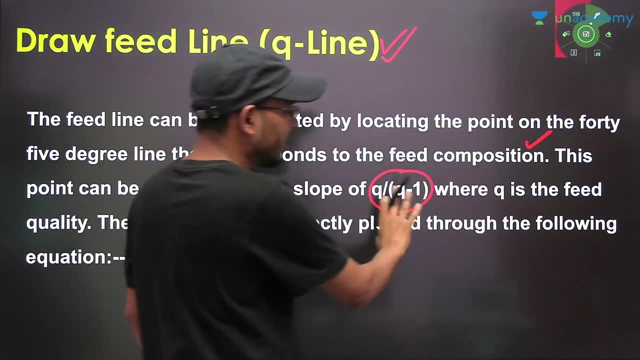 this point can be extended with the slope of Q upon Q. what will you do with that line? you will extend it further. ok, where Q is the feed line. yes, you will directly plot this by the equation of. this is the second method. first we will talk about the graphical method. 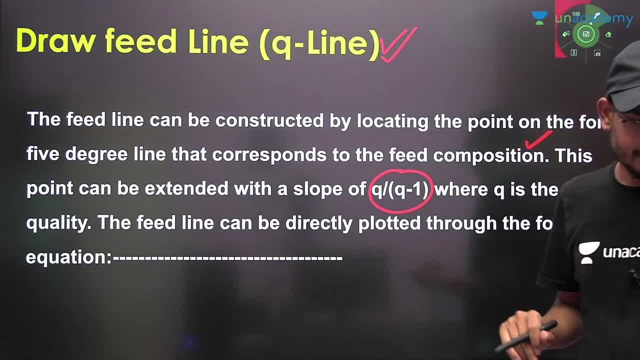 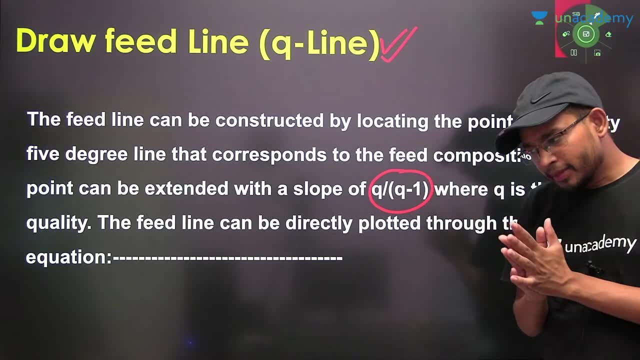 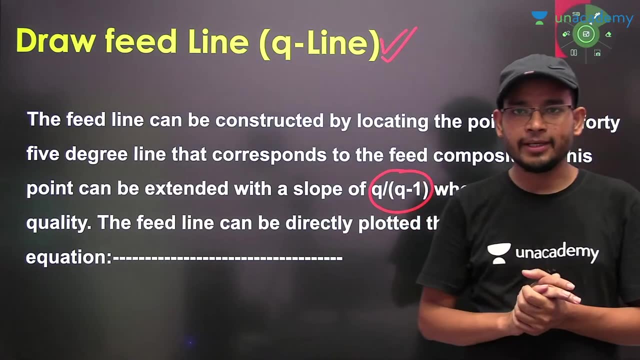 first write this, then I will plot it and show you. write this first means how will you draw the same thing that you have written here. I have told you how to construct the Q line. you know the feed composition and the slope. ok, what is the slope? 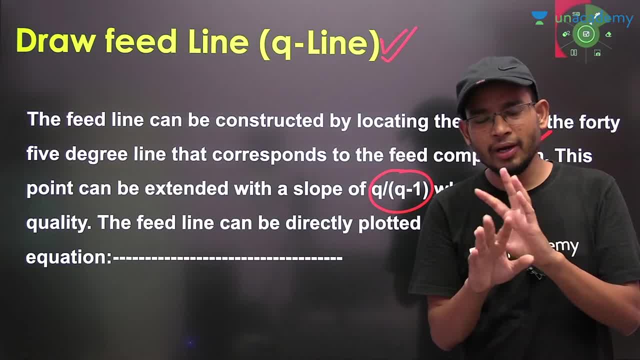 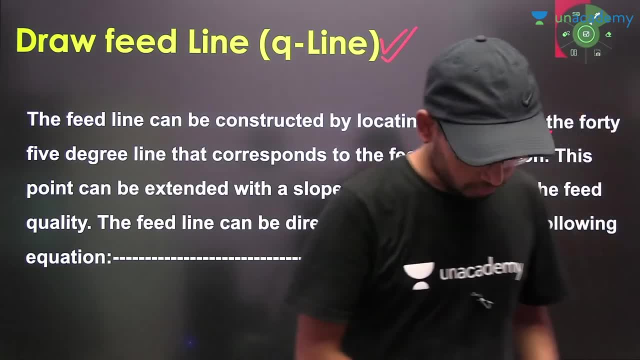 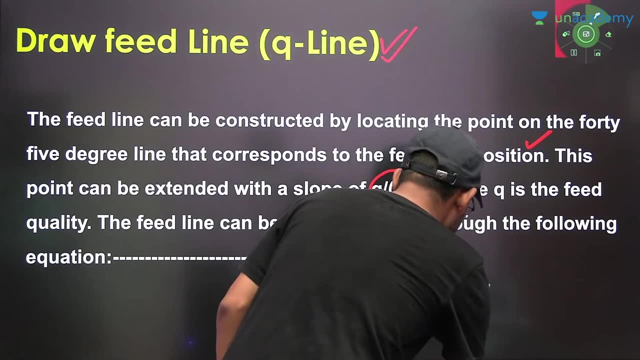 Q upon Q minus 1. this is the slope of the feed line. now I will tell you the equation of the operating line. from there this slope comes. write the equation first. write the equation. Y is equal to Q upon Q minus 1, X minus XF upon Q minus. 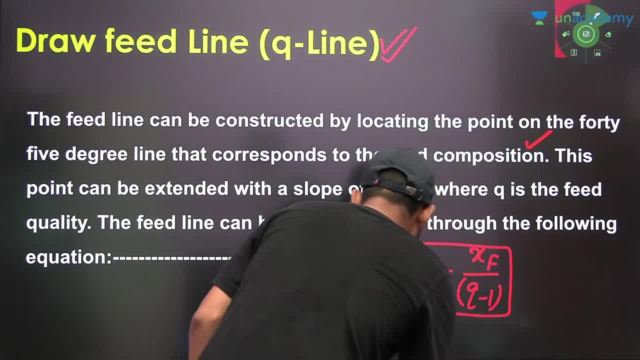 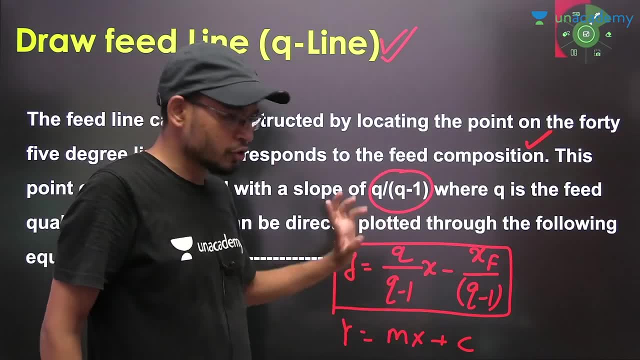 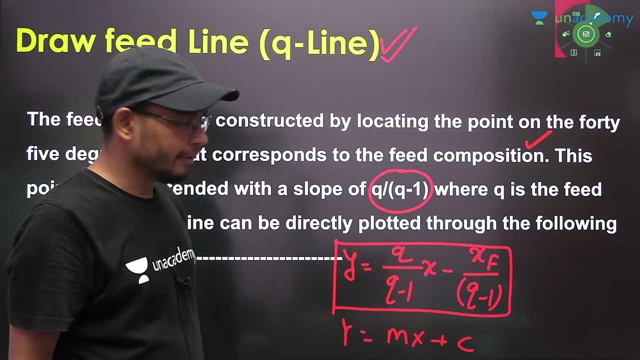 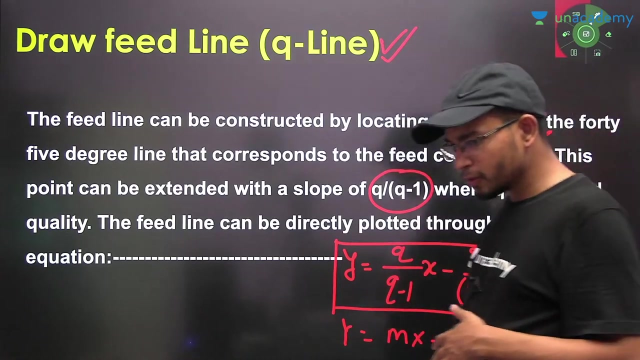 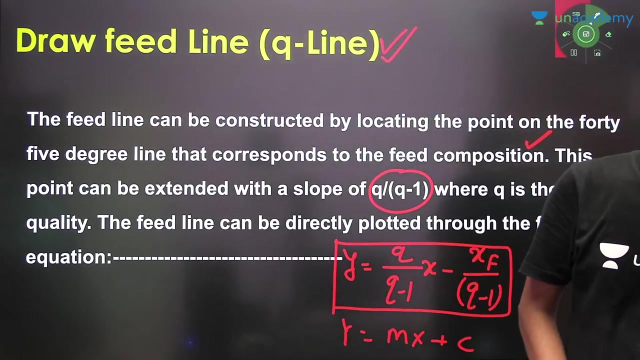 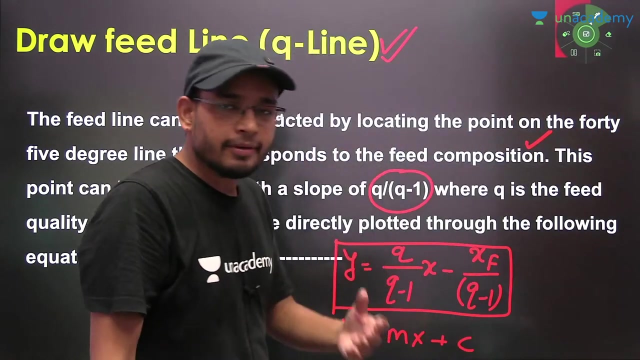 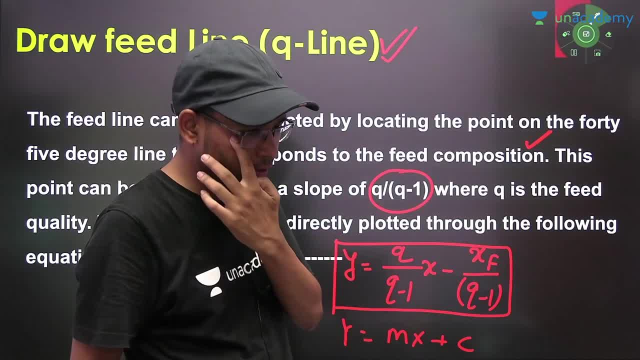 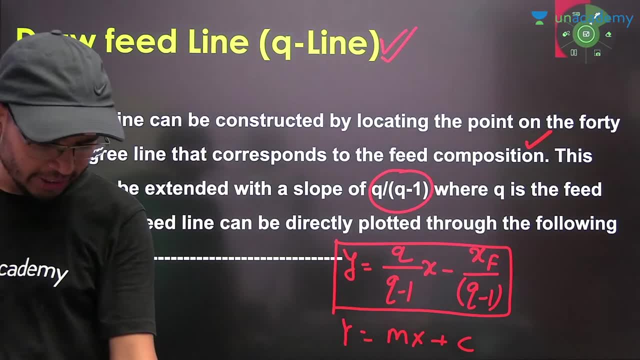 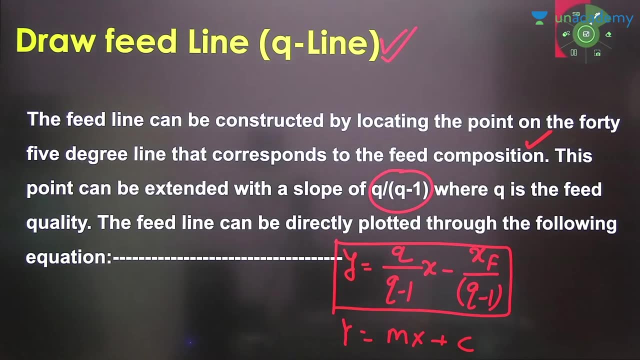 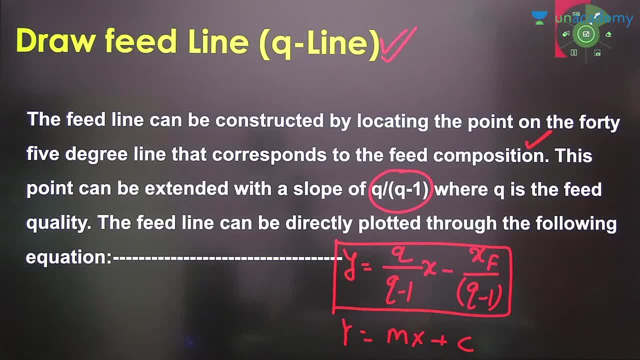 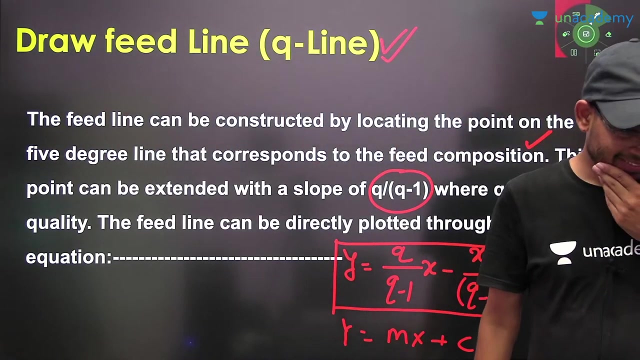 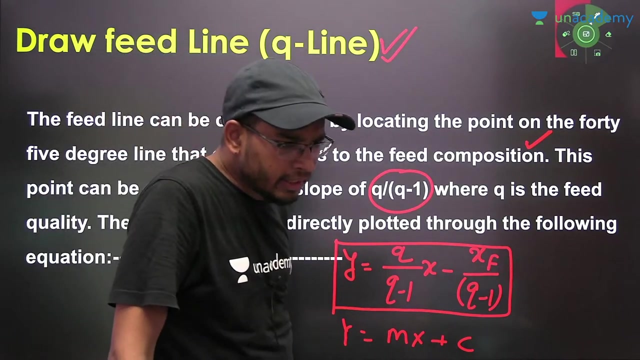 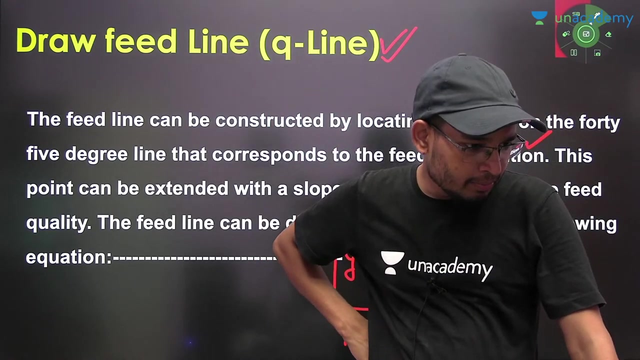 All right, Thank you. Thank you, Sir. there is a big doubt that if there is W at the bottom, then will it be a mixture of both the components, in which more volatile and less volatile will be present, Means we can say that there will be a condition like feed. 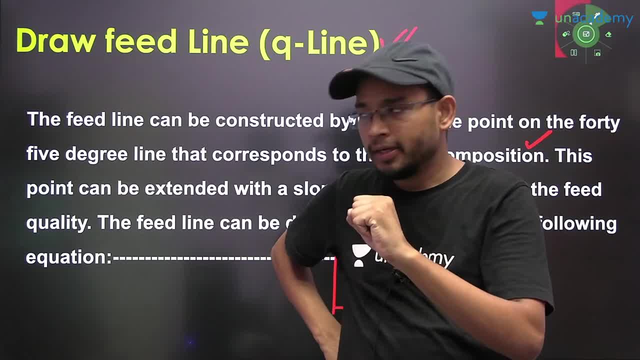 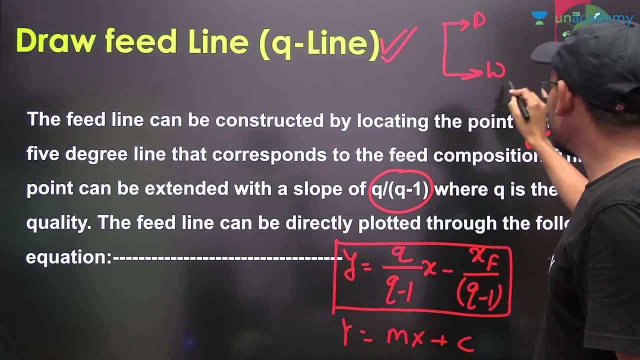 Yes, there will be both in W. W is the bottom flow rate, W is the simple bottom flow rate. There is a big doubt, sir, D or W. This is the bottom flow rate. Here also A plus B and here also A plus B. 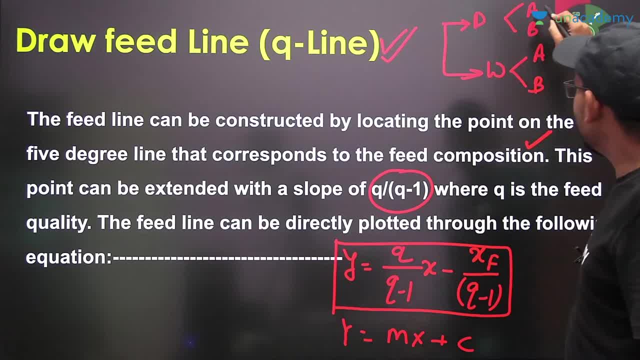 See it is getting clear in a minute. Give them a minute's time. A is the more volatile, B is the less volatile. Here, A will be more and B will be less. Here, A will be less and B will be more. 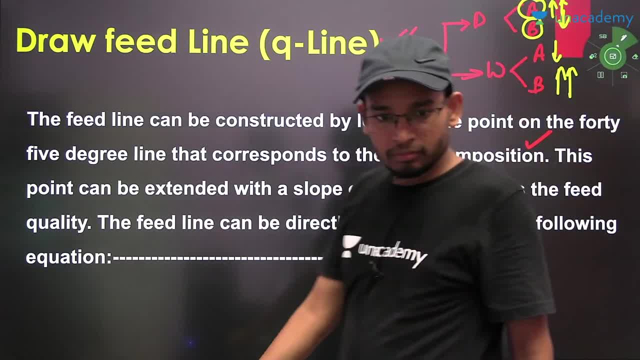 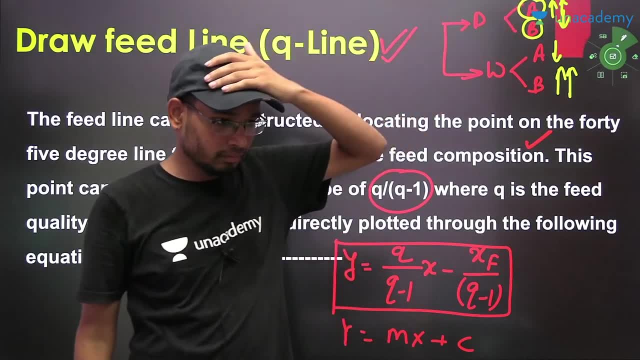 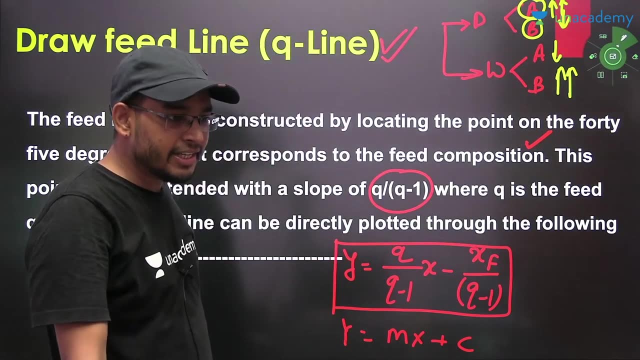 Here, A will be more. That's it Finished, Tick. There will be more B at the bottom. There will be more E here, But there will be both. Yes, I am bringing the entire crash course of MT, Okay. 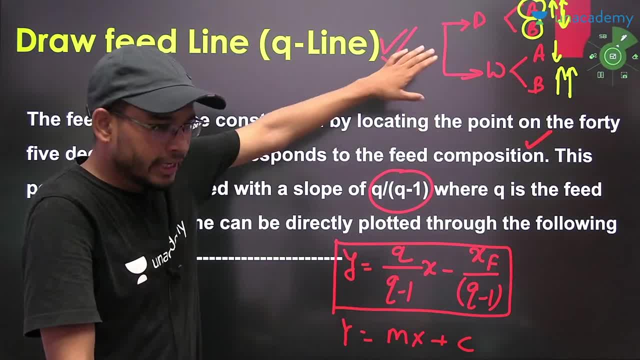 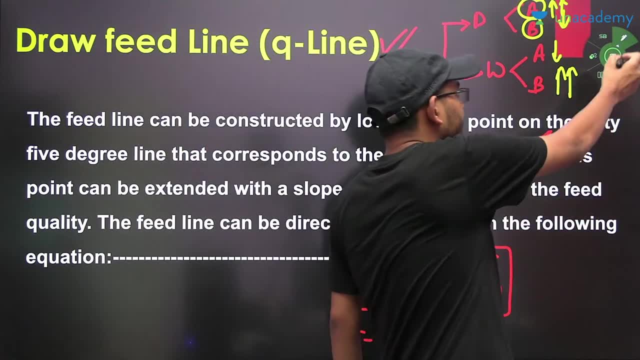 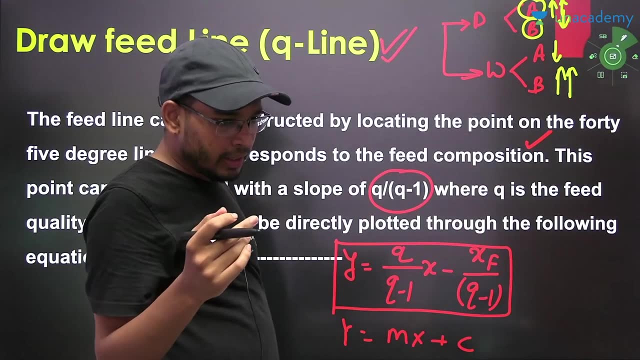 You will get the entire crash course of MT Siv. your doubt is clear? First tell me this: 800: 00.. 0000.. There was a minus sign this time. Okay, getting open. Ok, Option 1.. 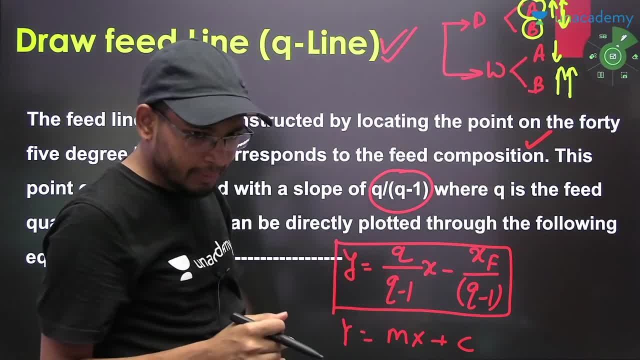 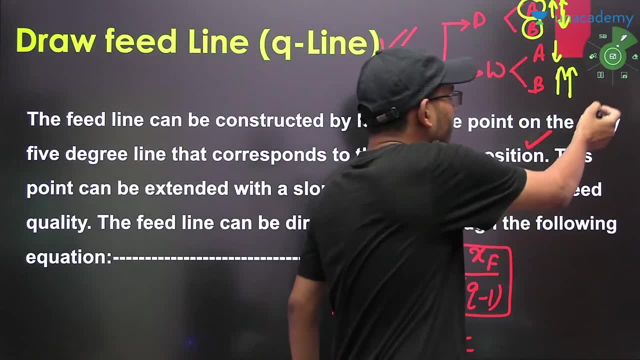 Turn towards the other school. そう 템你说. The first school will be sing. Okay, Now I get out of here. How many was it? Two in A cliques? No sensitivity. It wasn't nice. No sensitivity. 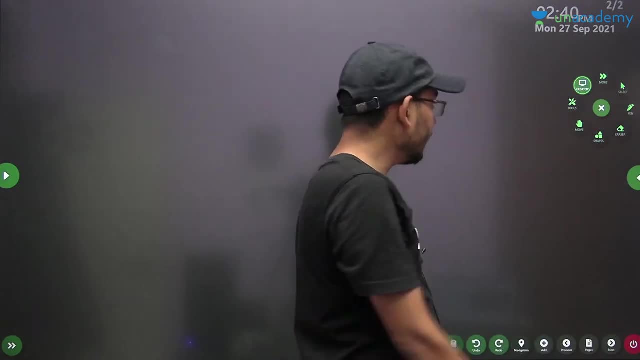 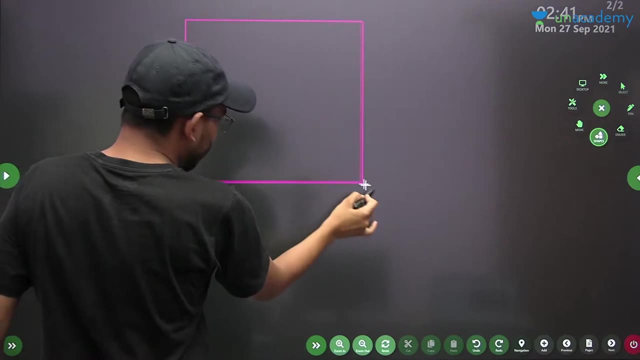 Now what you have to do is you have to draw the line, then you have to draw the line in your copy. okay, In the same copy you guys are writing properly. you don't just have to listen, you have to make it too. 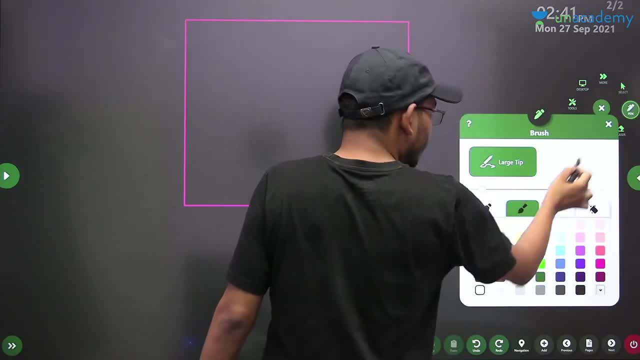 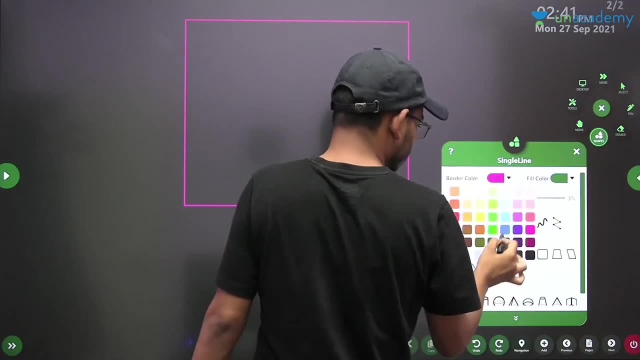 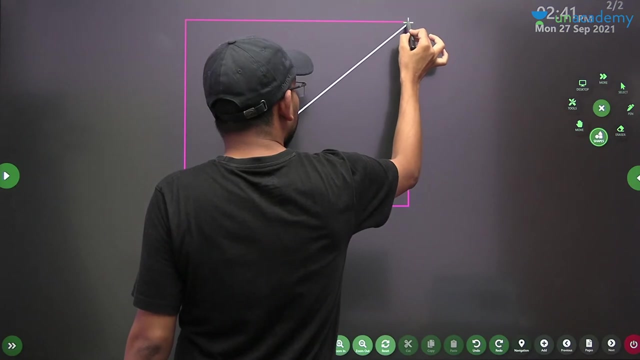 Okay, this work will come, write it in your copy. you will go to give this interview, then you will find it. It will take a lot of time to read the book, etc. Okay, you know this diagonal line. there is no problem in making a line, you will draw. 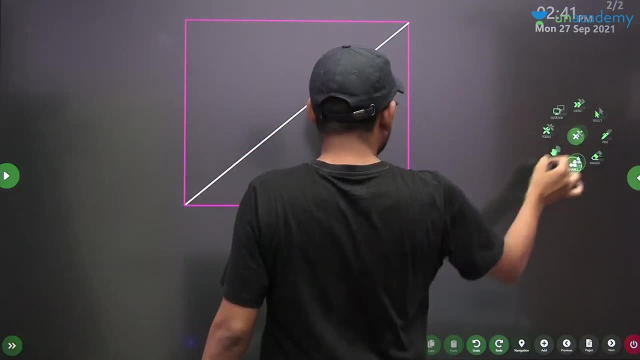 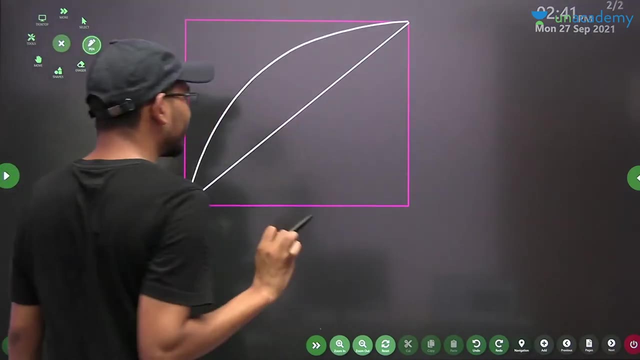 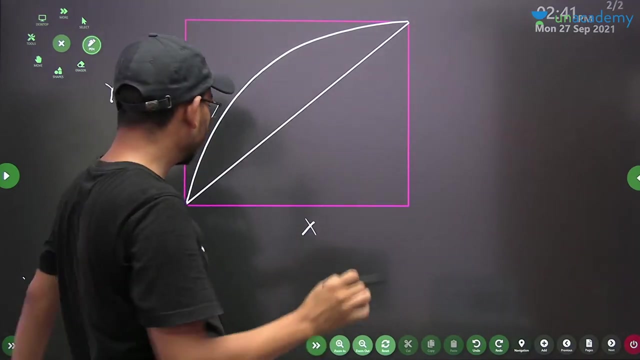 a line of 45 degrees straight. and what will you do from here? how does this equilibrium curve come? I have just told you: okay, this is y and this is our x. okay, how does the equilibrium curve come? I have told you three methods. okay, what was our x dub? okay, now I am talking about 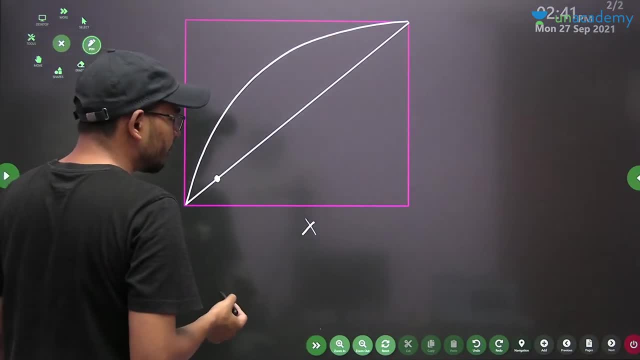 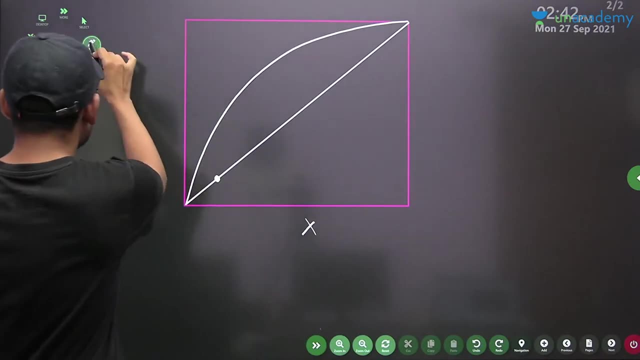 the feed line. So I am talking about the feed line. so it means you will know the condition of the feed. right, The condition of the feed will be known. it means you will know the xf. xf will be known to you, so xf will be known. so what will you do? you will go from here, xf and you will. 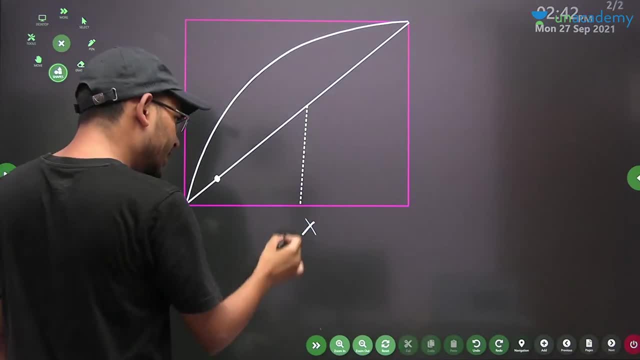 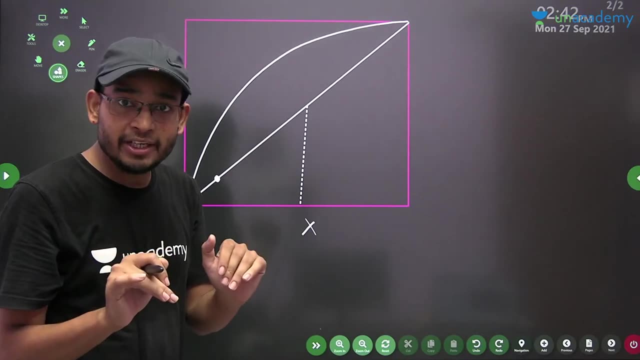 pull it straight. okay, you will know this. xf, it is known. that's why you are pulling. you have found out. you have found out. you will not do anything like this from your mind. you will calculate everything first. only then you can design. okay, you should know. 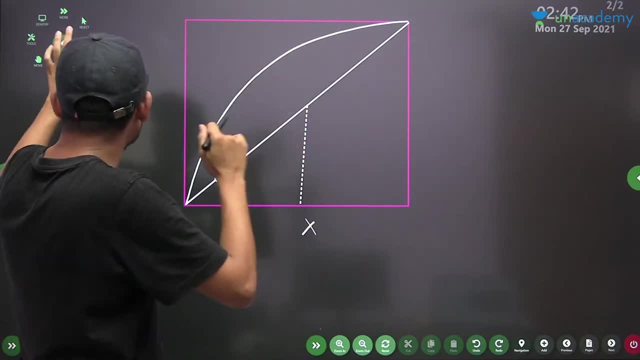 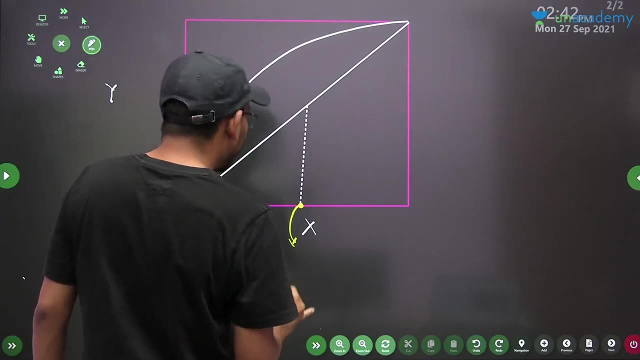 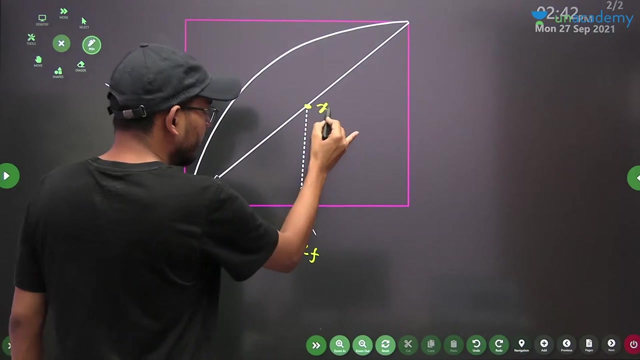 everything. first, This xf. you knew the condition of the feed in the first step, okay, only then you are able to do this work. this is the xf, okay, this is the xf. okay, and what will be? xf? because what happens on the diagonal? xf, comma, xf, xf, comma, xf. okay, it is the mole fraction. 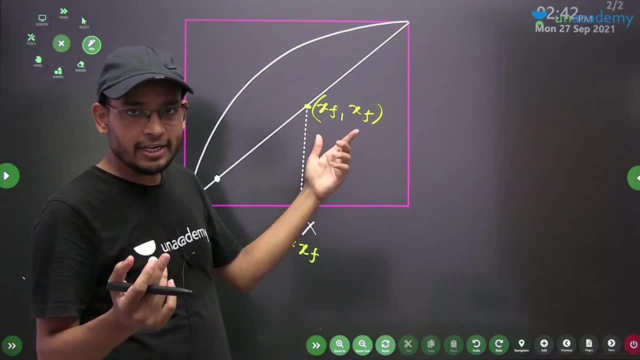 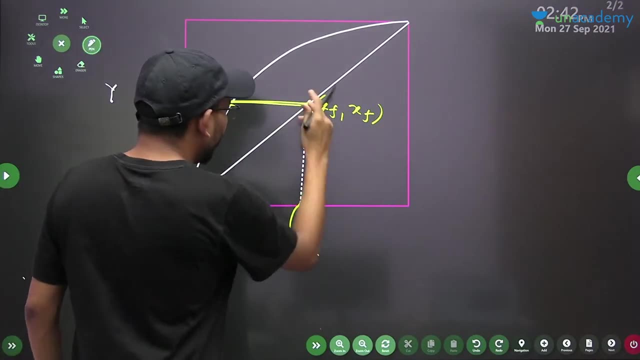 of light components: okay. mole fraction of more volatile component in the feed. you can see that Now you have to pull the slope from this line. If you do not have this slope, then do this: Okay, and you can draw this slope from here, because the condition of the feed will be. 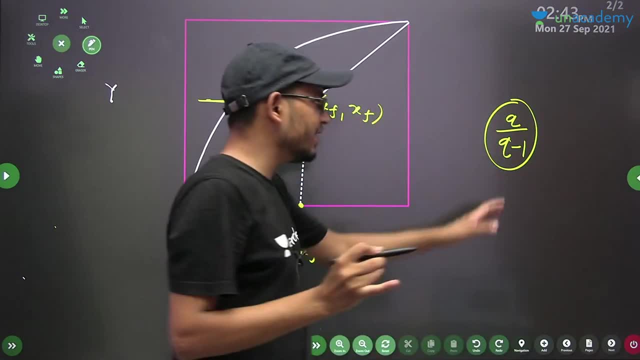 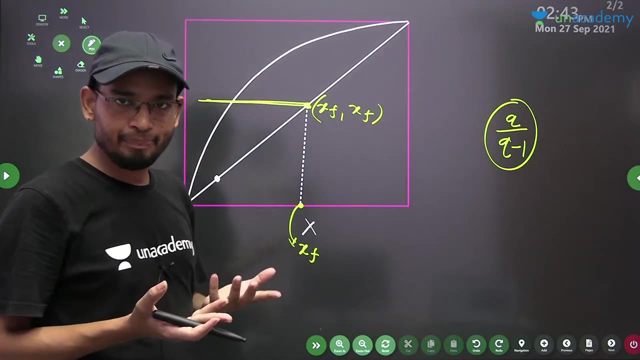 known, then q minus q, q upon q minus 1, you will know this value. this is the slope. if you know this value, then you can easily draw the slope from here. there is no problem. okay, then you suppose that the slope of your feed line came. it was looking like that. 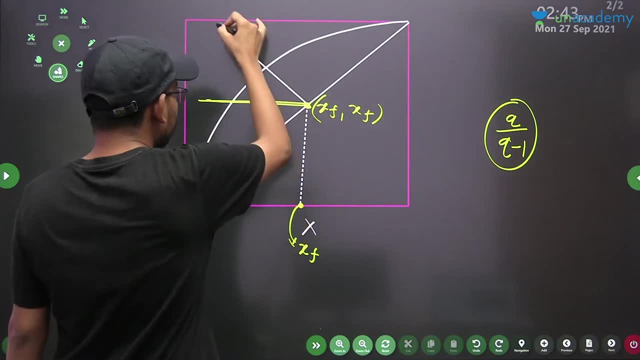 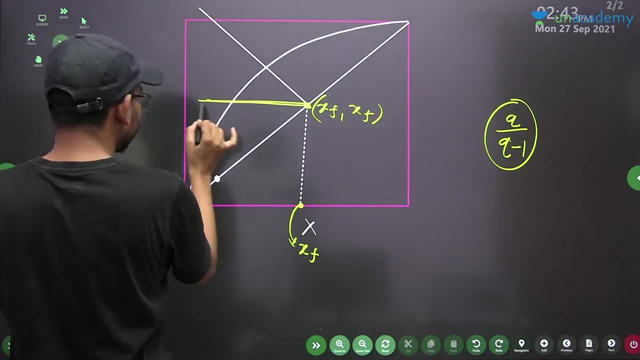 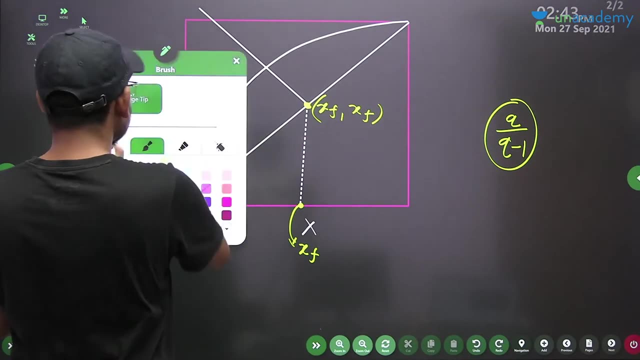 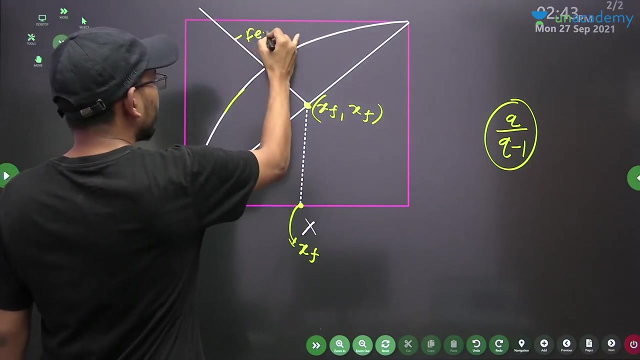 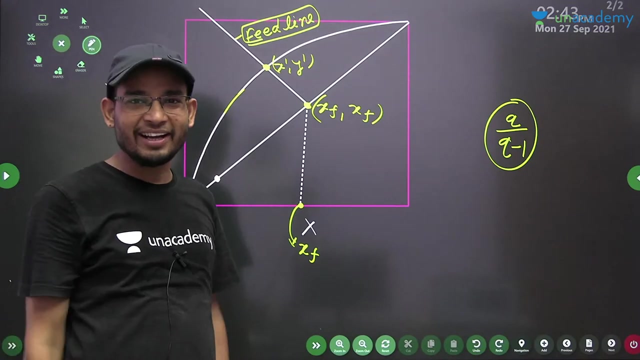 like this you draw the feed line. like this you draw the feed line. this is your feed line, this is the feed line. this is the point x, dash, comma, y, dash, equilibrium point. now you will see a slight difference in the minimum reflux ratio. now you will see. 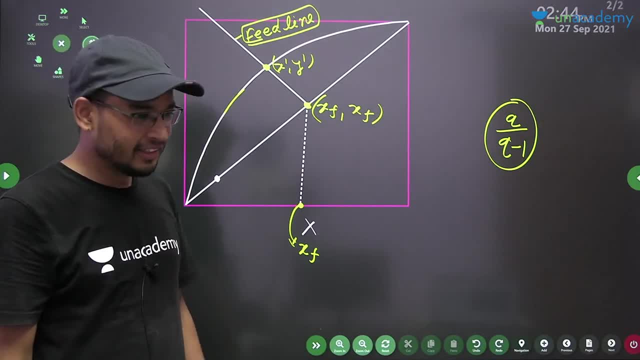 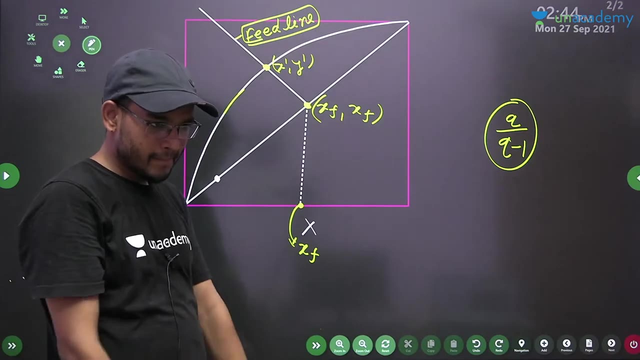 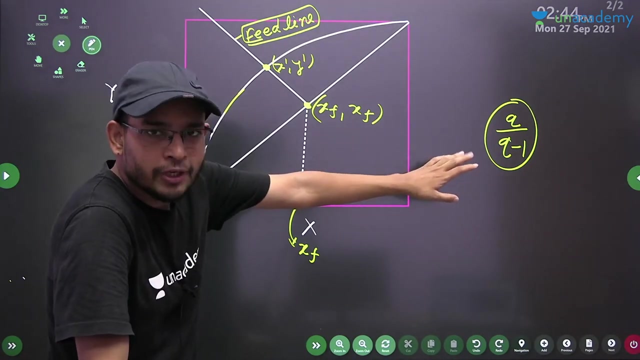 that you have reached the minimum reflux ratio. you have reached the minimum reflux ratio. yes, you can draw from angle and without angle you can draw from angle. you know the value of this slope. change the value of slope in degree. change the value of slope in degree. 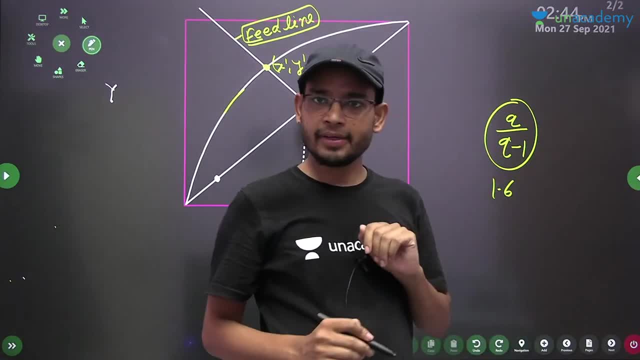 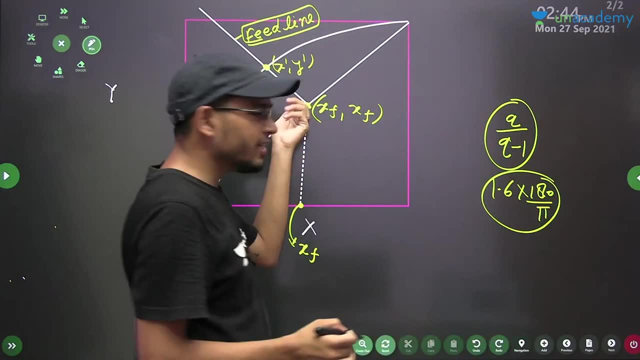 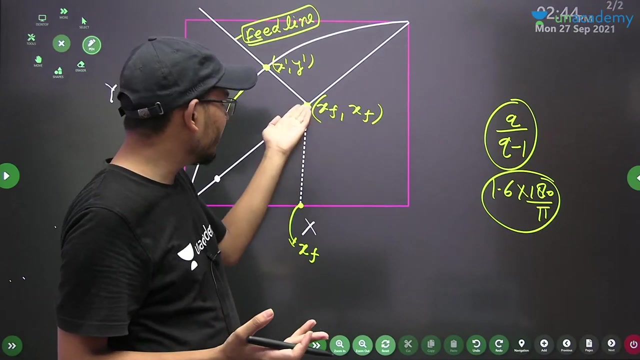 suppose this is 1.6. now this is the value. now this is one eighty divided by pi. now you can draw the slope in degree. if you want to take the value of degree, then take the value of 10 theta. then take the value of 10 theta. 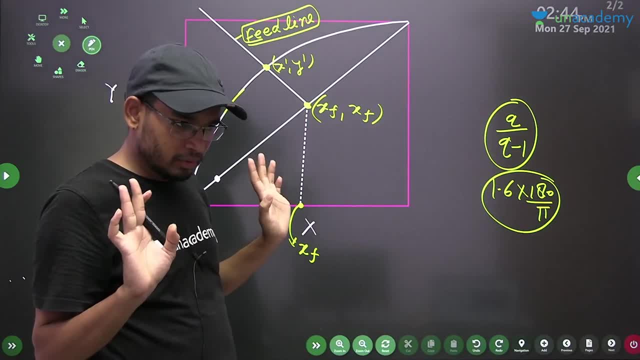 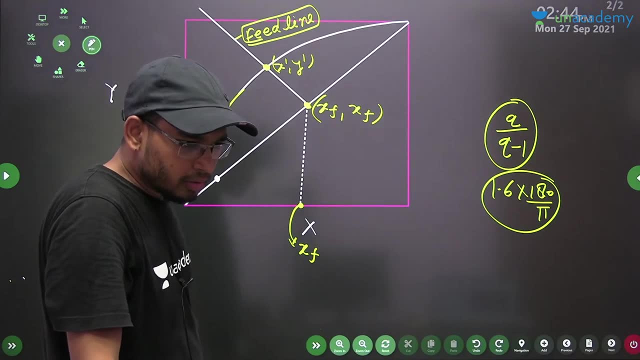 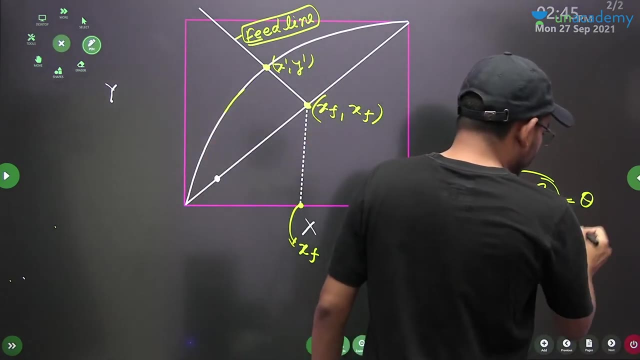 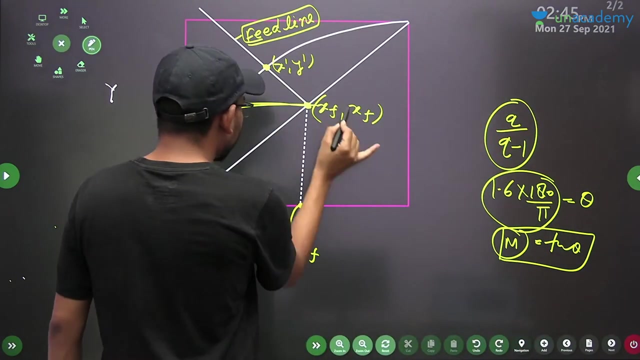 from here, no problem. ie, there is nothing in every set. what you have to do is to convert it to degree. suppose your theta is here now. what happens? tan, theta is there. this is your slope, so the value of m will come. now you have silver, you will keep it here and pull it. 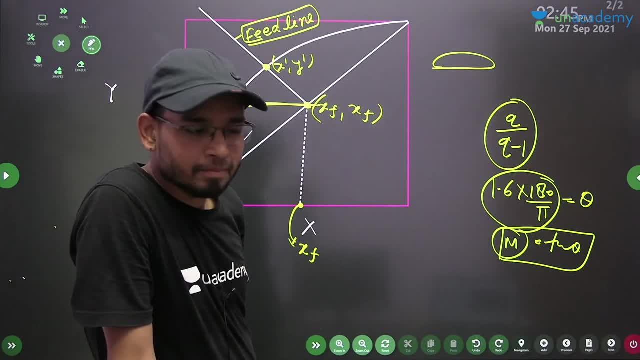 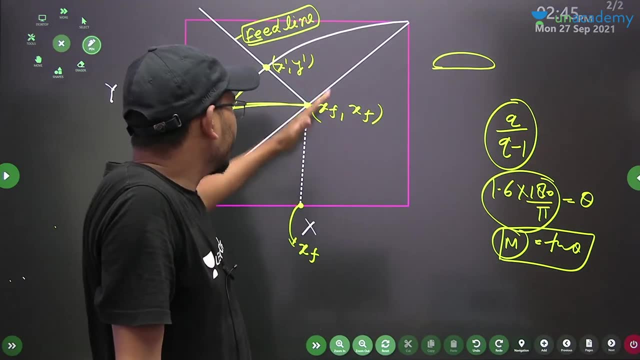 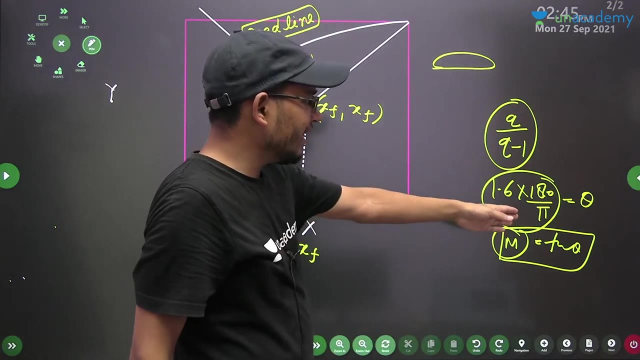 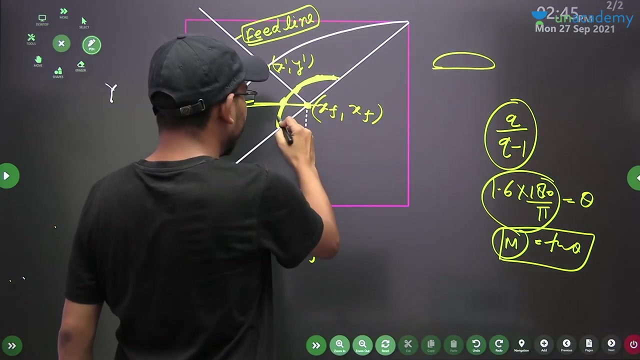 it will come. you will keep it here. here it is given in degree, so it is in degree. it is in degree, so it came in degree. it came straight in degree, so it has a degree in it: 45 degree, 60 degree, 30 degree. keep it here like this and pull the degree as much. 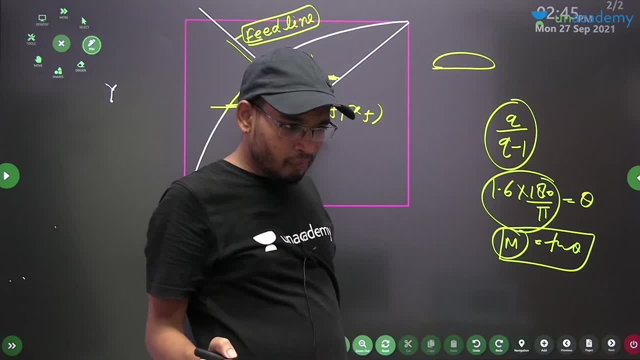 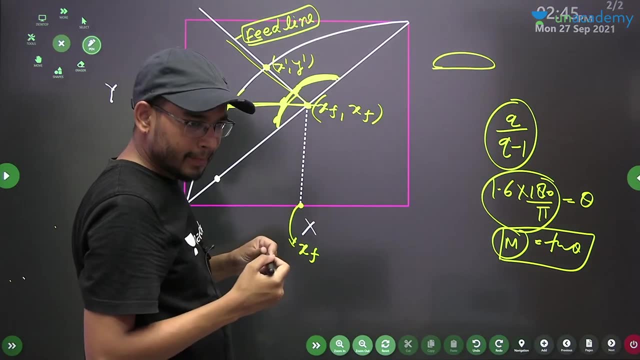 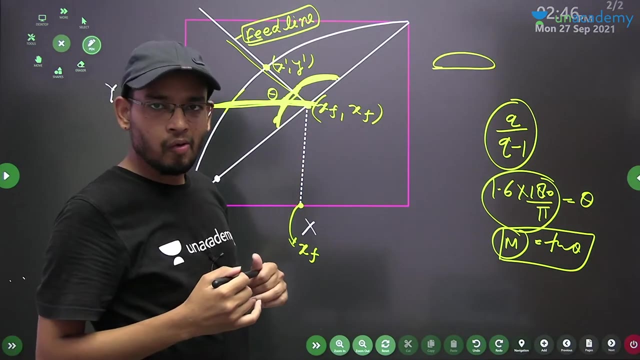 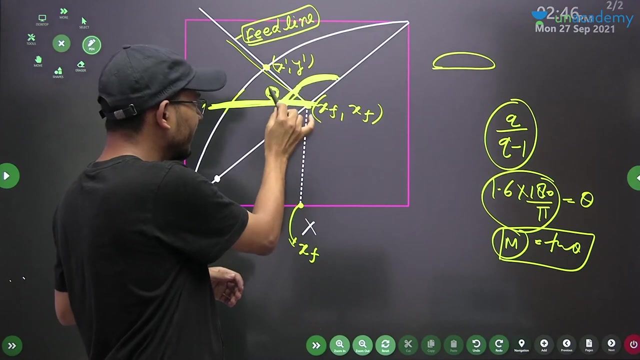 as possible. Oh brother, keep it on this straight, okay, and pull it from here. this theta will come. yes, it will be on x axis. this theta, this is the theta. alright, this theta, it will decrease like this: this is the theta from horizontal: the angle that will be made from. 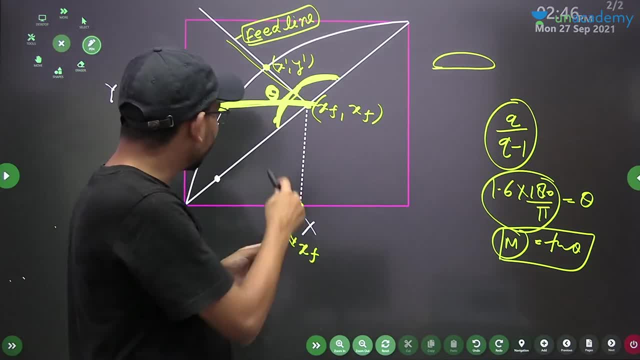 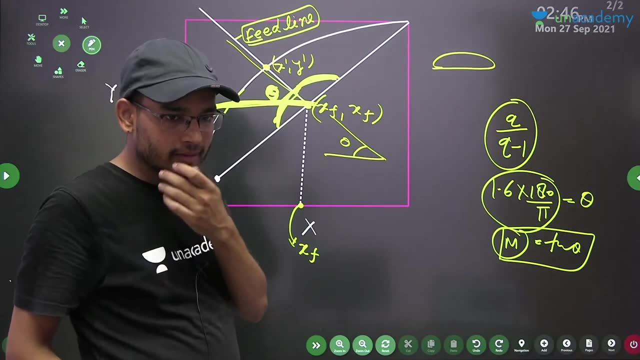 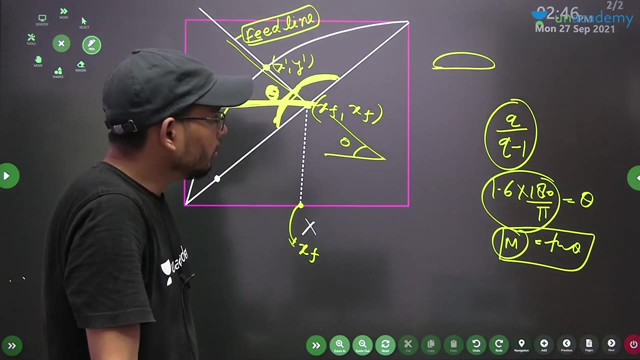 horizontal. this is called slope, the angle that will be made from horizontal. this is the slope. okay, this, this is the theta. okay, fine, now the process will go further. now, the process will go further. now your long mean there are many large lectures, okay. 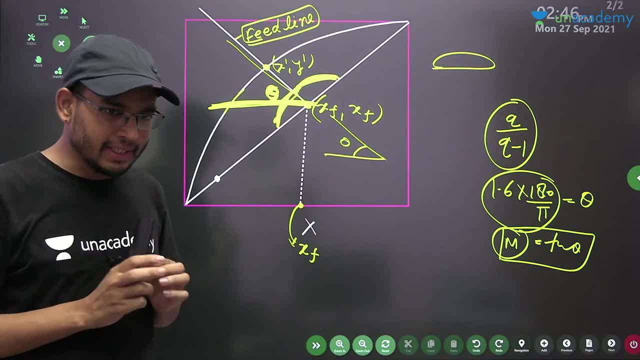 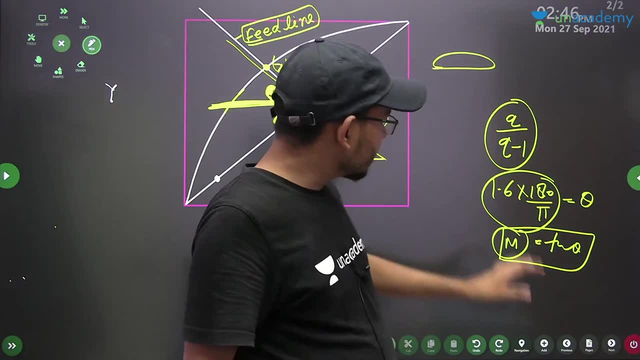 hopefully you will understand that you have come here to understand. till here you have come to understand. okay now, after this, we will continue tomorrow because our time is over. okay now. we will continue tomorrow because our time is over. okay now, if we. 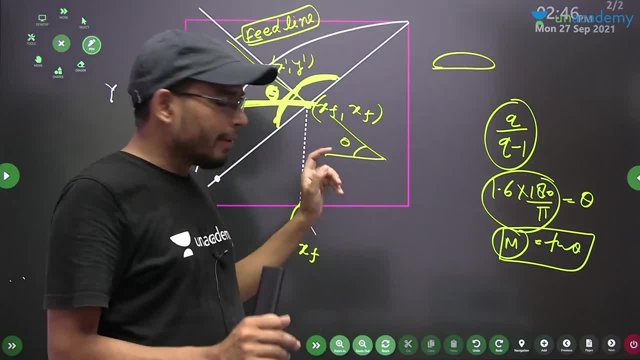 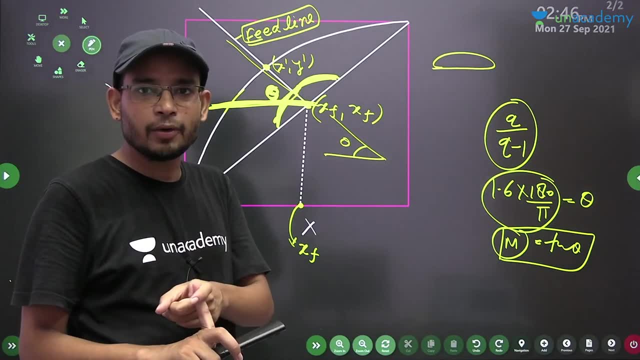 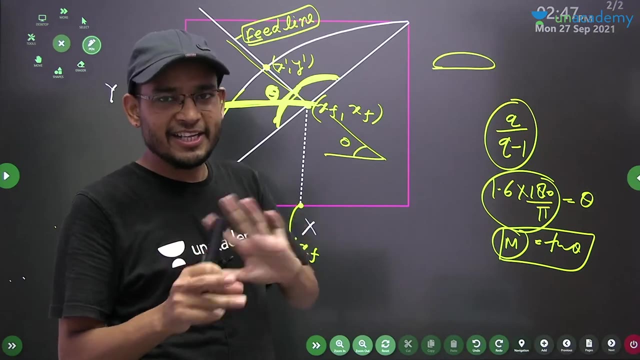 After minimum reflux ratio, you will decide the location of the tray. you will calculate the number of trays. you will calculate the column diameter. you will talk about beeping flooding, seep tray, bubble tray, cap tray. all these will come in the designing part. 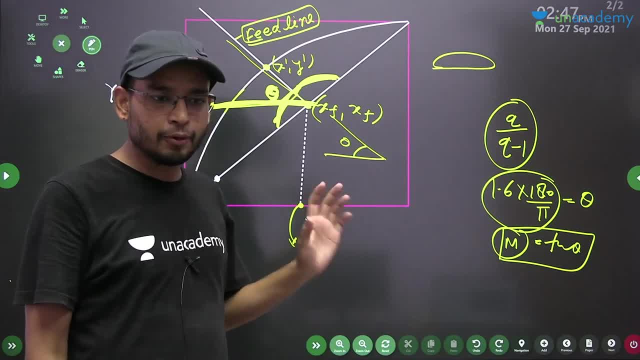 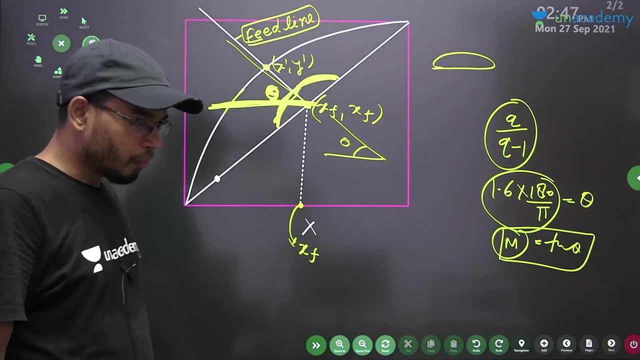 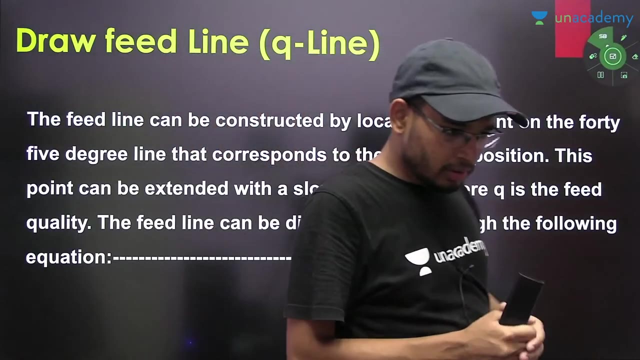 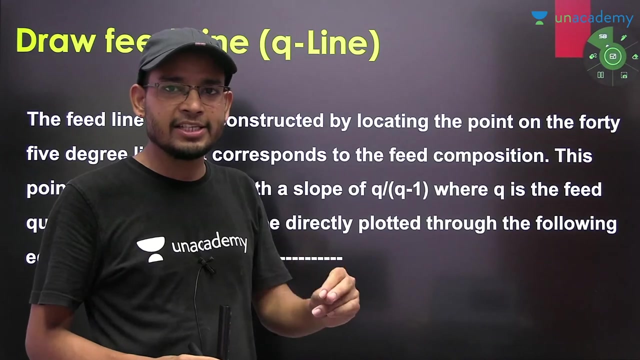 So the process will go on till here. you must have enjoyed till here, right? ok, fine, so we will keep today's session till here. tomorrow will be the same time. tomorrow will be the same time. this designing part will go on till it is not finished. it will go on for 3 to 4 days. it will be finished, ok, in the same time. 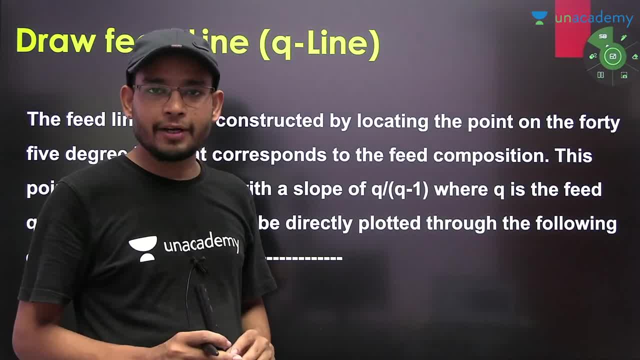 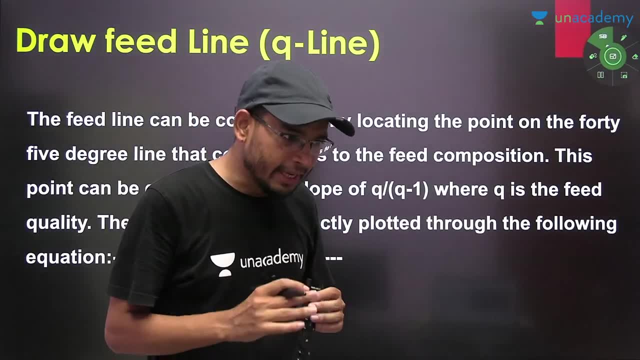 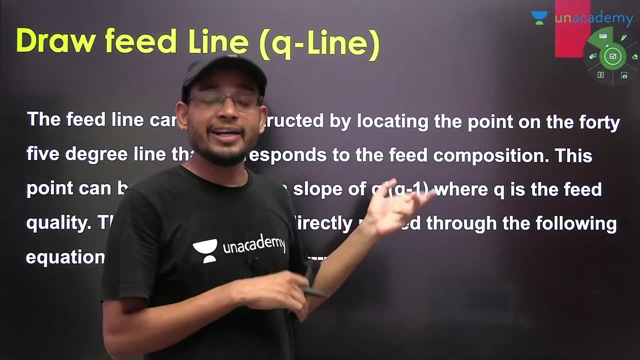 ok, in the same time. ok, in the same time. I hope you must be enjoying it. ok, in the same time, and you share the message so that everyone sees this thing. ok, these lectures are very important. these are the importance now. you will know about it in future. ok, this main game will change you. 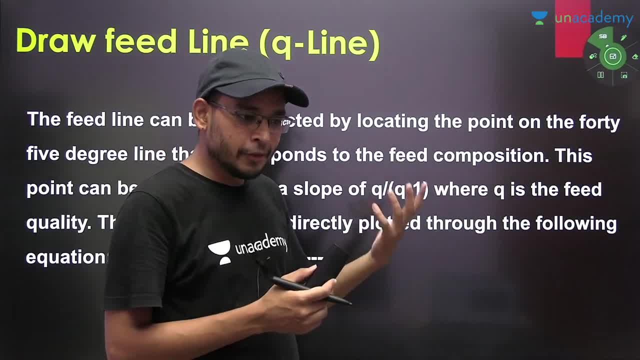 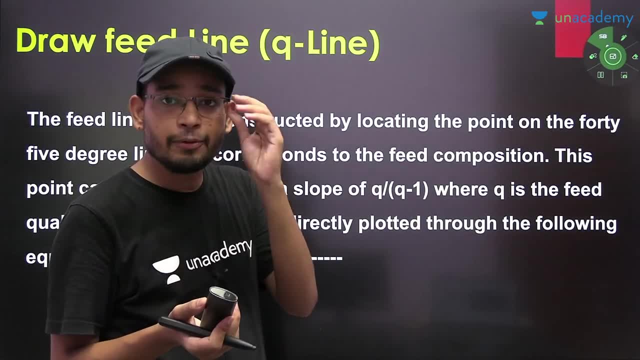 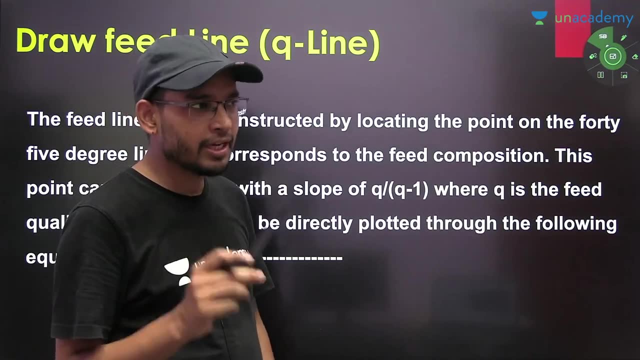 In case you have taken these things very well, then I will do all the design for you. this is very helpful. in case you have good feedback and you have enjoyed it, then I will do all the design for you. I will do evoperator design, heat transfer design. 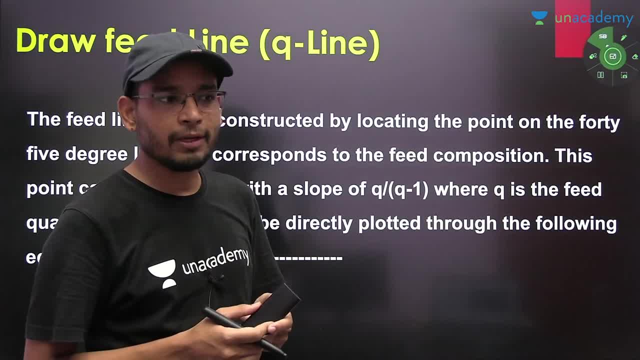 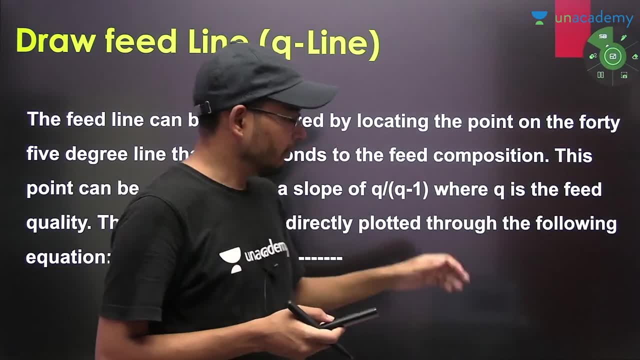 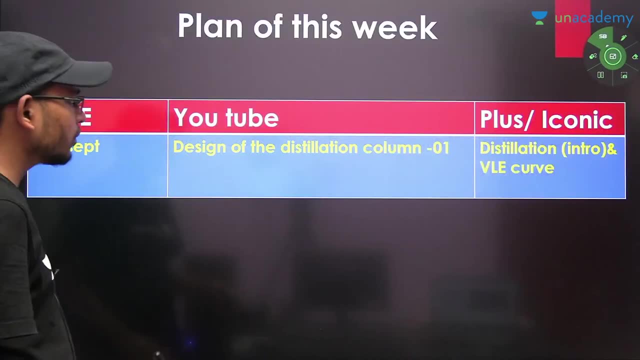 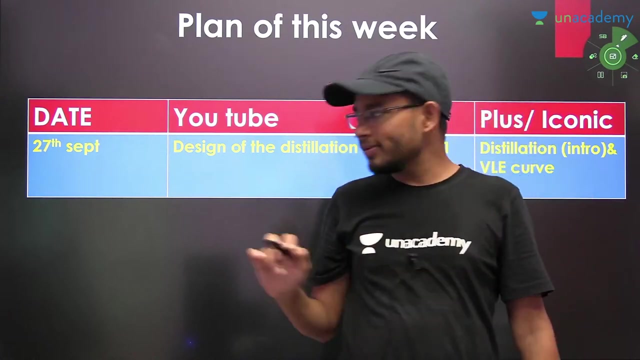 absorption column: I will do design for that. extractor column: I will do design for that. ok, then we will keep this session till here. this was all part. we will complete it tomorrow. tomorrow, your class will be at 9 in the morning. ok, your class will be at 9 in the morning. 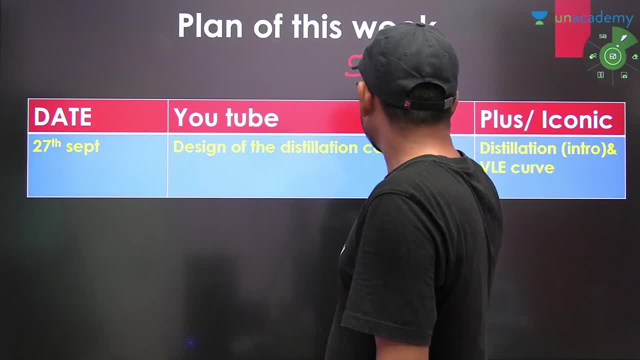 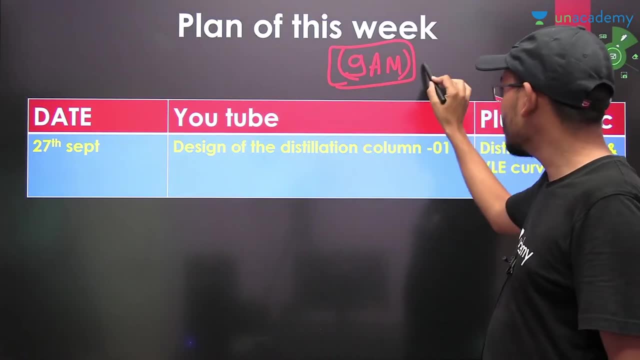 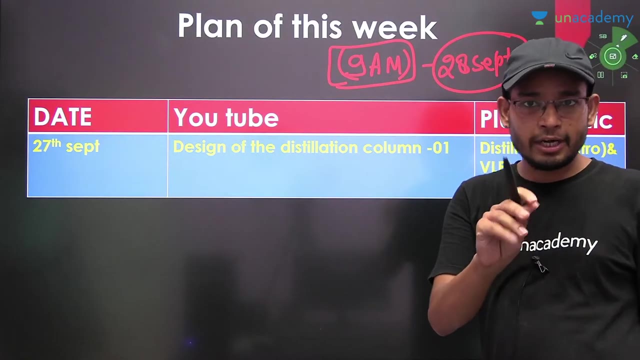 in which IPC revision session is going on. ok, at 9 am. at 9 am tomorrow, your class will be ok. tomorrow, tomorrow class will be in the morning. ok, so I will give the link to all of you in the evening. everyone will be added to the group. 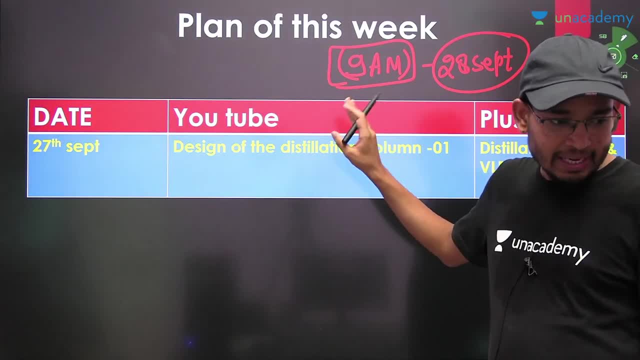 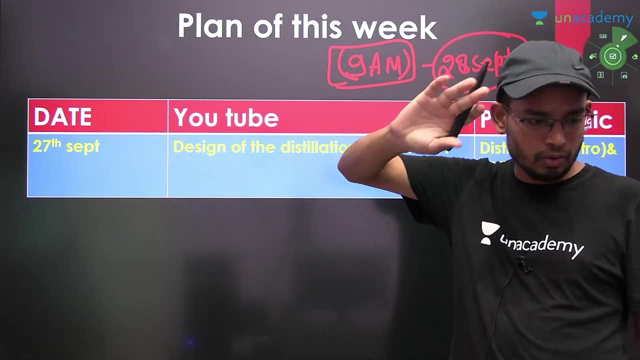 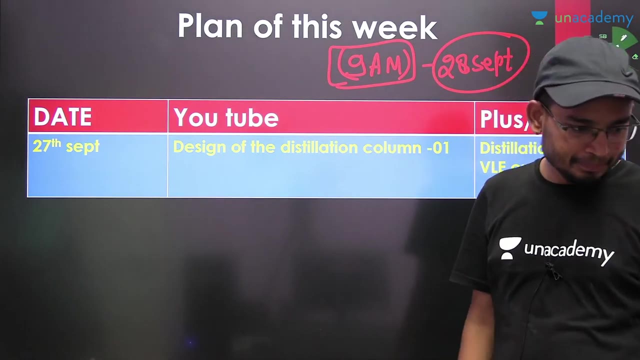 you can see it today. ok, you can see it today. tomorrow will be in the morning. tomorrow will be at 9 in the morning. in the morning I will continue the revision session of IPC. ok, I will keep the revision session continue. I will do it in that. 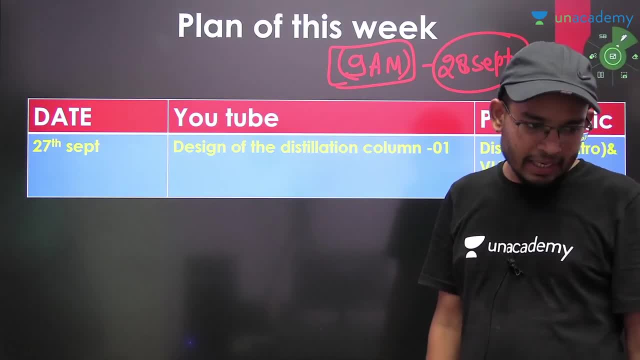 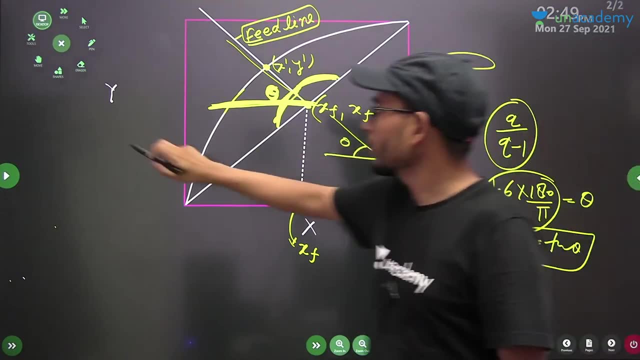 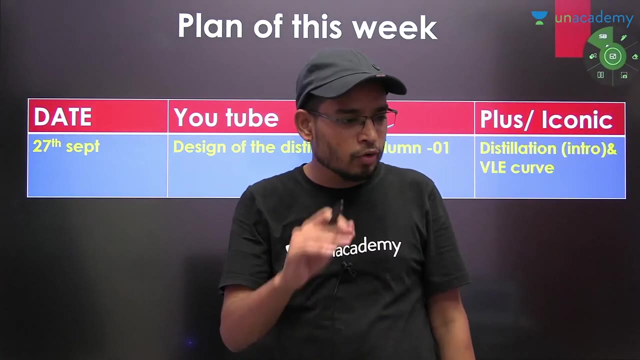 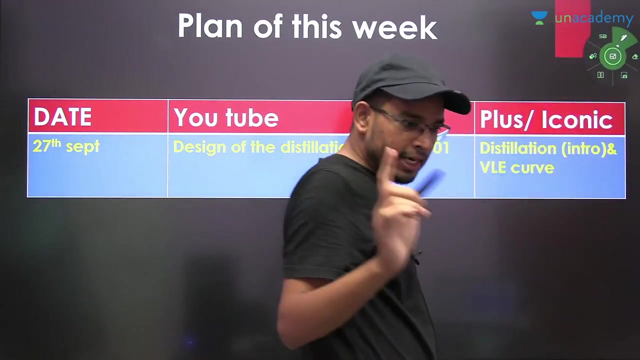 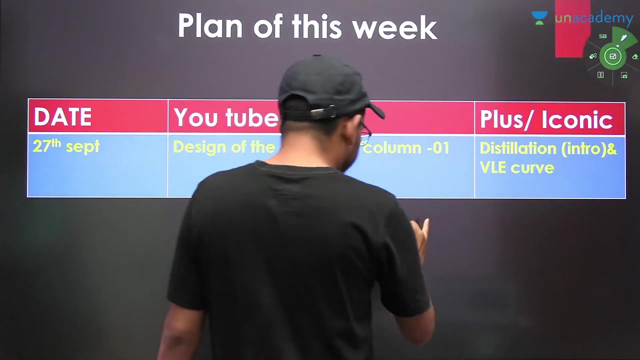 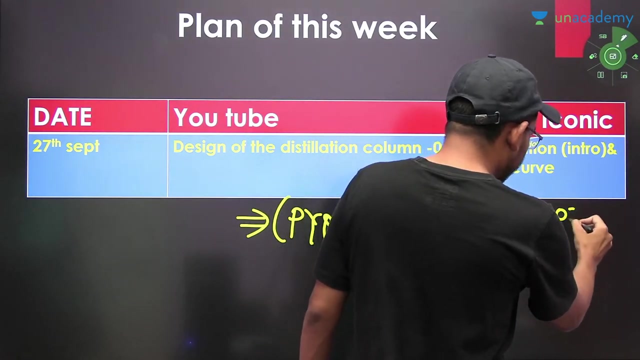 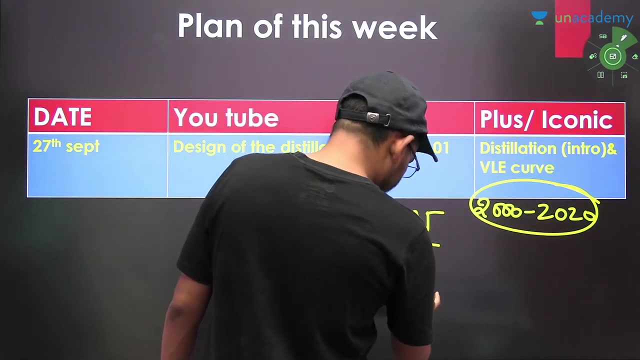 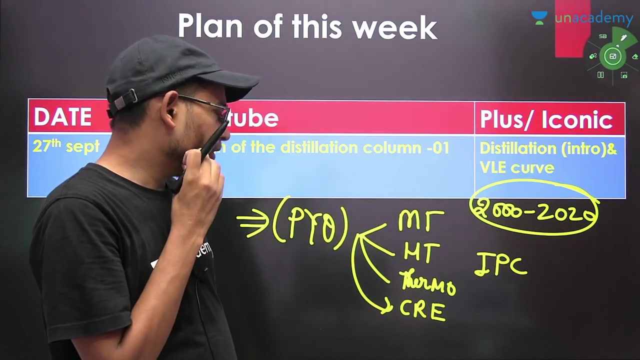 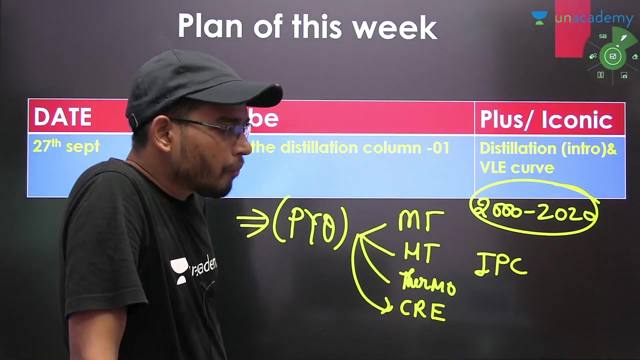 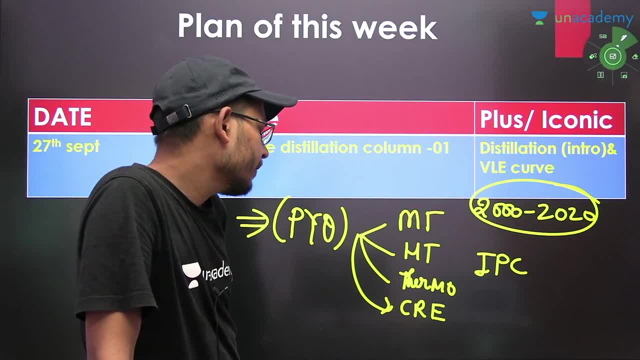 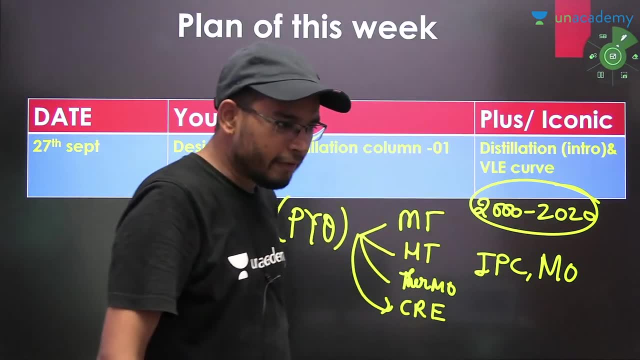 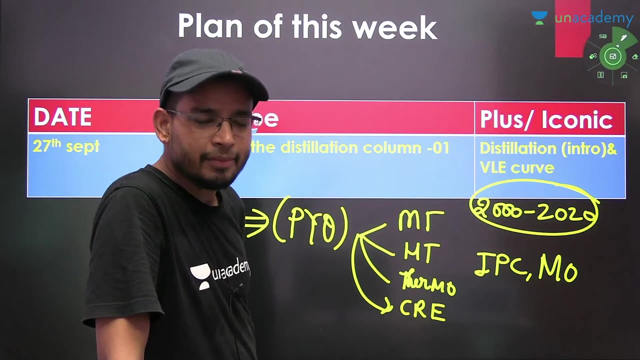 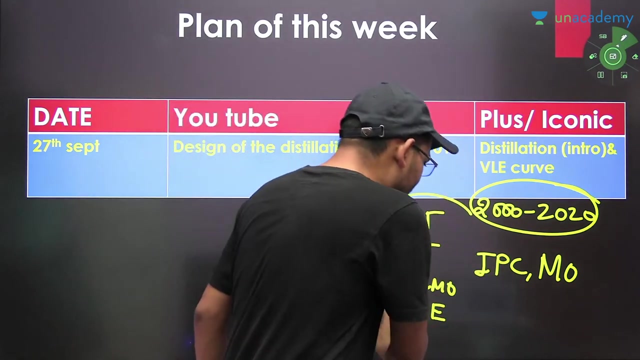 one more subject is left: mo one mo. fm's side is not there, it is of mo. fm's side is also there, so it may be of fm. it is not of fm, it is of mo. so I have given you so many subjects with answer key. 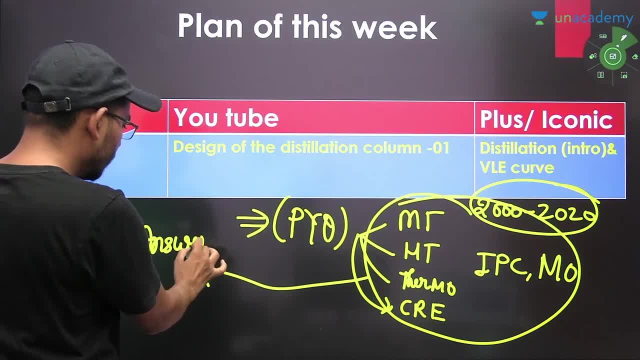 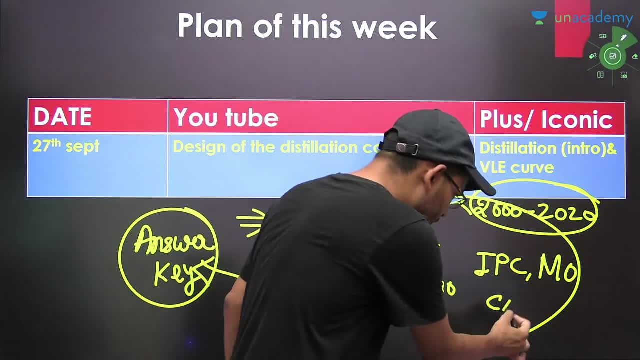 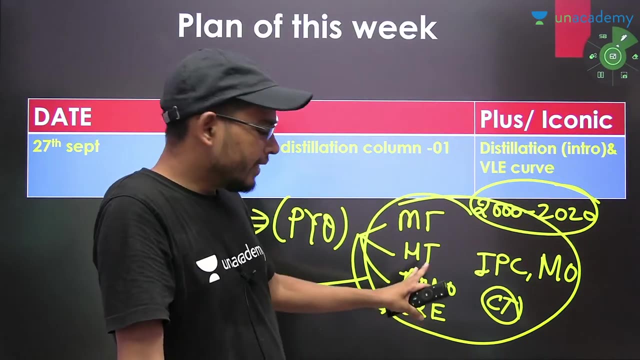 answer key is also available at the back. answer key is also available. everyone will see it. answer key is also available at the back. it is also of ct. it is also of ct. answer key is also available at the back. everyone will see it. ok, this work was going on for last 2-3 months. 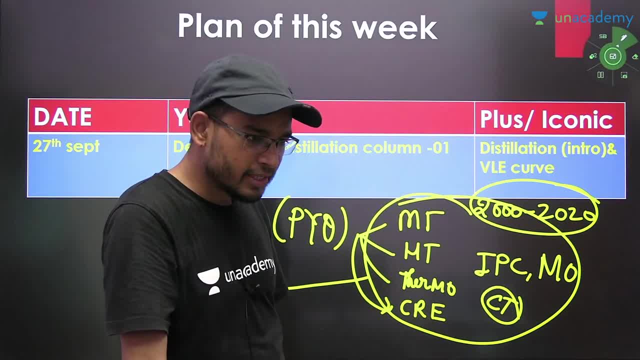 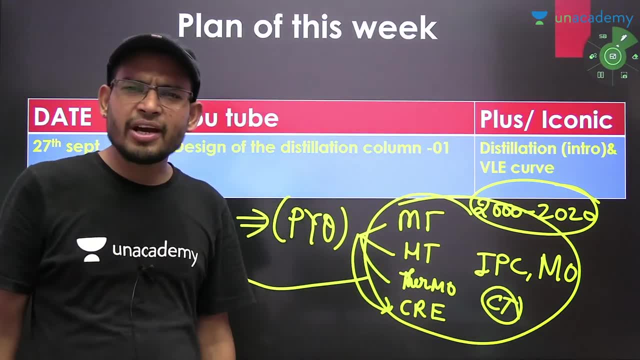 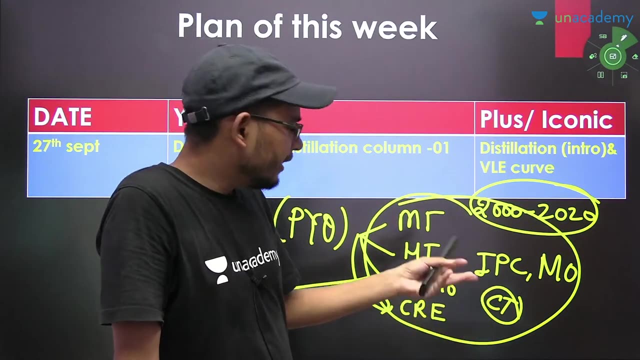 so it came yesterday. I have sent you, like it came to you, ok, 7 subjects. so ct will also be included. ok, math and ft are accepted. math and ft are not needed. almost all of them are accepted. PC and PD are not of ct. you will also need PC and PD. 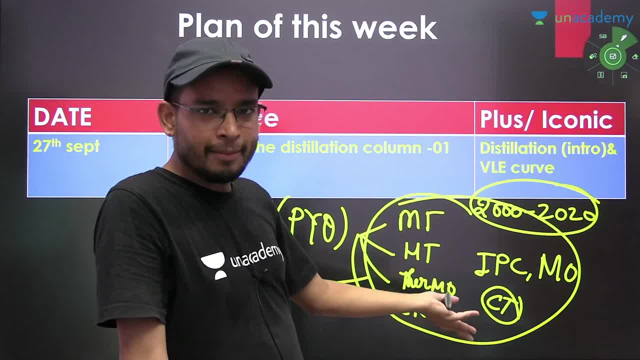 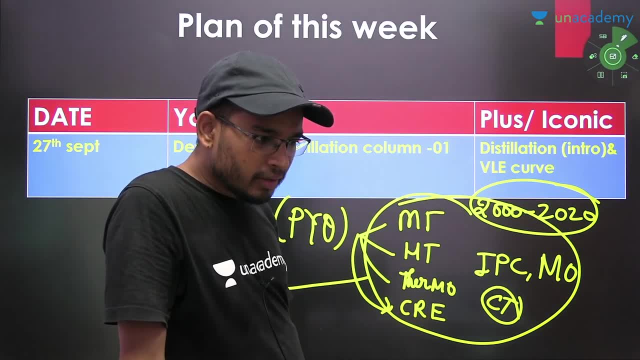 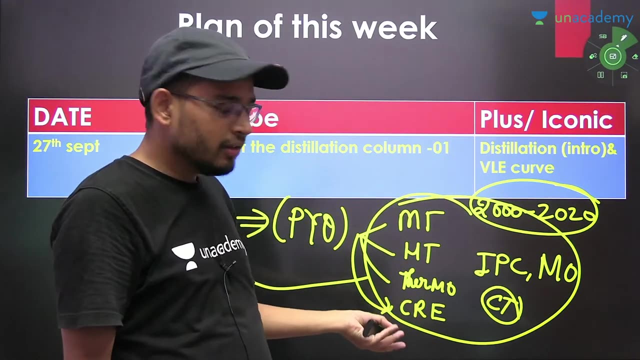 so I will give it. it is not of any use. i have given you the main subjects. i have given you the main subjects. ok, the answer of PYQ is KUNAL. you just collect. if you add in the group of Manish, sir chemical engineer, then you will get it. 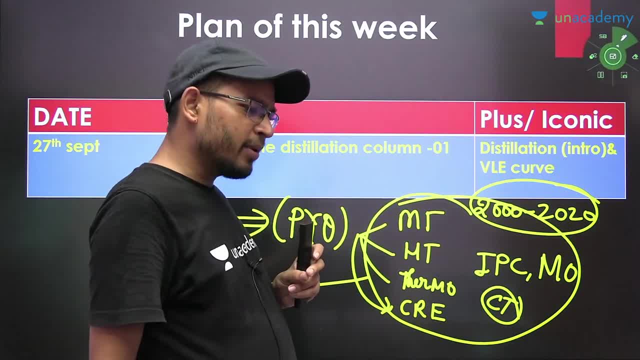 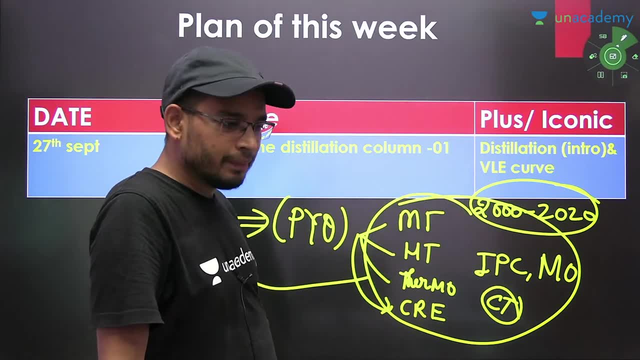 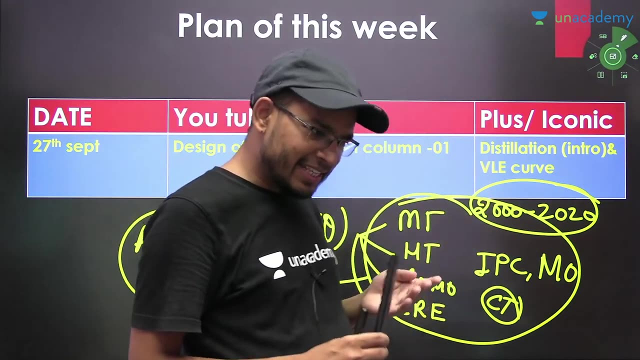 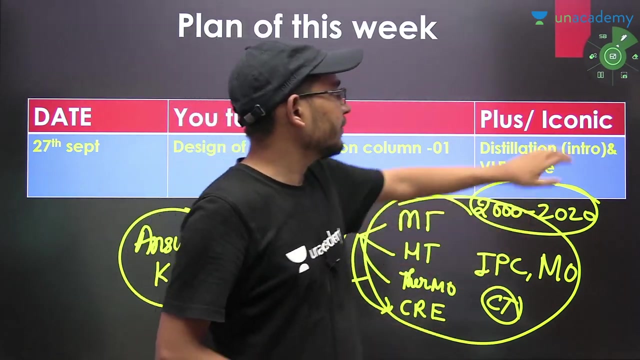 FM is left, we will give FM also FM also use it and if you don't have it, then sell it. it is not of CRE. it is of CRE. it is of CRE KUNAL. you don't know where it is. I have sent it yesterday. it is of CRE. 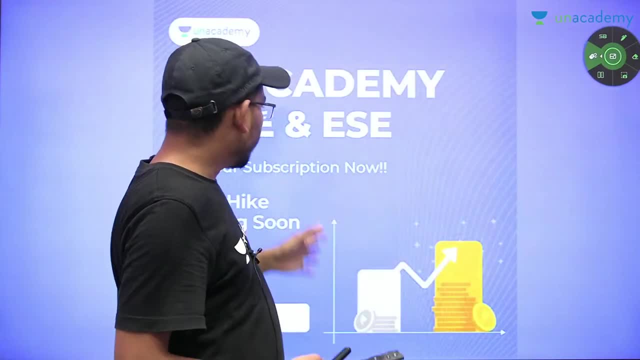 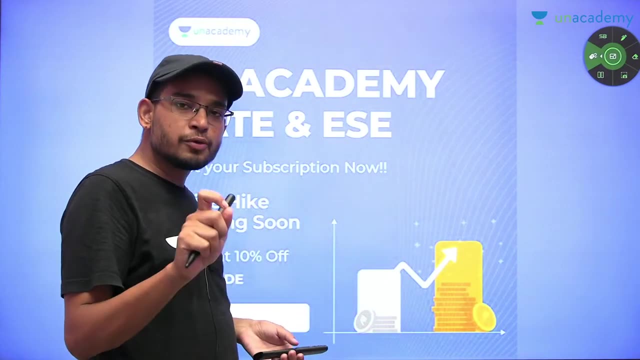 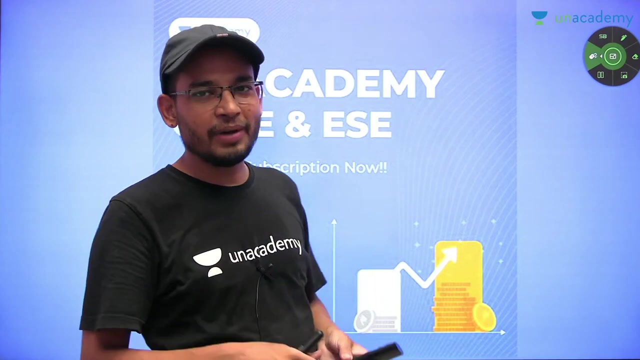 and if you want to join, then you can join. the fee is going to be high. so all the students of YouTube are thinking a little. they are also going in plus and minus. so join in plus and quickly go. what can I tell you? come and understand, friends. 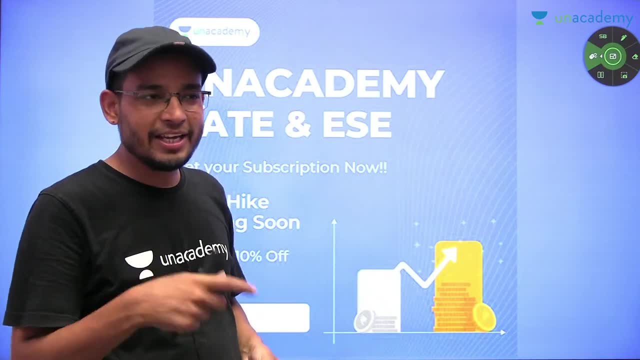 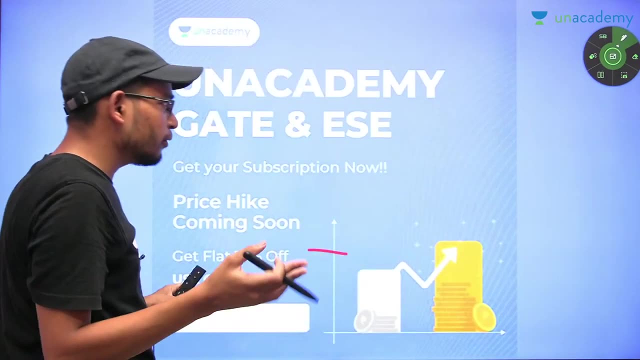 ok, now invest as much as you can for your career. ok, even if you take a trace once, no problem, but you can invest for your career. then you can also do it from YouTube, whatever you want. ok, I think that by taking plus, I think that the students of plus 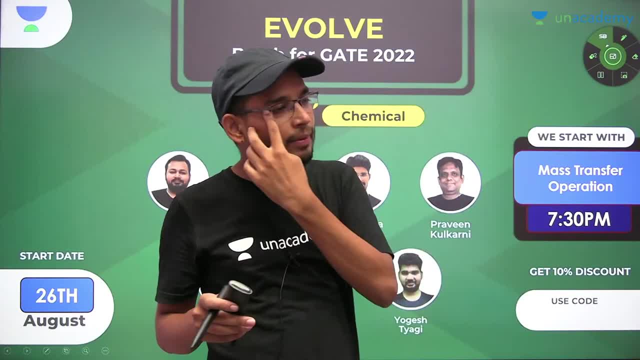 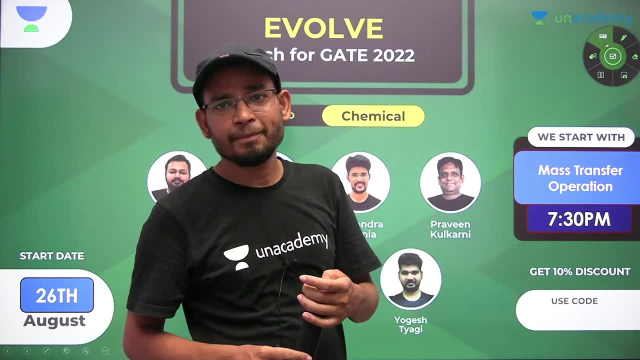 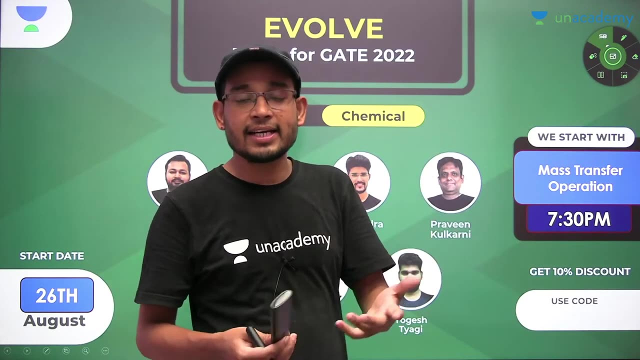 then I take any session, I take plus. there are also children of plus and there are also people of plus and there are also people of YouTube. so I see that there is a better response of people of plus. this is my personal observation till now. ok, so you can see that the comments that come, the answers, come quickly. 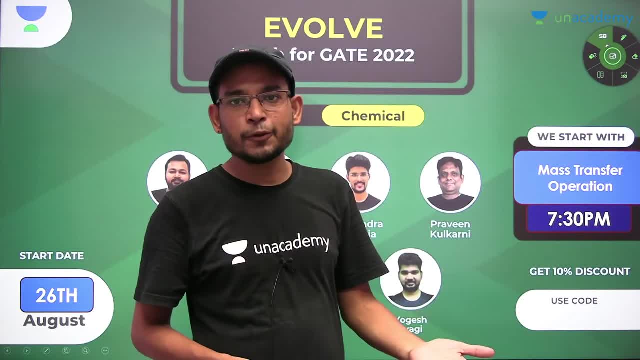 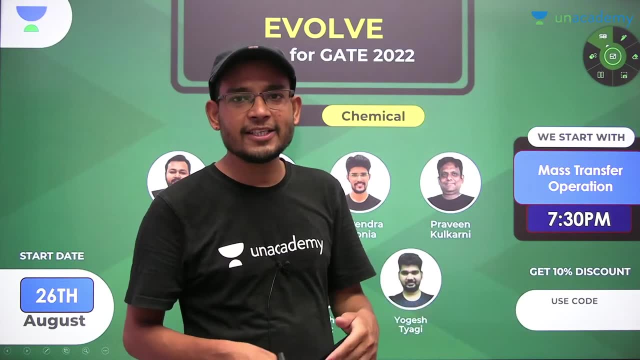 they come from the students of plus because their subjects have been completed very early and they have done revision many times. ok, so the more you do revision, the better your subject will be. so this is the advantage. so if you want to join, then you can move with it. 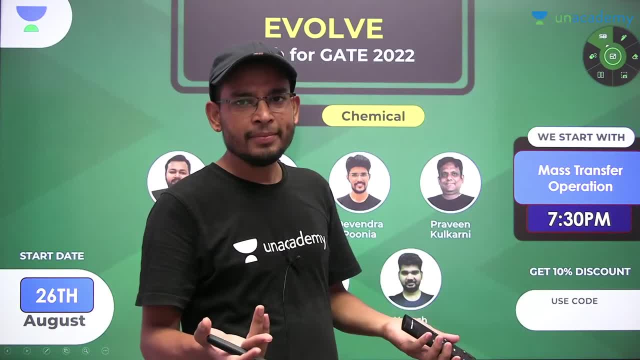 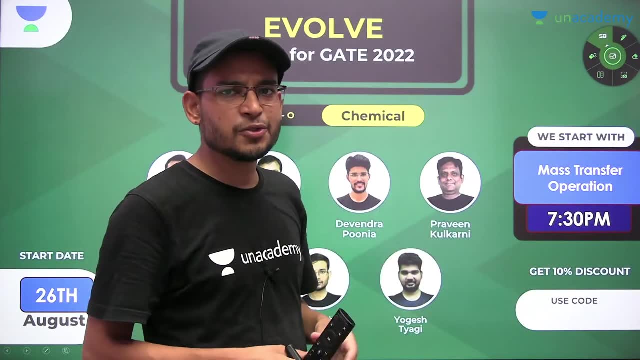 ok, otherwise there is no problem. you can also move from YouTube. and those who think a little that I don't want to play in plus and minus, ok, if you want to make a mood once, then you can join properly. ok, you can contact me. if you have any problem, then you can contact me through the Unacademy app. 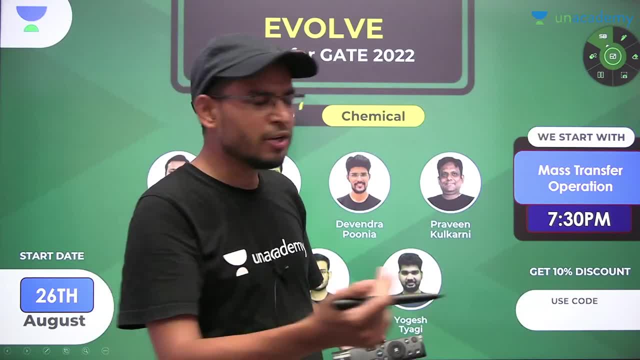 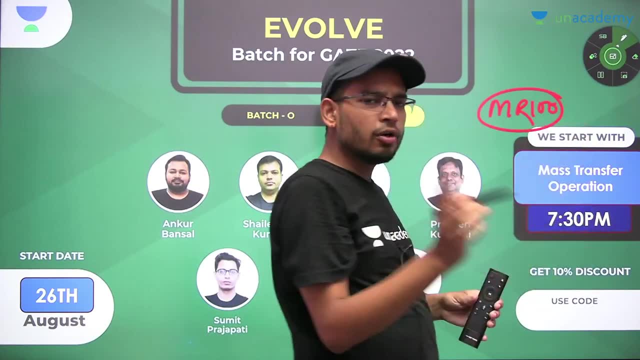 if you want to have a discussion, you can have a discussion. you know my code, so if you want to take a course, then you can use the code. ok, if you want to take a course, then you can use the code MR100. those who also want to move with it? then you can move. 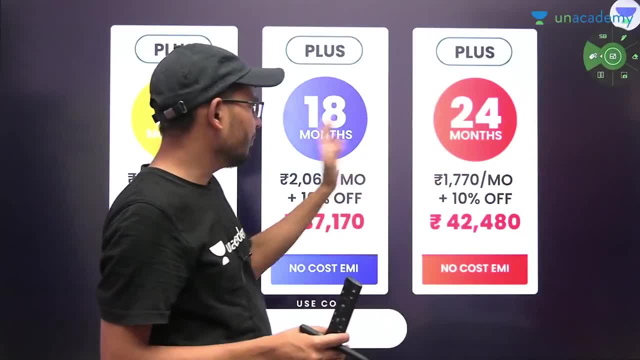 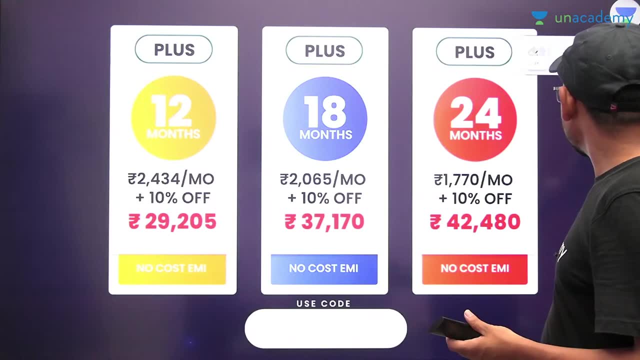 ok, save time. the main important thing is to save time and move forward for 12 months, 18 months, 24 months. the structure is shown here. those who also want to join, then join. ok, if you want to join, then you will have to keep the fees structure here. 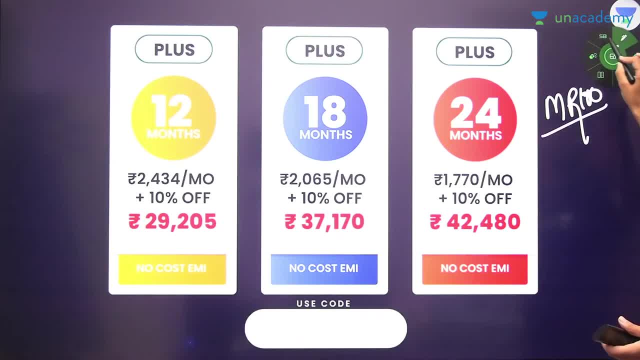 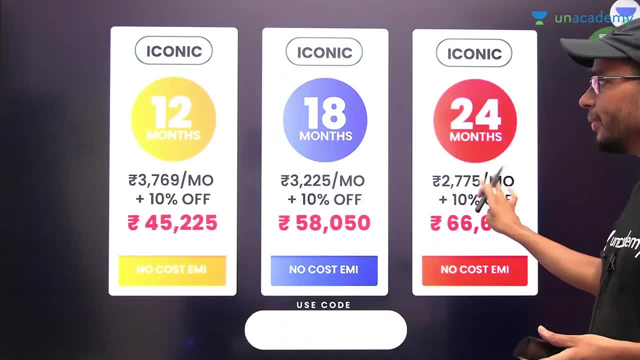 don't forget to use the code, that is the MR100. right go now. after this, I will talk about Iconic. keep the fees here for Iconic, and this feature has been launched by the Unacademy, in which you can ask any doubt by mistake. 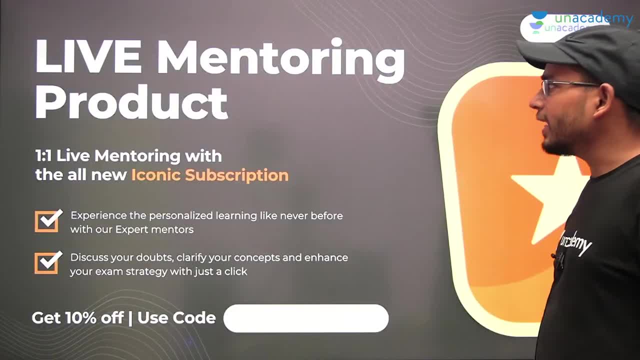 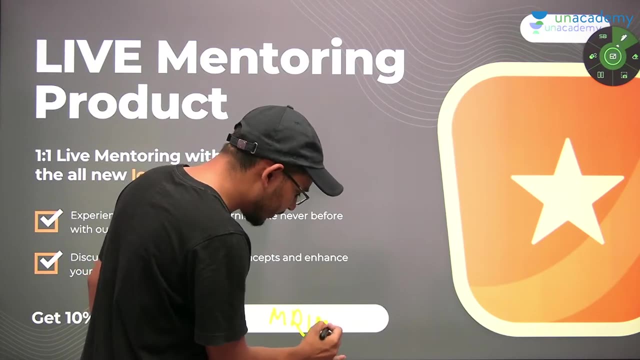 how many doubts you can ask. then you can join here. this is the live mentoring product launched for you. this is for Iconic subscribed students. ok, so here also, you have to take help from this and use it. and to clarify your discussion properly, then you will use the code MR100. 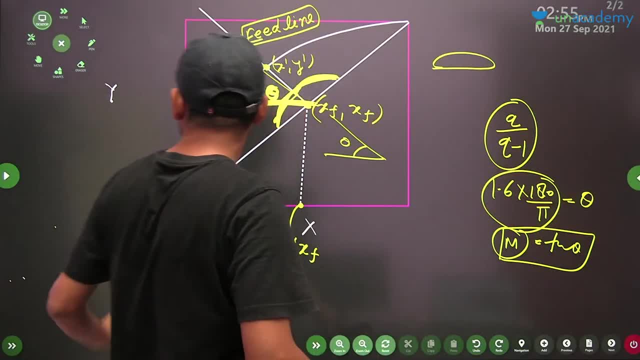 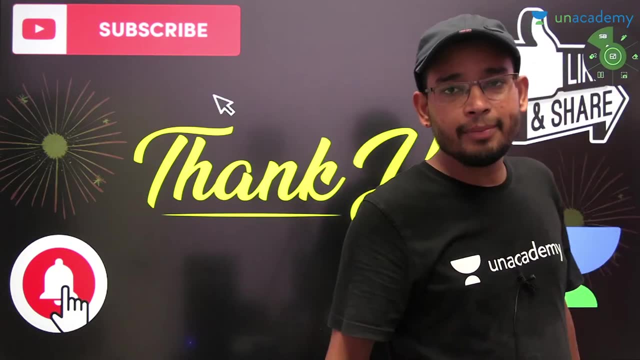 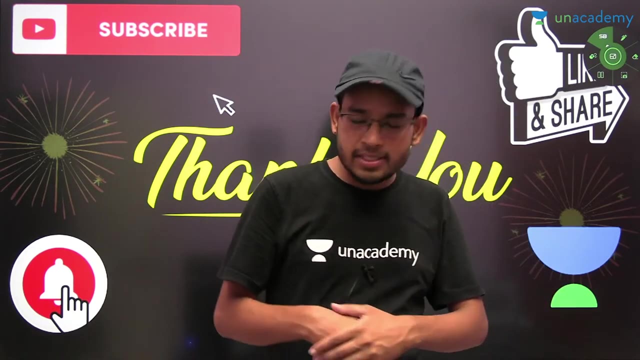 ok, let's go. so thank you so much. see you tomorrow in the morning at 9 am. ok, at 9 am and at 1 am. this is our continuous class. ok, teach HT and solution thermo. yes, in the next session you can also get HT.